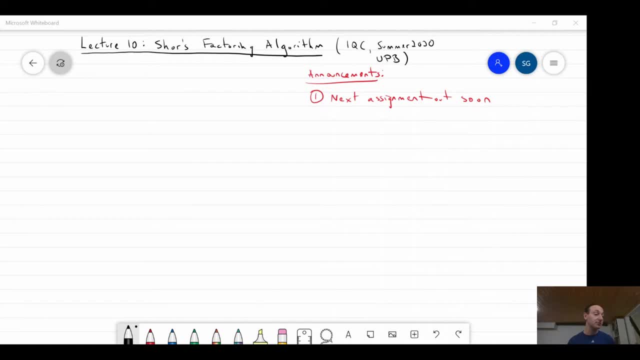 it caused or forced the classical computer science community to really reevaluate one of its core assumptions. Okay, so which assumption are we talking about? Well, essentially, at that time, the problem of factorizing large integers. basically, so, if I give you a large integer n, can you factorize it into its prime factor? 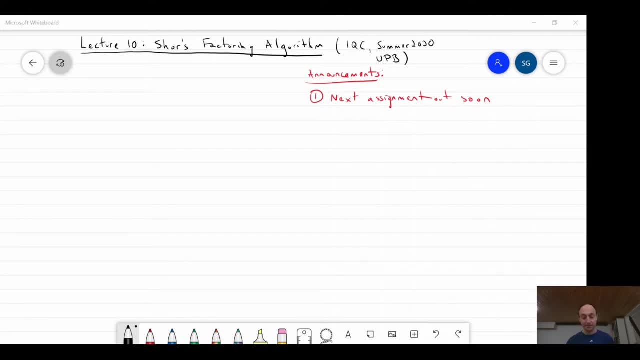 Can you factorize it into its prime factor? Can you factorize it into its prime factor? That problem was believed to be hard for a classical computer. Okay, And in 1978, Rivest, Shamir and Edelman came up with a cryptosystem, or cryptographic scheme. 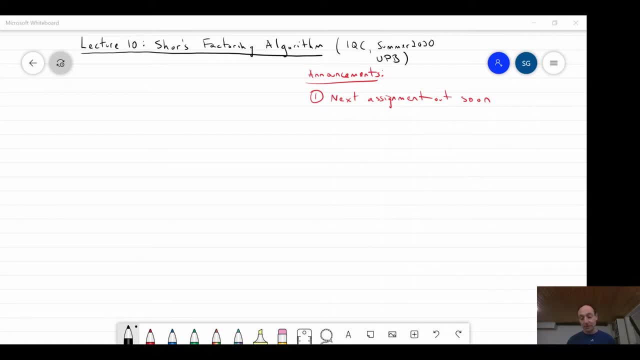 commonly now known as RSA after the founders, which basically is remains widely used in practice. right, It's used to basically secure data online. Okay, And you know, RSA had been presumed secure basically since its inception, because people believe factoring was hard Okay. 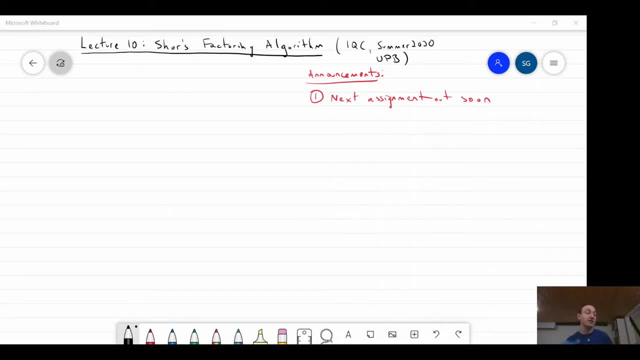 I mean, let's be clear that even in- I mean just looking at, of course the algorithm makes it clear. the RSA algorithm makes it clear that factoring will break this thing. But you know, even in the abstract of the paper it was very clear what the assumption is. It read, you know. 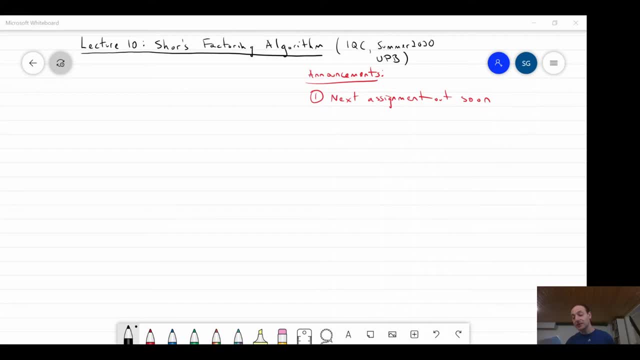 here's a quote from the abstract. you know, the security of the system rests in part on the difficulty of factoring the published divisor n Okay. so in some sense it's an Achilles heel that's hiding in plain sight, if you will, right. And so you know. lo and behold in 1994, you know. 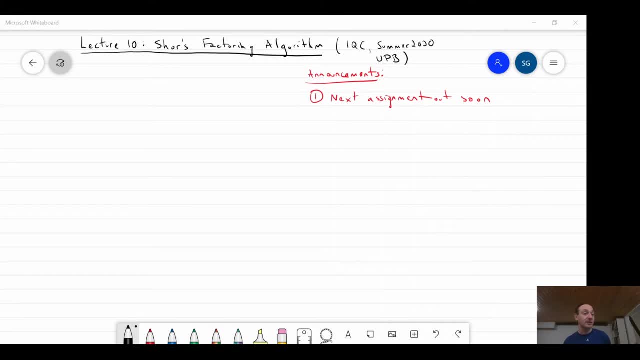 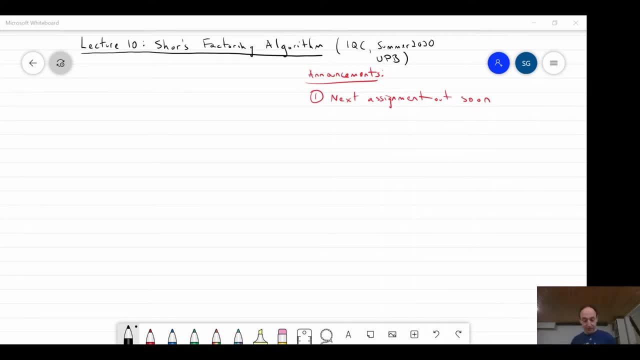 very popular crypto system, RSA. Okay, so that's why we're going to talk about the factoring algorithm And that's roughly why it's so important. So in this lecture, of course, we'll talk about the algorithm And at the very end I'll briefly go over. you know how you. 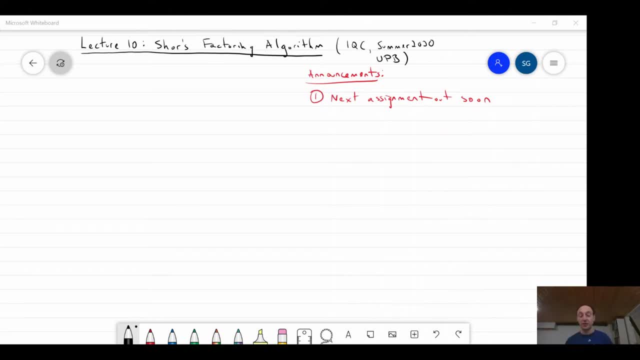 use it to break RSA, Okay, and in particular that means reviewing RSA very quickly. The factoring algorithm itself. it can be thought of as having kind of three steps. The first step is you're going to not actually solve factoring, you're going to first reduce factoring to. 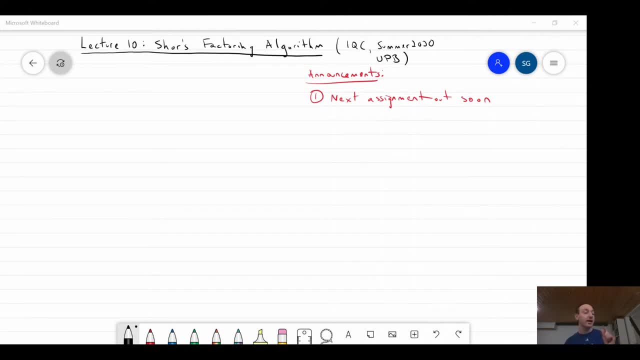 something called order finding and then you're going to solve order finding And order finding. to solve that we're going to need two things. we're going to do a sampling step using the quantum phase estimation And then we'll have a classical pulse processing step using something. 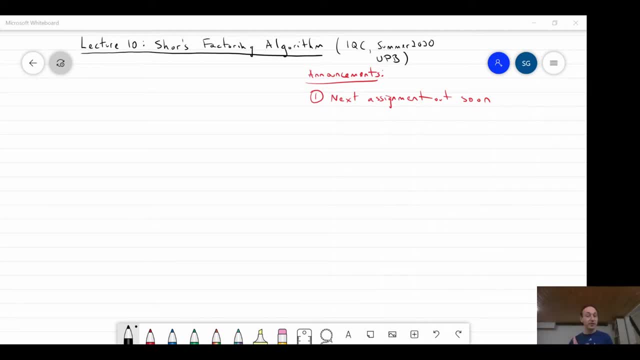 called the continued fractions algorithm. So before you're doing any of this- however- okay, we're computer scientists, that means we'd like to be formal about things- we should start by formally defining what we mean about the integer factorization problem, And we should. 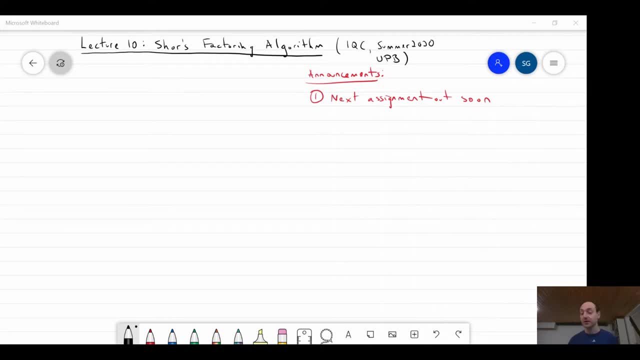 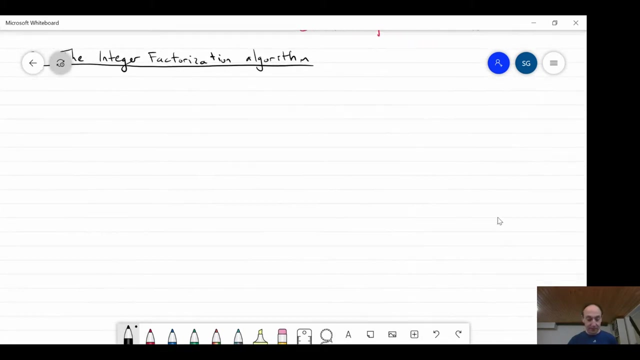 understand the complexity theory context of this problem. Okay, before we talk about any sort of algorithm for it. Okay, so section two of the notes is just basically the integer factorization algorithm. Okay, Okay. So, as you guys probably all remember from your math classes, basically in university, 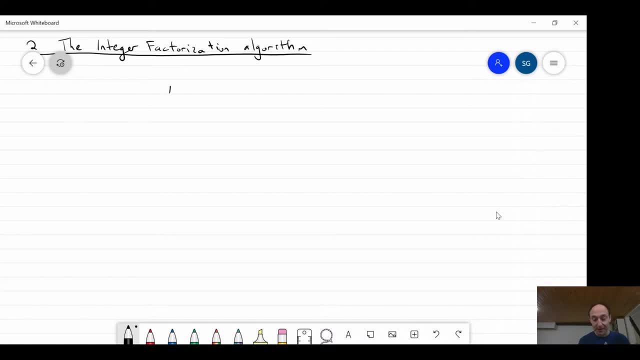 the fundamental theorem. arithmetic says that if I give you any composite number, n right some integer, I could always decompose it into its prime factors right. So P1 to some power, k1, P2 to some power, k2, dot, dot dot, Pm to some km. 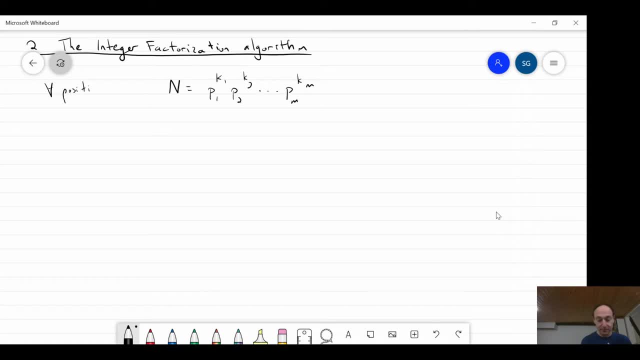 So this is for all positive integers. n Okay, so maybe I'll write z plus to the positive integers. We can always write n this way, right? And you know each of these pi's. these are all primes, Okay, and of course you have some multiplicity for each prime. 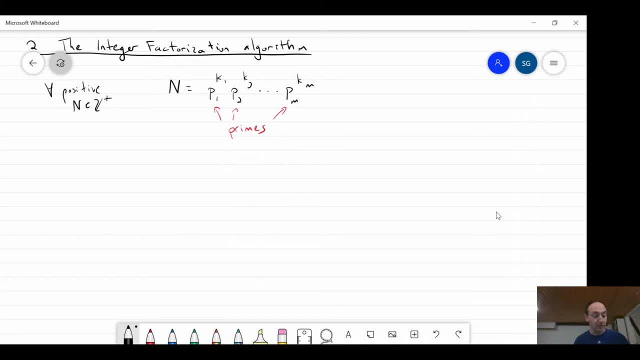 In general, each prime can of course appear more than once. Okay, and of course each pi is going to be distinct. Otherwise I'd write them together And this decomposition is of course unique. So, intuitively, you know, the factoring problem is going to be. 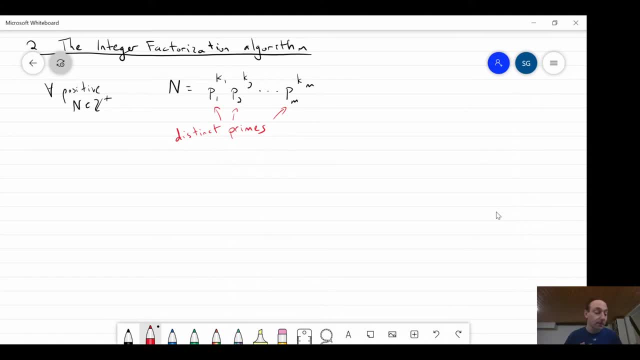 I'm going to give you n and I'm going to ask for the prime factors. Okay, so before I go any further, let's first do the first exercise in the notes, And now, by the way, we've started the numbering exercise in the notes. 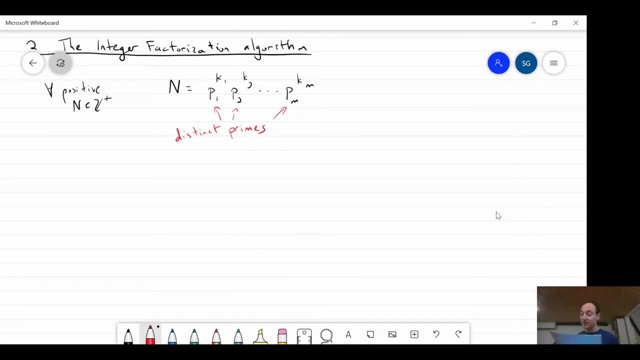 Woohoo, Okay, so now I can refer to exercise one, right? So exercise one in the notes is something everybody should do the first time they stare at this problem to convince themselves that really the naive, the algorithm for this problem is not polynomial time. 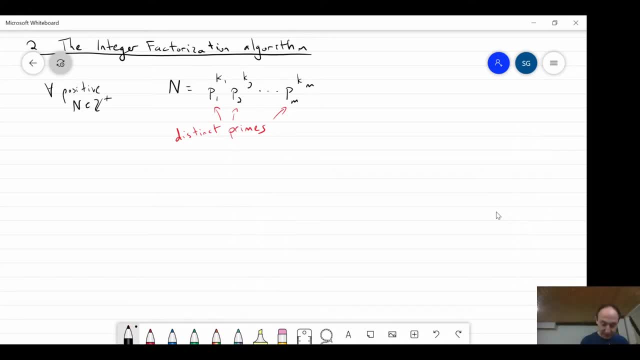 Okay. So consider this naive algorithm. This is exercise one. So the naive algorithm is you basically write a for loop And what you do is you go from say i equals to say 2, all the way up to say roughly the square root of n. 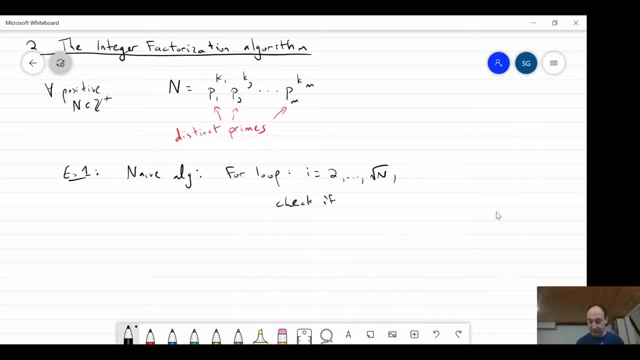 And then you just check if i divides, And okay, and so you basically try all the factors via brute force, from 2 up to square root n, And then whenever you find a factor, you just return it right, Roughly speaking, okay. 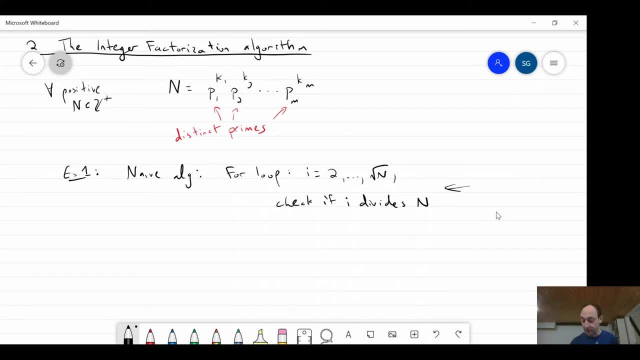 And you know this algorithm. roughly speaking, let's just say you're looking for one factor, not all of them. You know this will take at most order square root n field operations over the integers or the real numbers, right. 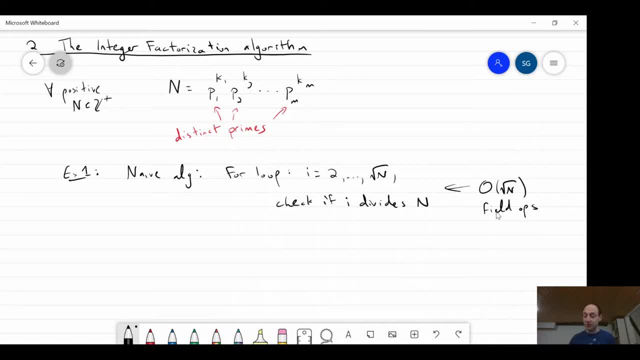 I mean, you're going to every time you division do one division, it'll be one field operation. So why is this not polynomial time? Because it looks like it's. you know scaling with n. basically right, And the key point is that. so here's the question. 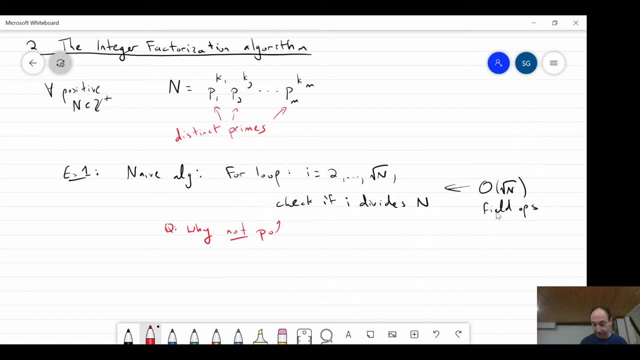 why is this naive algorithm not a polynomial time? Okay? so I highly encourage you to pause this video right now and think about this for a second, And the hint is going to be that you need to think about the encoding size of the input n. okay. 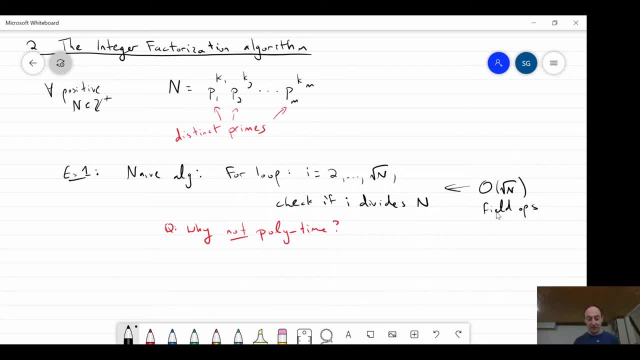 Okay. so if you haven't paused the video or if you restarted, let me give you the answer. Basically, the answer is that the encoding size of the input is going to be what If I want to write the integer n? I don't write out n bits, right? 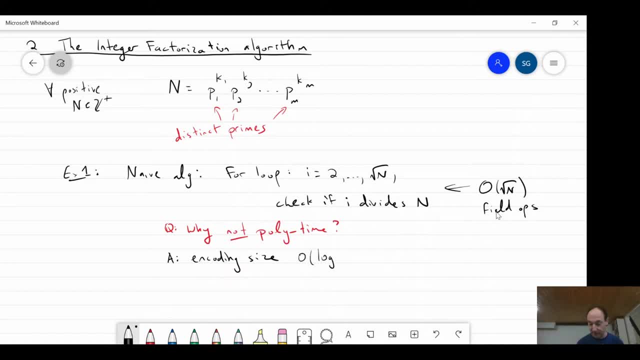 I write out log n bits, So let's order a log n, right, That's if I feed this thing into a Turing machine. that's how I specify n in binary. And so a runtime, a poly runtime. remember we say polynomial always in the size of the input. 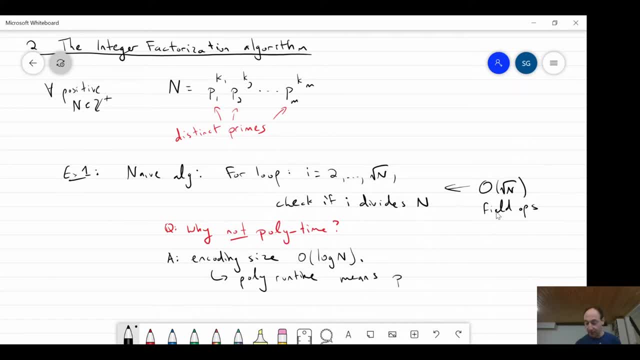 It means something that's going to scale like poly log n. Okay, that's what we would consider efficient, But of course you know this thing over here is not poly log n. It scales with n, basically right Square root of n. 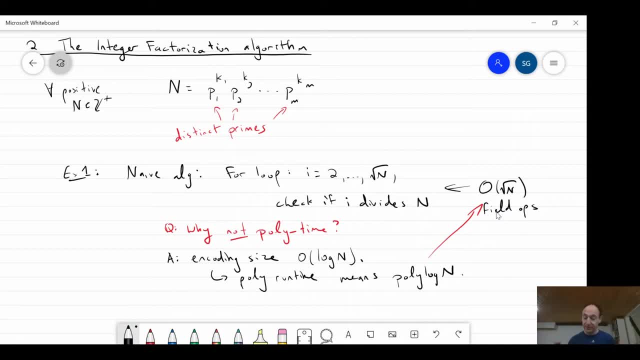 So that's why this thing is not efficient. Okay, if you didn't understand that yet, I would certainly encourage again pausing the video, going back and thinking about it some more, because I think it's crucial to understand that before you move forward. 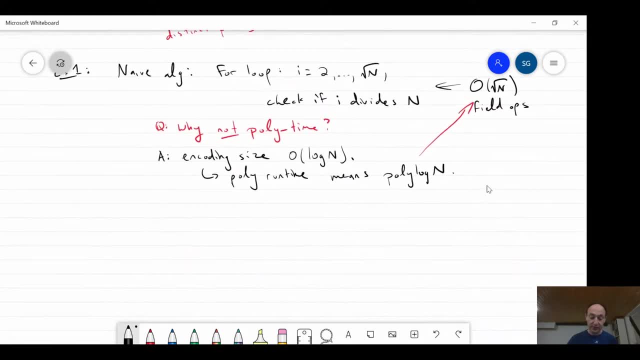 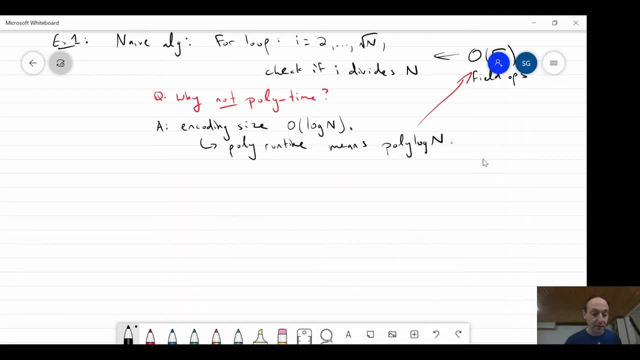 Okay, Okay. so this is exercise one. This is why the very naive algorithm you probably think of first just doesn't work. Okay, so now I'm going to formalize what I mean by factoring. So I gave you kind of a hand-wavy definition. 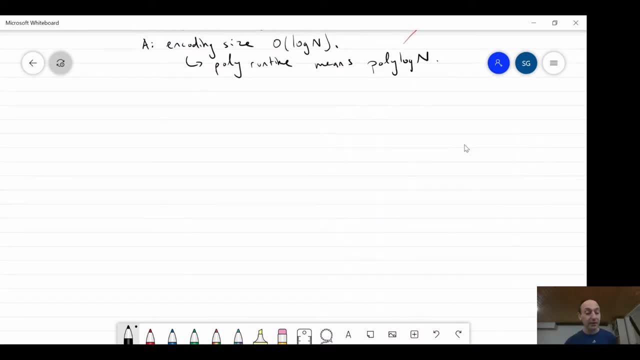 but again, we're theoretical computer scientists, We want to be very formal And we like to think about decision problems in particular. Okay, so that means that we like yes or no answers, Okay, or questions with yes or no answers, because that's how we define complexity classes like P and NP, right? 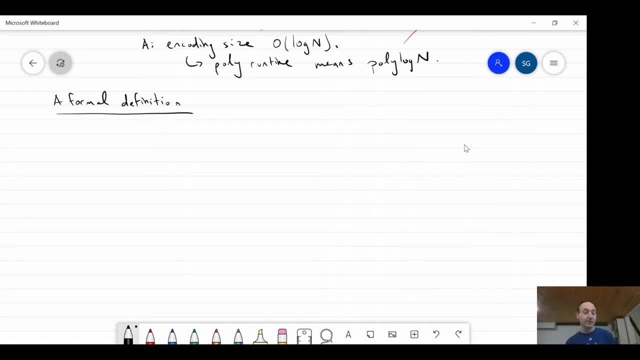 They're always defined in terms of yes or no, No questions, Okay, so the way we're going to do this, this is definition three in the notes, And I'm going to henceforth just call this problem factor in capital letters. The input is going to be a positive integer. capital N greater than one. 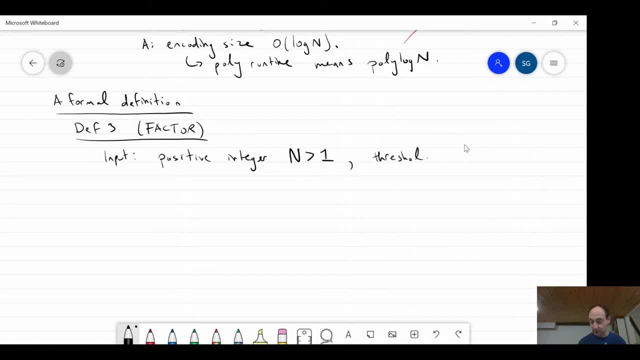 And you'll also get some threshold parameter. Let's say it's capital K and it's also a positive integer And the output is: whoops. does N have a prime factor smaller than K? Okay, so all I'm doing is I'm turning this into a yes or no question, right? 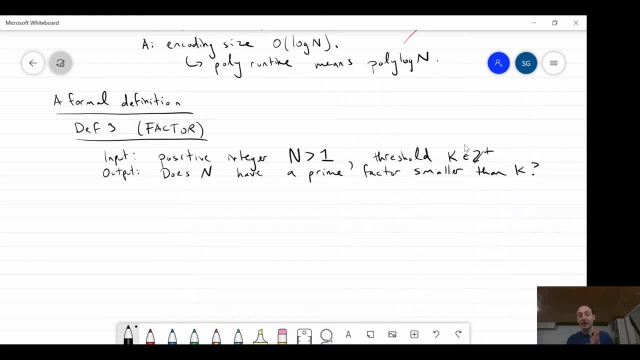 I mean. so I have to give you a threshold. Is the prime factor smaller than K or not? You can, Sorry, is there a prime factor smaller than K? And you know any sort of optimization problem. typically you can also turn it into a decision problem. 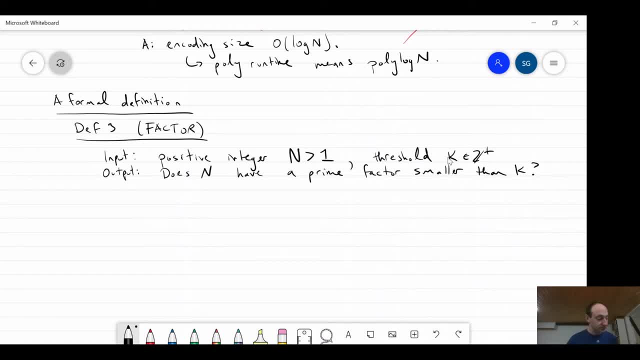 using this sort of threshold trick. So this is very general. And exercise four in the notes shows that without loss generality, if you want to compute all the factors you know it suffices to be able to solve this decision problem right. 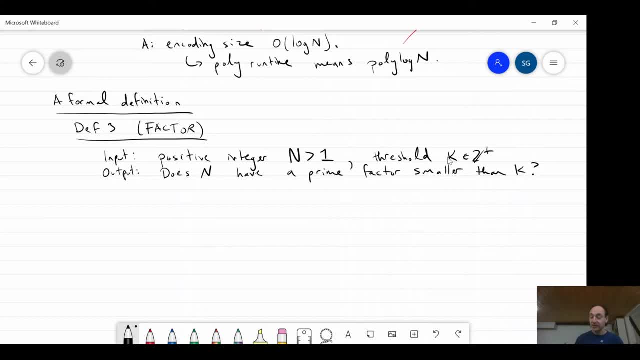 So why is that? Well, if you want to figure out, say, the smallest factor, then what do you do? Well, you could use this threshold. You could use this threshold to do binary search, right To figure out, to zoom in on the right factor very, very quickly in the log of N iterations, basically, 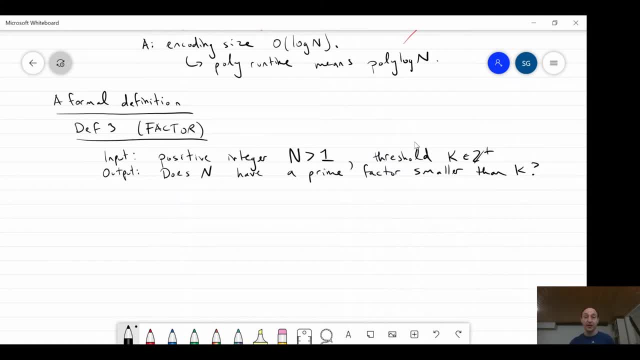 And once you have one factor, you just divide it out and you remove it, And then you repeat the entire process over again to find the remaining factors. Okay, So you know it's without loss, generality, in some sense, that we talk about decision problems. 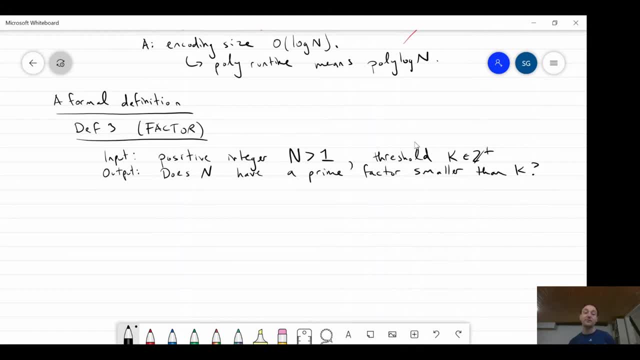 because typically you can solve the optimization version, given the ability to solve the decision version. Okay, So that's it, Okay, Okay, So that's the formal definition of factoring. Let's think a little bit about where this thing lives in terms of complexity: land. 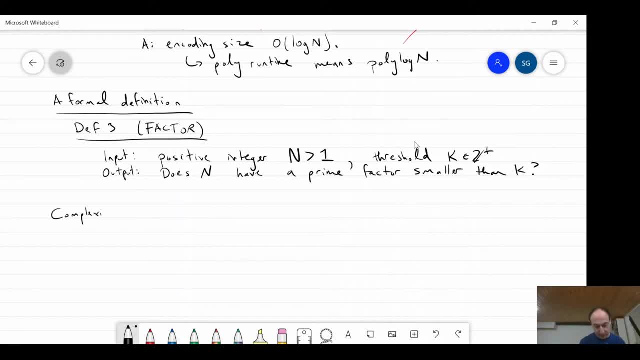 Okay. So complexity, theoretic considerations: Okay. So what's not known, Obviously, is that factor is in P. So remember, P is the complexity class of problems or languages that can be decided using a polynomial time Turing machine. So that's not known. 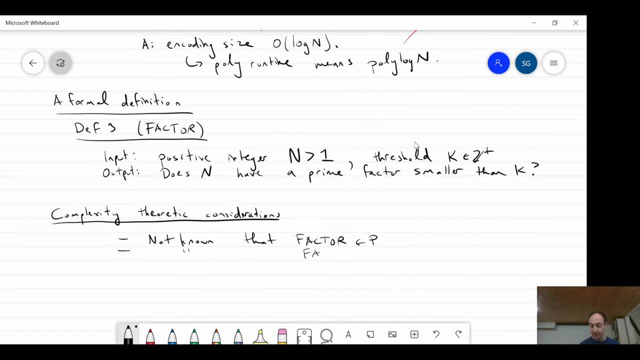 But it's also not known that factor. is NP complete Okay? So remember, these are the set of problems that can be reduced to any other problem in NP, such as 3SAT is the canonical one, And so we also don't know. 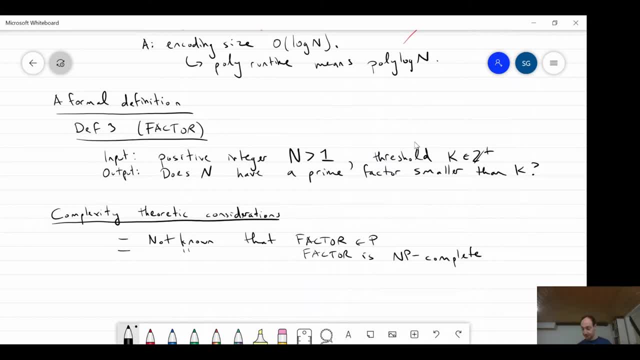 Okay, So we also don't know that. you know, factor is rigorously hard in some sense. Okay. Now the funny thing, however, is that there's a problem that's very closely related to factor Looks almost you know. this problem is the primality testing problem. 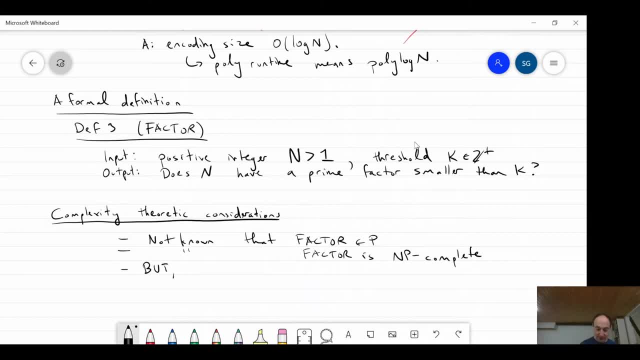 Okay. But so there's a big but okay the the primality testing problem. So let's just go back to the same example. our first problem Is NP. Okay, So this was a breakthrough result that I think was in the early 2000s. 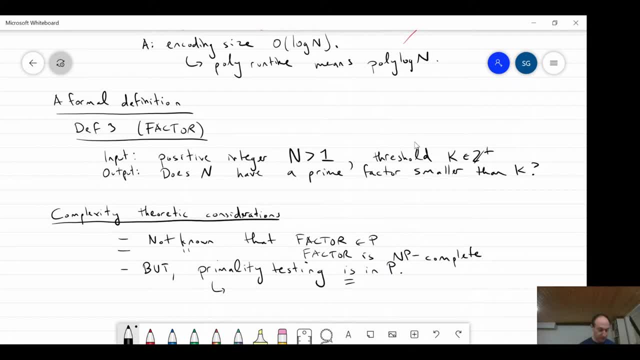 That the following problem. now let me just formalize the problem first. So you're given again a capital N in the positive integers, just like for factoring. You just want to know: is N composite Okay? By which I mean. 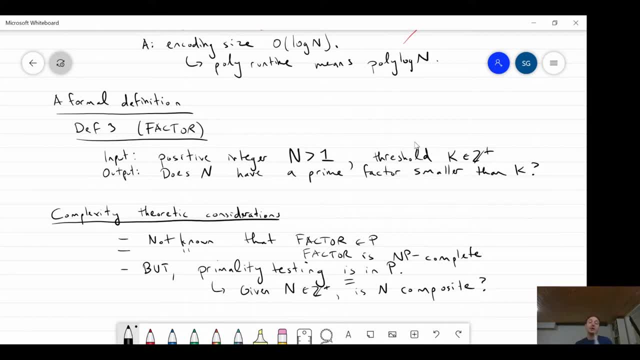 Is it the product of more than one non-trivial prime, And even though this sounds extremely similar to factoring, it's the same kind of idea. Certainly, if you can factor, then you can answer this problem. Primality testing is in P. 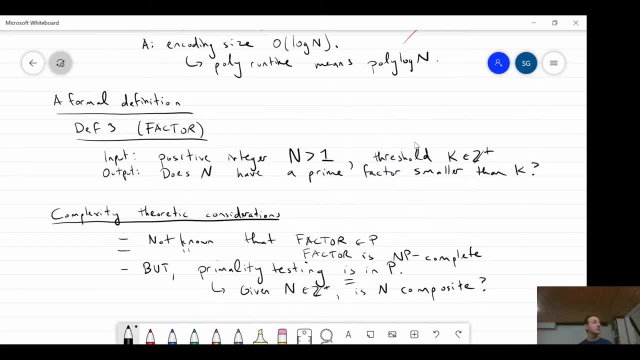 Again, this was a breakthrough result. This happened in, I think, early 2000s. But let me be clear also that the breakthrough was to make the algorithm deterministic. Before that there had long been known a randomized algorithm for primality testing. 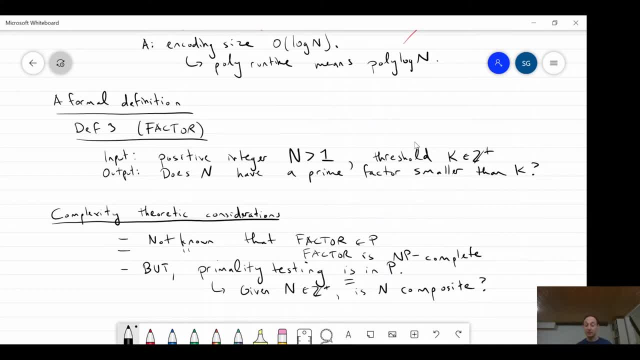 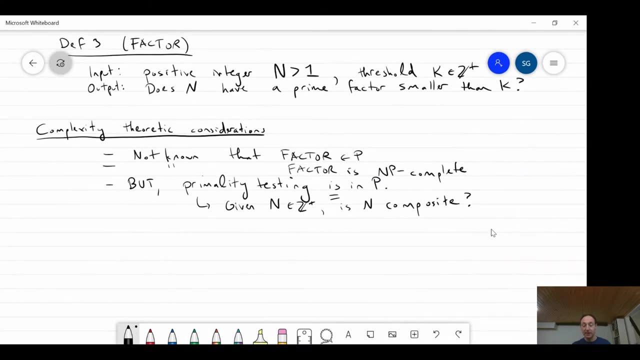 that essentially worked for all the input instances you can care to solve essentially. So, interestingly, this closely related problem is in P, but we don't know what to say about factoring Now, what we can say as a result, however, because primality testing is in P. 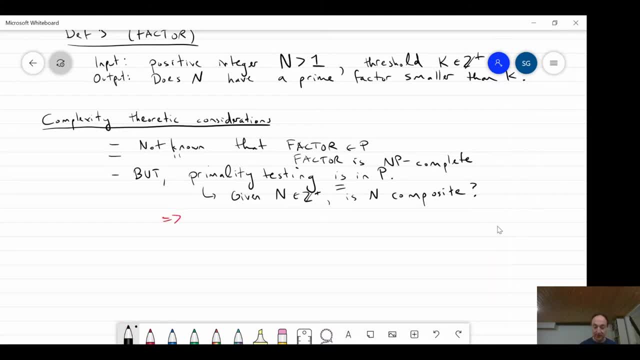 a consequence of this is that one can show that factor is in both N and P interchangeably. So, to be fair, if you can find the true answer, then you are going to be able to prove the factoring is in P for both N and P. 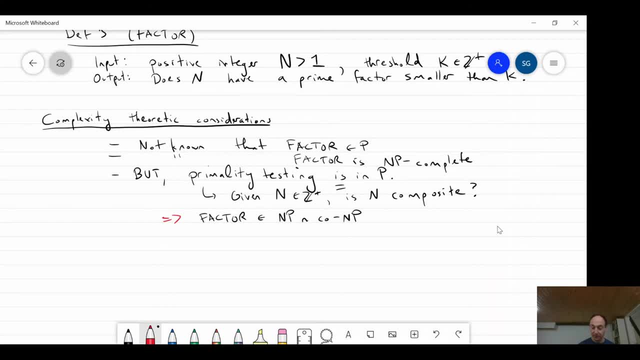 So remember that very briefly For N and P, whenever you have a yes instance, then that means that there exists a proof you could feed to a verifier To accept. So I'm going to assume a little bit of basic complexity, theoretic background here in terms: 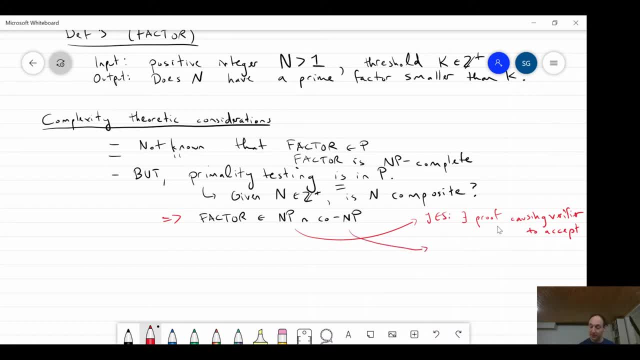 of P and N and P, And remember that co-N and P is basically the opposite of this, in the sense that In the yes case, for all proofs, the verifier- well, okay, formally speaking, you might define it as accepts or rejects. 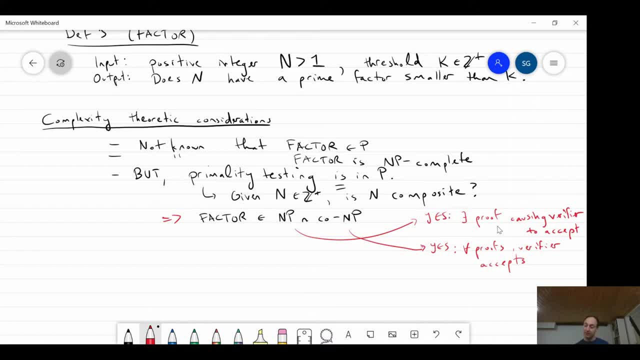 I mean it doesn't really matter in some sense. Okay. so this is kind of the difference right. So in some sense, yes, instances can be proven in p and no instances can be proven in co-np. Okay, so factor would fall into both complexity classes. 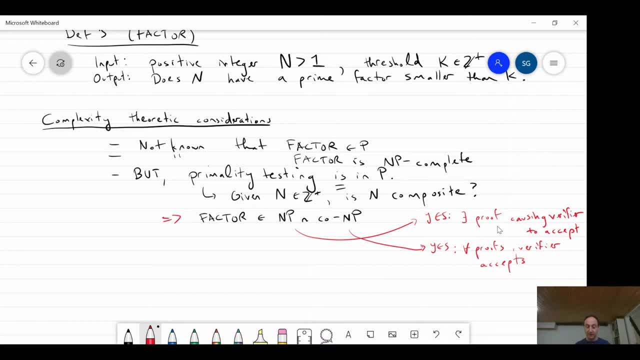 So why is this true? These are- this is exercise five and six. And so, basically, why is factor in np? Well, you know, if, if you know, factor, the number n has a prime factor smaller than k. remember, that's how I defined it, right. 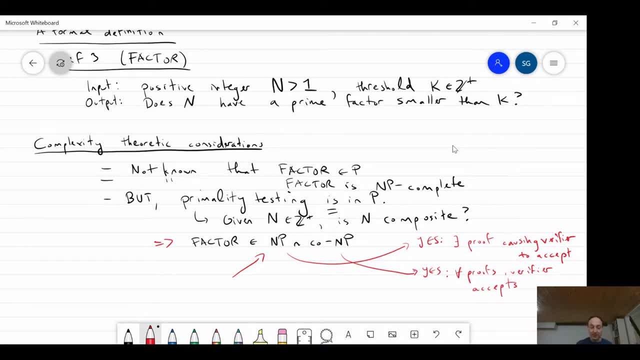 Then it's very easy to prove to me, right? You just give me that prime factor, right? So you just give me the prime factor Which is less than or equal to k, right? And then I can just divide n by that prime factor and I can check that indeed it's a factor. 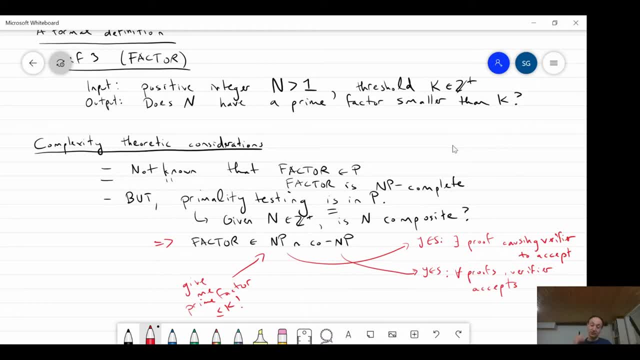 Okay, And, of course, the what you gave me. I can also check that it's a prime factor because I have a primality testing algorithm right Here. it is, So I could also verify that. And how about this thing? 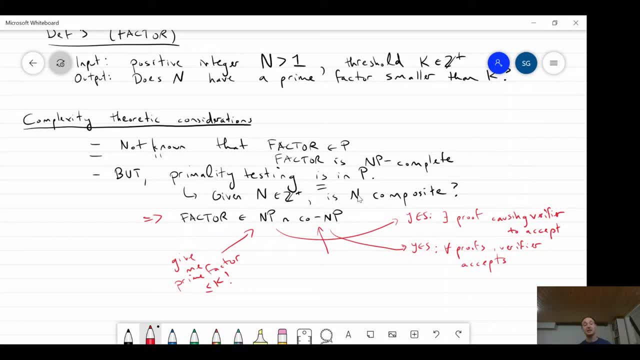 How do you prove that this thing is in co-np? Well, basically, what you need is that, when there is no prime factor smaller than k, you should be able to prove this to me, right? So for all proofs, right. 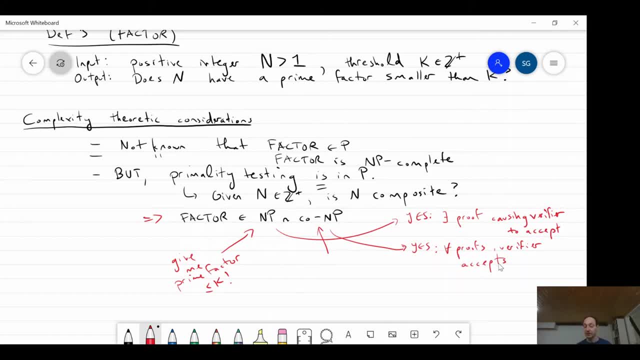 Okay, So for all proofs, right. Okay, So for all proofs you give me. you know the verifier will, you know, accept or reject, however you want to define that criteria, right, But it's going to do the same thing on all proofs. 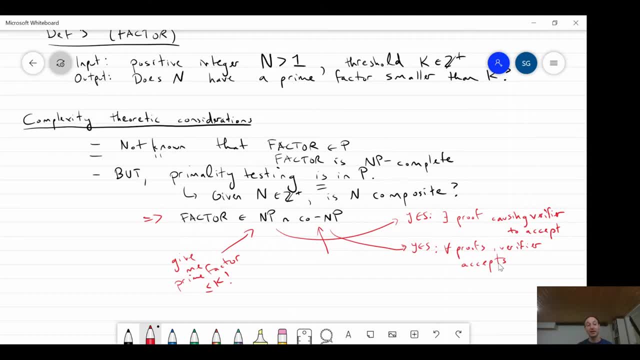 So, in particular, if this thing does not have a prime smaller than k, you need to be able to prove it to me. And well, how do you do that? Well, you just give me the prime factorization, the full prime factorization. 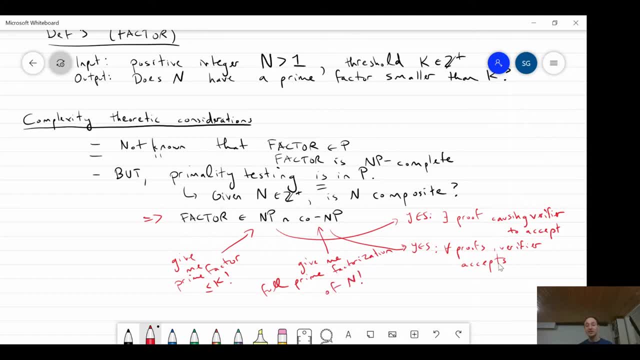 Okay And you know, with a bit of thought you could see that this doesn't. This doesn't take a lot of space to write down. You'll never have more than you know. order: poly log n: prime factors, basically not including multiplicities. 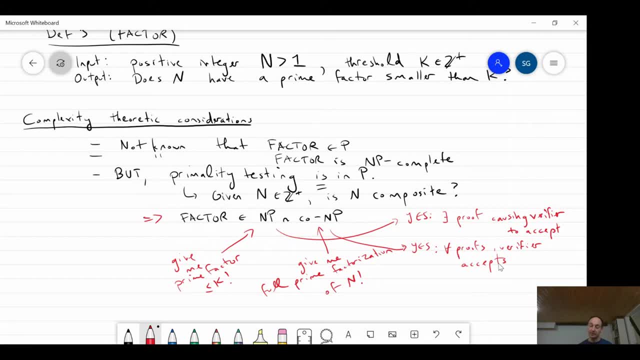 Well, I guess even including multiplicities. And so if you were to give me the full prime factorization and I can check- indeed you know the factors you give me are prime because again I have a primality testing algorithm- then I can verify myself that indeed you know, there is no prime factor smaller than k. 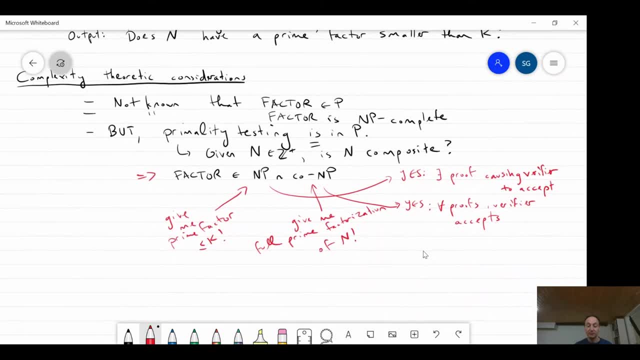 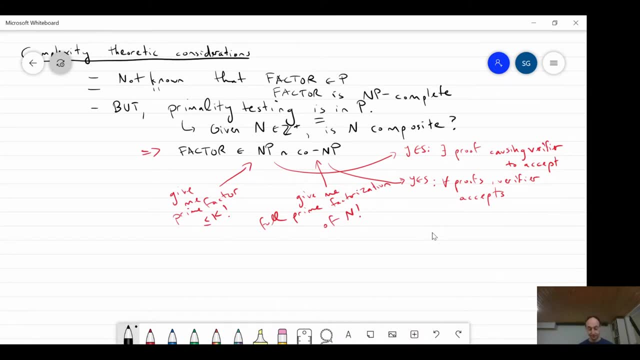 Okay, So factor is in. In this sense it's in both these complexity classes Whether there is a small factor or not. in both cases you can prove it to me, Okay, And now there's a big, but which is that, you know, with a bit of thought you can show, and we won't do this here. 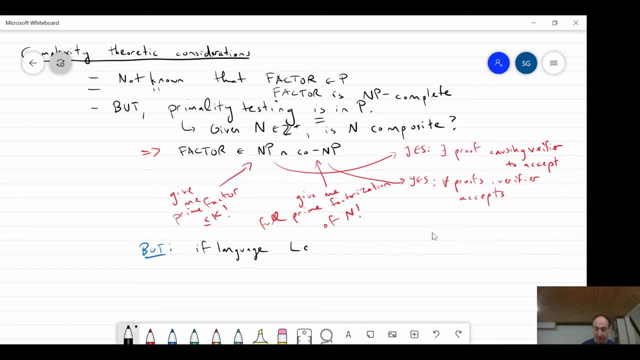 So if we have a language, such as factor, that happens to be in both np and co-np and it's np complete or say co-np- complete doesn't really matter- Then it would imply that np equals to co-np. 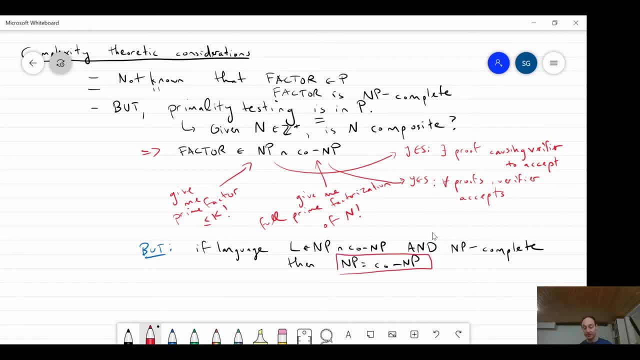 Okay. So you know we said earlier that we don't know that factoring is np complete, but this is basically saying that because we know that factor is in np and co-np. if it were to be np complete, then there would be a pretty strong consequence to this. 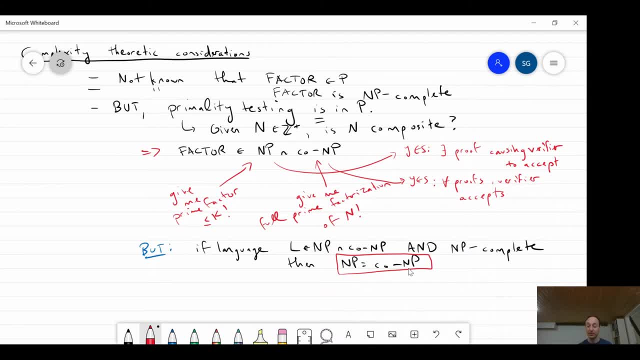 The consequence would be that np would equal to co-np- And again, this is something you can prove. I'm not proving it here. And this consequence: np equals to co-np- again you can prove this, but I'm not going to because I don't want to introduce more definitions here. 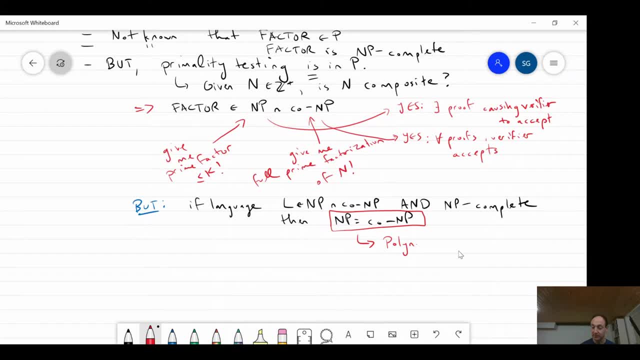 This implies that something called the polynomial time hierarchy- polynomial time hierarchy- Okay. If you haven't seen this before, I certainly recommend you take a moment to pause this video and go look it up on wiki. This thing would collapse. Okay, And so that collapse is you know. 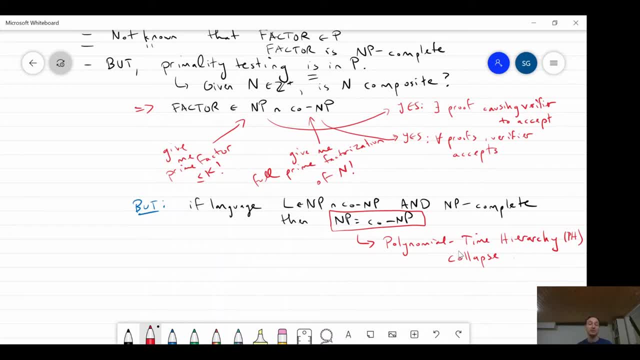 More or less deemed, you know, just as unlikely as p equaling to np. It's a really. it's really strongly believed to be a highly unlikely consequence for this ph to collapse. So, in a nutshell, what this is basically saying is that it's highly unlikely that a factor is going to be np complete. 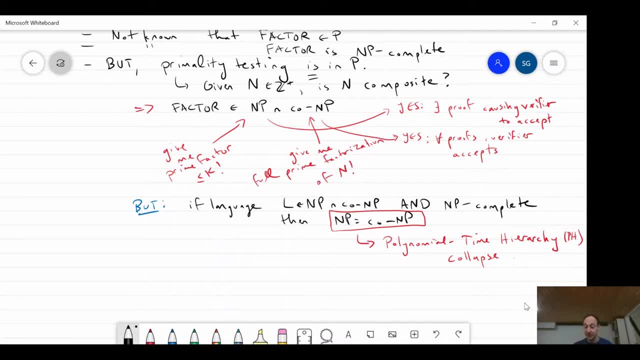 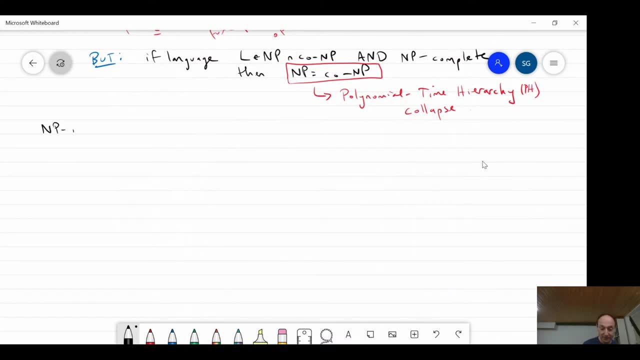 Okay, So it's not necessarily known to be np, but it's also not known to be np complete And, moreover, we don't think it's np complete, Okay, Okay, So this might sound very, very Dissatisfying or unsatisfying. 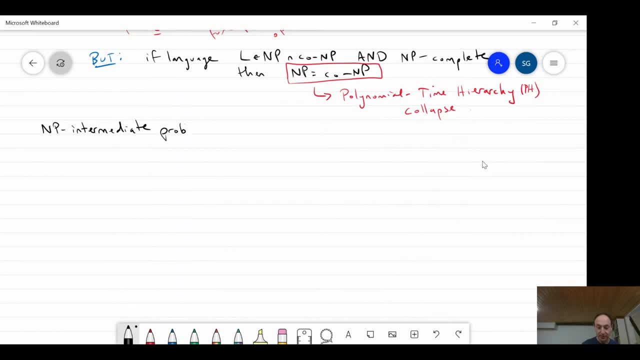 Now I really should know which of those two is the correct word to use. But there is kind of a silver lining, And the silver lining is that there is such a thing as np, intermediate problems. Okay, And in particular, what Ladner proved- I think this is 1975, right. 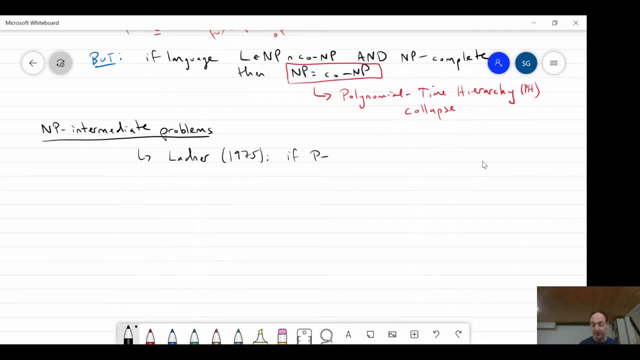 What he proved is that if p is not equal to np, Okay, Then there exists. There are so-called intermediate problems, which are, you know, there are languages, l, such that l is neither in p and l is not np complete. 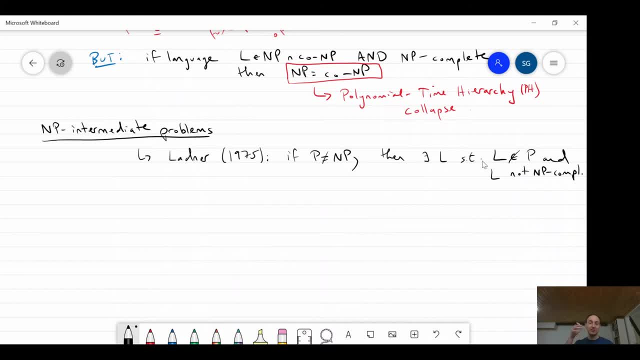 Okay, So that's kind of amazing, right? This is basically saying that you know, there's a kind of a complexity class or something that's sandwiched in between things that are polynomial time solvable and things that are not necessarily polynomial time solvable, but they don't capture the difficulty of all of np. 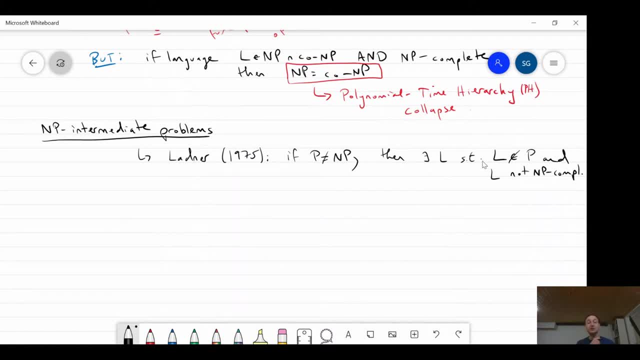 Okay, And you know Ladner's construction is arguably quite artificial, but you know it works for what it's supposed to work for. Ideally you want natural problems which are np intermediate, And there are very, very few of those. 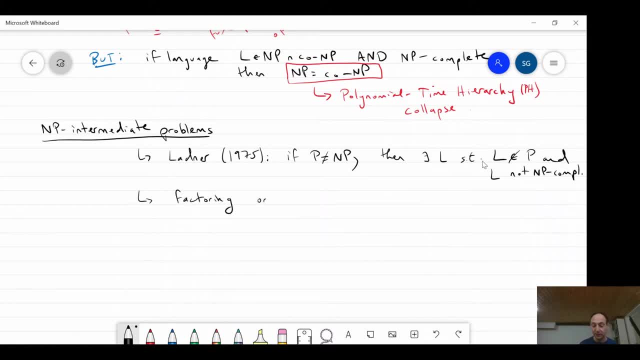 And factoring is one of the few known natural np intermediate problems. Okay, So that's something nice that comes out of this. Okay, So it's not polynomial time solvable as far as we know, but we also strongly disbelieve that it's np complete. 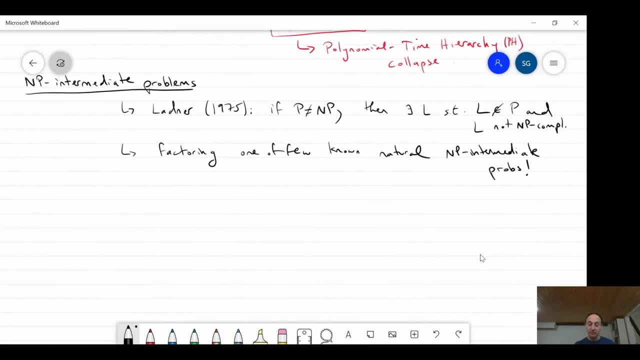 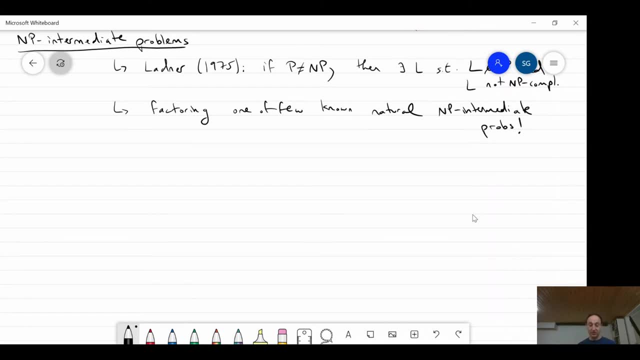 Okay. So you know, for all intents and purposes, you know we probably believe this problem is np intermediate. Let me just say a little bit about, And you know, I don't think you can get away with talking about the factoring algorithm without talking about the extended Church-Turing thesis. briefly, 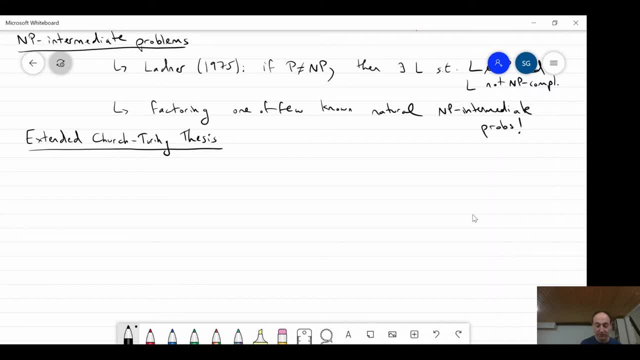 Okay, And so you've probably seen the regular Church-Turing thesis in your Introduction to Languages and Automata courses. So remember that the Church-Turing thesis is basically the backbone on which most of theoretical computer science rests right, And in particular, the Church-Turing thesis basically says that you know Turing machines capture everything there is to know about computation. 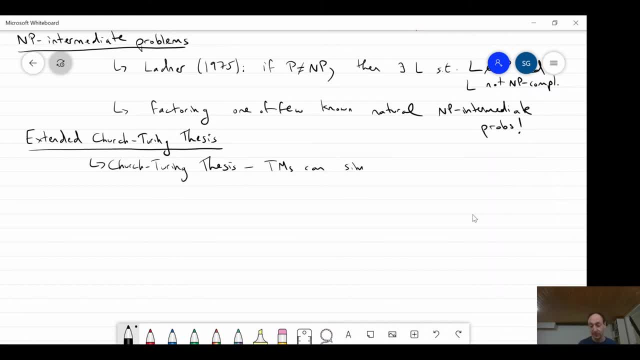 In the sense that Turing machines can simulate- in quotes, you know- any other model of computation. Okay, So that's very roughly what the Church-Turing thesis states. Okay, So we might as well just solve Turing machines, you know, and that tells us everything we need to know. 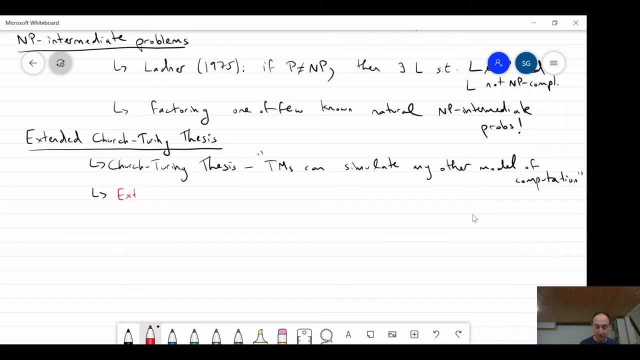 But there is a slightly different version, an extended version. Okay, And then the extended Church-Turing thesis. Right, And this looks almost the same. So you know, I'll put these guys, Except we're going to insert one word here. 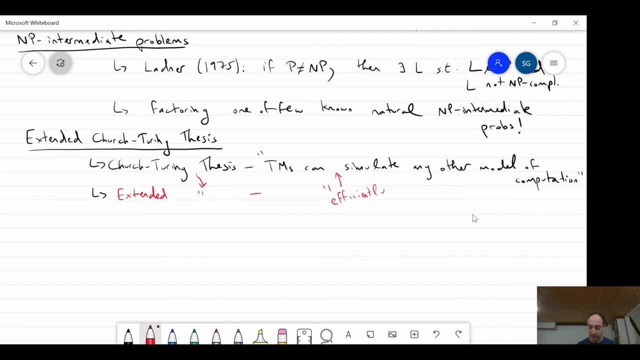 We're going to insert the word efficiently, Okay. And the other thing we're going to do for the extended Church-Turing thesis is: Here we're going to say that the model of computation should be Okay, Okay, Okay, The model of computation should be physically realizable. 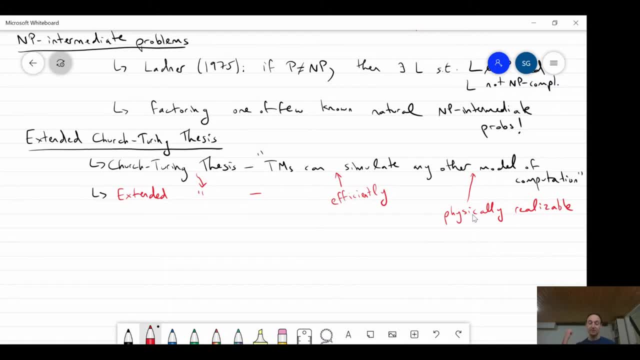 Okay, So we want to talk about, We want to posit that. And let's be clear, Of course, both of these, theses are theses. They're not proven facts There's. I mean, it's not clear at all how you'd even begin to prove this thing. 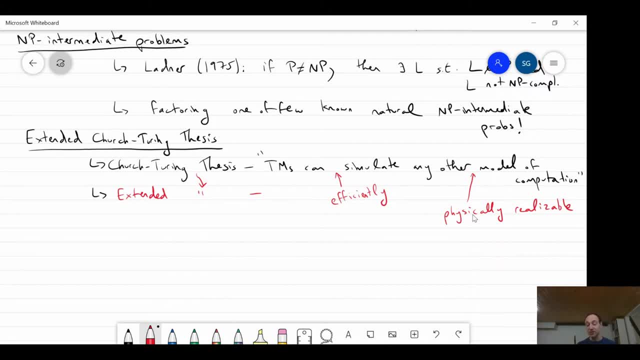 Okay, But if we're going to demand on top of this that Turing machines can efficiently simulate other models of computation, then you know it's very reasonable to ask that the model of computation at least be physically realizable, Right? So the laws of physics should allow this model to be actually built on a large scale. 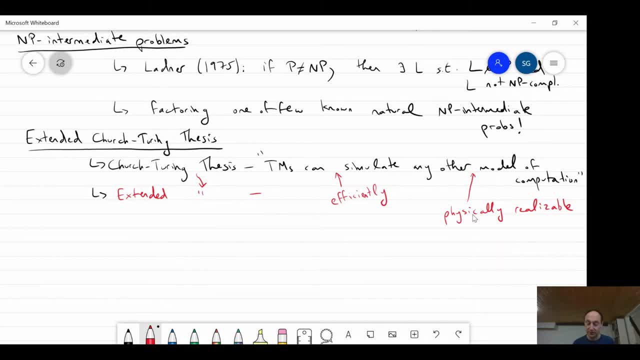 Okay, Otherwise, obviously, who cares if you can efficiently simulate it or not? Okay, So these terms in red are basically what you add to the regular thesis to get the extended version of the thesis. And let me be clear that you know, the extended version of the thesis is much less commonly accepted than the standard Church-Turing thesis. 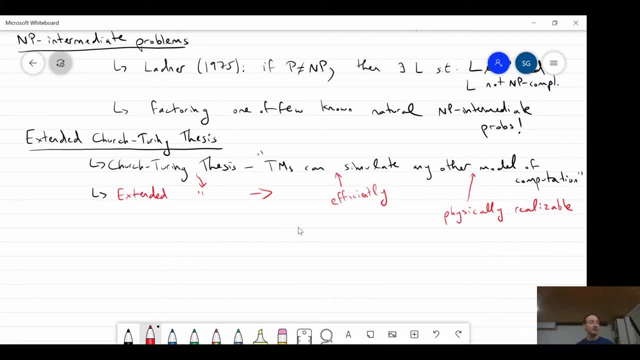 which is, you know, very broadly accepted. Okay, So there's a sense in which it was a discovery of a Schwarz factoring algorithm which kind of made the extended version More quote-unquote popular, Not in the sense of people believing it, but necessarily- but just gave it more visibility. 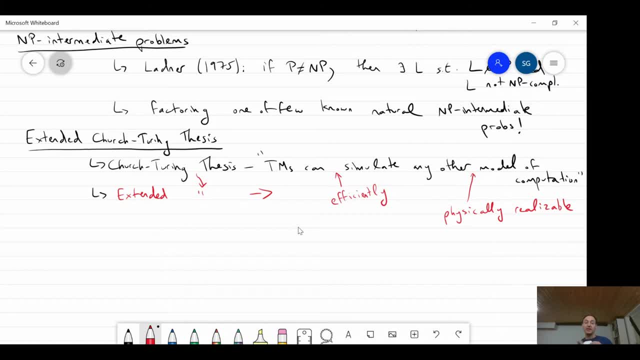 Okay. So the point is that, because we have these added constraints of efficiency and physical realizability, you'll see now that Schwarz factoring algorithm and the extended Church-Turing thesis basically clash, And what we've learned is that, assuming Schwarz factoring algorithm is correct- which I think everybody agrees- 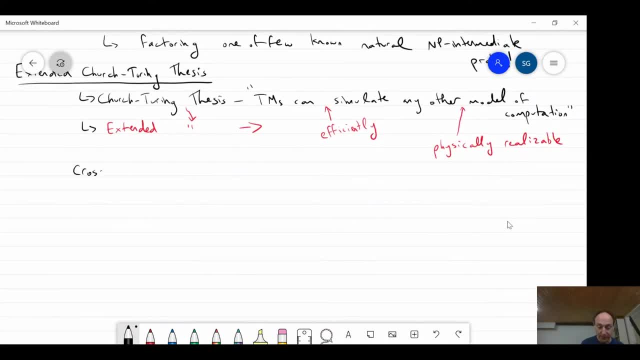 we're now at a crossroads in theoretical TCS, theoretical computer science. Okay, So one of the following, one of the following is false. Okay, So I'm going to write down three statements and one of the following must be incorrect. 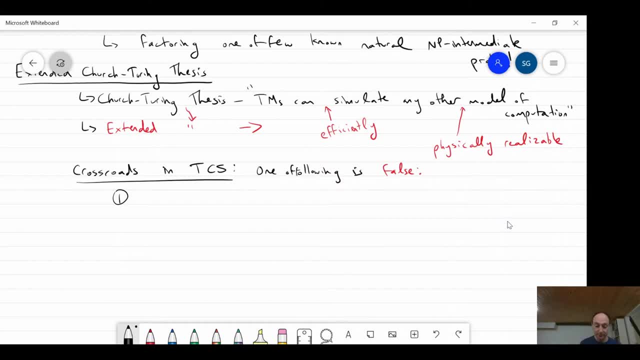 Okay, So the first statement is that the extended Church-Turing thesis is true. Okay, So that's the first statement. The second statement is that factor or factoring does not have an efficient classical algorithm. So this is basically what most of the classical community believes. 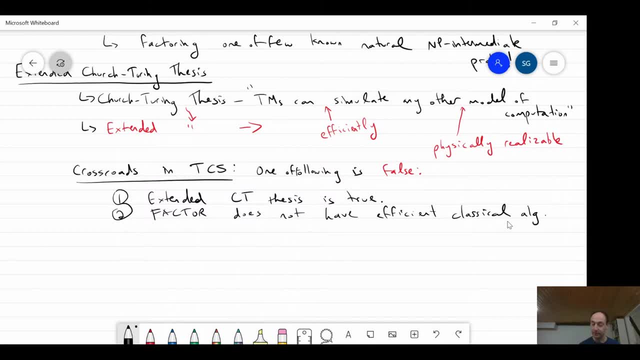 Okay, So factor is not in P. And the third statement is what the quantum community believes, which is that, for the most part at least, which is that large-scale quantum computers can be built. Okay, So one of these three statements has to be false. 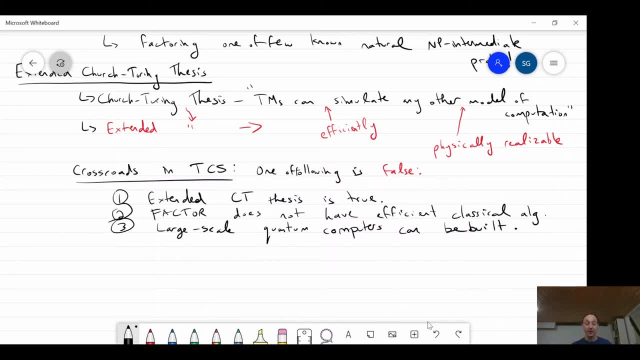 Okay, So let's just do an example of this. right, If the Church-Turing thesis is true and you can build large-scale quantum computers, well, what that tells you basically- that is sorry, what that tells you basically- is that: because the Church-Turing thesis, the extended version, says that any classical computer can simulate a quantum one efficiently, and because quantum computers are realizable, you know, you can build them. basically, then, that means that there must also be a classical algorithm for factoring right. 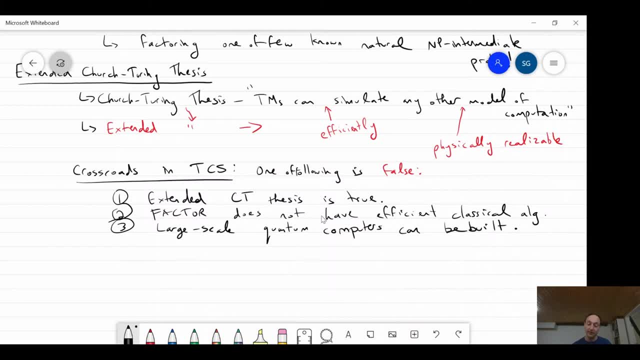 We just haven't found it yet. Okay, Of course, if factoring doesn't have an efficient classical algorithm and we can build large-scale quantum computers, then the extended Church-Turing thesis is false. Okay. And finally, the other interesting direction is that, well, if the extended Church-Turing thesis is true, 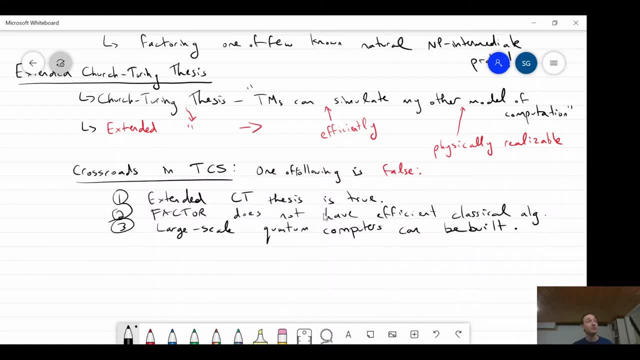 and factoring does not have an efficient classical algorithm. well, that means that somehow you shouldn't be able to do factoring quantumly right, And so mathematically you can do it. So the only other logical conclusion is that you must- you know we must- fail this criterion, right? 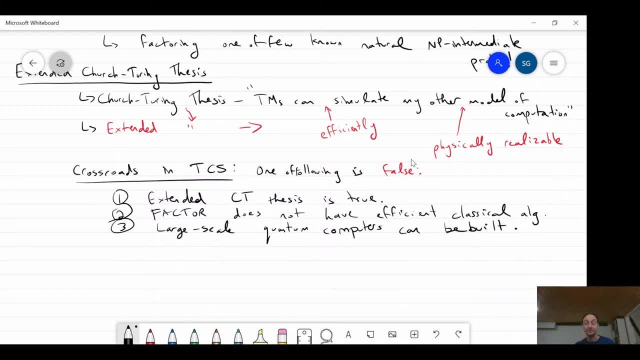 That the model must not be physically realizable on a large scale. Okay, So it's really interesting. It's very exciting, One of these things, you know, some of which are arguably more strongly believed than others. you know, I'd probably argue that two and three are the most strongly believed out of the 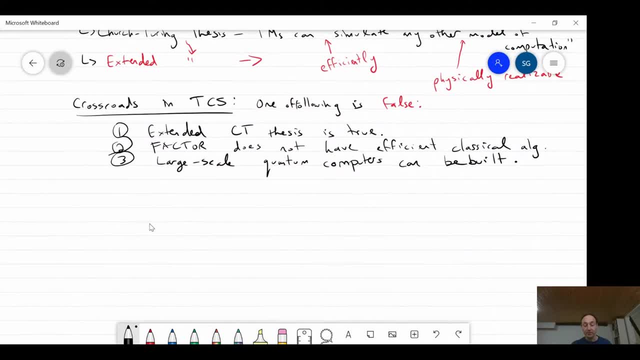 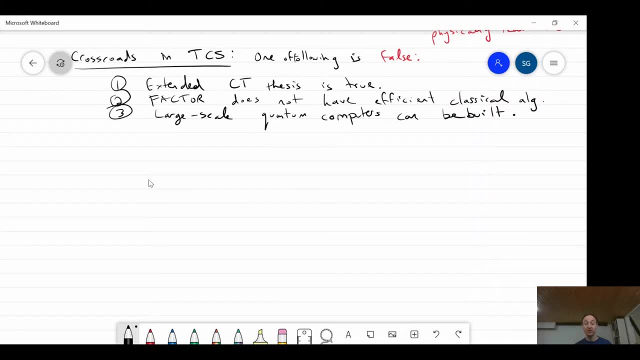 and one is the least strongly believed, But one of them must be false. Okay, So this is all I want to say about formalizing factoring as a decision problem in terms of its complexity theory that we don't necessarily believe it's MP. 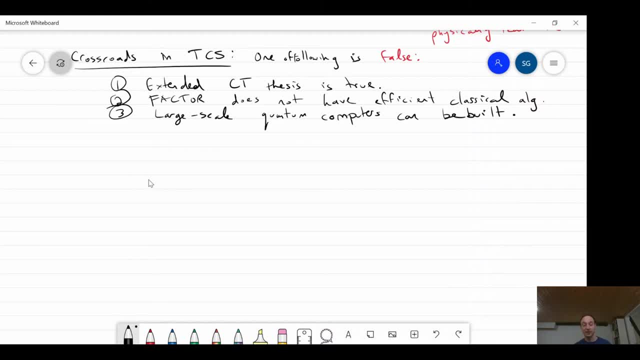 and we certainly don't believe it to be MP-complete because it would collapse the polynomial time hierarchy. It's believed to be MP-intermediate And finally it leads to this very nice crossroads in which one of these statements I've written down must be false on the screen. 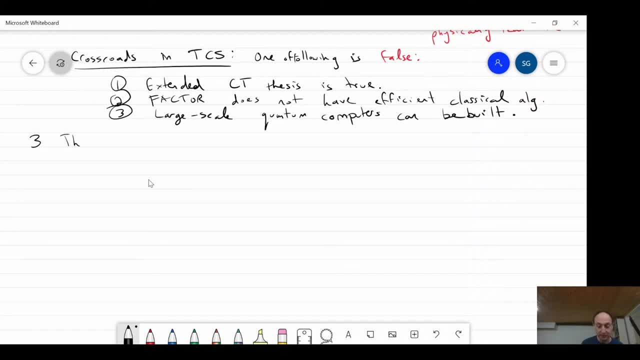 Okay, So now we can talk about the actual factoring algorithm. Okay, So this is section three, And again, this proceeds basically in three high-level steps. First, we're not going to solve factoring. We're actually going to reduce factoring to order finding. 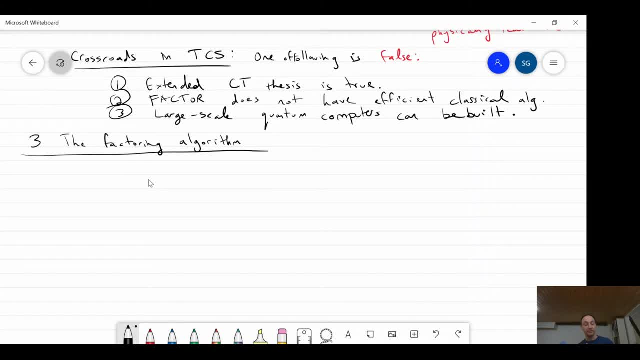 So I have to define that and show you the reduction. So we're going to do that first And then, once we have reduced order finding, we can solve order finding by combining quantum phase estimation and something called the continued fractions algorithm. 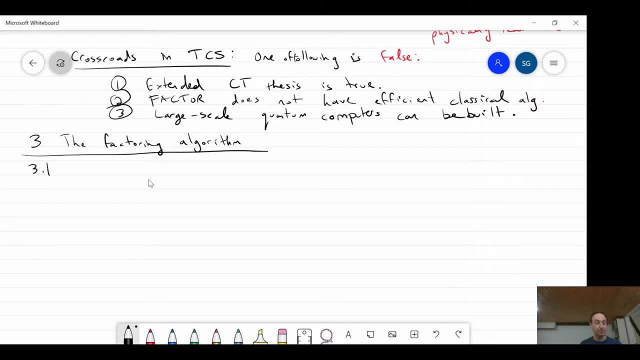 So let's start with the reduction, reducing factor to order finding. Okay, Section 3.1 in the notes. So let me define order finding Again. the short, the acronym I'll use is just capital order. So for this you're going to have to think back. 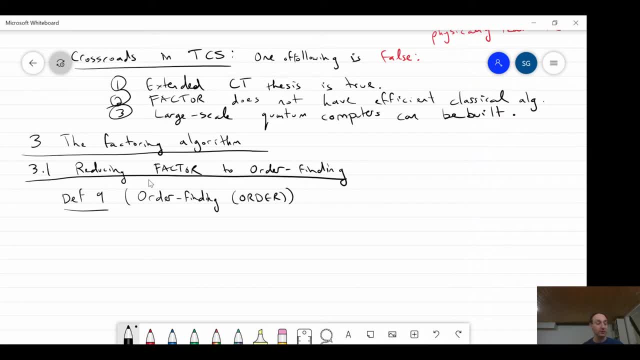 to kind of like your basic modular arithmetic that you probably learned in one of your first years in your university degree, And what it says is the following: Input output. right, So what you give me are positive integers, And okay. 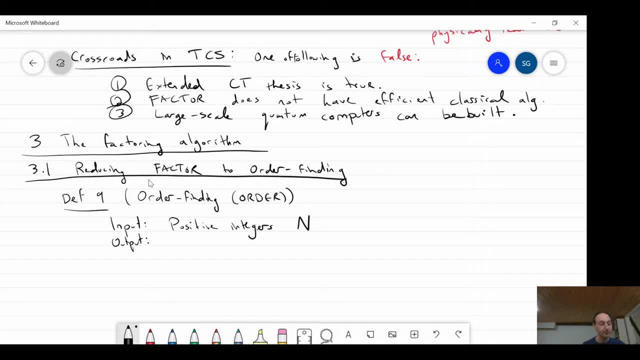 And some x, that's between 1, but strictly smaller than n, And x is co-prime to n. Okay, So co-prime to n means that, you know, remember this means that x and n, if you write them both in their prime, factorization. 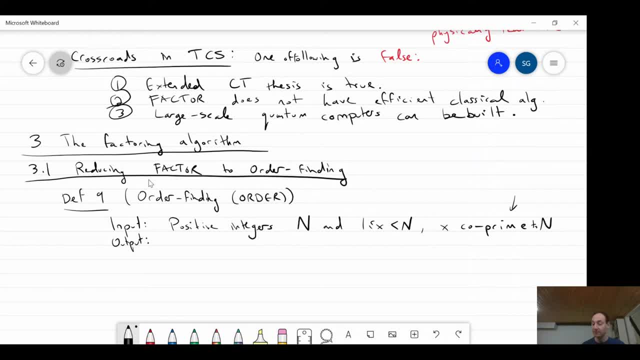 they will not share any value. Okay, So what we're going to do is we're going to- we're going to do this. So what we're going to do is we're going to do this. So what we're going to do is we're going to do this. 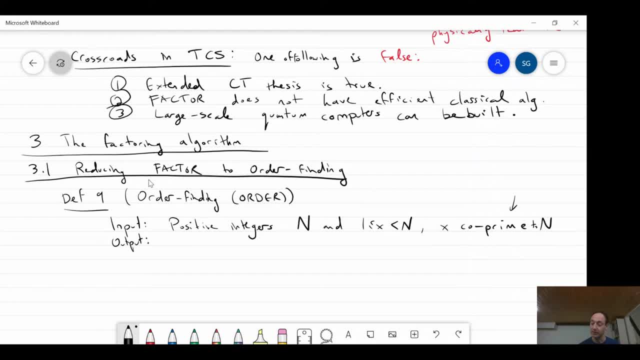 So we're going to do this. Okay, So what we're going to do is we're going to do this. So we're going to do this. So what we're going to do is we're going to do this. 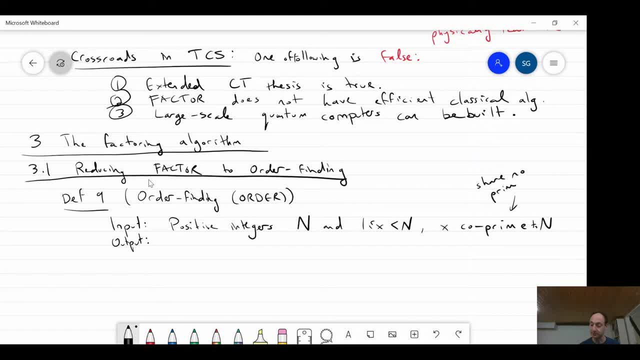 So we're going to do this. So that's the definition. you get the objection: They will not share any prime factors. Okay, So So they share no prime factors And hence no factors in general, Right. 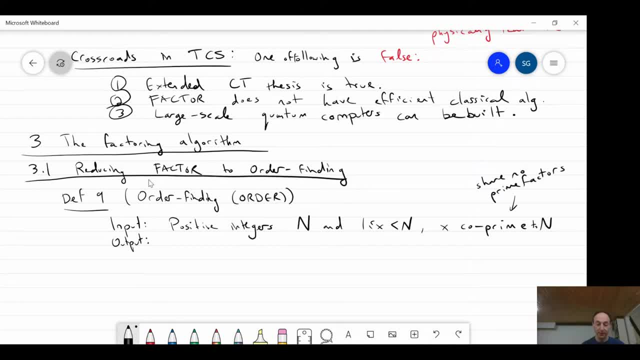 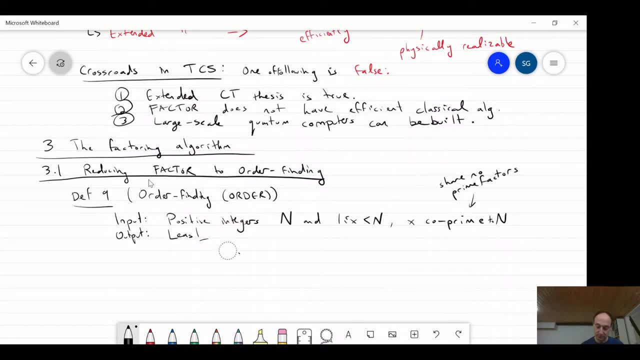 Okay, So that's just the definition, just to refresh your memory. Okay, And what is the output? The output is the smallest positive- whoops, what happened there? Okay, Well, we'll just keep going. The least positive value. 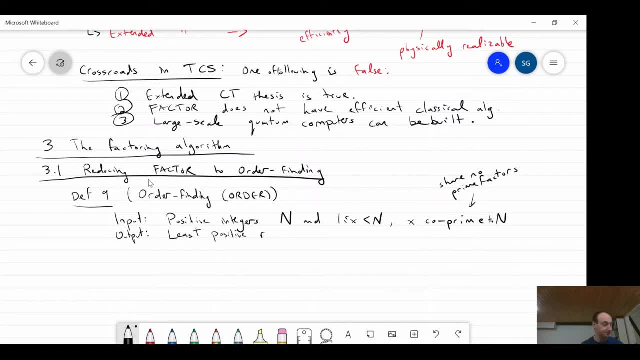 There is no value here, right? There's no value here. integer r, and so this is going to be called the order. that's why it's called order finding. you're trying to find the order that satisfies x to the r is equivalent to 1 modulo n. 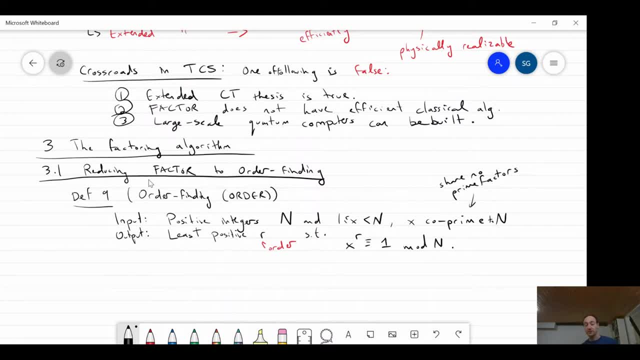 okay, so remember. this just means that if i take the left side of this thing and i divide through by n, the remainder i get is 1, and you know it's always good to remind yourself what is the equivalent definition of this equation: modulo n right. that just means that x to the r is equal to. 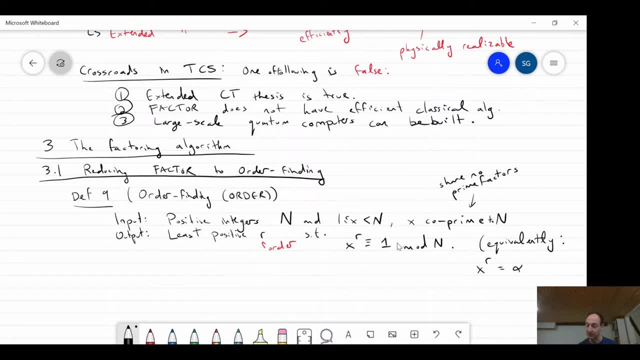 you know some number. let's call it alpha times n, so some multiple of n right. so this is an integer right plus one. so if you want to express x to the r, it's just some integer times n right. that part disappears when you divide by n and then you have the remainder one. 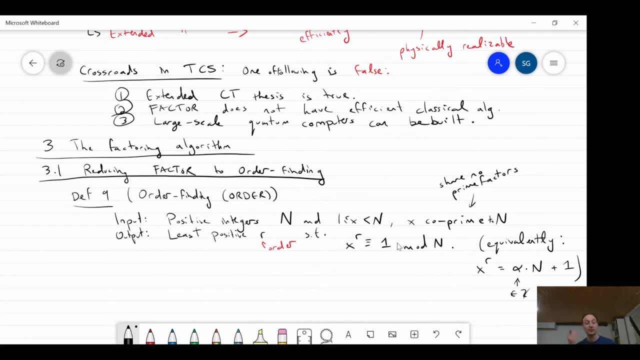 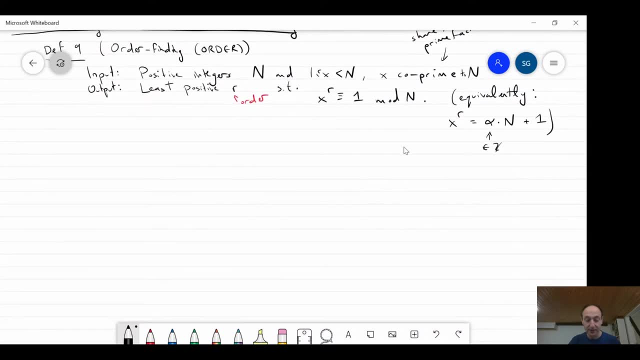 so just, it's always good to keep that alternate definition in your mind when you think about modular arithmetic. so this is the order finding problem, and the claim is that if you can solve order finding, then you can solve factoring, and that's what we're going to show now. 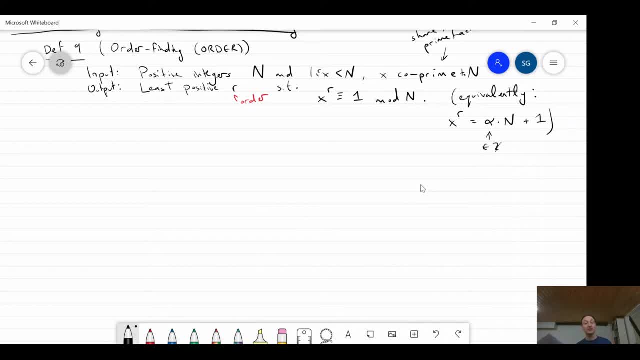 note that, by the way, i did not write this as a decision problem, like i did factor, just to keep things a bit simpler. one less parameter floating around, because i just said: give me the smallest positive integer, r. of course you could turn this into a decision problem, just like we did for factor. 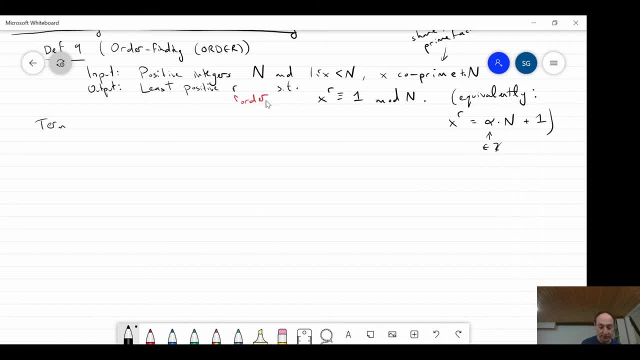 okay, so just some brief terminology that we're going to need. so we are. we already reviewed what co-prime means, gcd- greatest common divisor. basically is the. the greatest common divisor x and y, okay, and these are natural numbers, so you know just what's the biggest common divisor. 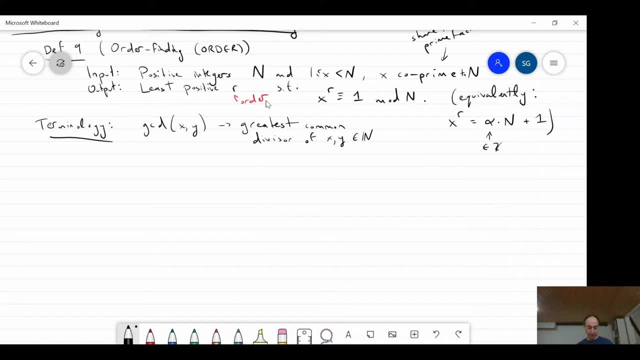 is the biggest number that basically divides both of these two. okay, and now i can be slightly more formal. when i say x is co-prime to y, that's equivalent to saying that the gcd of x and y is one right, the, the biggest number that divides them both. 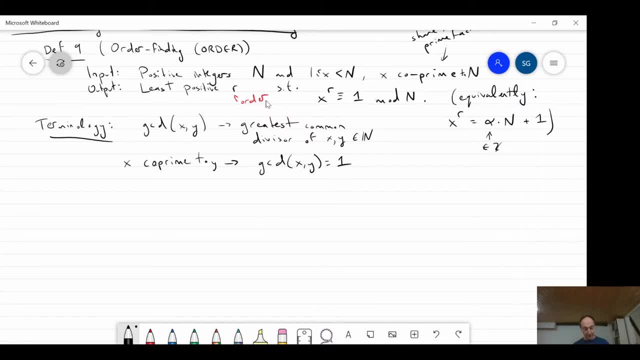 is just one. there are no other non-trivial factors. okay, so to reduce, factor into order, finding we're basically going to start at a almost a trivial exercise. okay, and so this is exercise 10.. i'll sort of sketch it here, but basically this is going to give away our strategy, okay. 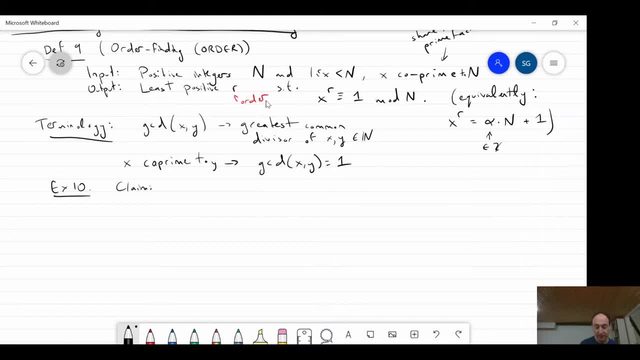 so? so the claim is that, uh, let you know, x be a non-trivial solution to um x minus one. so i'm going to write down an equation: a constraint, basically, is equivalent to zero mod n. okay, so find me an x that satisfies this and um non-trivial. what do i mean by non-trivial right? i mean it's kind of trivial to solve this. 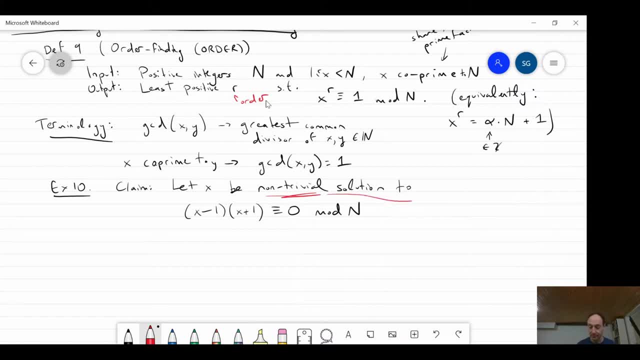 right, i could just plug in x equal to one or x equal to minus one, so that means that x is not in one or minus one mod n. okay, so suppose i have some non-trivial solution to this equation. and um, then basically um gcd of x minus one. 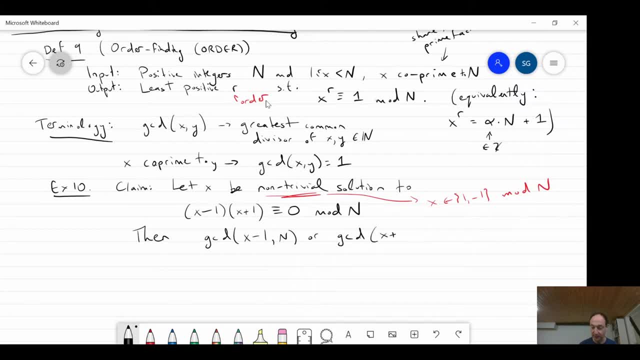 and n, or the greatest common divisor, x plus one. so these are the two terms you see here. right, here's one, here's the other. um is a factor, a non-trivial factor of n, okay, okay. so why is this true? right, i mean, because obviously what we're looking for is n, right? 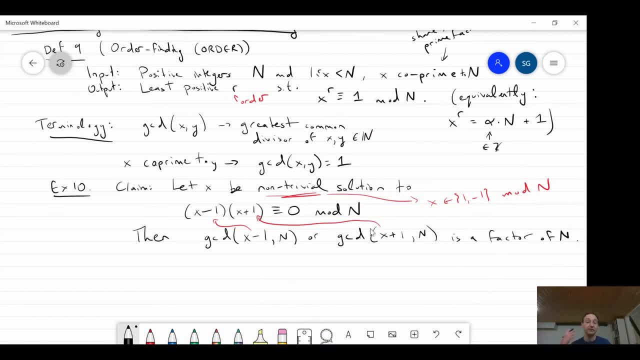 um, sorry, a factor of n, and so this gives us a kind of a first, uh way to make a step towards that. and so how do we do this? well, um, what we're seeing is that you know n, of course. what does this mean? this equation says that n divides basically this product x minus one. 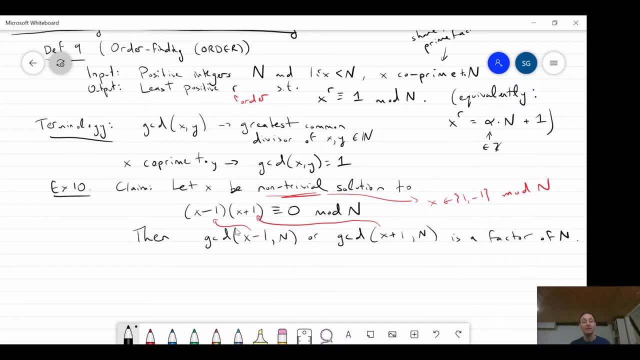 times x plus one. that's what the equation says. okay, there's no remainder, and so, um, there are three possible ways this could happen, right? um, there's a number of possible ways this could happen. right, either n fully divides x minus one. right, it goes into that bracket, or it divides x plus one. okay, 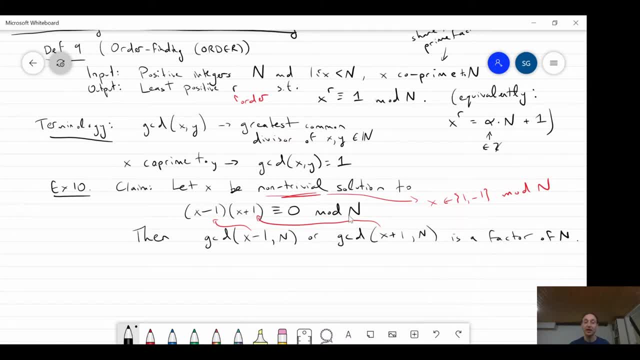 or n doesn't divide either of the brackets, um, but the prime factors of n kind of split up and some of them will divide this bracket, some of them will divide this bracket. right, those are the only ways this could work, and the first two uh paths i told you are actually impossible, right. 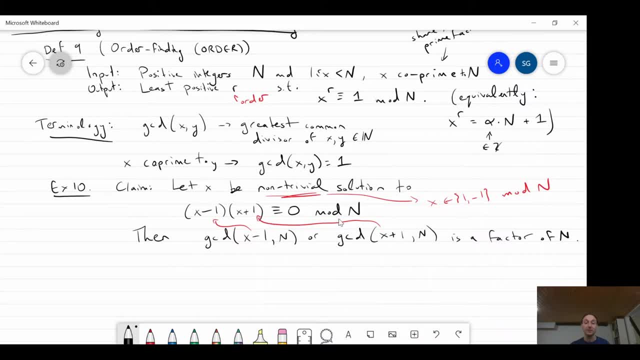 because we're we're asking for a non-trivial solution, right? so, um, we assumed that, um, so note that we assumed a non-trivial solution, which, for example, means that we don't want x to be equivalent to one mod n, and of course, this is the same thing as saying that, um, it's not true that x 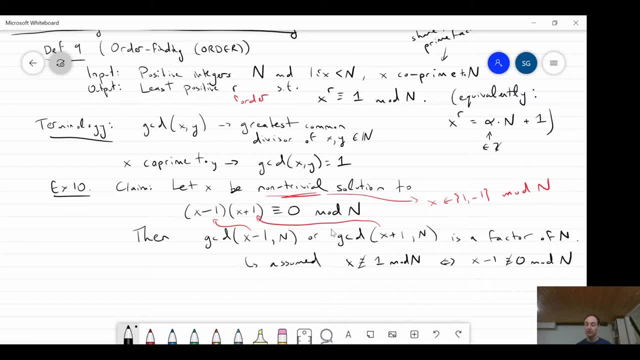 minus one is equivalent to zero mod n. okay, or in other words, we're assuming a non-trivial solution- means that n does not divide x minus one. okay, so it just doesn't divide this and it also doesn't divide this. that's the other assumption and therefore, um, the only way this division could. 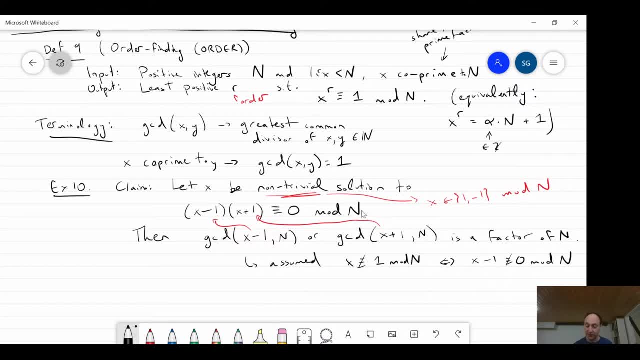 happen is that the prime factors of n, you know um. if, for example, if n is equal to p times q, for example, right then, as we'll see, for you know rsa, then the only conclusion is that you know p, let's say, must divide x minus one and q must divide x plus one. 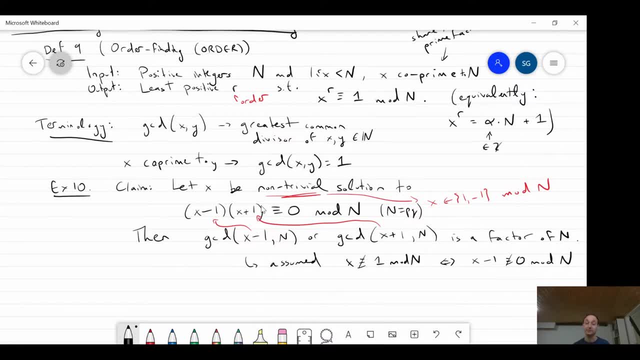 okay, or the other way around, okay, that's the only other way this division could work. okay, so, um, so that's why basically, um, and that's basically what they're saying. this gcd basically is that if x is equal to x minus one and n would return the prime factor of n that goes into x. 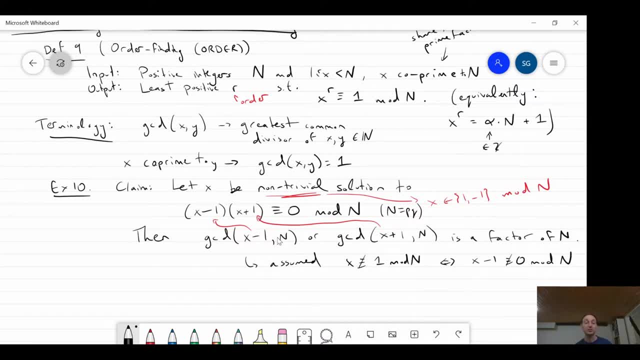 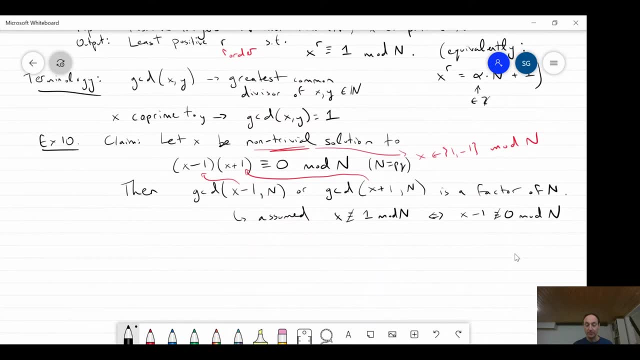 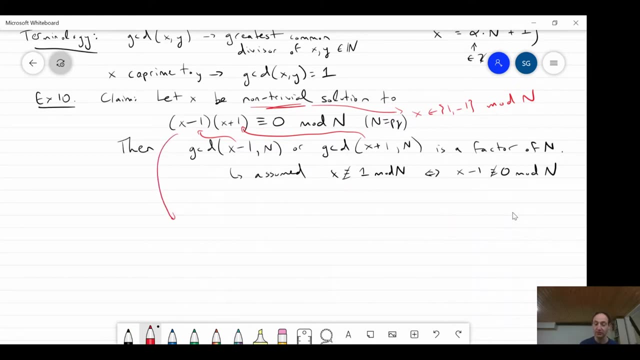 minus one in this case. okay. so this is, very briefly, um the intuition as to why this exercise um holds okay, why the claim holds okay. so all this is saying is that you know, let me rewrite this in a nice way, in a nicer way. so this equation, you know, this is just the difference of squares, right? uh, this is just the same as the. 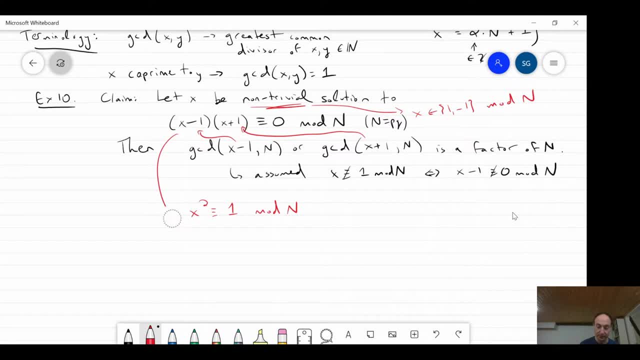 equation x squared is equivalent to one mod n. okay, that's all that is, and so what we conclude from this exercise is that finding a non-trivial solution x satisfying this thing allows us to factor in, or to, more accurately, to procure at least one factor event. 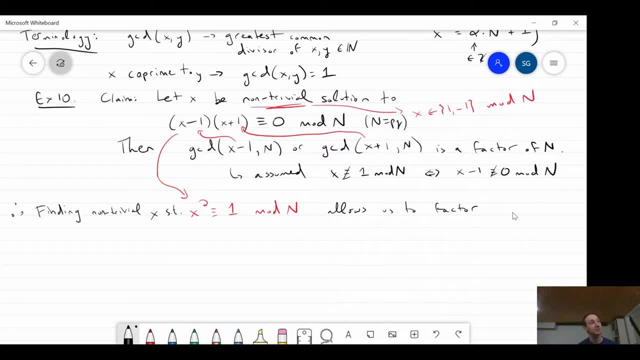 well, i suppose if you have more than one factor, multi, sorry, if you have multiple factors, the gcd of x minus one and then might not itself be prime, you know. but you can recursively keep applying this at this point, okay, but in our case, um, certainly for rsa n is always going to be a product of 2 prime, so um, the gcd will always. 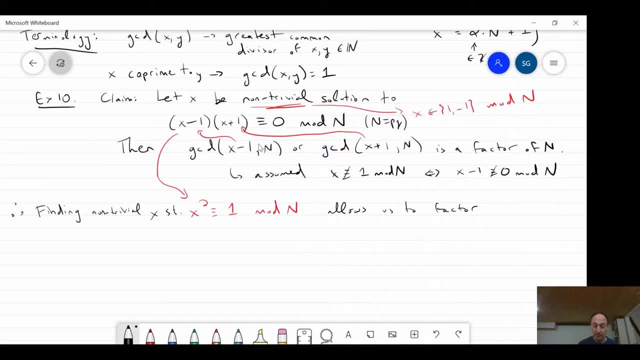 return for either p or qt. okay, so allows us to factor n, that's the, that's the first thing we take out of this. okay, so now we can kind of forget about um factoring. and now we're gonna say, you know, fixing n, which is going to be our composite value of gcd to x, to the power, and we're going to 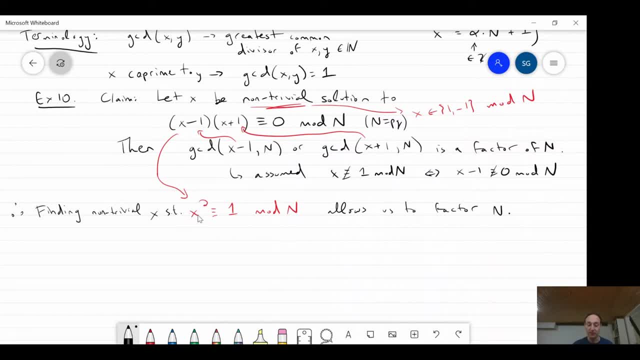 number we want to factor. how do we find a non-trivial x satisfying this equation? Okay, and you know this sounds very complicated, but it turns out like the simplest possible idea works, which is that. so the question is: you know how to find x, and here it pays off to be really stupid, and by that I mean all you have. 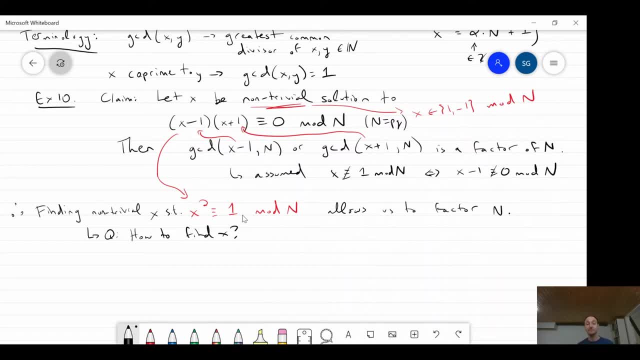 to do is pick a random x that, in addition, has to be co-primed to n. So the answer is: pick uniformly at random x. and here I want to start introducing some notation. So whenever I write down zeta, I'm referring to the set 0, basically the numbers mod. sorry, I'm referring to the. 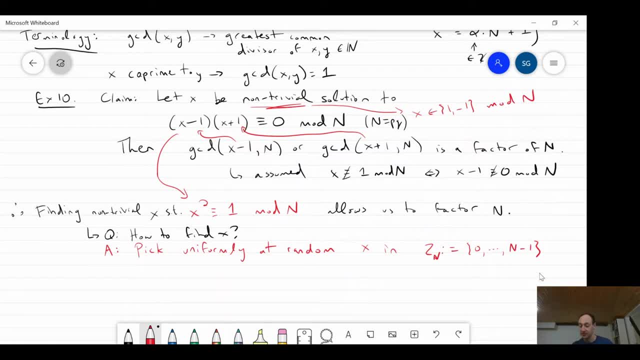 numbers mod n, the integers mod n, and so you're talking about this. set 0 up to n minus 1.. So pick an x uniformly at random from z n, okay, and additionally we need x to be co-primed to n, right, because n is not necessary prime in our 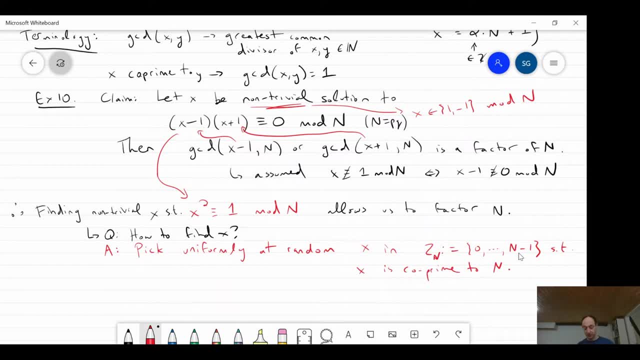 case n is a composite number p times q, so we need this additional restriction. Okay, and it turns out that when you do this, with high probability, if you can extract the order of r from x, so sorry. when you pick this x uniformly at random, it's order allows you to construct a solution to x. squared is equivalent to: 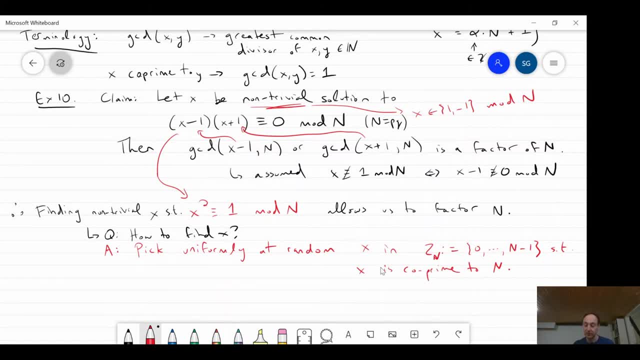 1, mod n in a non-trivial fashion. Okay, so basically to review, pick a random x co-primed to n, compute its order. and its order will allow you to solve this six habeas in a trauma model. So basically, closing off with an example: bind a multiple produto using all negative behaviors. plus a function of x, and we can then just have a nine, seven. another name, Alright, you wrote down some Japanese-scientific ones that make this rounding down, And we can check these new equations even though our names are not totally Theinternational-typen age that people find. the project that comes with this 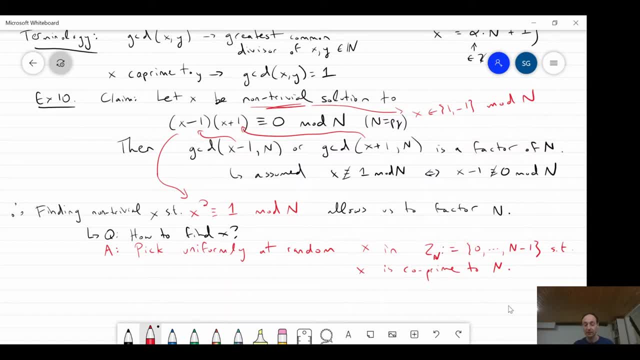 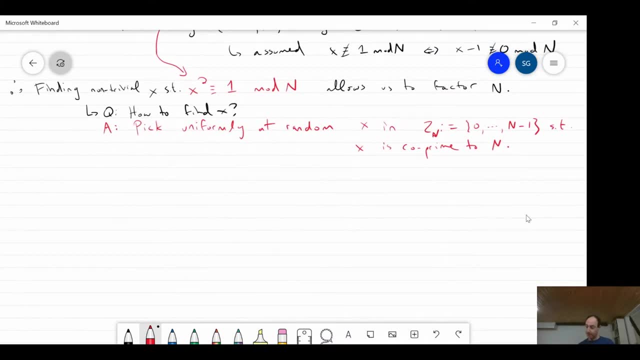 solve this equation: x squared is equivalent to one mod n. now i need to be more clear than that. of course, that's just the high level view. so let's give some of the intuition. okay, so maybe just intuition here. okay, so this is exercise 12. okay, so let's suppose let r be, and here i'm going to stress that r needs to be even. 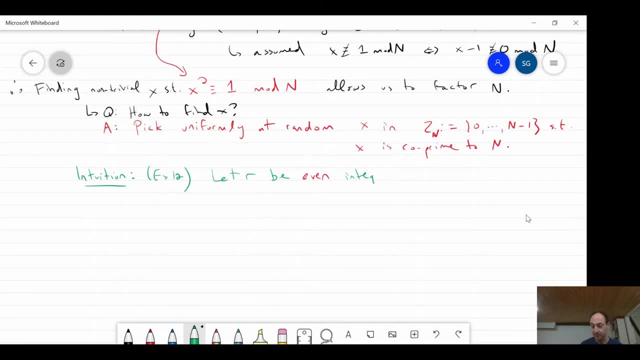 um, integer, satisfying, you know, x to the r is equivalent to one mod n. okay, and so i'm just going to give you a little bit of an example. i'm just going to give you a little bit of an example, so. so this is supposed to give you a little bit of the intuition as to why. 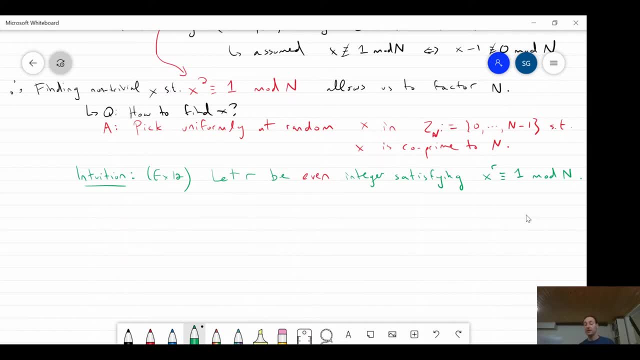 if you can find the order of an element x, then you can use it to find a solution to x. squared is equivalent to one mod n. okay, so how do we do that? well, let's assume we had some way of computing um finding an x who has an order r which is even. 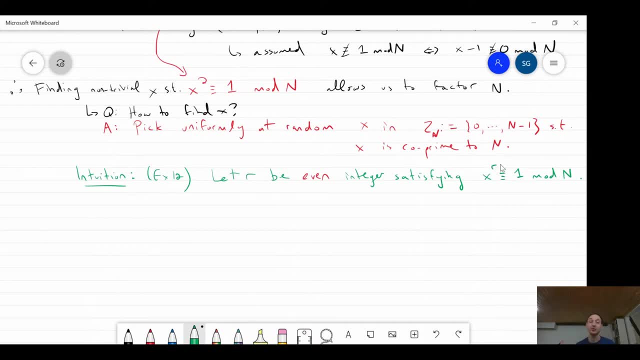 basically. so that's what this is saying, and suppose we can compute the order r right, for which later we're going to need the quantum algorithm. we don't know how to do that classically. well then the question is: you know you want to come up with? 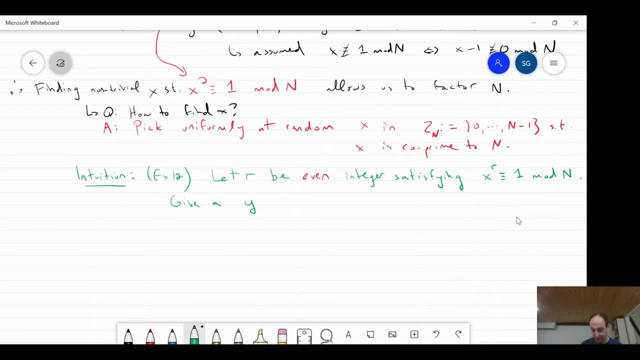 you know, give a y um satisfying y squared is equivalent to one mod n. okay, so, in other words, give me a y which satisfies this equation up here. okay, so how do you do this? you know, the obvious uh thing is this, right, uh, you know, if you think about it just a little bit, the obvious solution is that. 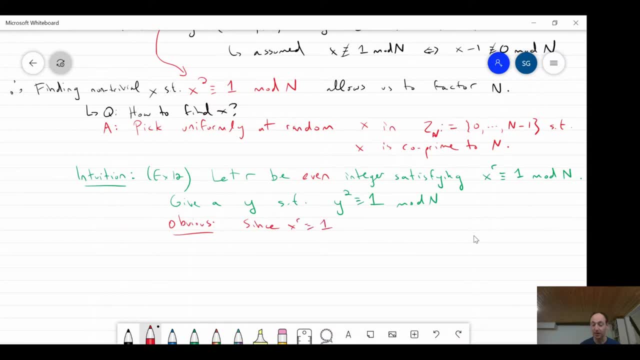 um, you know, since x to the r is equivalent to one mod n, right, then, certainly you know, x to the r over two times, x to the r over two, right? if you just take the square root, essentially is also equivalent to one mod n, and so let's just define y to be equal. 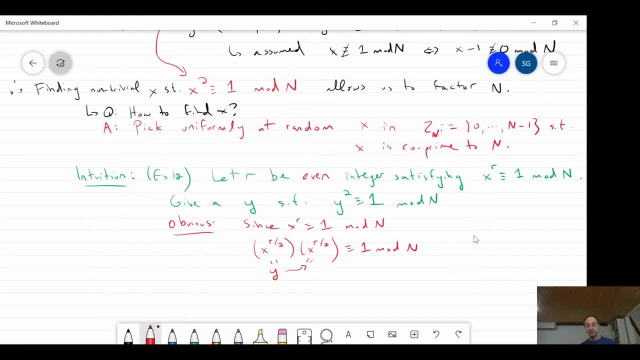 to this right, it's just x to the r over two. okay, so if i can find um, you know um, an x with an even order and i can figure out the order itself, then i could immediately kind of write down what y should be: x to the r over two. 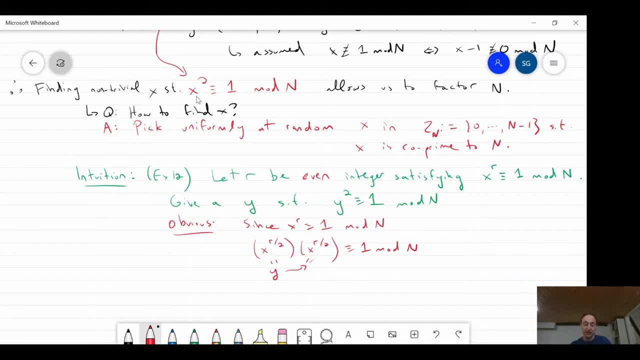 right, and then i'll know for sure that it'll satisfy this equation: x squared is equivalent, or y squared is equivalent to one mod n. now of course this is not enough because, remember, we said we want to find x first of all. not obvious how to do that, right, so we're going to randomly. 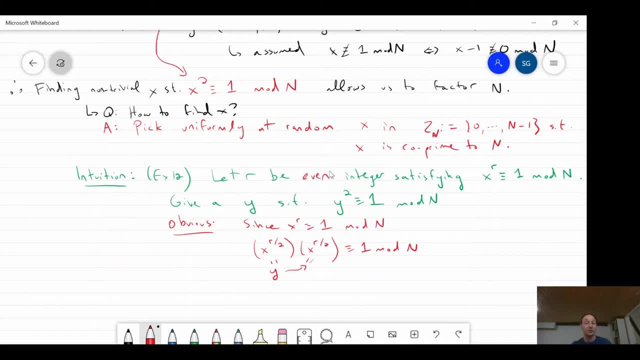 sample. we're going to cross our fingers and hope that that x has an even order, number one and number two um. it's not enough just for y to satisfy this right. we also needed y- um to be a non-trivial solution to this equation right. we didn't want the trivial. 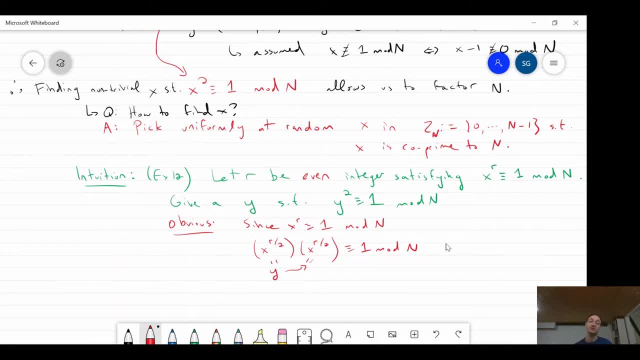 solutions. so we have to argue now that random sampling allows us to find an x with high probability which has an even order, and so that the square root of x to the r, this thing over here, that thing- is not going to be a trivial solution to this. 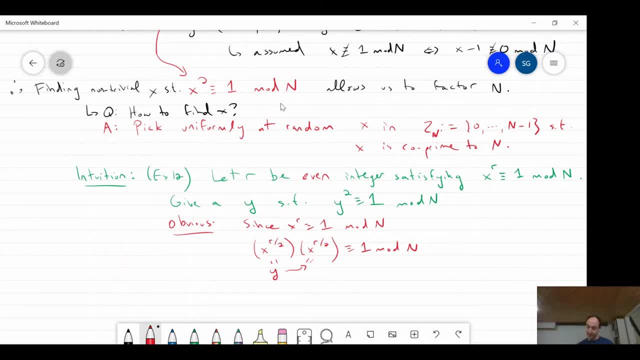 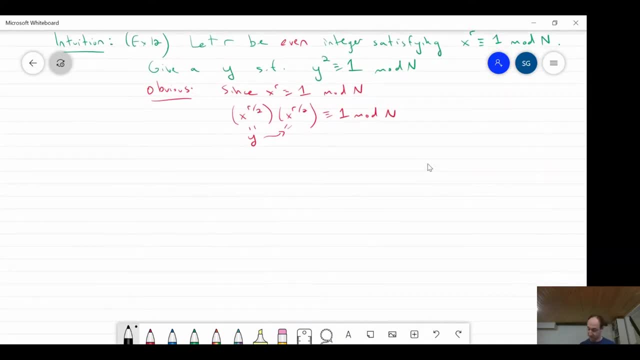 it will be a non-trivial solution to this equation. okay, and so that leads us into um, the next kind of heading which says: you know how do you find a non-trivial solution to x? squared is equivalent to one mod n. okay, so for this we're going to have to take a little bit of a detour into number. 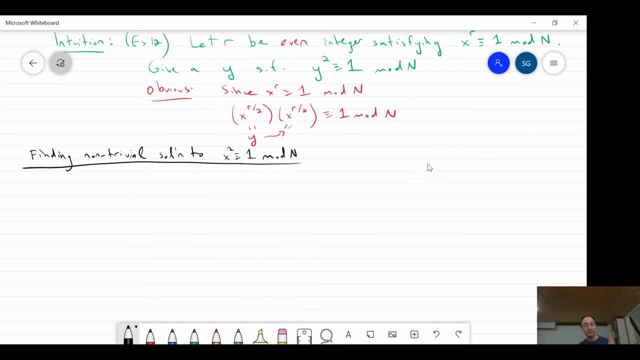 theory, and i think it's um worth seeing some of these facts again, because, um again, you've probably seen these at some point, but you know, the last time, for example, we did a little bit of a detour into number theory, and i think it's um. 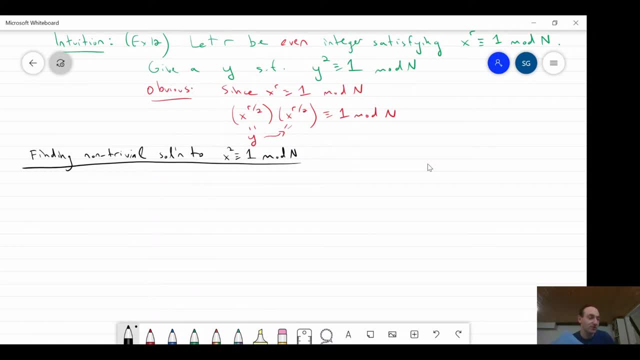 worth seeing some of these facts again, because, you know, the last time we did a little bit of a detour into number theory- and i think it's um i learned about the chinese romanian theorem was, you know, aside from shore's factoring algorithm, of course it was um, i think. 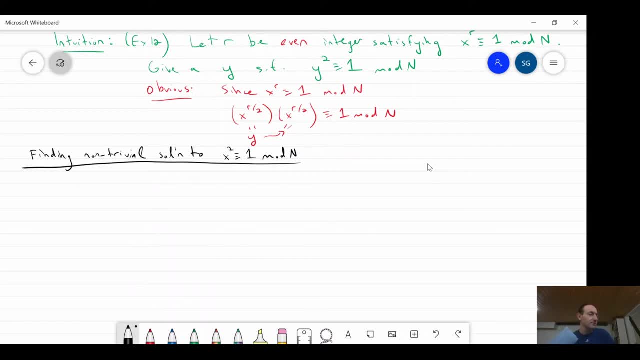 first year of undergrad at the university of waterloo, i mean, um, so it had been a long time since i'd seen it. so i think it's a good idea to to make sure to write these facts and just to refresh your memory of them, and maybe some of these you haven't seen before. 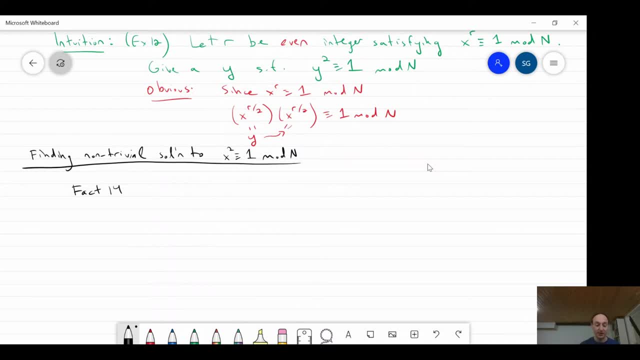 but basically to prove what we need to prove, we need three facts. i'm going to write them down as facts 14, 15 and 16 in the notes. the first one is fermat's. fermat's um little theorem, and i'm just going to abbreviate this. 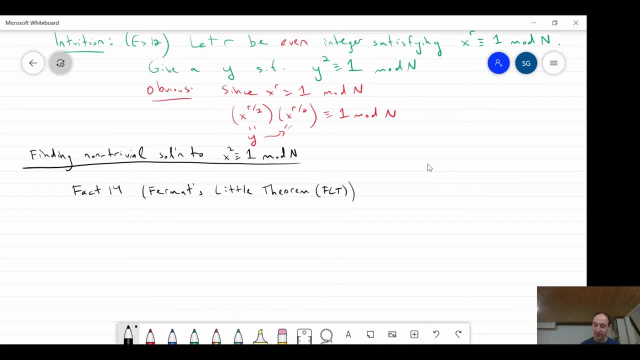 theorem, you know it's. it's funny how, when you spell things wrong, it's like it's almost like your. your brain has a spasm for a second when it sees it like a like a spidey sense. anyway, um, fermat's little theorem, right. 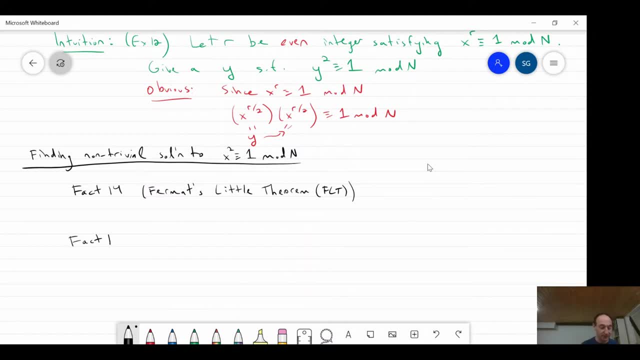 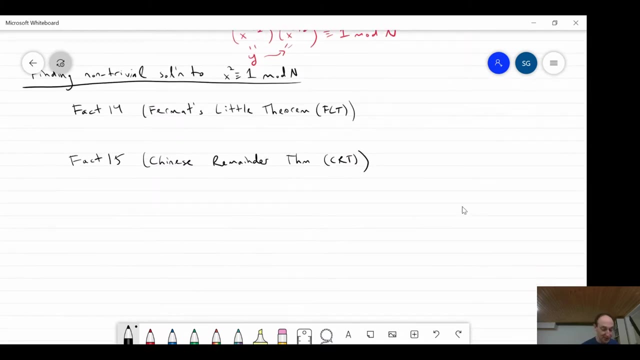 uh, is the first one i'm going to write down. the second fact i'm going to write down, fact 15, is the chinese remainder theorem, print and sugar, blah, blah. let me come back here, okay, and abbreviated, just crt here. and finally, the last fact, which is, i mean, out of all the facts of the, perhaps the one you 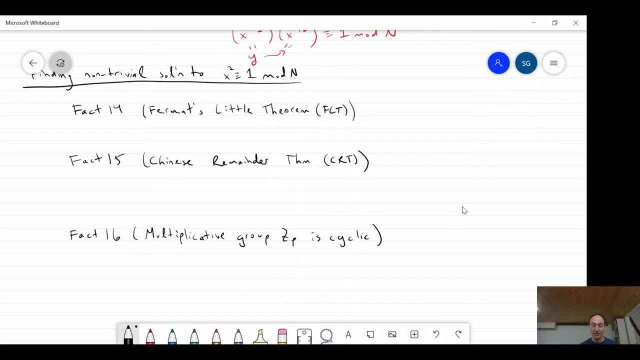 me or may not be familiar with is. i'm just going to write it as the Chris anticipations. you know there's a group theory that's underlying all of this, but you know nothing of what I'll talk about, will really mention the words group theory and you don't really need to know it to. 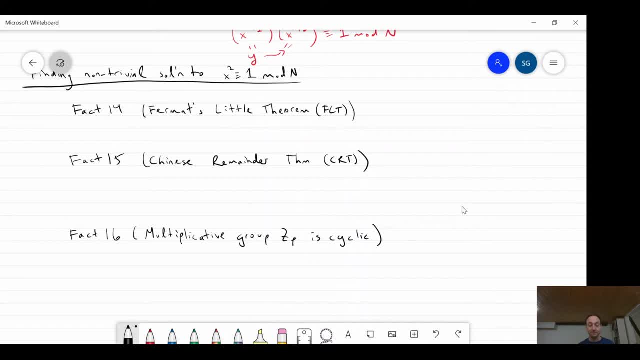 prove some of these basic facts. basically okay. So again, as the quote atop last lecture by John von Neumann said, you know a lot of mathematics is not. you know it's not really understanding the math and there's a sense in which you never really understand it. it's more. you just have to. 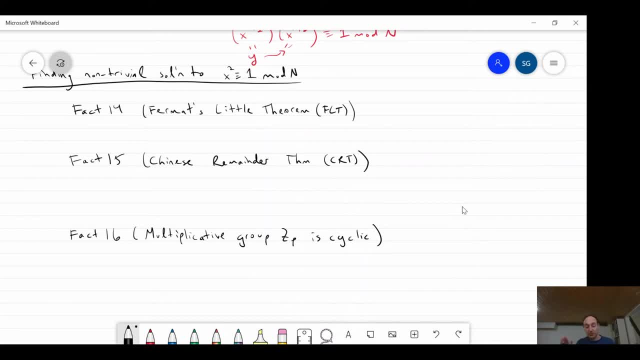 get used to it, right. And so, again, group theory is another example where, once you get used to it, it makes sense. but even without really knowing the formal words group theory, you know you can make sense of a lot of this just by thinking of it long enough. okay, So let's start with. 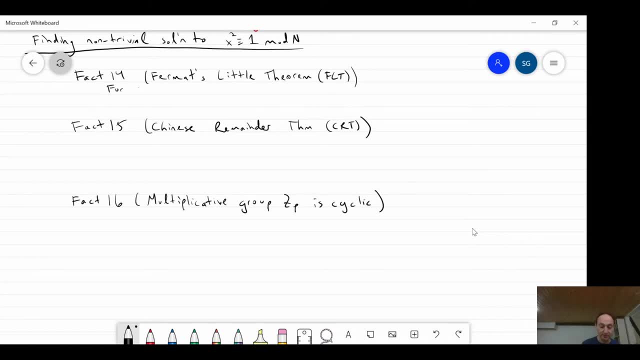 Fermat's Little Theorem. It says, for any prime p, an integer a a to the p is equivalent again to a mod p. Okay, And moreover, and the version we'll be using here, if the prime does not, whoops. 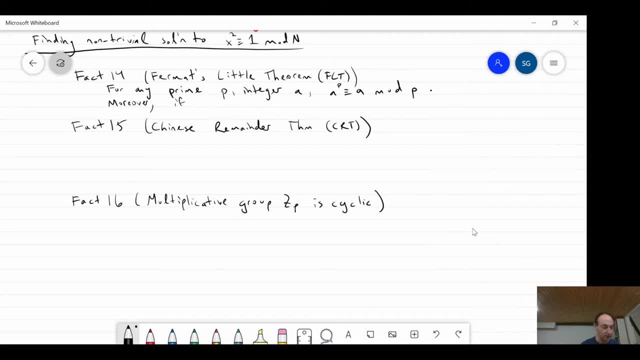 let me not use that notation. I'm also trying not to use division notation if p does not divide a, so then you can say something even more, which is that a to the power p minus 1 is actually equivalent to 1.. 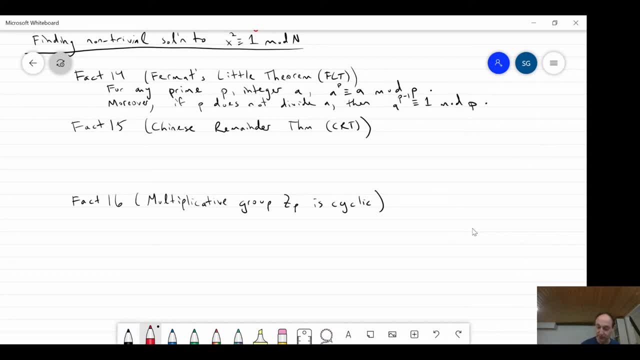 Mod p. okay, So this is the version we're going to use. So you know, if you give me an integer a and a prime p, so that p does not divide through a, then you know this equality to 1 holds. 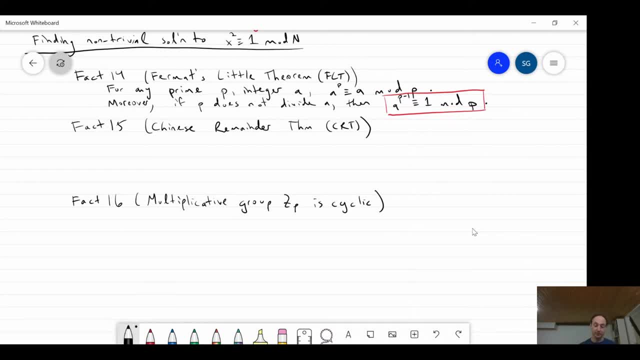 Okay, so that's Fermat's Little Theorem. Let's state the Chinese Remainer Theorem. So this basically says that maybe I'll start writing it here. So let's start with a set of integers larger than 1.. So I give you a set of integers, m1 through mn be integers greater than 1.. 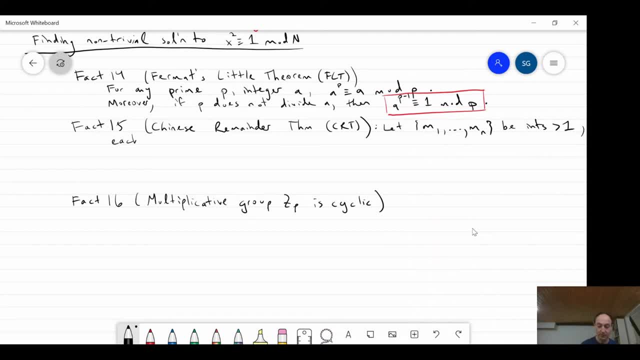 Okay, And each pair of which is co-prime Okay. so what that basically means is that if I take any- you know, mi and mj- from this list that are distinct, then they're both co-prime. their gcd is 1.. 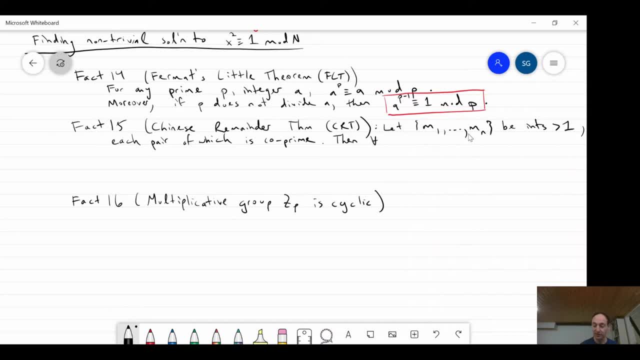 Okay, Then you know, for any other set of integers you could give me a1 through am an sorry. the following linear system. So I'm going to write down a system of equations and the claim is going to be that this system will always have a solution. 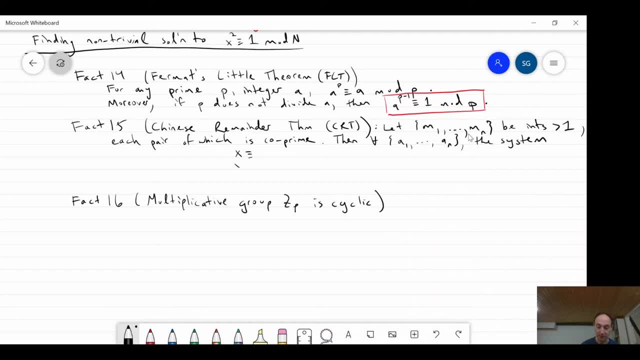 So we have: x is equivalent to: so all of these are the same on the left, right. Okay, I'm going to write down a system of equations. So the first thing, let's fix the moduli. So those are the m1, m2 that you started with, Right? These are these bad boys over here, right? 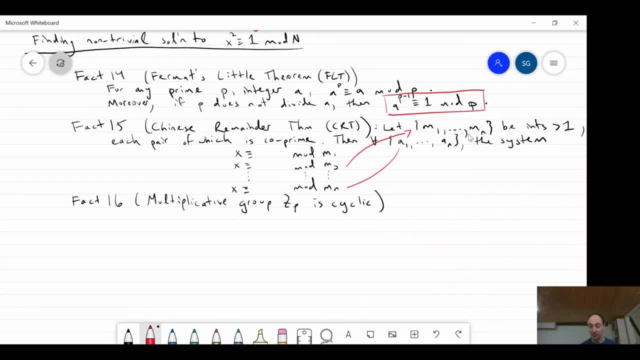 And so the other thing I need are: you know what should x be equivalent to Mod each of these moduli which are co-prime? And then there we're going to write, you know, a1, a2,. 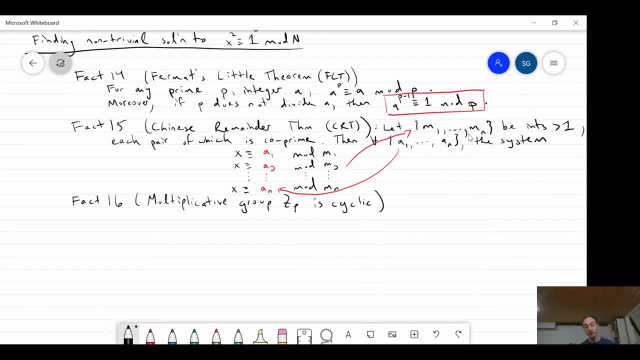 up to am Okay, And so you should think of it this way, that you know these, you should think of these moduli as being just fixed, you know, And what's kind of a variable here is? you know what is the equivalence right? 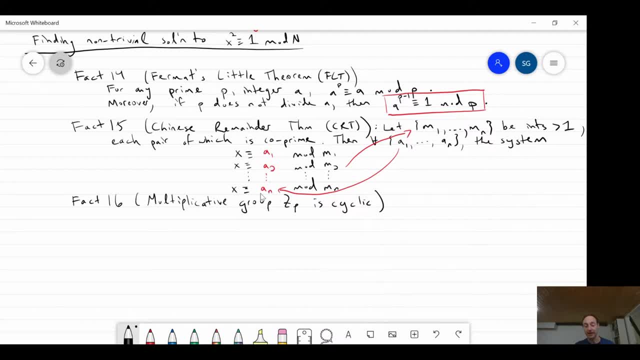 What is the sequence of numbers you write down here in terms of the moduli, And what this is basically saying is that always has a solution. Okay, So in other words, you know, if we fix the moduli, no matter what sequence of integers- a1 through an, you write down basically: 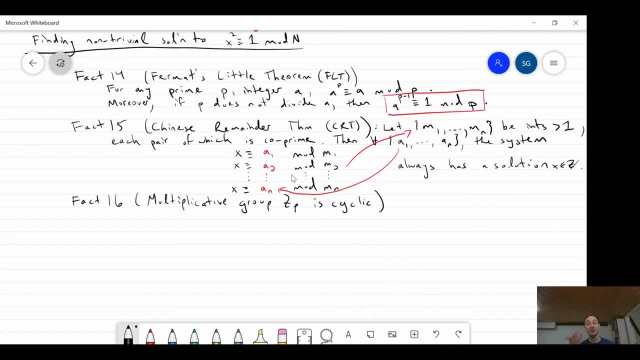 there's always some x which will satisfy all these equations simultaneously. Okay, And also x. how did I want to write this? Basically, you know, all the solutions are equivalent to modulo the product of the prime, So let me more. 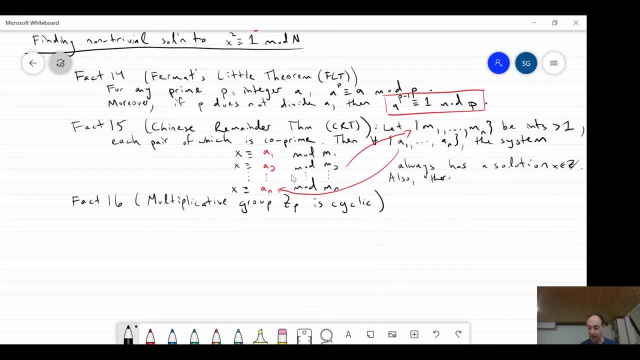 There are multiple solutions, but there is a unique, such x, which is in the range you know: 0, dot, dot, dot up to m, which you know is just the product of these moduli. Okay, Let's see if I could move this thing, because it's getting in my way and I'm not very happy. 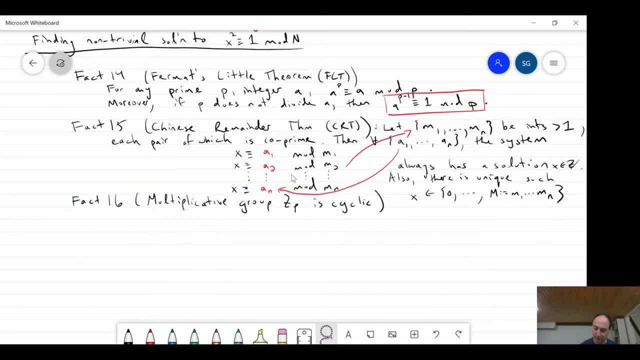 It's not very happy. Okay, It's not good to be unhappy with these things. right, We will do what we can to fix it. No, Oh, maybe I need to use my mouse, Is that right? Hey, no, not good. 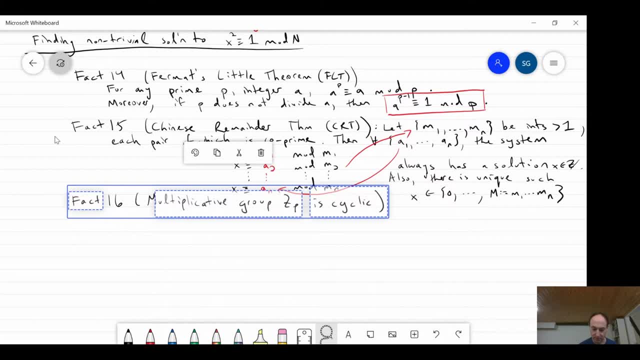 All right. well, maybe, Why is it not All right? maybe we'll just leave it for now, Okay, Okay, so that's the Chinese remainder theorem, right, And basically it just says this: that intuitively Is this an exercise here. 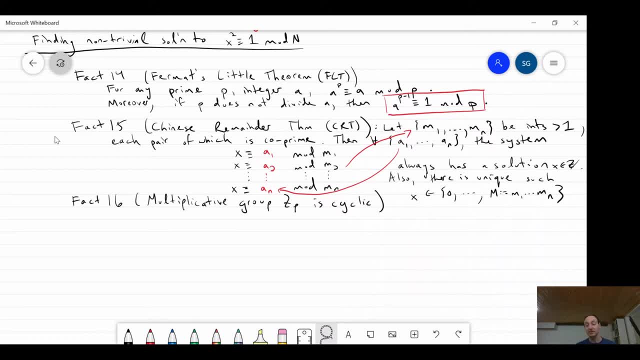 So okay, intuitively, what the Chinese remainder theorem is going to buy us is that you know, instead of talking about you know x mod, capital, M, right, we can instead talk about. you know each of these integers a1 through an mod, each of these moduli, right. 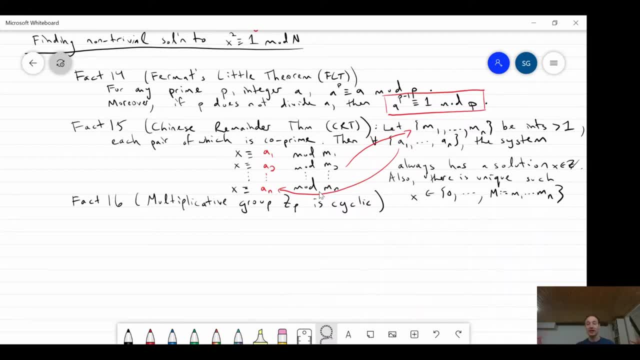 You can kind of switch back and forth between these so-called global view, which is mod, capital M, and the local view, which is, you know, mod, each of these little m1 through mn Okay, and it'll turn out that there's a bijection between these two sets. 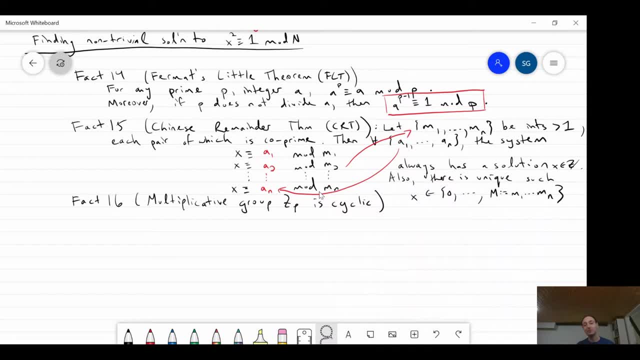 They're completely. You can always map between any a1 through an to some unique x and vice versa. Okay, And the last fact I'm going to give you this multiplicative group. Maybe I'll just put some underlines to kind of separate these things just a little bit. 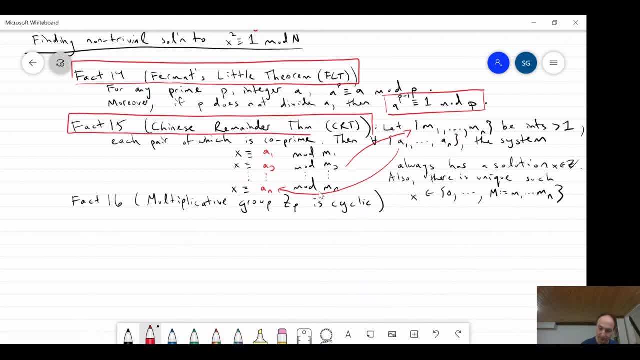 Okay, Probably should have left a little bit more space. So this fact. what it basically says is the following: It says that fix any positive prime p- Okay. Then there exists a so-called generator- Okay, Just a fancy name- In the set zp. 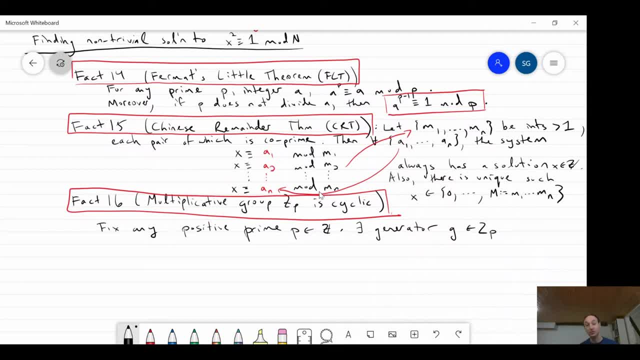 Okay, So remember this is going to be the integers from 0 up to p minus 1.. So there's some integer in that range, basically such that any non-zero element e which is also in that set can be written: g to the k is equivalent to e. 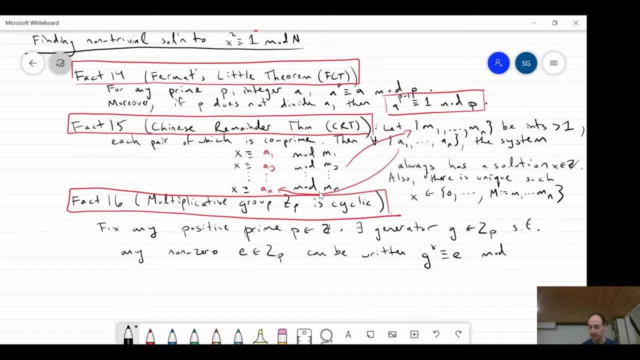 mod zp: Okay, And this is for some k, And k is also. Well, k is in this range. Again, it's non-zero, Okay. So what this is basically saying is that, in fancy terminology, this just says that if 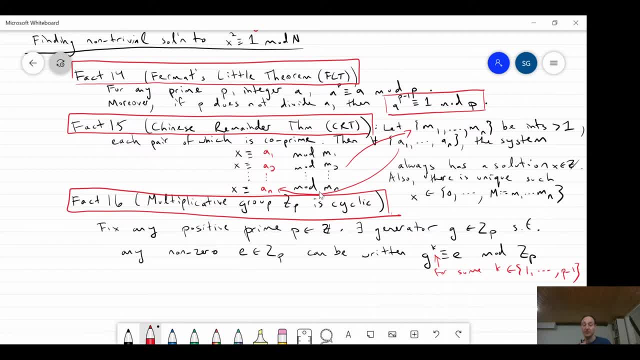 p is a prime, then this zp is basically going to be a cyclic group. What does that mean In plain language? It just basically means that, as long as we're talking about the number 0 up to p minus 1, for p being a prime, if you want any number in that set, let's just call it e, you could. 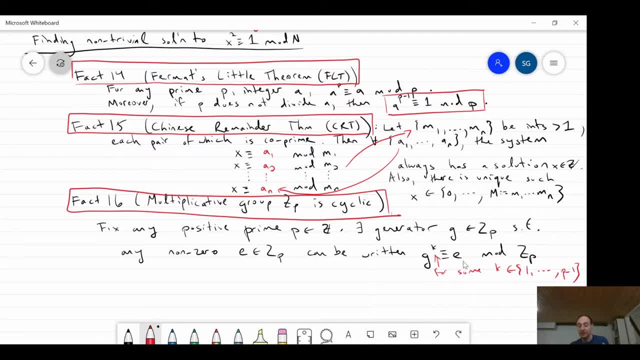 always generate that number equivalently, Instead of writing the number down. there's some magical version of g which is for any p. there's some fixed choice of g. Okay, So you tell me p and I fix g. And whenever you pick an e- now any other element- you can always generate it just by. 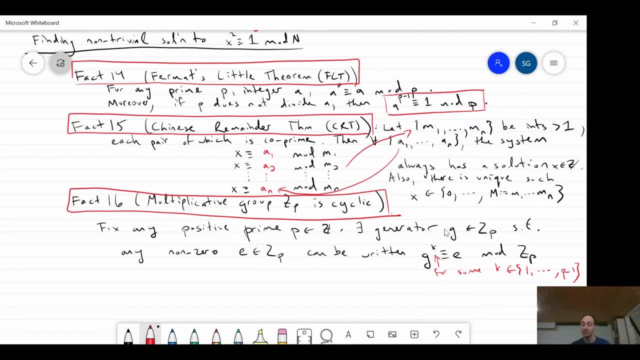 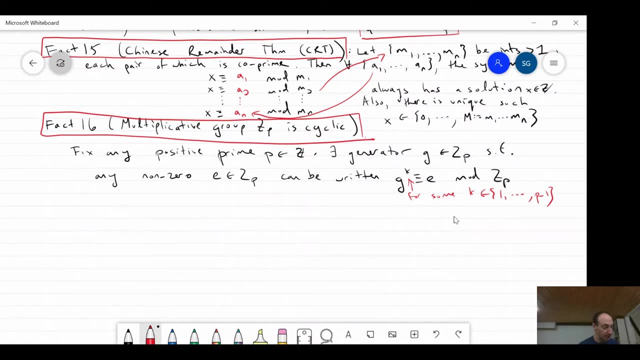 raising g to a sufficiently high power. Okay, So that's why g is called a generator. It just generates this entire set, basically from 1 up to p minus 1, just by taking higher and higher powers. Okay, And so one thing I want to mention is that, you know, by combining, you know this fact. 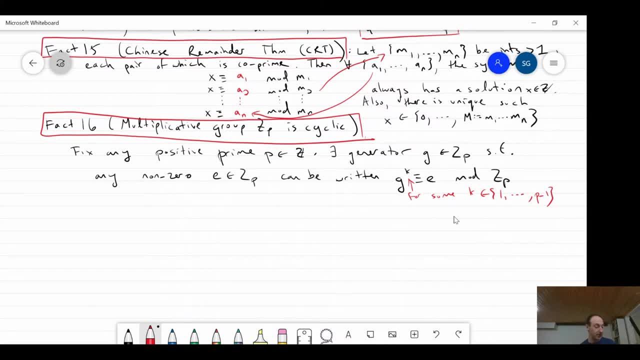 here this generator fact with Fermat's Little Theorem, you know, in exercise 17, basically. so if you're combining this with Fermat's Little Theorem, maybe I'll try and keep that on the page for a second. Yeah, 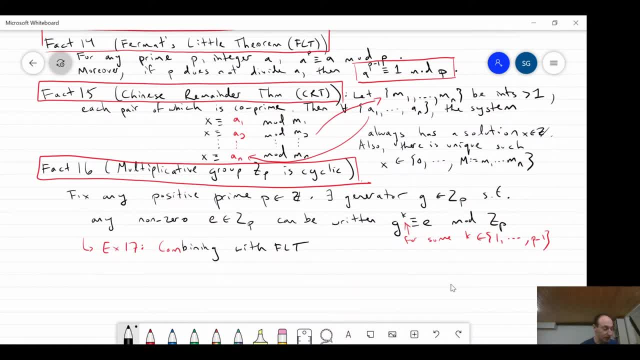 So if you combine this with Fermat's Little Theorem, what it basically says is that there exists a bijection, Okay, A one-to-one onto map, basically between elements, Okay. So what I'll do is I'll take this e and powers k. 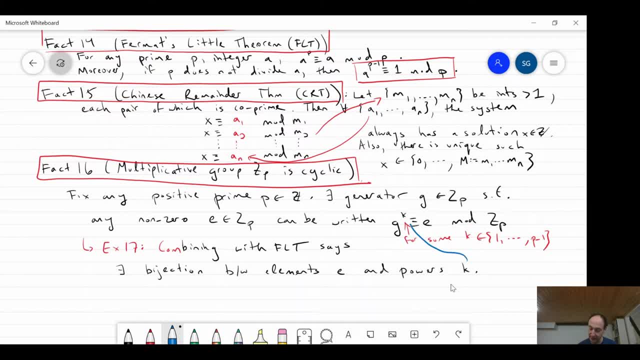 Okay. So when I say powers k here, I mean I'm talking about this k over here, right, And e is referring to this e. Okay, So you know. what this basically just says is that you know, I can think of picking. 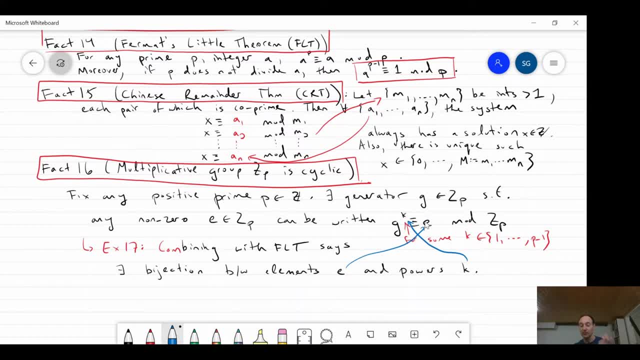 a random element of z- p in two equivalent ways, right? One way is I could just pick a random element, e, But equivalently, remember g is fixed, conditioned on the choice of P. so equivalently, instead of picking E, I can. 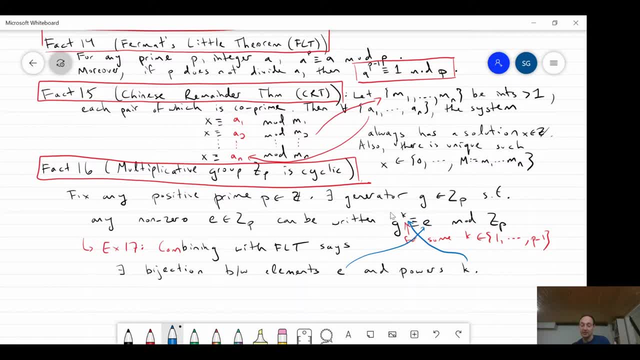 instead, just pick a uniformly random K in this range and you know, for any fixed K there's a unique E, and vice versa. so you know, whether I randomly sample E's or K's, it doesn't matter, it's completely equivalent. okay, okay, so this implies that randomly sampling E is equivalent to random sampling K. okay, there's a. 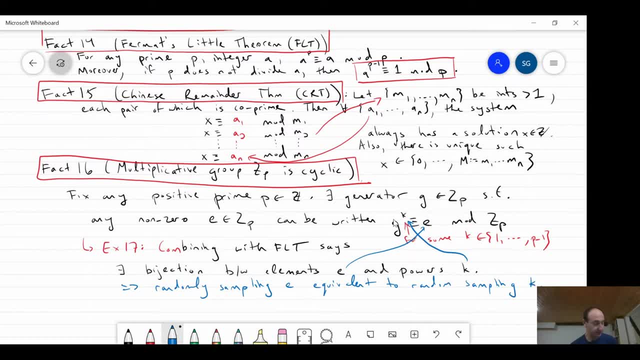 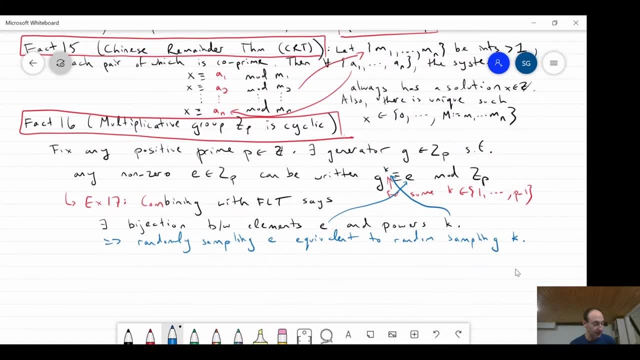 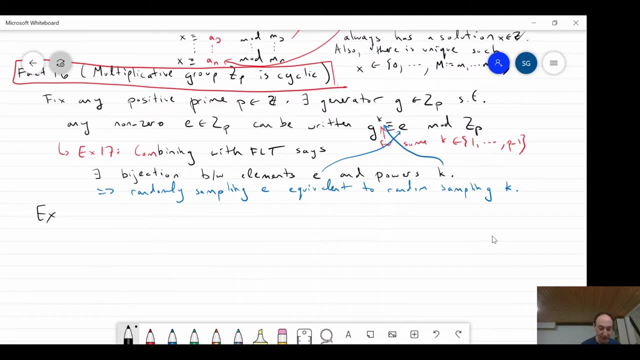 one-to-one onto correspondence. okay, so here these are just a bunch of facts. let's just do a quick exercise so that we're just a little bit comfortable with this order stuff. so this is not a fact, but you know we'll get used this idea in this proof will. 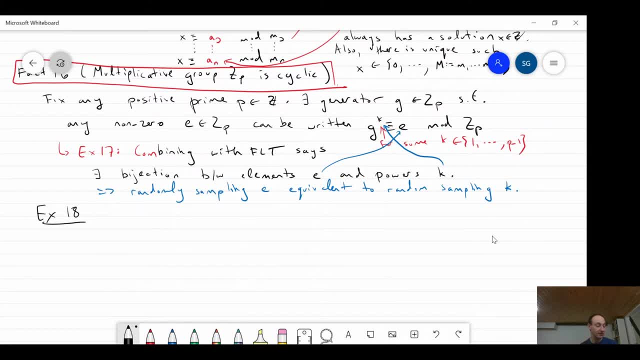 get used, so I do put it here, and so make sure you understand both of these exercises before you continue. I think it's it's good to do exercise 17 and 18, so pause the video and do them. so this just basically says that let R be the. 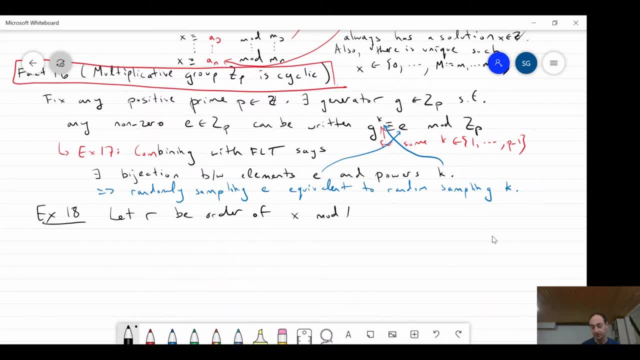 order of X mod N. okay, and let's consider some X prime, sorry, some R prime. okay, and let's consider some X prime, sorry, some R prime bigger than R, right, that also satisfies this type of equation. right X to the R. bigger than R, right, that also satisfies this type of equation. right X to the R. 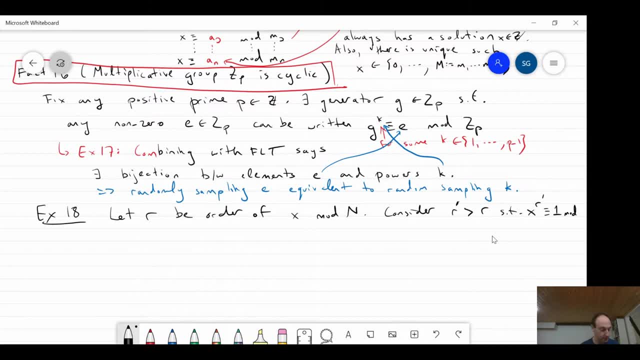 prime, just like X to the R, is equivalent to 1 mod N. okay, and the claim is that R prime divides R. okay, so if I have any number bigger than R that also satisfies this type of equation, then it's always true that R prime is just some multiple. 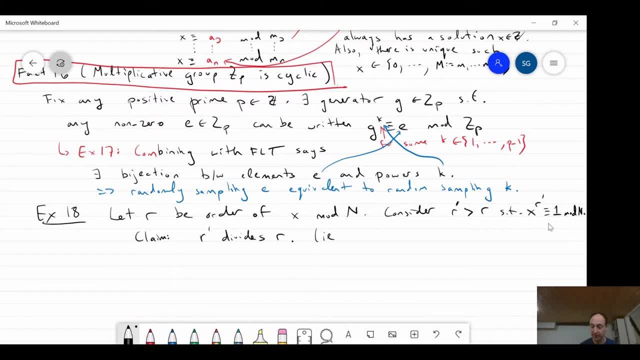 this type of equation, then it's always true that R prime is just some multiple of the. this type of equation, then it's always true that R prime is just some multiple of the actual order R. so ie, you know, R prime just equals to some alpha times, R, right? 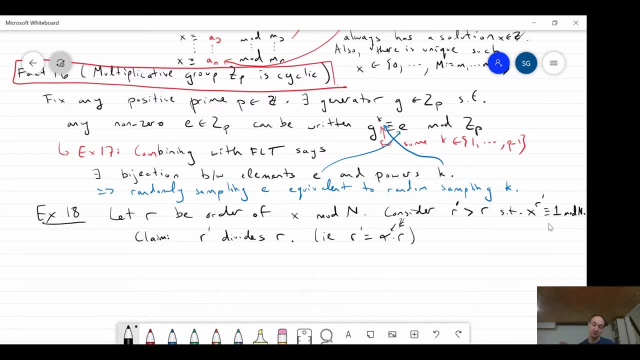 actual order R. so ie you know R prime just equals to some alpha times. R right. actual order R. so ie you know R prime just equals to some alpha times. R right for some integer. let's say positive for some integer. let's say positive for some integer. let's say positive integer alpha- okay. so why is this true? 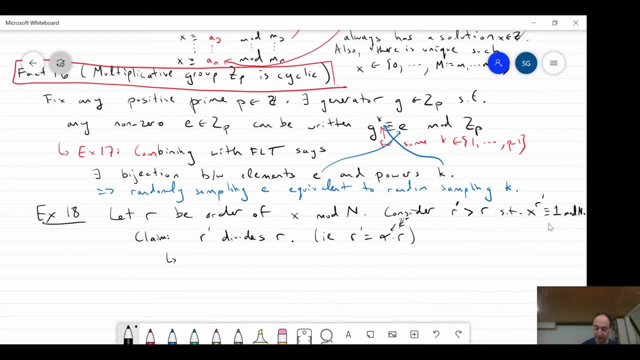 integer alpha- okay, so why is this true? integer alpha- okay, so why is this true? well, let's just look at you know, here's well, let's just look at you know, here's. well, let's just look at, you know, here's a proof sketch. and again, the point of a proof sketch. and again the point of a proof sketch. and again the point of this is just to just a little bit of this is just to just a little bit of this, is just to just a little bit of practice with this before we get into practice with this, before we get into. 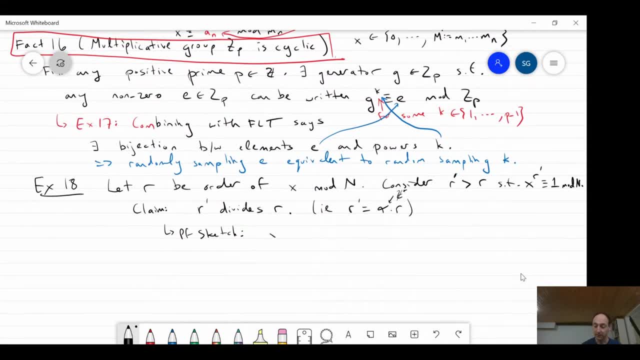 practice with this before we get into some more serious proofs, right? well, what some more serious proofs? right? well, what some more serious proofs? right? well, what is X to the R prime, right? well, I know? is X to the R prime, right? well, I know, is X to the R prime right? well, I know that. well, if I have X to the R prime a. 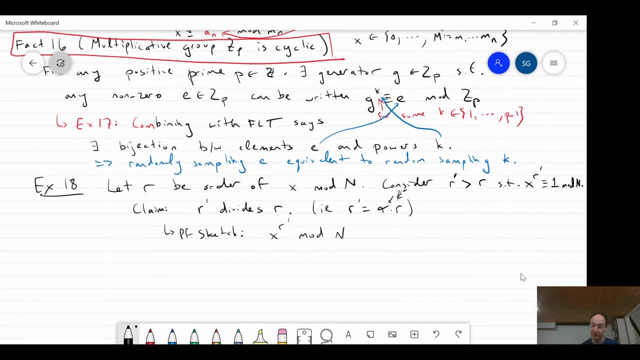 that well, if I have X to the R prime a, that well, if I have X to the R prime a mod n, basically, whatever that equals to mod n, basically, whatever that equals to mod n, basically, whatever that equals to you right, we know it equals one of. 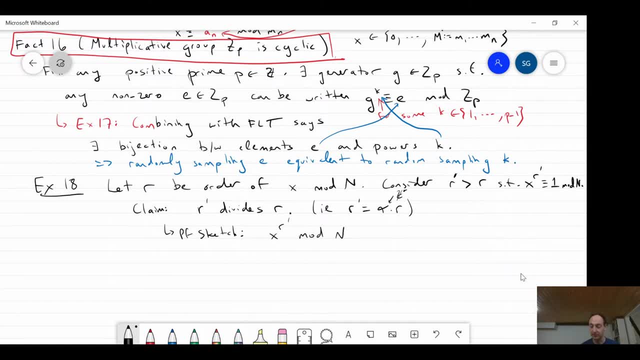 you right, we know it equals one of you, right, we know it equals one, of course. I know that X and the R is course. I know that X and the R is course. I know that X and the R is equivalent to one mod n right, and I know. 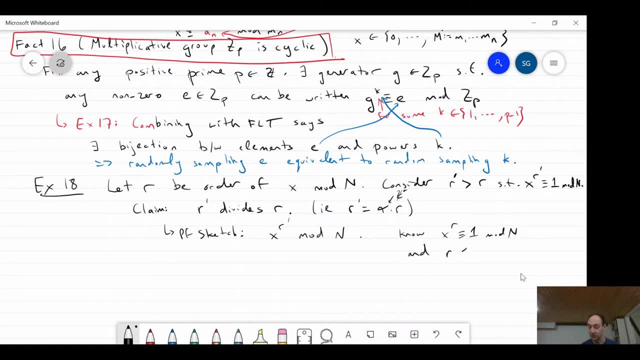 equivalent to one mod n right and I know equivalent to one mod n right, and I know that and R is strictly smaller than R that and R is strictly smaller than R that and R is strictly smaller than R prime right. so what I can always do is I: 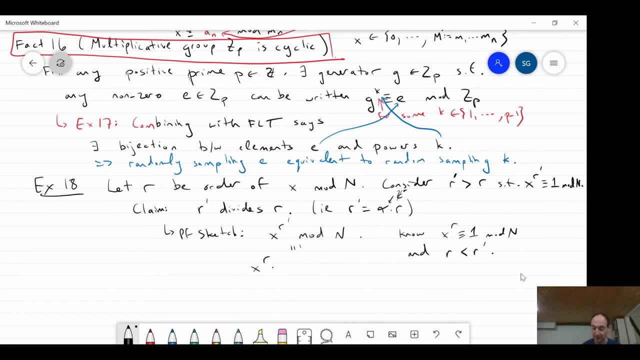 prime right. so what I can always do is: I prime right. so what I can always do is: I could always rewrite this, as you know. X could always rewrite this, as you know. X could always rewrite this, as you know. X to the R times, X to the R prime minus R. 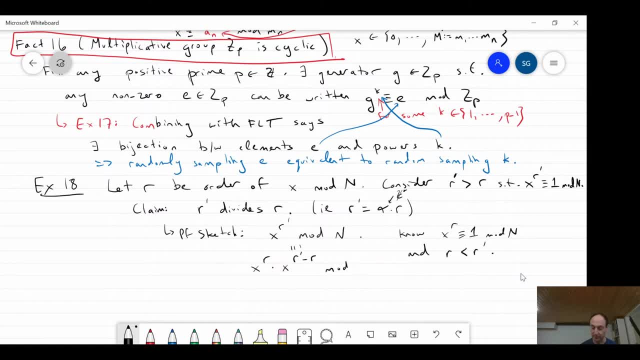 to the R times X to the R prime minus R. to the R times X to the R prime minus R. right, just just trivially right. I didn't right, just just trivially right. I didn't right, just just trivially right. I didn't do anything interesting, mod n right. but 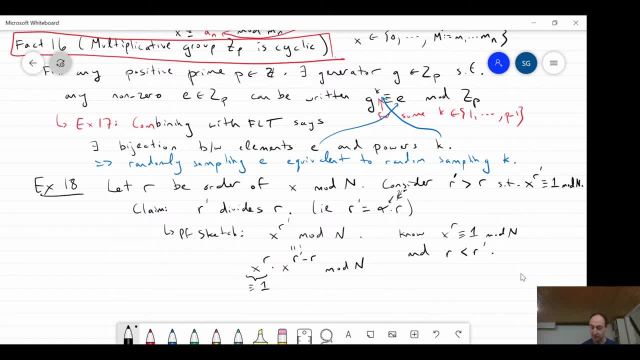 do anything interesting mod n right. but do anything interesting mod n right. but this, I know, is equivalent to one right. this I know is equivalent to one right. this I know is equivalent to one right. here it is right. I assume this fact up. here it is right, I assume this fact up. 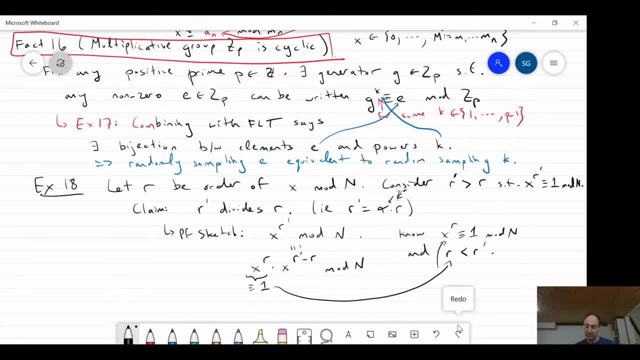 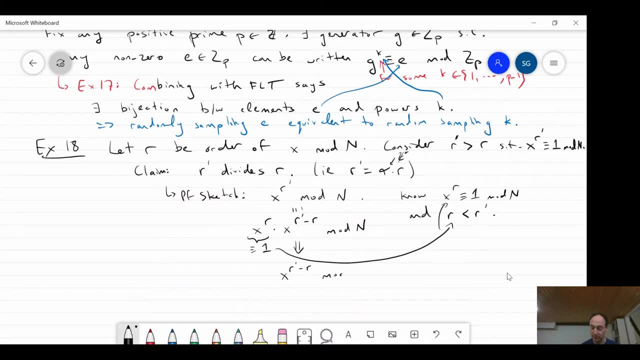 here, it is right, I assume, this fact up here. well, technically up here, right. so here. well, technically up here, right, so here. well, technically up here, right. so this now implies that X to the R prime. this now implies that X to the R prime. this now implies that X to the R prime minus R is also okay, is also equivalent. 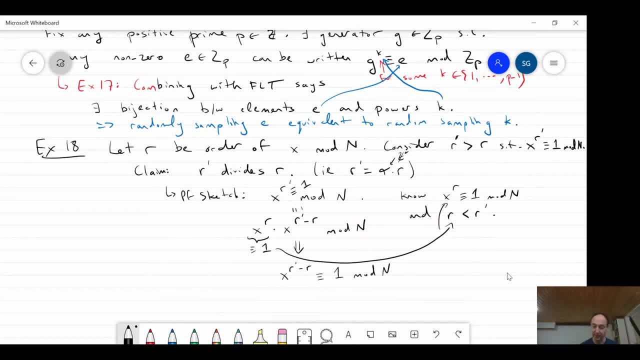 minus R is also okay, is also equivalent. minus R is also okay, is also equivalent to one mod n, right? because, well, this was to one mod n, right? because, well, this was to one mod n, right, because well, this was equivalent to one mod n. and all I did is: 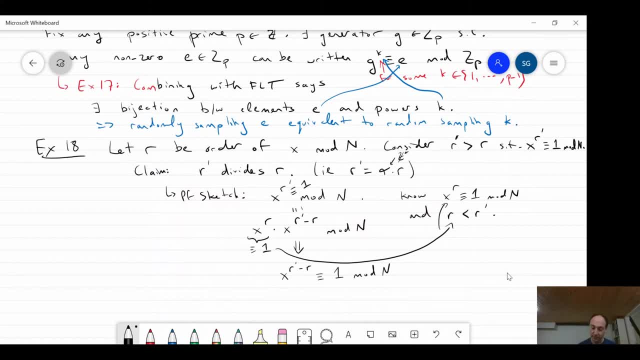 equivalent to one mod n, and all I did is equivalent to one mod n. and all I did is I just kind of cancelled off some. I just kind of cancelled off some. I just kind of cancelled off some redundant part on the left, so maybe I redundant part on the left, so maybe I. 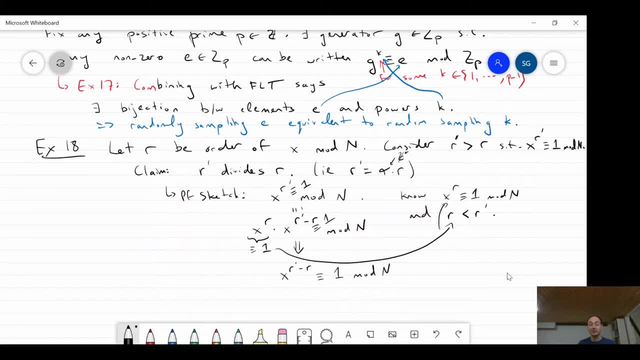 redundant part on the left. so maybe I could add this in right and now you can. could add this in right and now you can. could add this in right and now you can just keep repeating this right. you can just keep repeating this right. you can just keep repeating this right. you can keep subtracting off copies of R right. 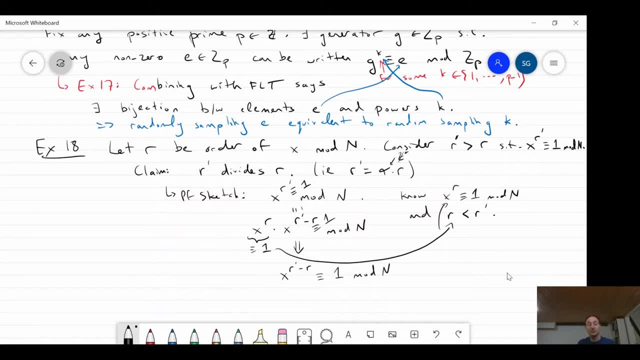 keep subtracting off copies of R right, keep subtracting off copies of R right, and what's gonna happen is eventually, and what's gonna happen is eventually, and what's gonna happen is eventually. you know, either the exponent will go to you know, either the exponent will go to. 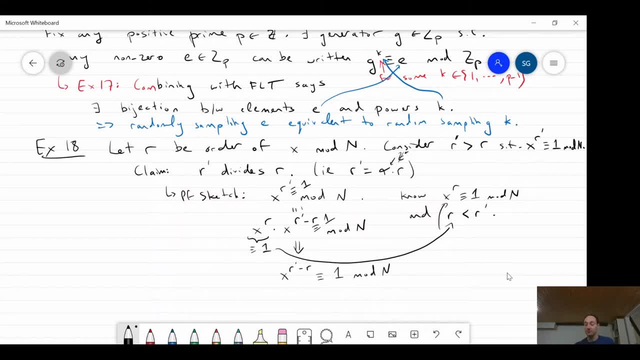 you know, either the exponent will go to zero of course, in which case you zero of course, in which case you zero of course, in which case you, perfectly divided through our prime of R, perfectly divided through our prime of R, perfectly divided through our prime of R. meaning, you know, indeed, our prime was a. 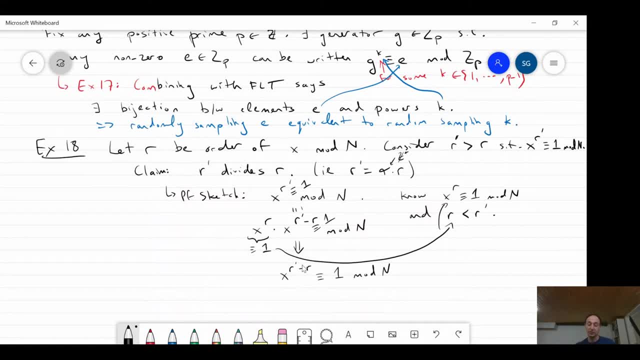 meaning. you know, indeed, our prime was a meaning. you know, indeed, our prime was a multiple of R. or you're gonna end up multiple of R, or you're gonna end up multiple of R, or you're gonna end up with an exponent which is strictly, with an exponent which is strictly. 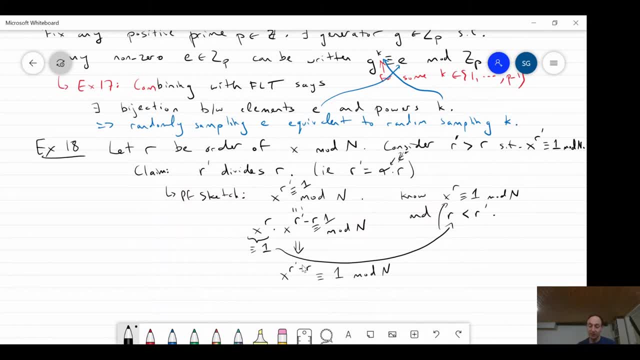 with an exponent which is strictly smaller than R the order right, and at smaller than R, the order right, and at smaller than R, the order right, and at that point you're gonna have something. that point, you're gonna have something. that point you're gonna have something. like you know, you have X to the let's. 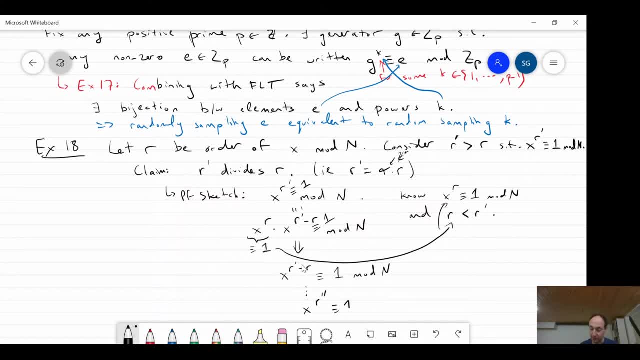 like you know, you have X to the let's. like you know, you have X to the. let's call it our double prime. whatever that call it our double prime, whatever that call it our double prime, whatever that is right, is equivalent to 1 mod n- right. 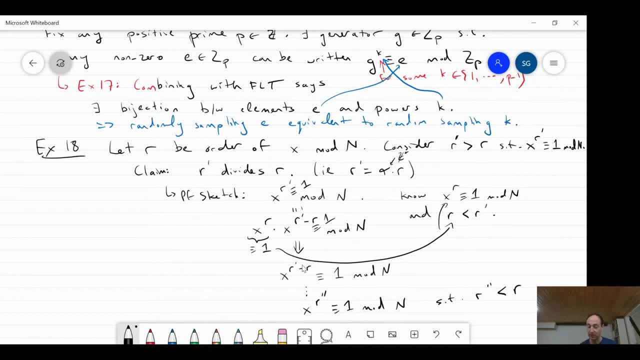 is right is equivalent to 1 mod n right is right is equivalent to 1 mod n right. because R was supposed to be the, because R was supposed to be the, because R was supposed to be the smallest choice of exponent. basically. smallest choice of exponent, basically. 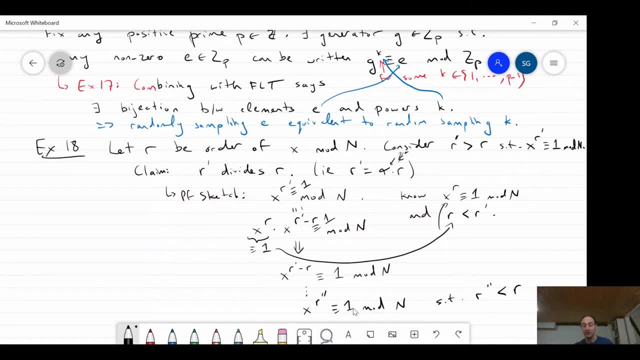 smallest choice of exponent. basically, which caused this quantity on the left? which caused this quantity on the left, which caused this quantity on the left to go to 1 right that causes X to go to to go to 1 right. that causes X to go to to go to 1 right that causes X to go to 1. so our prime cannot be both equivalent. 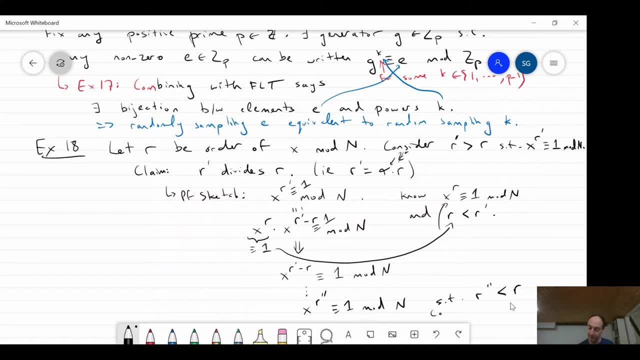 1, so our prime cannot be both equivalent 1, so our prime cannot be both equivalent to 1 and smaller than R. right, that's a to 1 and smaller than R. right that's a to 1 and smaller than R. right, that's a contradiction. so this is a contradiction. 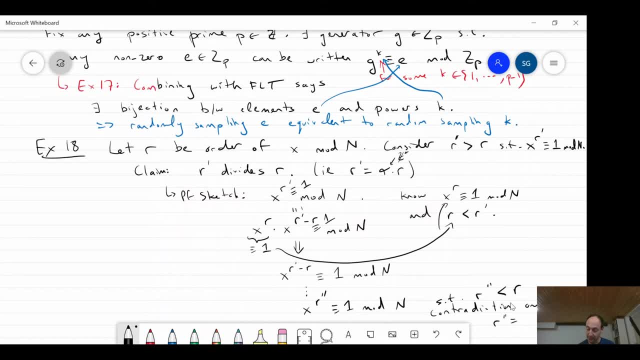 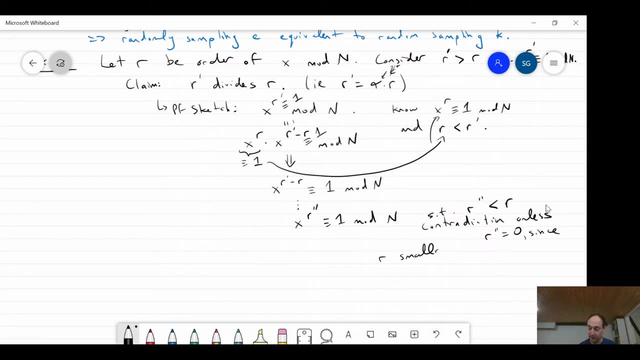 contradiction. so this is a contradiction, contradiction, contradiction. unless our double prime equals to 0, unless our double prime equals to 0, unless our double prime equals to 0, okay. and so, since R is the smallest, okay, and so since R is the smallest, okay, and so since R is the smallest, satisfying smallest integer, I should say: 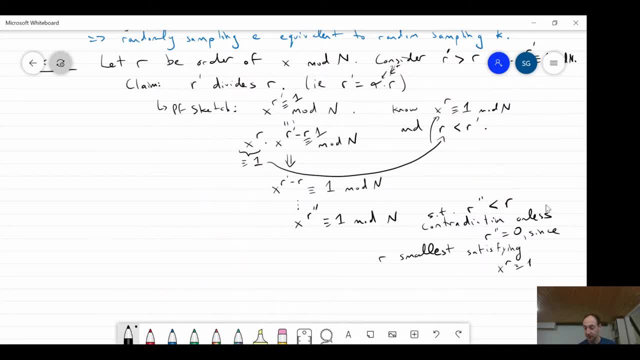 satisfying smallest integer. I should say: satisfying smallest integer, I should say: satisfying X to the R is equivalent to satisfying X to the R is equivalent to: satisfying X to the R is equivalent to 1 mod n. okay, so that's, it's gonna be 1 mod n. okay, so that's, it's gonna be. 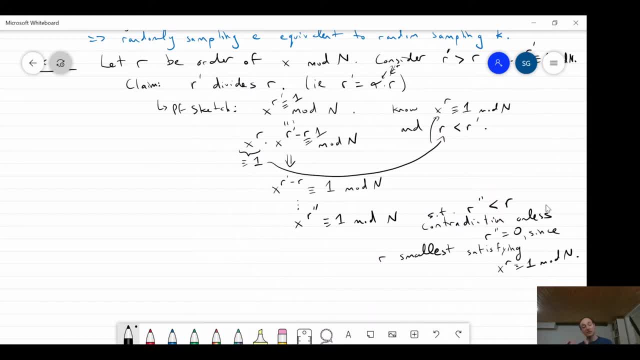 1, mod n. okay, so that's, it's gonna be useful to use this kind of proof idea. useful to use this kind of proof idea. useful to use this kind of proof idea that you know we can if I know something, that you know we can if I know something. 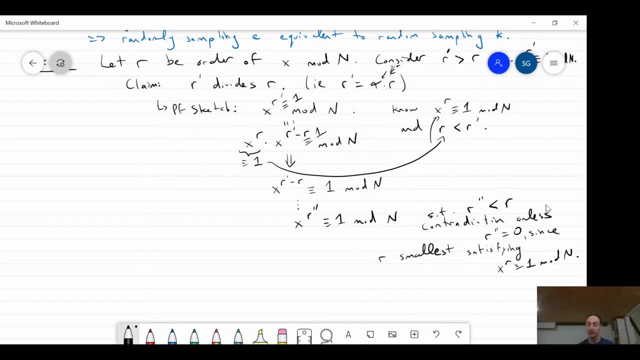 that you know we can, if I know something is equivalent to 1 mod n. I can kind of is equivalent to 1 mod n. I can kind of is equivalent to 1 mod n. I can kind of keep dividing out of the left side. okay, keep dividing out of the left side, okay. 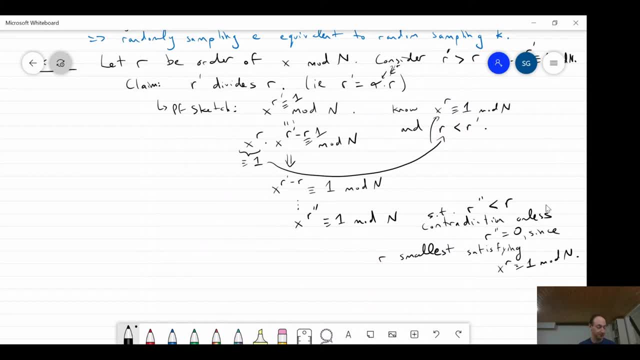 keep dividing out of the left side, okay, and this also gives us just some. and this also gives us just some, and this also gives us just some practice with playing with modular practice, with playing with modular practice, with playing with modular arithmetic. okay, so that's just all set. 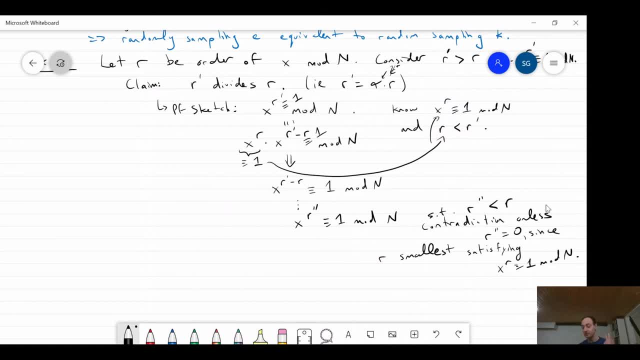 arithmetic: okay, so that's just all set. arithmetic: okay, so that's just all set up. we define Fermat's little theorem. we up, we define Fermat's little theorem. we up, we define Fermat's little theorem. we define the Chinese remaining theorem. we define the Chinese remaining theorem. we. 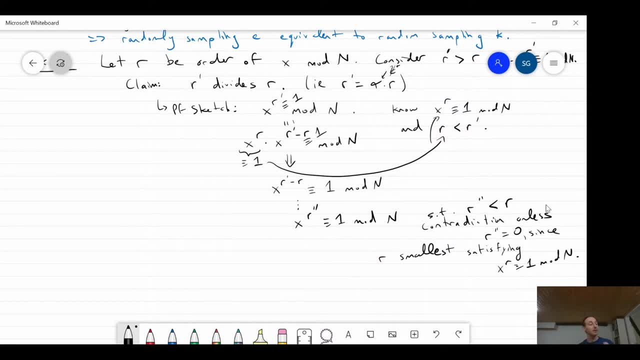 define the Chinese remaining theorem. we talked about the multiplicative- well. we talked about the multiplicative well. we talked about the multiplicative- well. we talked about that in Z P for P being talked about that in Z P for P being talked about that in Z P for P being prime. any element of the group can. 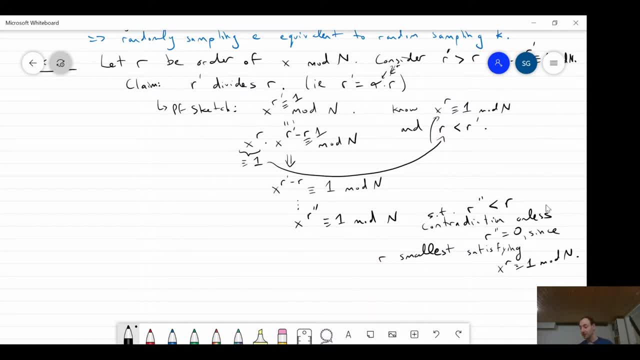 prime. any element of the group can prime. any element of the group can always be written, as you know. some always be written as you know, some always be written, as you know. some generator to some power- okay. and now generator to some power- okay. and now generator to some power- okay. and now we're gonna use all these to prove kind. 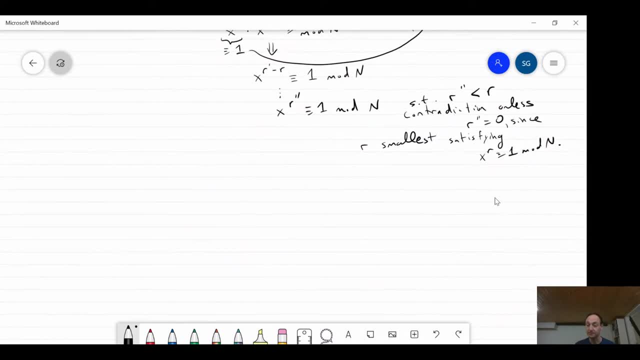 we're gonna use all these to prove kind. we're gonna use all these to prove kind of the main theorem of the section, which of the main theorem of the section, which of the main theorem of the section, which is the following: the main theorem of the is the following: the main theorem of the 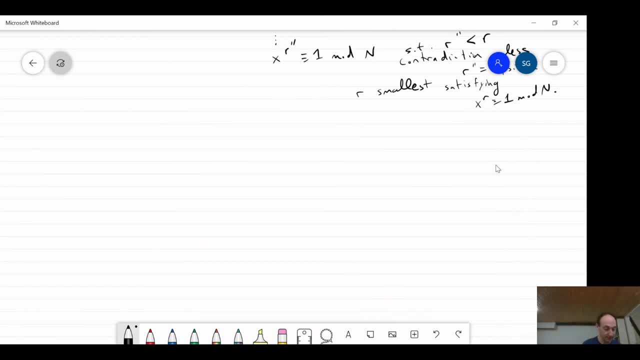 is the following: the main theorem of the section just keeping an eye on time here section- just keeping an eye on time here, section just keeping an eye on time here- is theorem 19. okay, so let me just write. is theorem 19. okay, so let me just write. 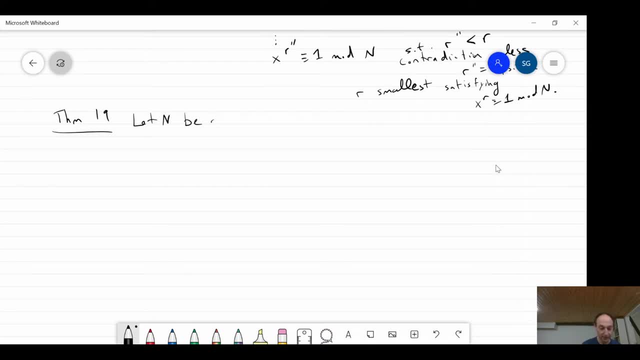 is theorem 19. okay, so let me just write out the theorem. so let n be an odd out the theorem. so let n be an odd out the theorem. so let n be an odd composite natural number, or positive composite natural number, or positive composite natural number or positive integer. okay, so obviously it's got to be 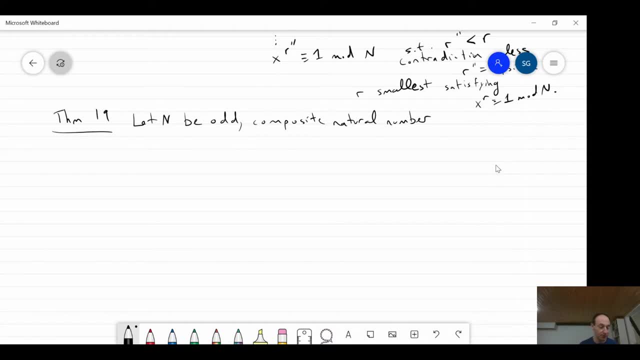 integer. okay, so obviously it's got to be integer. okay, so obviously it's got to be odd. because if it's even as trivial to odd, because, if it's even as trivial to odd, because if it's even as trivial to factor this thing, you just pull out the 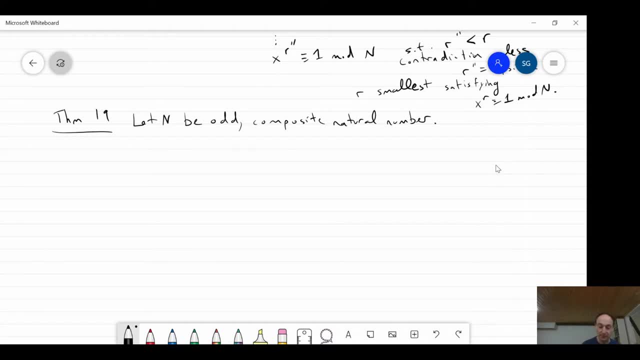 factor. this thing, you just pull out the factor. this thing, you just pull out the factor 2. okay, so let's define. now we've factor 2. okay, so let's define. now we've factor 2. okay, so let's define now. we've been talking about Z, n, which is all the. 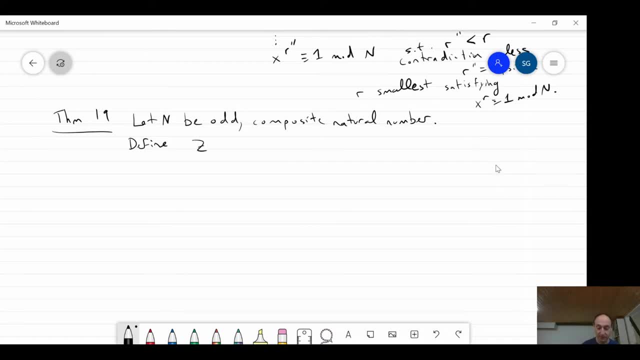 been talking about Z n, which is all the been talking about Z? n, which is all the numbers from 0 up to n minus 1. basically, numbers from 0 up to n minus 1. basically numbers from 0 up to n minus 1, basically. so let's define that n star, which is you. so let's define that n star which is you. so let's define that n star which is you. know a subset of that. so, instead of know a subset of that, so, instead of know a subset of that. so, instead of listing all the numbers, I'm just gonna. 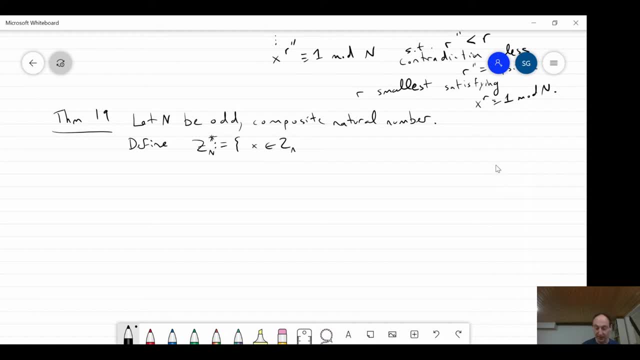 listing all the numbers. I'm just gonna listing all the numbers, I'm just gonna worry about the numbers. so all the worry about the numbers, so all the worry about the numbers. so all the numbers in Z n okay, such that X. numbers in Z n okay, such that X. 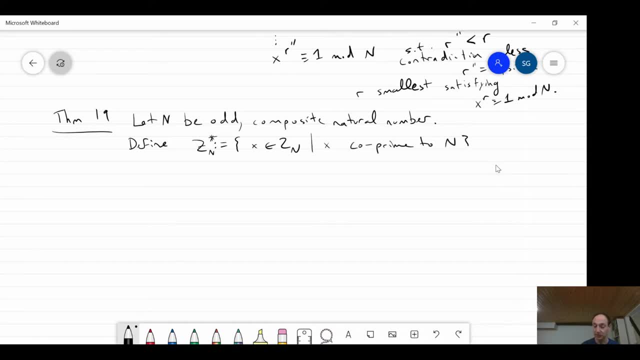 numbers in Z, n. okay, such that X additionally has to be co prime to n. okay, additionally has to be co prime to n. okay, additionally has to be co prime to n. okay, so you share no common factors of so you share no common factors of. so you share no common factors of that. so it's all the numbers between 0 and. 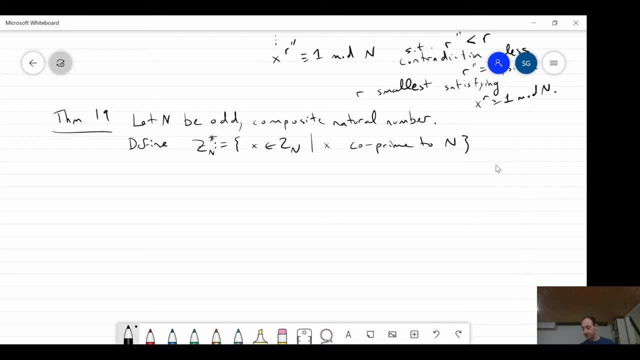 that, so it's all the numbers between 0 and that, so it's all the numbers between 0 and n minus 1, which share no common n minus 1, which share no common n minus 1, which share no common factors of that. okay, so in particular, you know. 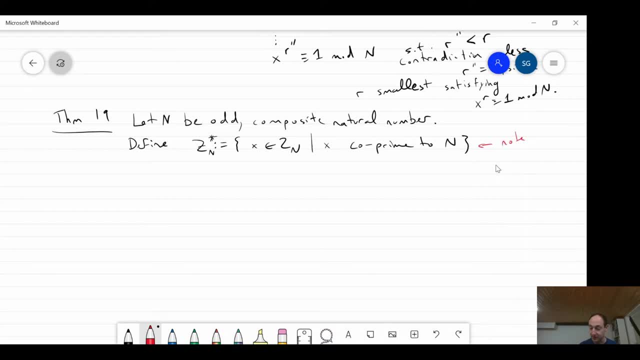 factors of that. okay, so in particular, you know factors of that. okay, so in particular, you know, think about this for a second. so think about this for a second, so think about this for a second. so note as a sanity check, you know is 0. note as a sanity check, you know is 0. 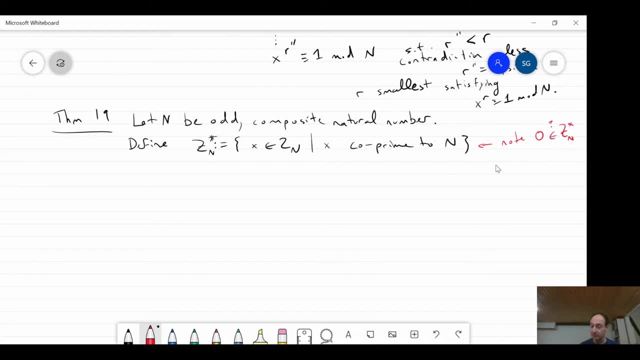 note as a sanity check. you know, is 0 question mark in Z n star? okay, it's question mark in Z n star. okay, it's question mark in Z n star. okay, it's certainly in Z n right. certainly in Z n right, certainly in Z n right. so why is it not in Z n star? well, clearly, 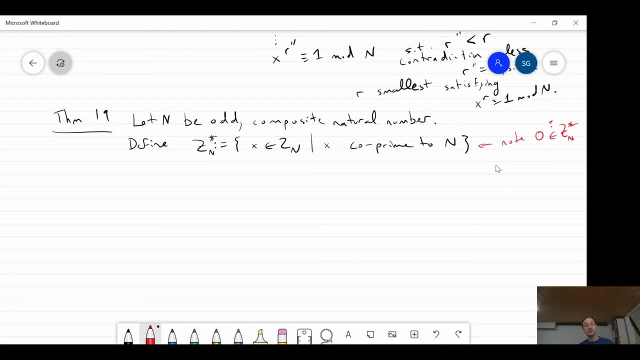 so why is it not in Z n star? well clearly. so why is it not in Z n star? well clearly: 0 is not co prime to n, because well n 0 is not co prime to n, because well n 0 is not co prime to n, because well n factors 0, right. so 0 divided by n is 0 I. 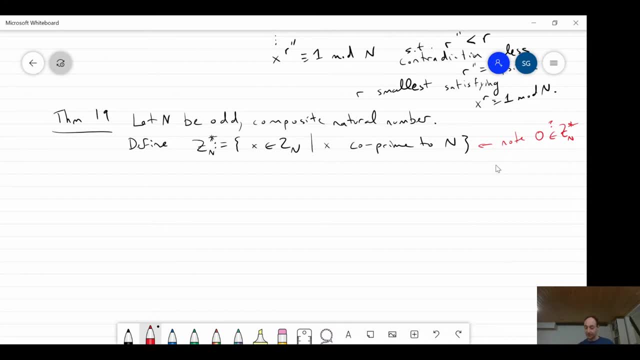 factors 0 right, so 0 divided by n is 0. I factors 0 right, so 0 divided by n is 0. I mean it goes through evenly in some mean it goes through evenly in some mean it goes through evenly in some sense. okay good, so let's keep going so. sense, okay, good, so let's keep going. so sense, okay, good, so let's keep going. so remember the goal was, and so why am I remember the goal was? and so why am I remember the goal was? and so why am I writing down this definition of Z? n? 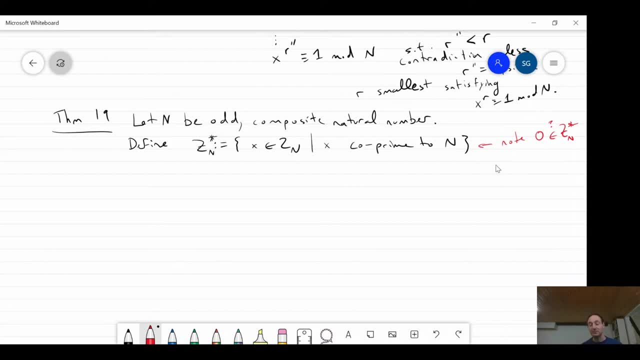 writing down this definition of Z n star. remember we said that to pick this star. remember we said that to pick this star. remember we said that to pick this magical X that allowed us to solve this magical X that allowed us to solve this magical X that allowed us to solve this equation. x squared is equivalent to 1. 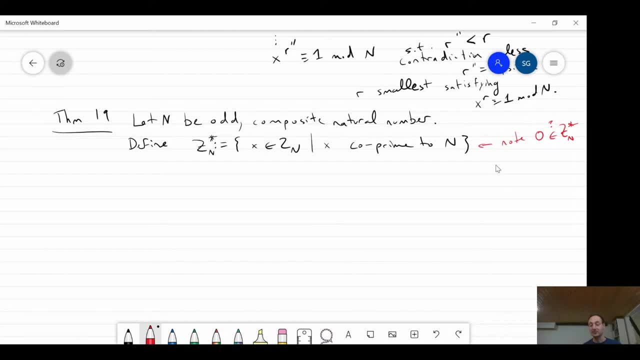 equation x squared is equivalent to 1. equation x squared is equivalent to 1. modern: the key was: we were just going to modern. the key was we were just going to modern. the key was we were just going to randomly sample all X in Z, n, which are: randomly sample all X in Z n which are randomly sample all X in Z n which are co prime 10. so in other words, we're just co prime 10. so, in other words, we're just co prime 10. so, in other words, we're just going to randomly sample from this set. 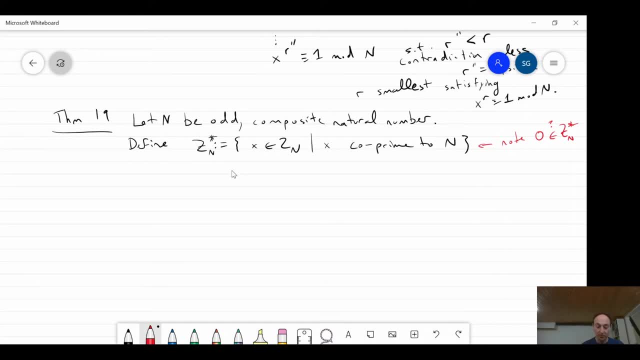 going to randomly sample from this set. going to randomly sample from this set. I'm just giving that set a name. okay, so I'm just giving that set a name. okay, so I'm just giving that set a name, okay. so, like we said before, you know, choose X in. 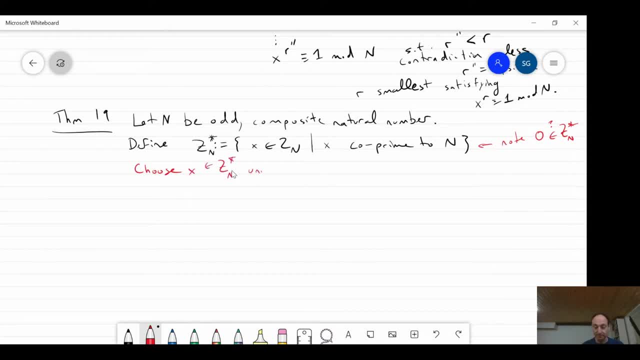 like we said before you know, choose X in. like we said before you know, choose X in Z and star uniformly at random- okay, Z. and star uniformly at random- okay, Z and star uniformly at random, okay. and then the claim is that with. and then the claim is that with. 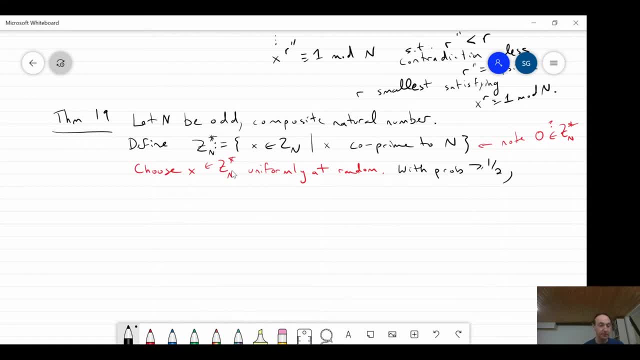 and then the claim is that with probability at least 1 half two things, probability at least 1 half two things, probability at least 1 half two things happen. number one: the order are, so let happen. number one: the order are, so let happen. number one: the order are so. let me write this in blue because it's 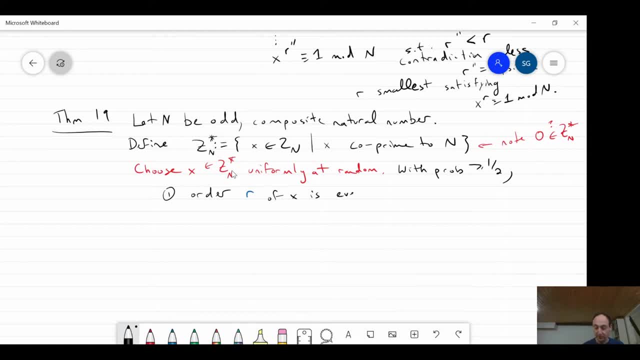 me write this in blue, because it's me write this in blue because it's a special parameter of X is even right. so a special parameter of X is even right. so a special parameter of X is even right. so that's the first thing we wanted, and that's the first thing we wanted. and that's the first thing we wanted. and why did we want the order to be even well? why did we want the order to be even well? why did we want the order to be even well? we wanted to be able to take R over. 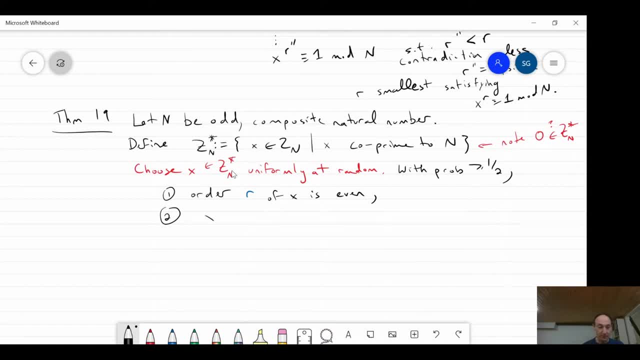 we wanted to be able to take R over. we wanted to be able to take R over 2 right and because remember that once I 2 right and because remember that once I 2 right and because remember that once I had X to the R is equivalent to 1 mod. 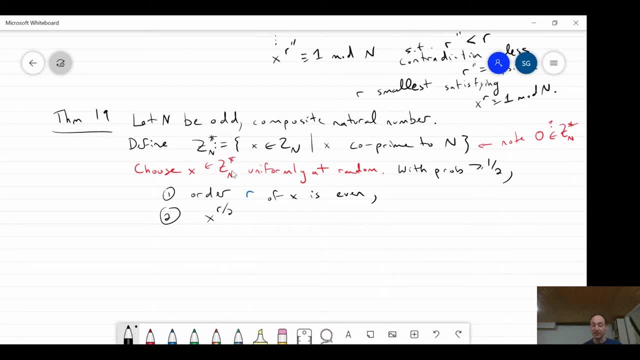 had X to the R is equivalent to 1 mod. had X to the R is equivalent to 1 mod n. then I took the square root, basically n. then I took the square root, basically n. then I took the square root, basically to find something that satisfies x. 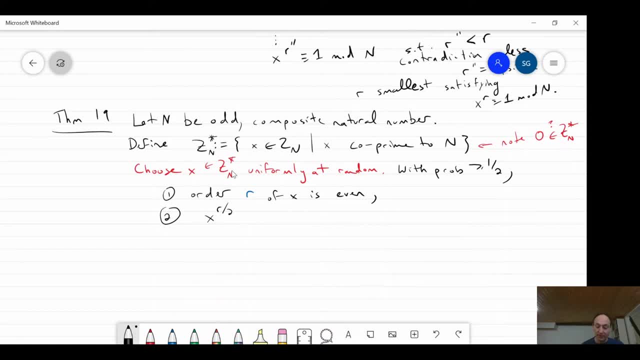 to find something that satisfies x. to find something that satisfies x. squared is equivalent to 1 y. squared is squared is equivalent to 1 y. squared is squared is equivalent to 1 y. squared is equivalent to 1 mod n. and so this thing equivalent to 1 mod n, and so this thing. 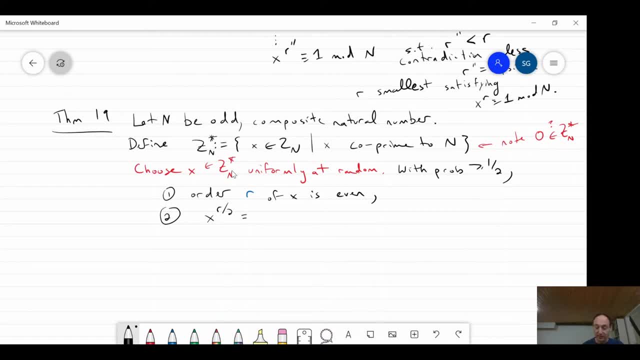 equivalent to 1 mod n. and so this thing here, which is now well defined since R, here, which is now well defined since R, here, which is now well defined since R is, even this thing is not a trivial is even this thing is not a trivial is even this thing is not a trivial solution to the to x squared is. 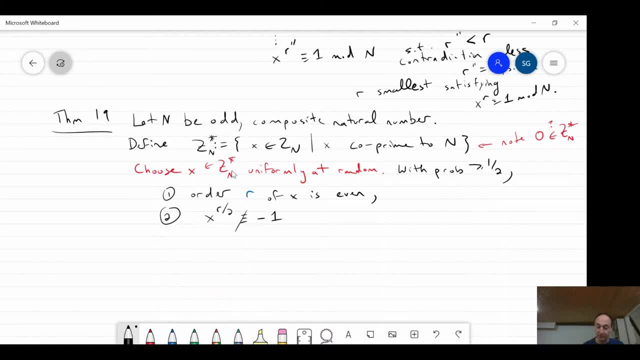 solution to the to x squared is solution to the: to x squared is equivalent to 1 mod n, meaning that it's equivalent to 1 mod n. meaning that it's equivalent to 1 mod n. meaning that it's not equivalent to minus 1 mod n. okay, so. 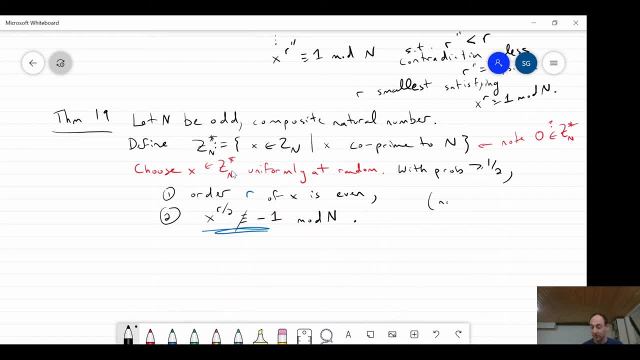 not equivalent to minus 1 mod n. okay. so, not equivalent to minus 1 mod n. okay. so this is the other main thing we wanted. this is the other main thing we wanted. this is the other main thing we wanted. so remember that we wanted a non-trivial. 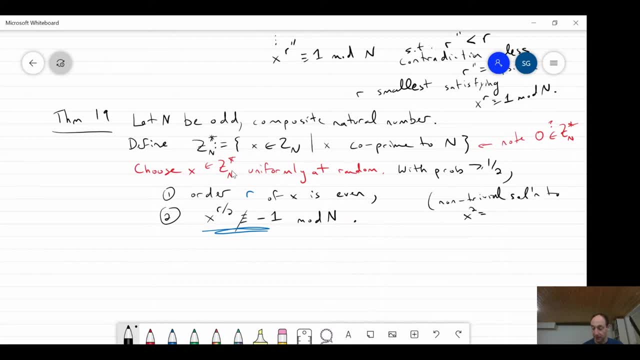 so remember that we wanted a non-trivial. so remember that we wanted a non-trivial solution to x. squared is equivalent to solution to x. squared is equivalent to solution to x. squared is equivalent to 1 mod n. okay, okay. so once we have this, 1 mod n. okay, okay. so once we have this, 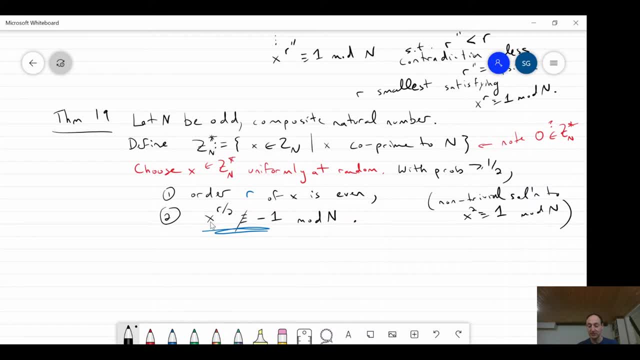 1 mod n: okay, okay. so once we have this right, once we can find such an X right, once we can find such an X right, once we can find such an X, basically remember from the previous, basically remember from the previous, basically remember from the previous exercise. that is a non-trivial solution. 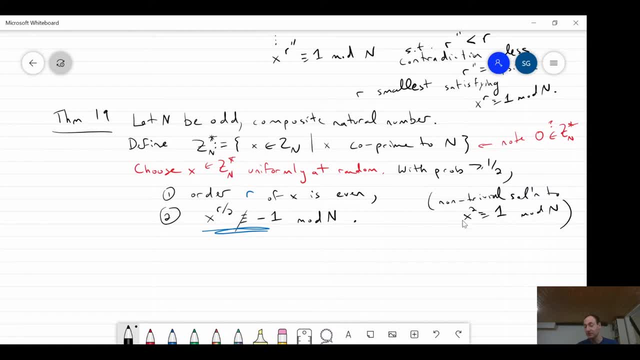 exercise that is a non-trivial solution. exercise that is a non-trivial solution. basically then remember we found a. basically. then remember we found a. basically then remember we found a solution to we. we said we can find a solution to we. we said we can find a. 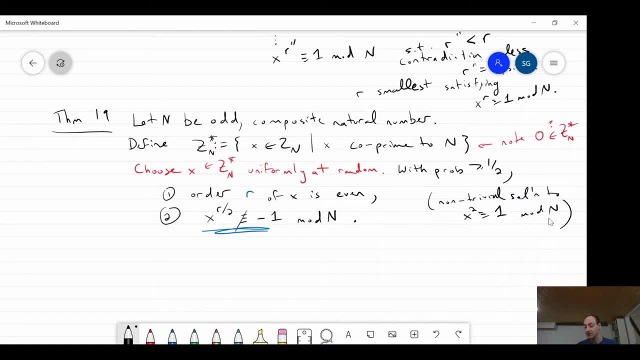 solution to we. we said: we can find a solution to this thing basically, and then solution to this thing basically, and then solution to this thing basically, and then this thing allowed us to compute. let this thing allowed us to compute, let this thing allowed us to compute. let me just go back and remind you of these. 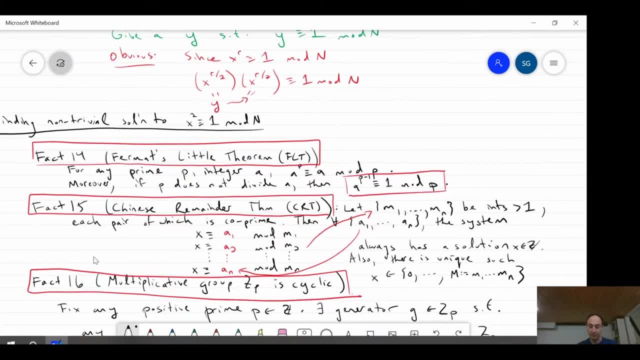 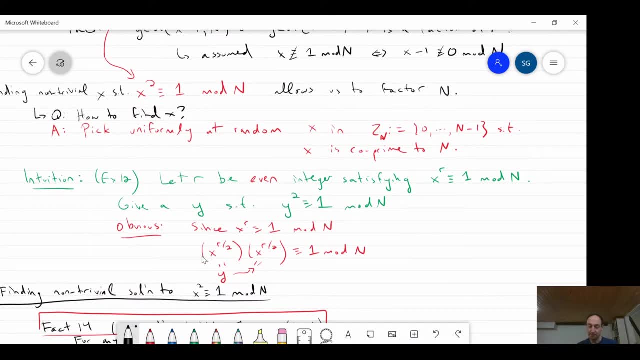 me just go back and remind you of these me just go back and remind you of these things right, right. so here we said that things right, right. so here we said that things right, right. so here we said that you know, if I can find something, an X. 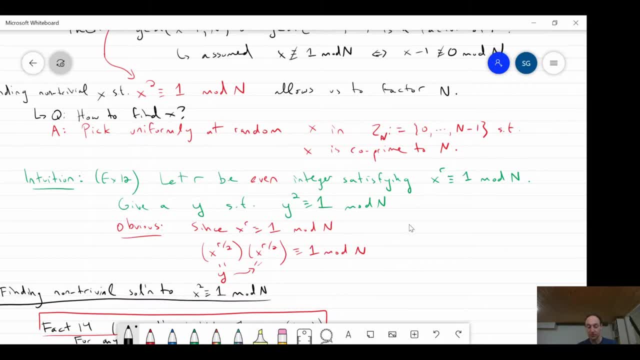 you know if I can find something an X, you know if I can find something an X with an even order. basically so that with an even order, basically so that with an even order. basically so that it's non-trivial, a non-trivial solution, it's non-trivial, a non-trivial solution. 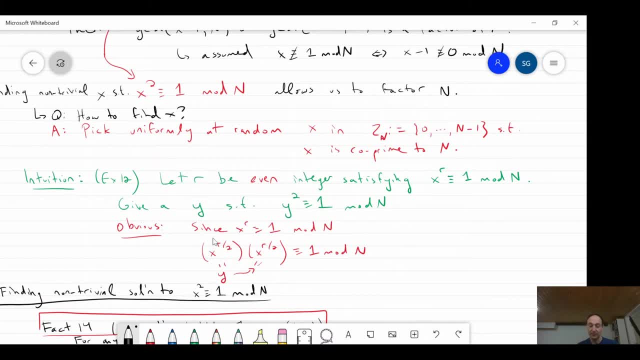 it's non-trivial, a non-trivial solution. it's right, such that when we divide this, it's right, such that, when we divide this, it's right, such that, when we divide this thing, this thing is not equivalent to thing, this thing is not equivalent to. 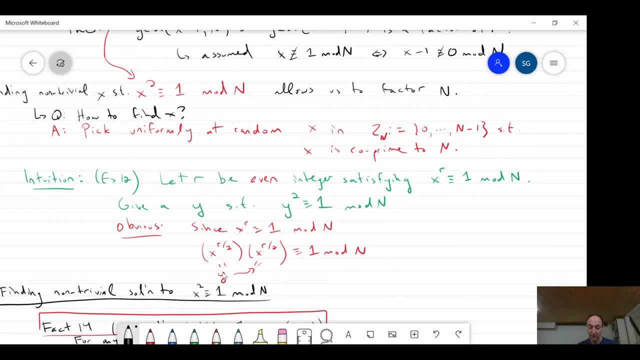 thing, this thing is not equivalent to plus or minus 1 mod n. then you know this: plus or minus 1 mod n. then you know this plus or minus 1 mod n. then you know this. thing with this Y here would indeed be. thing with this Y here would indeed be. 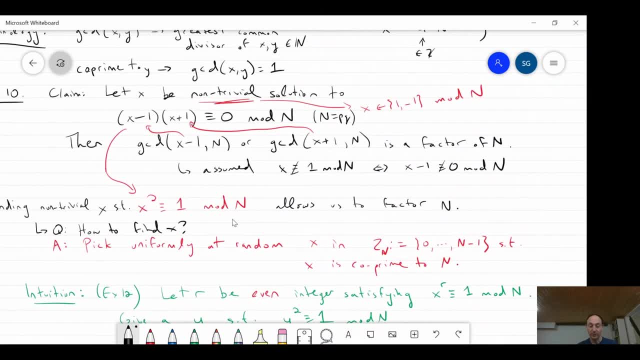 thing with this Y here would indeed be: a solution to x. squared is equivalent to a solution to x. squared is equivalent to a solution to x. squared is equivalent to 1 mod n, and once we had that, then 1 mod n, and once we had that, then 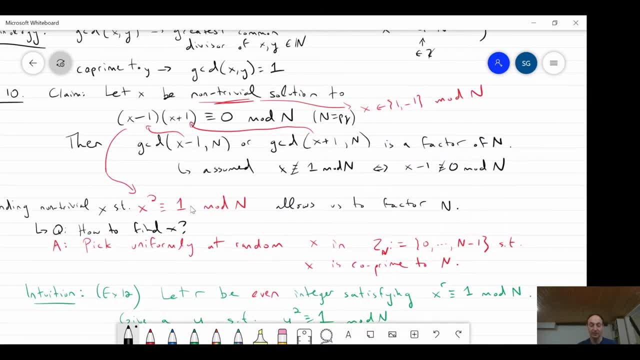 1 mod n, and once we had that, then remember that we said that, well, you know. remember that we said that, well, you know. remember that we said that. well, you know, you could factor this thing out this, you could factor this thing out this, you could factor this thing out, this expression like this, and we argued that. 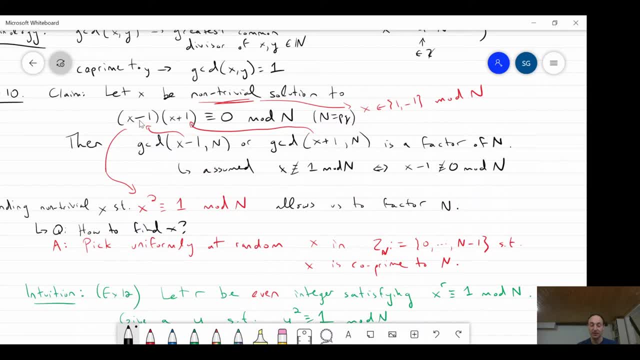 expression like this and we argued that expression like this and we argued that, therefore, and the factors of n would therefore, and the factors of n would therefore, and the factors of n would have to split up, some of which would have to split up, some of which would. 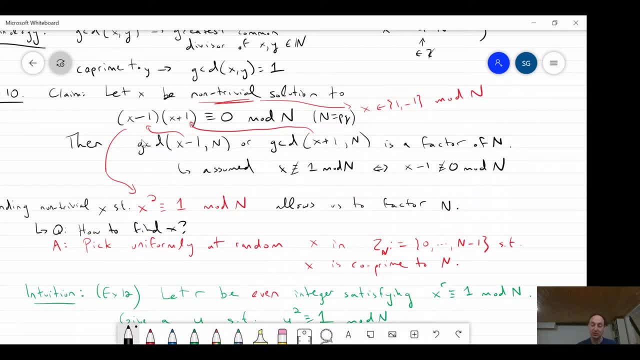 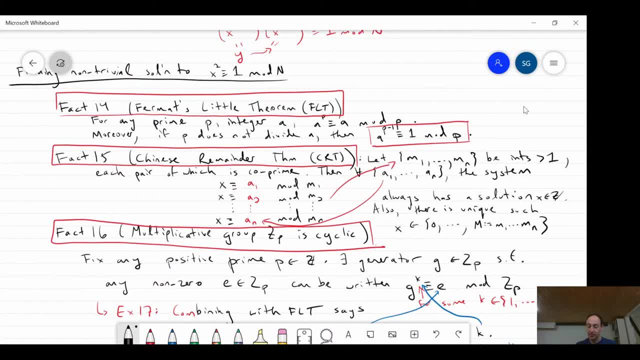 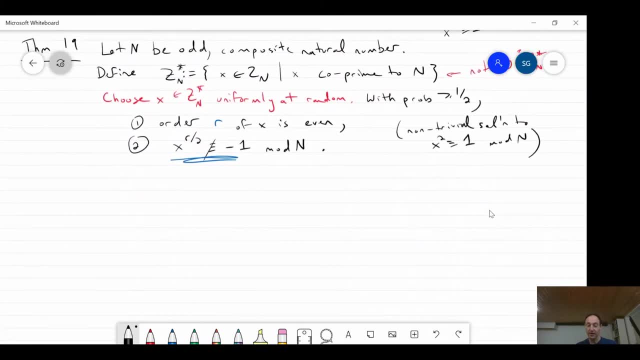 was the kind of the sequence of how we got, was the kind of the sequence of how we got here: okay, okay, so this is the claim here. okay, okay, so this is the claim here. okay, okay, so this is the claim. and this is why the claim allows us to. 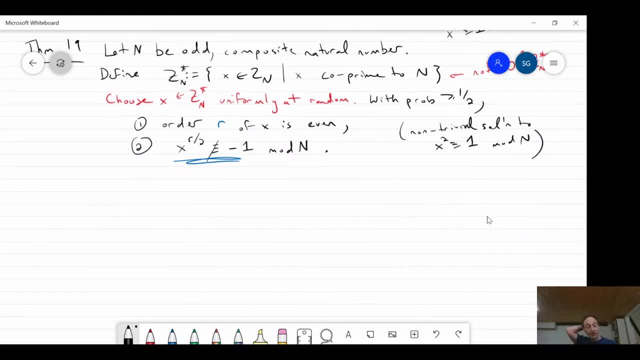 and this is why the claim allows us to, and this is why the claim allows us to prove or allows us to basically factor prove, or allows us to basically factor prove or allows us to basically factor. if we can prove that this random. if we can prove that this random. 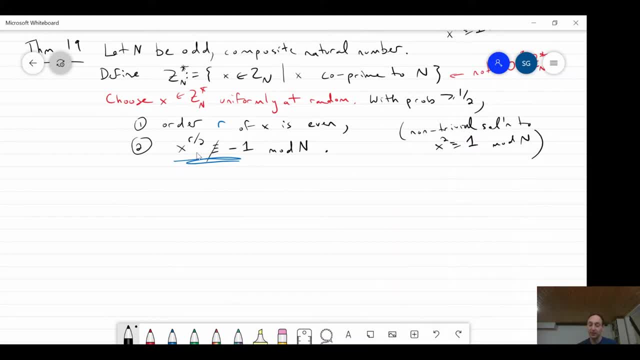 if we can prove that this random sampling works. and let me just be very clear: we sampling works. and let me just be very clear, we sampling works. and let me just be very clear: we also had said a trivial solution would. also had said a trivial solution would. 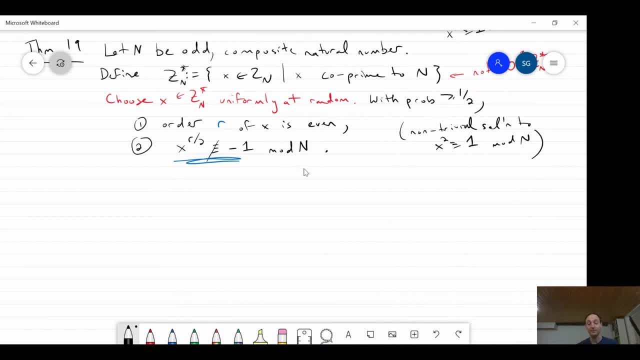 also had said. a trivial solution would also be when X to the R over 2 is also be when X to the R over 2 is also be when X to the R over 2 is equivalent to 1 mod n. so why? and that's? 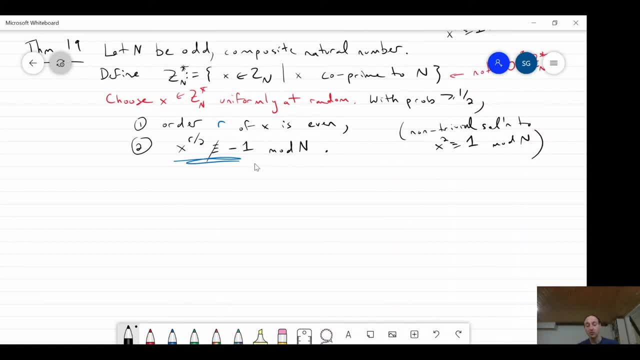 equivalent to 1 mod n, so why? and that's equivalent to 1 mod n, so why? and that's exercise part of exercise 20, so why have exercise part of exercise 20? so why have exercise part of exercise 20? so why have I not explicitly stated that we're going? I not explicitly stated that we're going. I not explicitly stated that we're going to exclude the case with high. to exclude the case with high. to exclude the case with high. probability that X to the R over 2 is. probability that X to the R over 2 is. 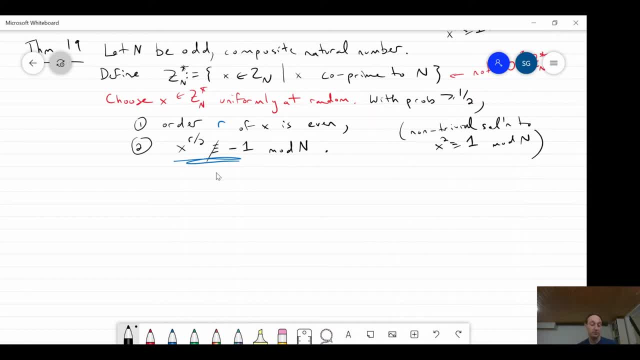 probability that X to the R over 2 is equivalent to 1 mod n. okay, why? well, equivalent to 1 mod n, okay. why well, equivalent to 1 mod n. okay, why, well, right, so so in that sense, that is just a right. so so, in that sense, that is just a. 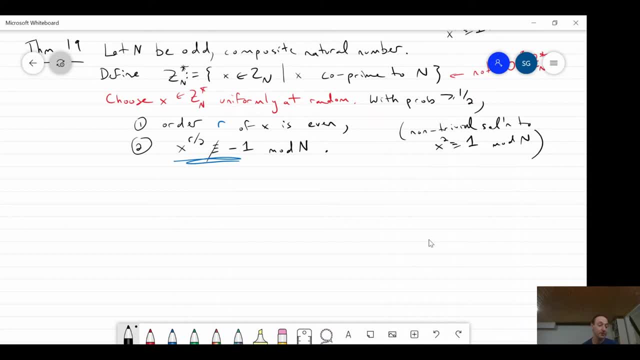 right, so so in that sense, that is just a redundant. you don't need to state it redundant, you don't need to state it redundant, you don't need to state it explicitly. okay, so let's prove it, and so explicitly okay, so let's prove it, and so. explicitly okay. so let's prove it. and so in the proof I'm gonna use a number of. in the proof I'm gonna use a number of. in the proof I'm gonna use a number of kind of facts which are exercises in the kind of facts which are exercises in the 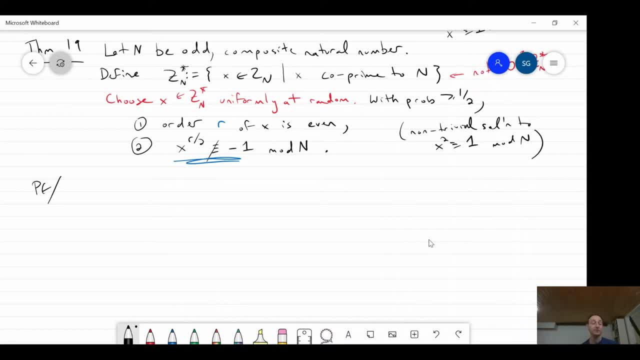 kind of facts which are exercises in the notes. you know, in the interest of time notes. you know, in the interest of time notes. you know, in the interest of time, I'm not gonna go through all of the. I'm not gonna go through all of the. I'm not gonna go through all of the, the proofs of these things I might sketch. 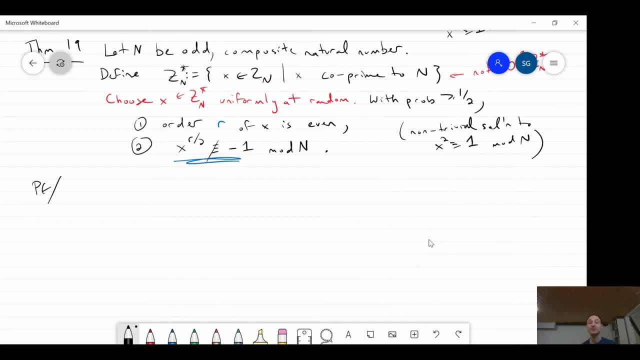 the proofs of these things. I might sketch the proofs of these things. I might sketch some of them basically okay, but some of them basically okay, but some of them basically okay. but again, I encourage you to kind of work through. again, I encourage you to kind of work through. 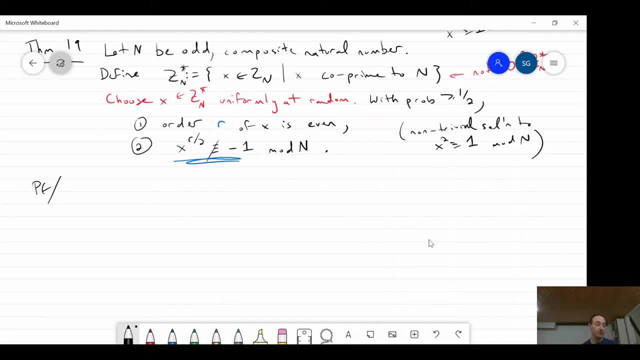 again, I encourage you to kind of work through this section on your own, okay. so this section on your own, okay. so this section on your own, okay. so what we're gonna do, so I'm not gonna prove. what we're gonna do, so I'm not gonna prove. 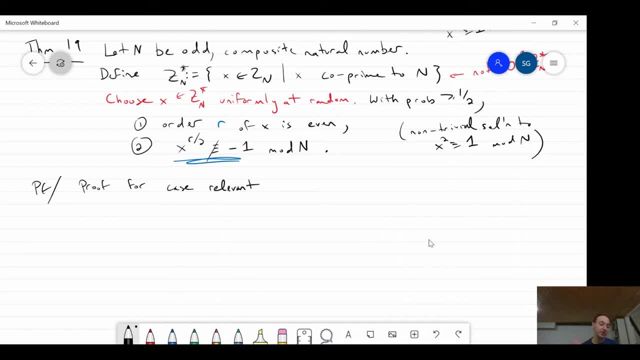 what we're gonna do. so I'm not gonna prove it in all generality, because the it in all generality, because the it in all generality, because the notation can get a bit cumbersome and in notation can get a bit cumbersome and in notation can get a bit cumbersome and, in particular, our goal is to break RSA in. 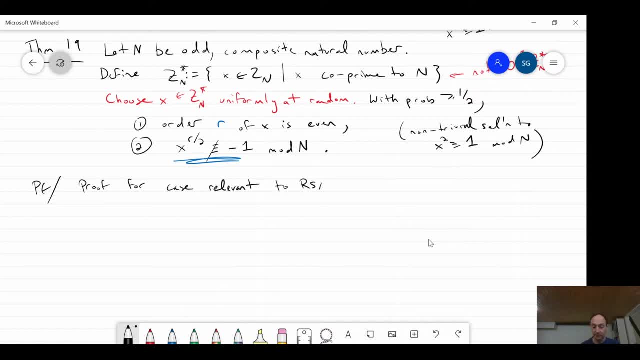 particular, our goal is to break RSA. in particular, our goal is to break RSA in some sense, so which we again will cover some sense, so which we again will cover some sense, so which we again will cover at the end of this lecture, section 4 of at the end of this lecture, section 4 of. 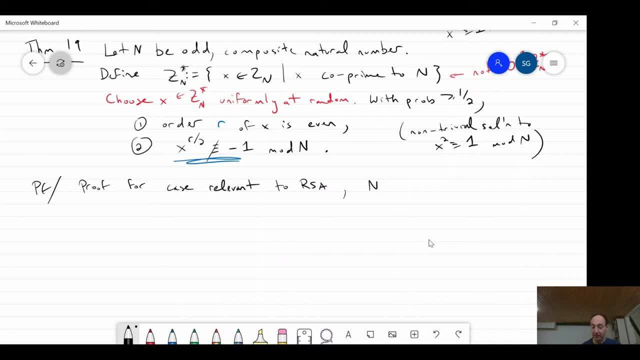 at the end of this lecture, section 4 of the notes, and so the case relevant to the notes, and so the case relevant to the notes, and so the case relevant to RSA is when n is the product of distinct. RSA is when n is the product of distinct. 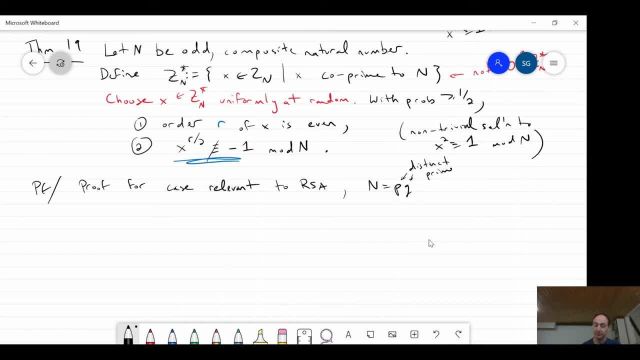 RSA is when n is the product of distinct primes P and Q. okay, because RSA starts primes P and Q. okay, because RSA starts primes P and Q. okay, because RSA starts by picking two primes- P and Q- and by picking two primes P and Q, and by picking two primes P and Q, and multiplies them to get n, okay, okay and multiplies them to get n? okay, okay. and multiplies them to get n okay, okay. and once you have it for two primes that you, once you have it for two primes that you, once you have it for two primes that you know, you can certainly generalize it to: 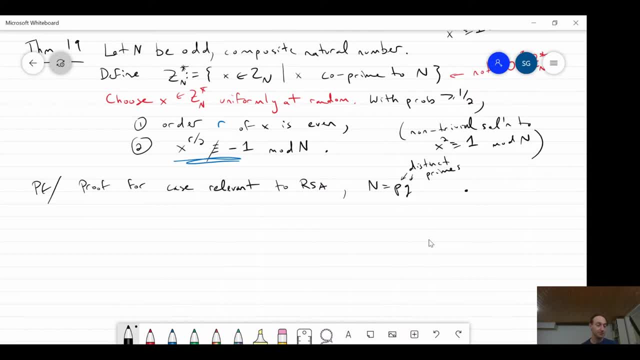 know you can certainly generalize it to know you can certainly generalize it to more than two primes with a bit more more than two primes with a bit more, more than two primes with a bit more work, but let's not go there. okay, so what work? but let's not go there. okay, so what? 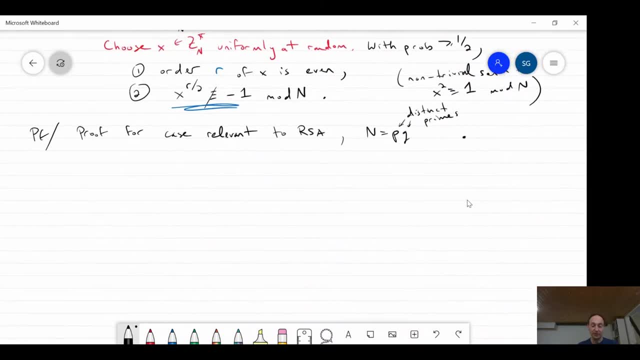 work, but let's not go there, okay? so what do we know about n? okay, at least in. do we know about n? okay, at least in. do we know about n? okay, at least in theory. right, sorry, let me try and keep theory, right, sorry, let me try and keep. 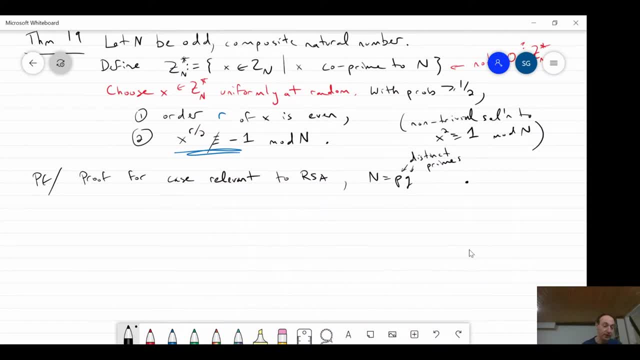 theory. right, sorry, let me try and keep this theorem here for now. okay, so we this theorem here for now. okay, so we this theorem here for now. okay, so we know. the only thing we know about n is know. the only thing we know about n is know. the only thing we know about n is, of course, our prime factor is P and Q at. 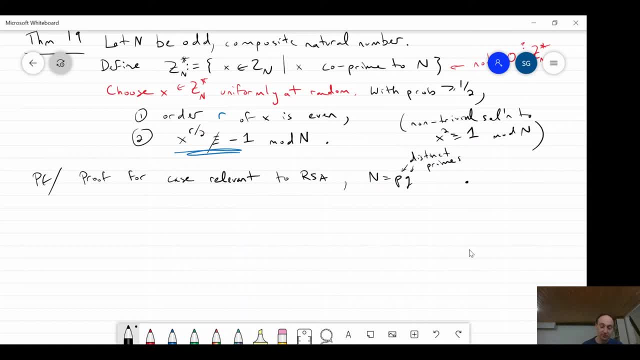 of course our prime factor is P and Q at of course our prime factor is P and Q, at least as far as the proof is concerned, least as far as the proof is concerned, least as far as the proof is concerned. right, and so step one, basically, in our 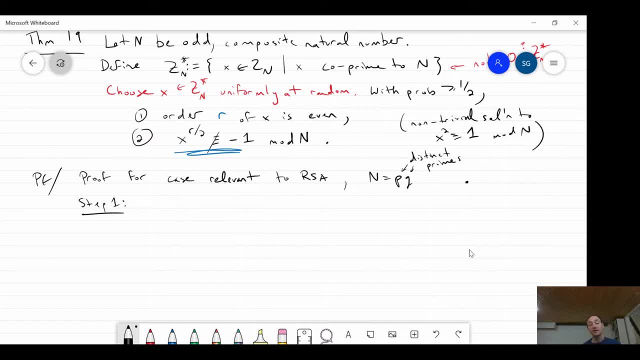 right, and so step one basically in our right, and so step one basically in our proof is: what we're saying is that you proof is. what we're saying is that you proof is what we're saying is that you know we're talking about picking a. know, we're talking about picking a. 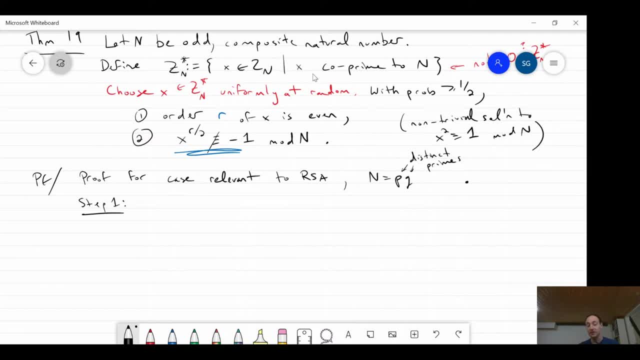 know we're talking about picking a random X. you know mod n basically such random X. you know mod n basically such random X. you know mod n basically such that X is co-prime to n- okay, so now. but that X is co-prime to n- okay, so now. but 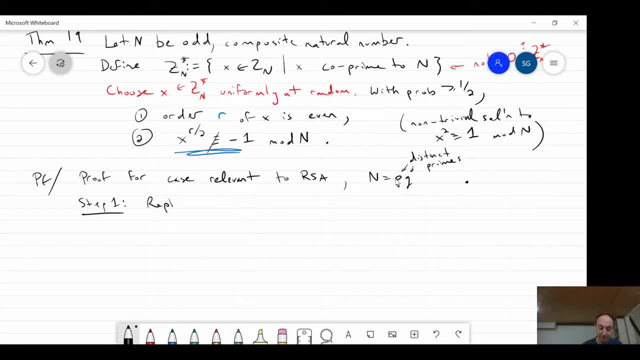 that X is co-prime to n. okay, so now. but I want to kind of rephrase this idea of. I want to kind of rephrase this idea of. I want to kind of rephrase this idea of rephrase random X in Z, n star or so. 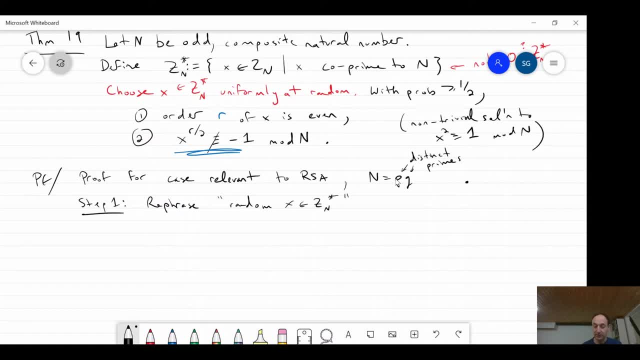 rephrase random X in Z n star or so. rephrase random X in Z n star, or so: co-prime, basically to n in terms of co-prime, basically to n in terms of co-prime, basically to n in terms of sorry, sorry, sorry, I should say in terms of the so-called 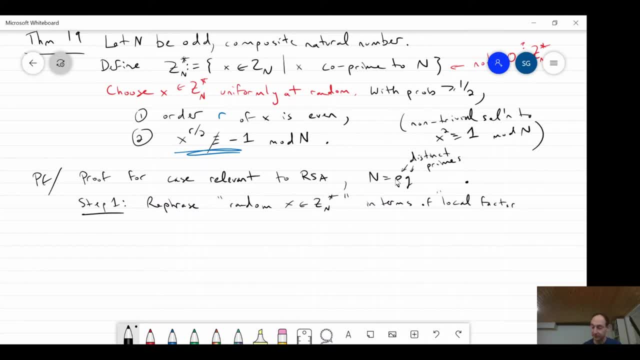 I should say in terms of the so-called- I should say in terms of the so-called local factors, which is just a name. I'm local factors, which is just a name. I'm local factors, which is just a name I'm making up, by the way, okay, so in other, 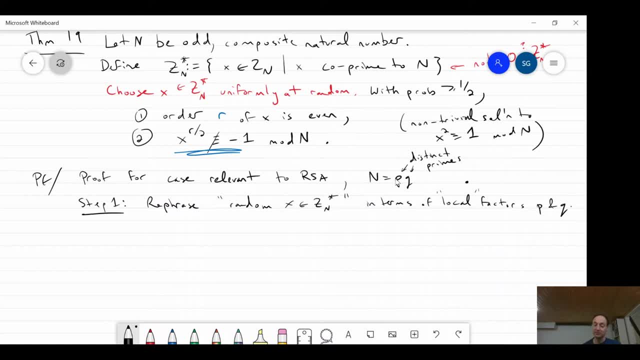 making up by the way, okay. so in other, making up by the way, okay. so in other words, I want to kind of be able to words. I want to kind of be able to words, I want to kind of be able to understand. what does it mean to if I? 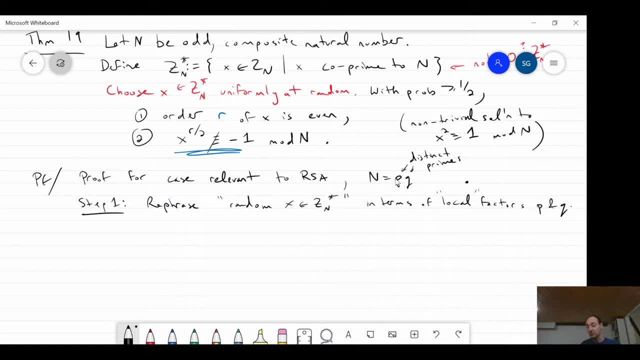 understand. what does it mean to? if I understand, what does it mean to? if I randomly sample X which is co-prime to randomly sample X, which is co-prime to randomly sample X which is co-prime to n, what does that mean in terms of the n. what does that mean in terms of the n? what does that mean in terms of the factors P and Q? what am I randomly factors P and Q? what am I randomly factors P and Q? what am I randomly sampling on that kind of more local, sampling on that kind of more local? 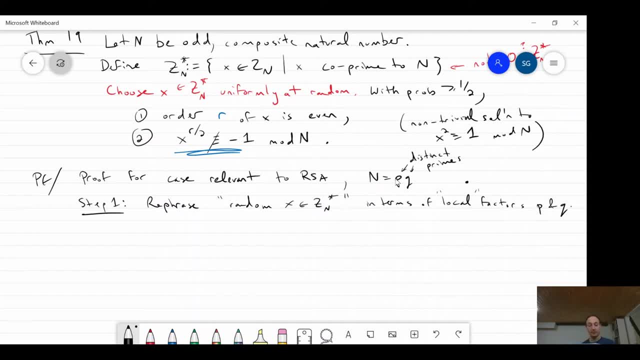 sampling on that kind of more local level. okay, so this is one exercise in level. okay, so this is one exercise in level. okay, so this is one exercise in which I'll briefly sketch. this is which I'll briefly sketch. this is which I'll briefly sketch. this is exercise 22, and the claim is that 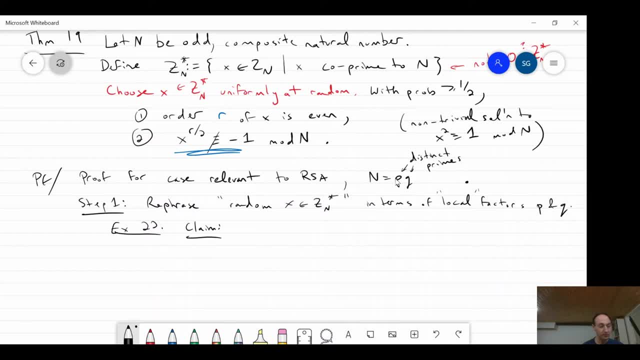 exercise 22 and the claim is that exercise 22 and the claim is that choosing X in Z and star uniformly at choosing X in Z and star uniformly at choosing X in Z and star uniformly at random is equivalent. random is equivalent. random is equivalent to to. 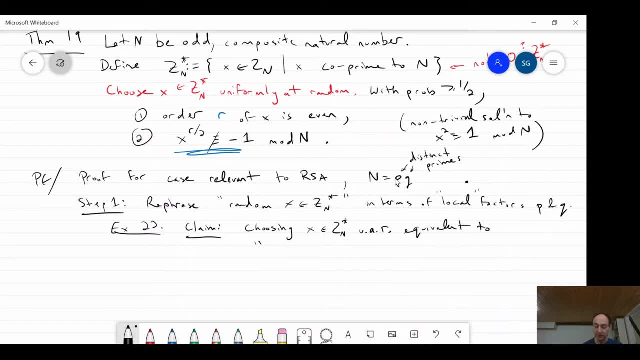 to choosing a pair of integers. let me give choosing a pair of integers. let me give choosing a pair of integers. let me give it up just a bit more space. a pair of it up, just a bit more space. a pair of it up, just a bit more space. a pair of integers in a set that depends on P and. 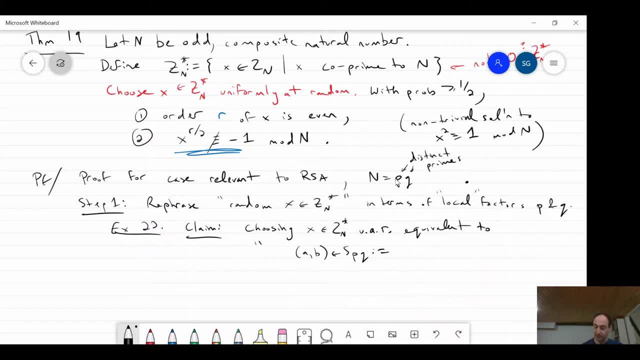 integers in a set that depends on P and integers in a set that depends on P and Q, which I'm going to define now. so this Q which I'm going to define now, so this Q which I'm going to define now, so this is a set of all integers, a comma, B, such 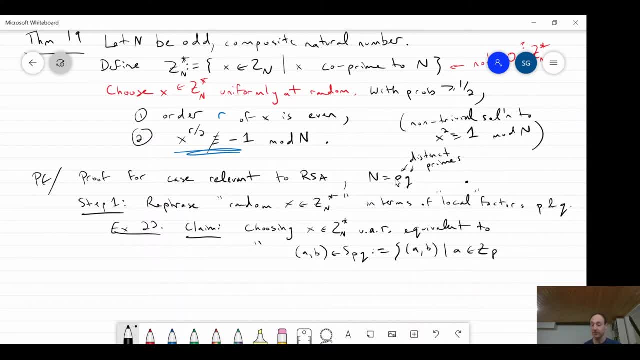 is a set of all integers a comma B. such is a set of all integers a comma B, such that a is some number between 0 and P, that a is some number between 0 and P, that a is some number between 0 and P minus 1 for P, a prime remember. 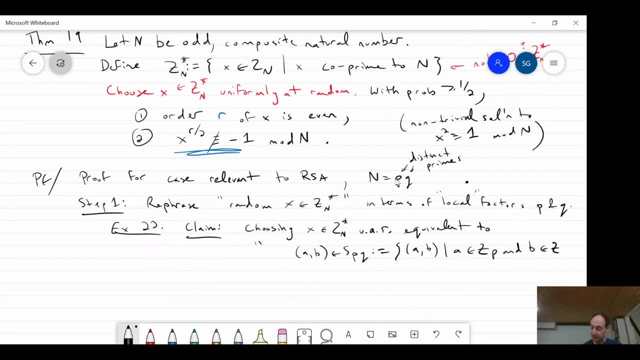 minus 1 for P a prime remember. minus 1 for P a prime remember. and B is in Z Q. okay, so this is the and B is in Z Q. okay, so this is the and B is in Z Q. okay. so this is the claim that you know, instead of sampling. 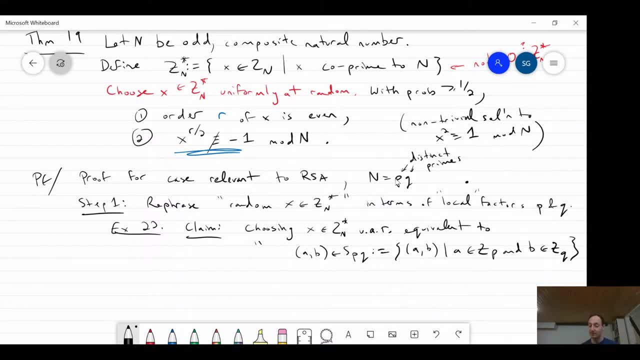 claim that you know, instead of sampling. claim that you know, instead of sampling: X. uniformity at random from Z and star. X. uniformity at random from Z and star. X. uniformity at random from Z and star. I can, equivalently, instead just pick some. I can, equivalently, instead just pick some. 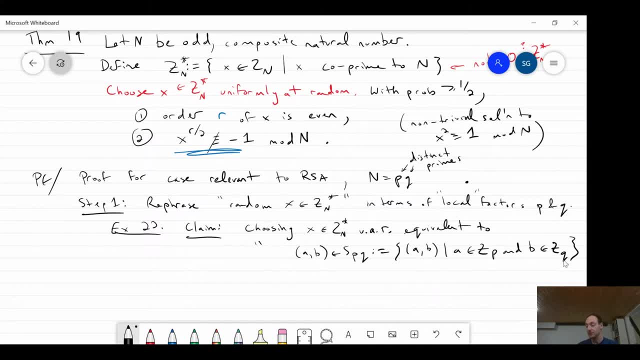 I can equivalently instead just pick some a between 0 and P minus 1 and some B a between 0 and P minus 1, and some B a between 0 and P minus 1 and some B between 0 and Q minus 1, P and Q being. 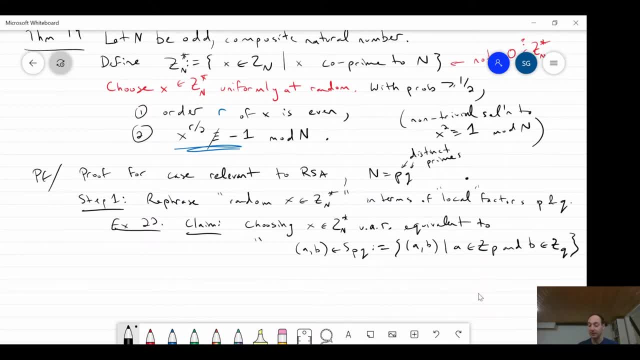 between 0 and Q minus 1 P, and Q being between 0 and Q minus 1 P, and Q being Prime's okay, and those are the factors: Prime's okay, and those are the factors Prime's okay, and those are the factors that remember right, n equals PQ, so 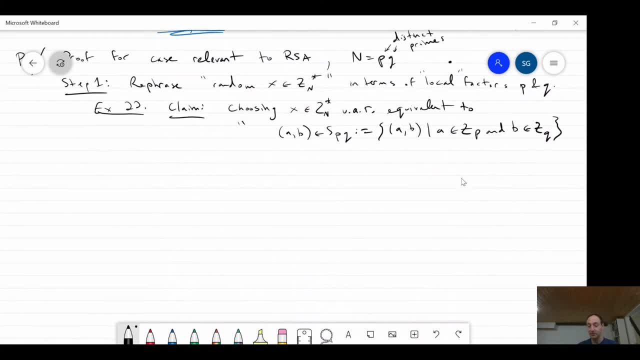 that remember right n equals PQ. so that remember right n equals PQ. so that's the claim and this local view is that's the claim, and this local view is that's the claim, and this local view is gonna help a lot. and so why is this true? 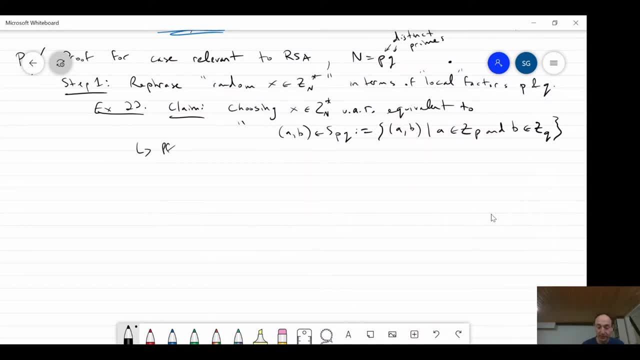 gonna help a lot, and so why is this true? gonna help a lot, and so why is this true? well, you know, this is just due to proof. well, you know, this is just due to proof. well, you know, this is just due to proof sketch. okay, the proof sketch is just. 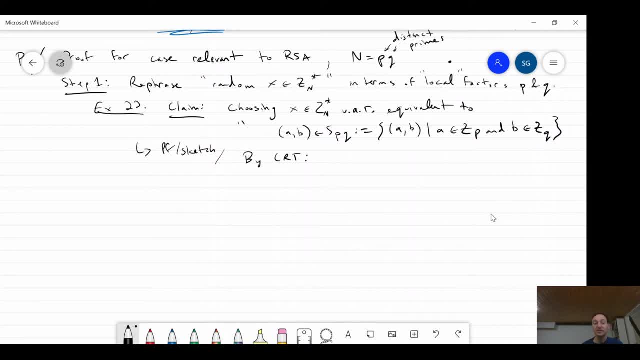 sketch. okay, the proof sketch is just sketch. okay, the proof sketch is just: basically by the Chinese remainder, basically by the Chinese remainder, basically by the Chinese remainder. theorem right which said that you know I. theorem right which said that you know I. theorem right which said that you know I can always write X. you know, pick your. 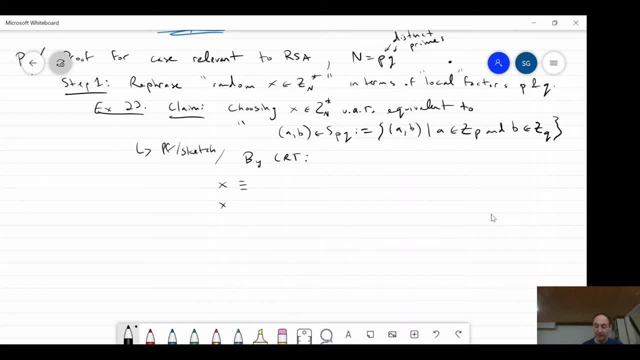 can always write X. you know pick. your can always write X, you know pick your favorite X right when I take X and I do favorite X, right when I take X. and I do favorite X right when I take X and I do mod P and I do mod Q, right, obviously. 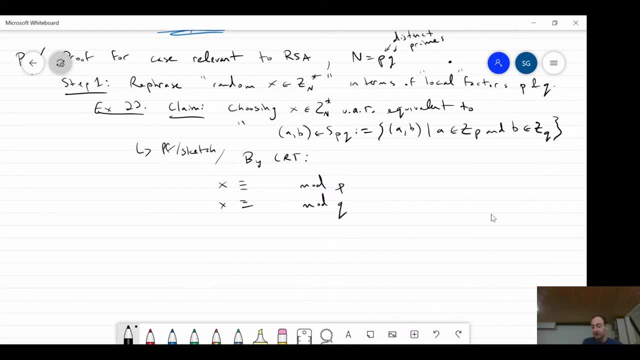 mod P and I do mod Q, right, obviously, mod P and I do mod Q, right, obviously, first of all, that's gonna give me first of all, that's gonna give me first of all, that's gonna give me something right. so if I fix X and I fix, 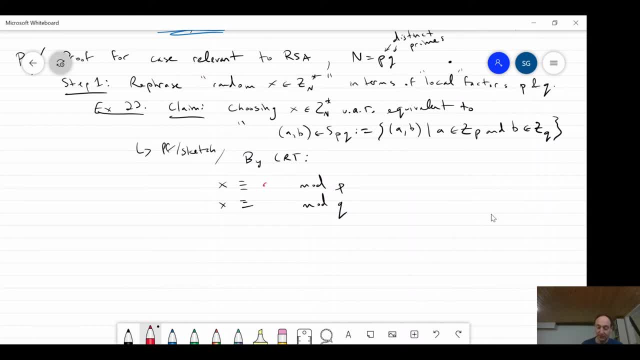 something right. so if I fix X and I fix something right, so if I fix X and I fix P, then obviously there's some remainder P, then obviously there's some remainder P, then obviously there's some remainder here. whatever that is right, so let's here. whatever that is right, so let's. here, whatever that is right. so let's call that a and let's call it B mod Q. call that a and let's call it B mod Q. call that a and let's call it B mod Q. right, so that's going in the forward. right, so that's going in the forward. 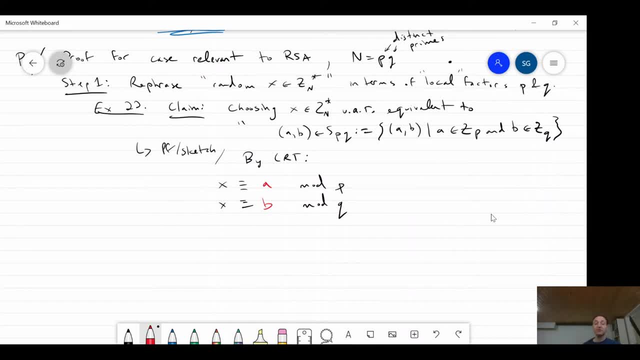 right, so that's going in the forward direction. and the Chinese remainder direction and the Chinese remainder direction and the Chinese remainder theorem told us that the the reverse theorem told us that the the reverse theorem told us that the the reverse direction was also true. right, if you? 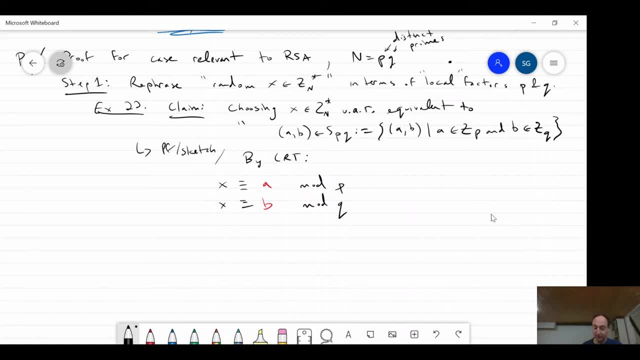 direction was also true. right, if you direction was also true, right, if you instead now think of so here, think of instead now think of so here, think of instead now think of so here, think of. you know, here, you know, we fix a P and Q. you know, here, you know, we fix a P and Q. 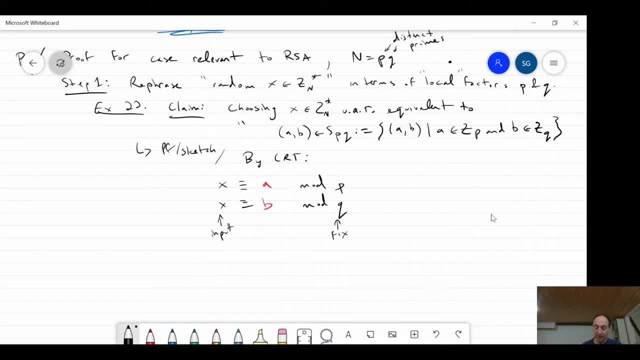 you know, here you know, we fix a P and Q, right, and now you input X and kind of right. and now you input X and kind of right. and now you input X and kind of. this is your output, right? that will X. this is your output, right? that will X. 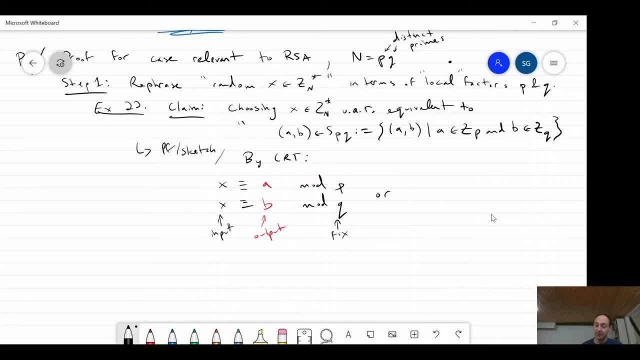 this is your output, right. that will. X. will define some a and B uniquely. will define some a and B uniquely. will define some a and B uniquely, obviously right, and now we can view this obviously right, and now we can view this obviously right, and now we can view this in the opposite direction. to write you. 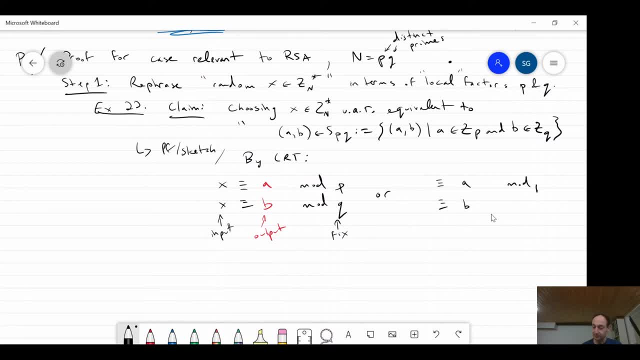 in the opposite direction to write you in the opposite direction to write. you can make it so that now we fix as input: so now these are fixed right, and and now. so now these are fixed right, and and now. so now these are fixed right, and and now. instead, if I fix a and B, the Chinese, 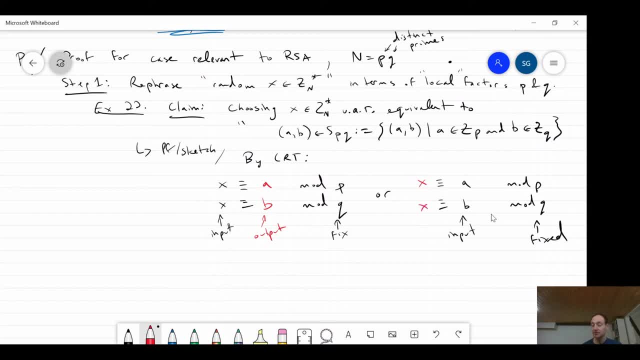 instead. if I fix a and B, the Chinese. instead. if I fix a and B, the Chinese, remainder theorem tells me that there's remainder theorem tells me that there's always some output x that gives me a and b when i do mod p and q. okay, and so this is by the chinese. 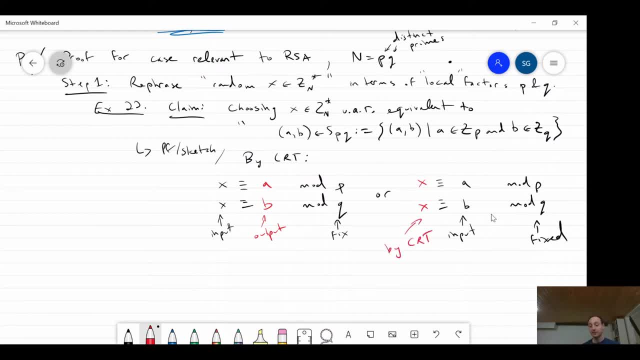 remainder theorem. okay, in fact x is unique right, at least between zero and p times q. okay, so in other words, we have a bijection between you know, all this set, basically z and star, and this set over here spq. so sampling x uniformly random from this set is completely equivalent to picking a. 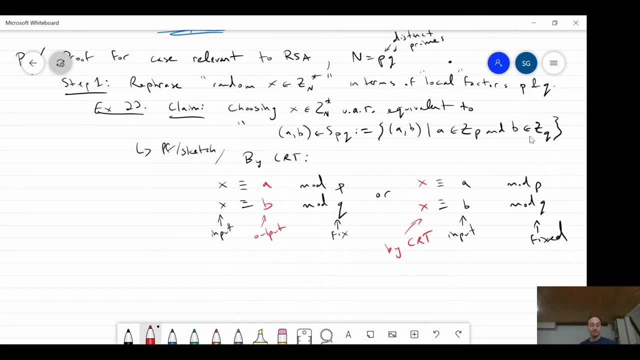 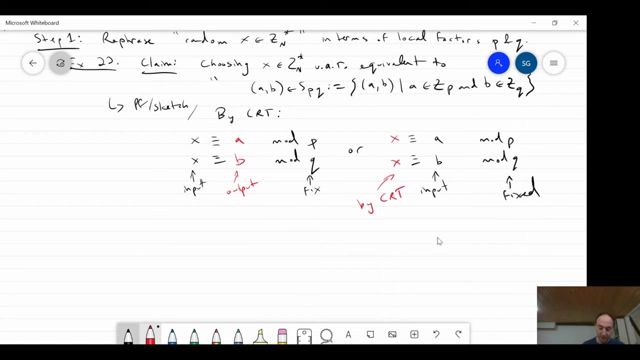 comma b from this set same thing. okay, good, so what have we learned? we've learned that, therefore, we can equivalently sample a comma b, uniformly, at random, of course, from this set spq. okay, and so now that we have this? so now we want to do two things. 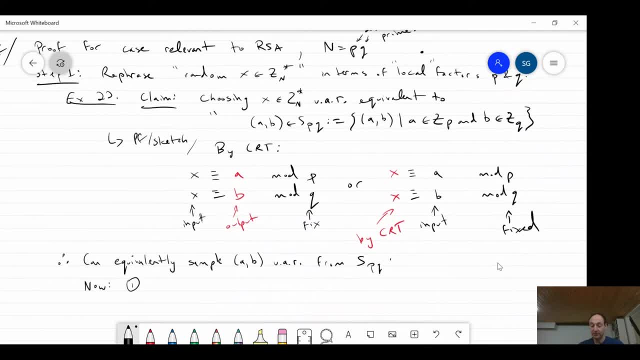 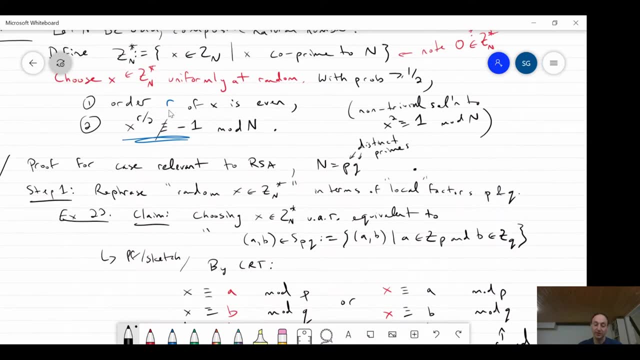 okay, remember that. let's just go back to what we have to prove right. so all i did right now is i just rephrased um what it meant to pick uniformly random x in terms of local factors. and i need two things right. i need to bound, you know, when i pick x uniformly at random. 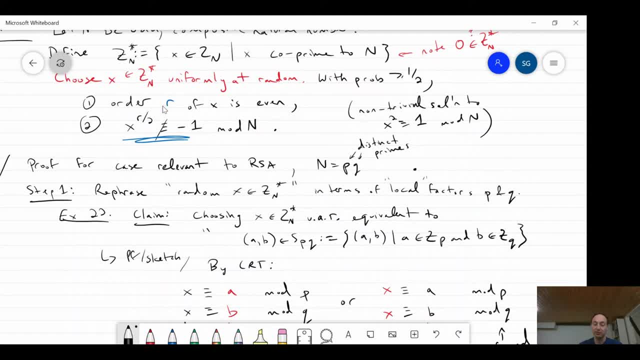 equivalently, i pick those local factors a, b. what is the probability that the order r is even number one and number two? what is the probability that x to the r over two, assuming r is even so? this is well defined that this thing is not equivalent to minus. 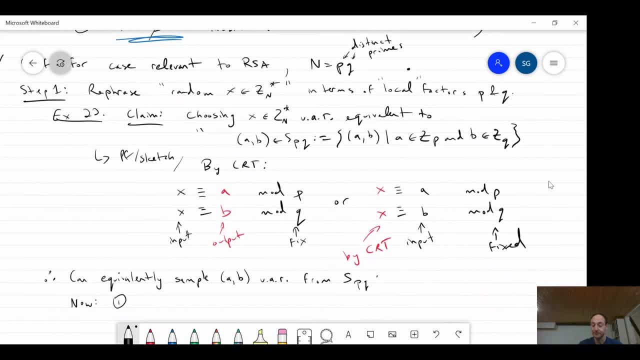 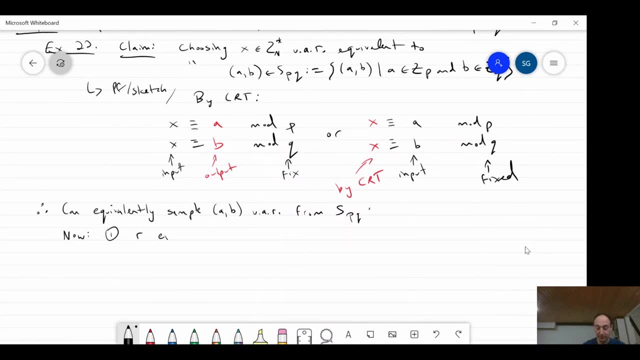 1 mod n. that it's a good solution. it's not a trivial solution, okay. so what i want to know is: um, what is the probability of r is being even and number two, what is the probability that x to the r over two is not in um? well, okay, technically i write minus one plus one. 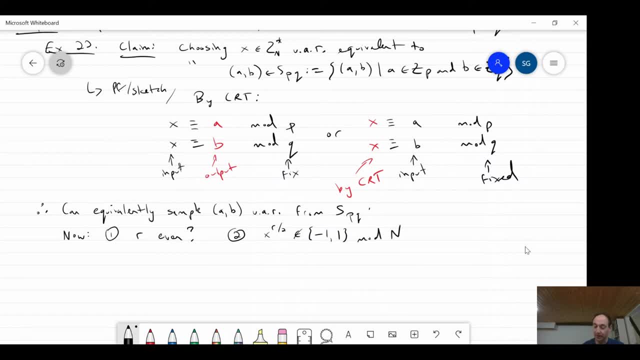 But remember the plus one case is not possible because x to the r is the order by assumption. So we need to bound the probabilities of both of these happening and the claim was that jointly these things will not happen with probability at least a half, I think we said. 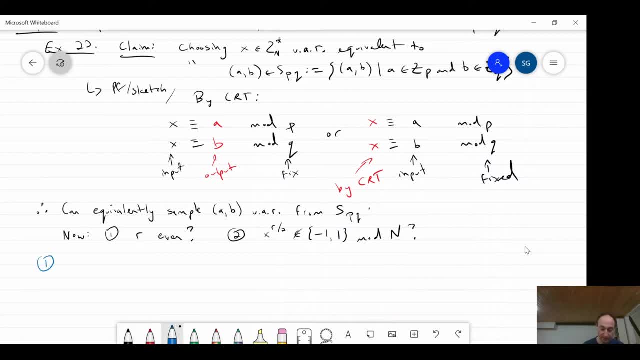 So let's first prove one. What is the probability that r is even Okay? so what do we know? Let's use green, Let's recall the facts that we have at our disposal. Well, I'm telling you already that we're assuming that any x I choose has some order, right? 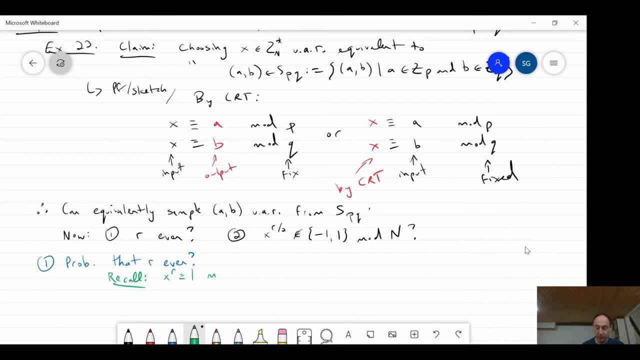 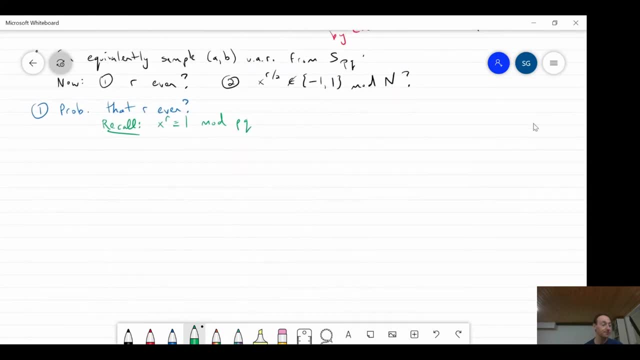 So there's some order r, basically, so that this thing is one mod pq, which, remember, is just equal to n. okay, And the other things I know by this Chinese remainder trick that we talked about is that x is equivalent to some a mod p and x is equivalent to some b mod q, right? 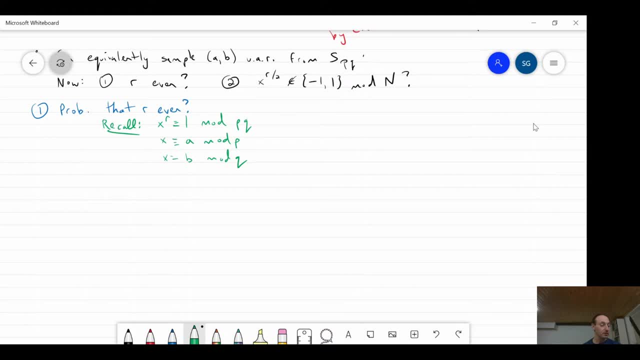 So these are the three things I know, And here what I'm going to do is I'm going to define r and r respectively, so that these are the kind of the local orders. So x to the r is equivalent to one mod p times q, but mod p it could be the order could. 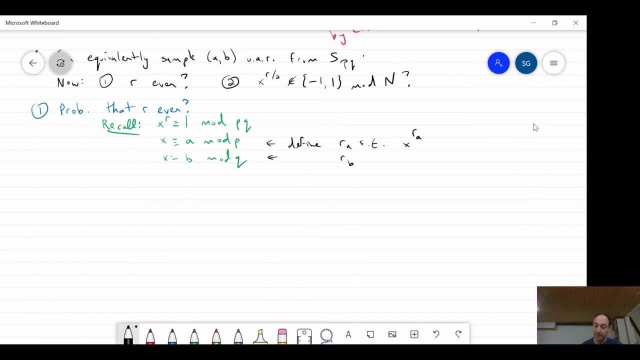 be different, right? So x to the r a mod. sorry, okay, so what's the order of a, basically, or b Mod q? Okay, so let's define the local orders basically. And of course, you know, because x is equivalent to a mod p, you know, this is completely equivalent. 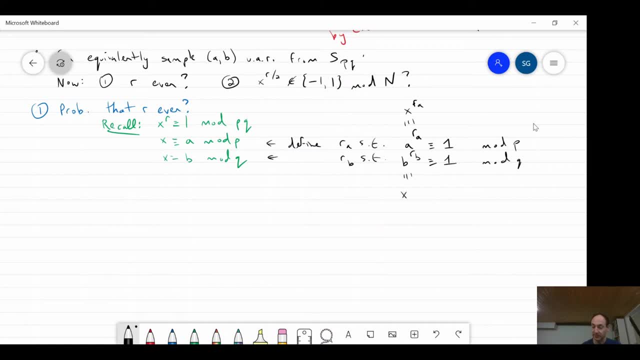 to x to the r a right, And this is completely equivalent to x to the r b right. Just simply because you know, we have these equivalences right- Mod p and q- So you might as well replace a with x mod p, not mod q, okay. 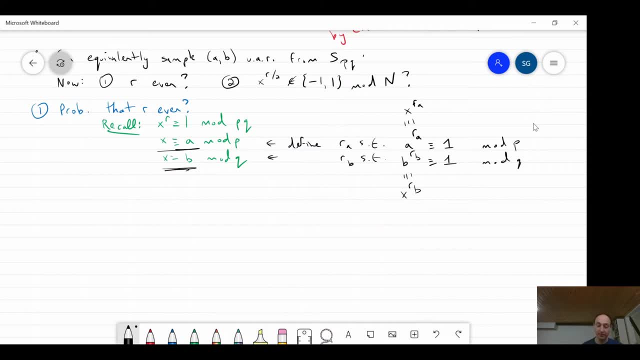 So these are kind of the basic things we could right away get. And now exercise 23,, which I'll let you prove on your own, because it should be similar to the previous exercise that we did that had to do with dividing orders. So what you can prove is that both r a and r b right- which are, you know, these local 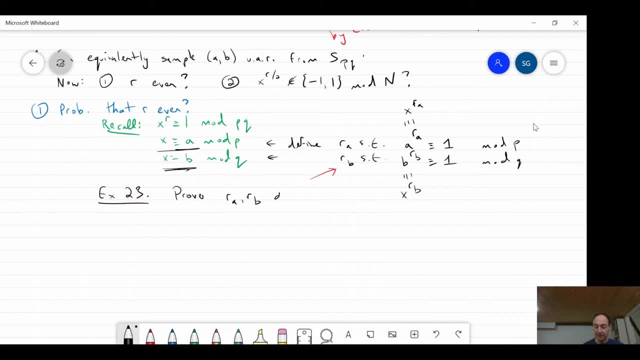 orders over here. basically, these guys must divide the global order r. Okay, so r was you know this order right here? Okay, so the global order mod pq. Okay Okay. so what does this mean? You know these local orders. they divide r right. 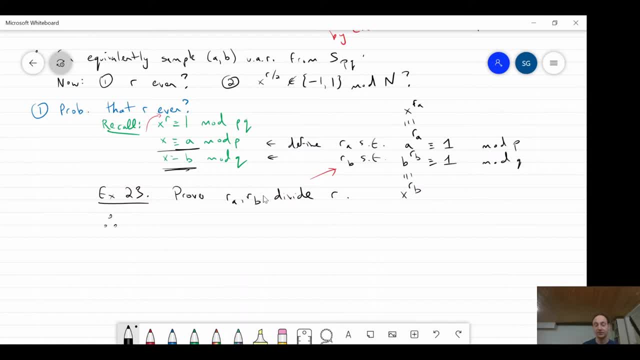 And so the conclusion, you know, assuming you believe this exercise, So if r a, you know, or r b, it doesn't really matter- is even, then r is even right, Because if r a divides r and r a is even, it contains a prime factor of 2, then certainly 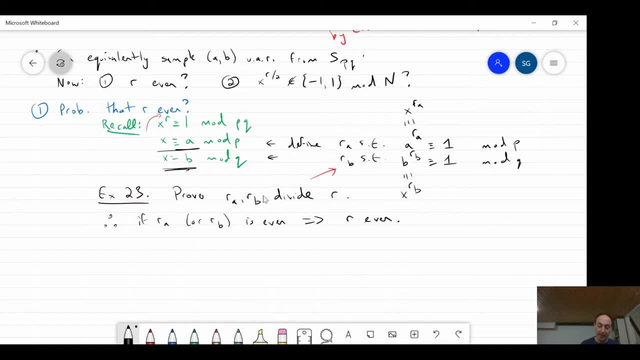 r also contains a prime factor of 2.. Okay, And so, therefore, the question is: you know, what is the probability that r a is even okay? And this turns out to be a little bit easier to prove because, remember, r a is not defined. 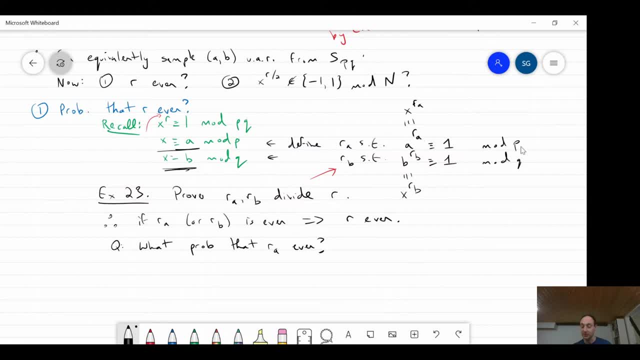 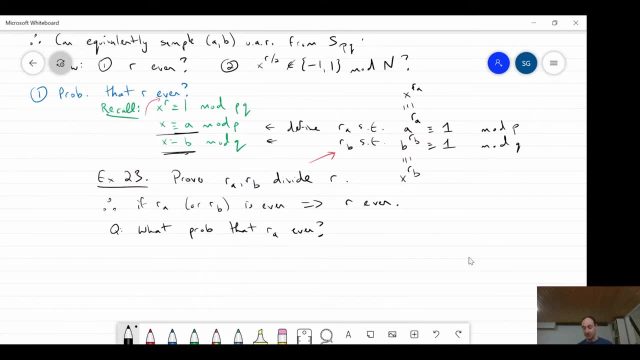 relative to this composite number, pq. it's defined relative to a prime, p. Okay, and that's a bit nicer to work with, And this is proven. basically, subsequent to this main theorem, there's a lemma which I opted to leave later. 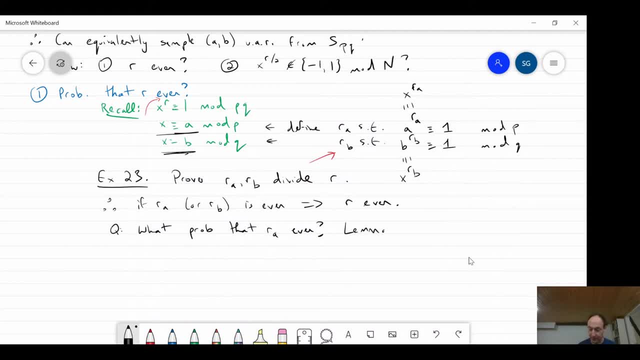 Okay, Okay, Okay, Okay Okay, Because I kind of wanted to show you the main lemma first and its proof and how things fit together, before we kind of fill in some additional details and we'll see if there's even time to do it realistically. 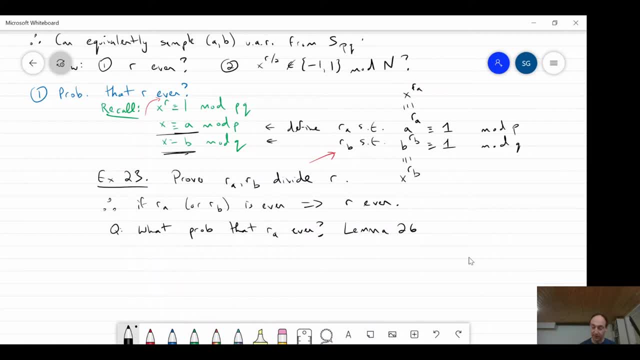 But it's in the notes, both the statement and the proof, And lemma 26 basically says that a uniformly random x in 0 to the dot dot dot p minus one has even order with probability at least a half. okay. so this is lemma 26 in. 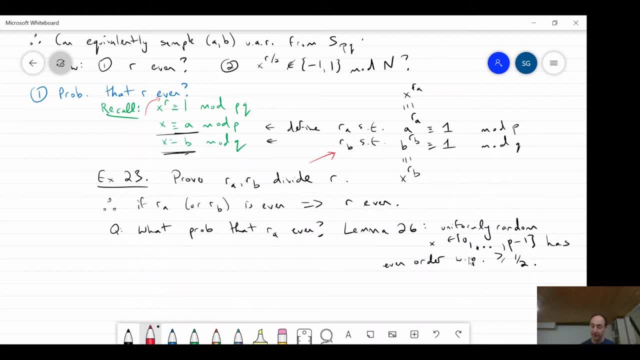 the notes. it's stated after this main theorem and proven there as well, and so, basically, when we just plug in this theorem, what we'll see, therefore, is that this probability is at least a half right. so we're talking about what is the probability that RA is even. that means that RA is even, with probably at least a. 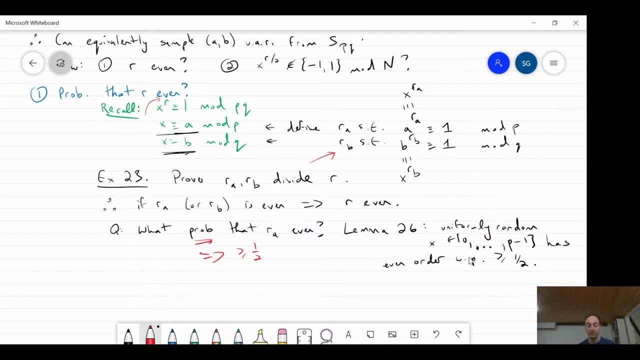 half okay. and likewise this is true for RB as well. right, so together this implies that RA is odd and RB. so the probability I should say that R is odd- I'd be a little bit less messy- and RB is odd is what? well, it's going to be at most a 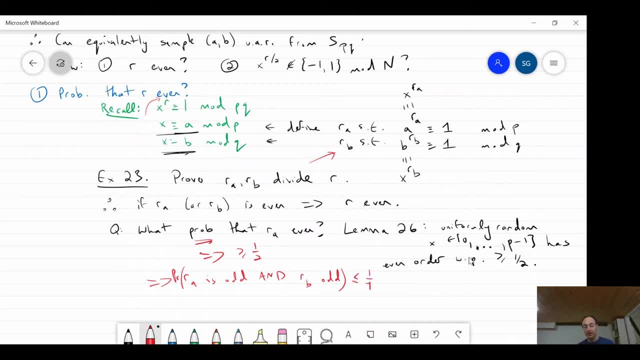 quarter right, because each of them is odd, with. probably the only way of they could both be odd is if you fail this test on both ends. right. so a half times a half is a quarter, okay. so, equivalently, at least one of them is even with probably at least three quarters, okay. so this implies that at 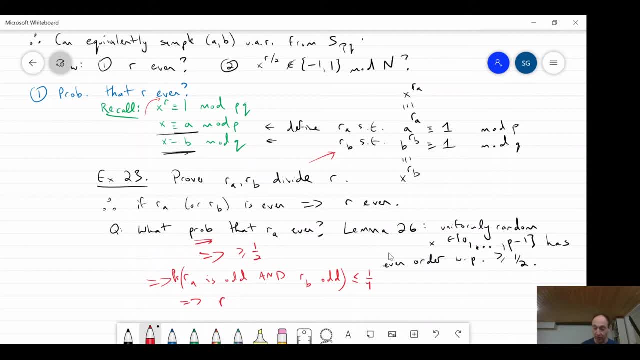 least one of them is, even with probability, at least three quarters, and hence R, the global order which is divided by both of these local orders, R is even. the probability of this happening is at least three over four. okay, so that's the first thing we wanted to check. if I pick X uniformly at random from Zn star, 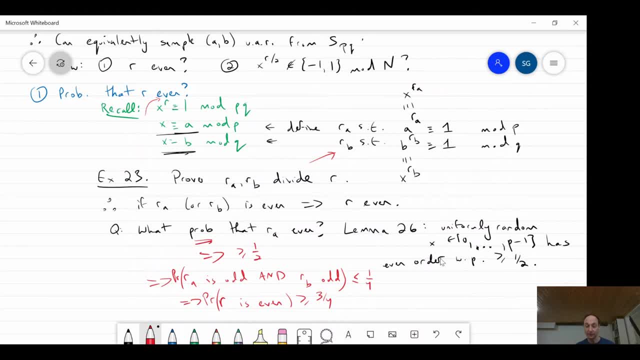 with probability at least three quarters, it's going to have an even order and so it's going to be well defined. for me to define this X to the R over 2 now and now, I need to check what is the probability that you know this solution. 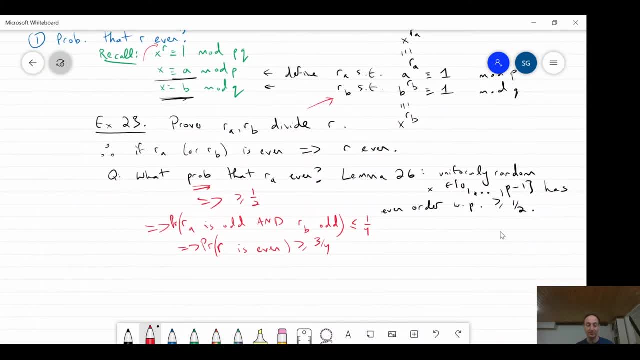 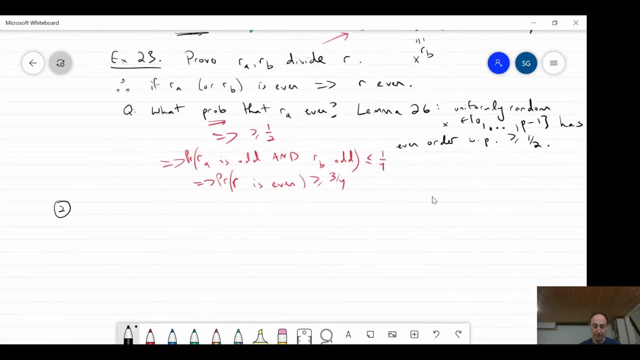 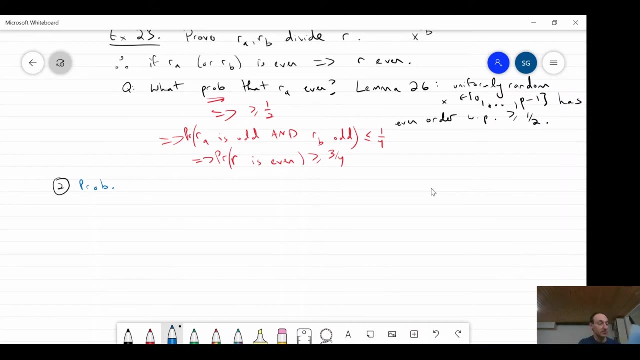 is trivial or not? okay, so let's do that now. so 2, did I do this with a color I did. let's be consistent. so what is the probability that X to the R over 2 is in the set plus minus 1 mod n? okay, and of. 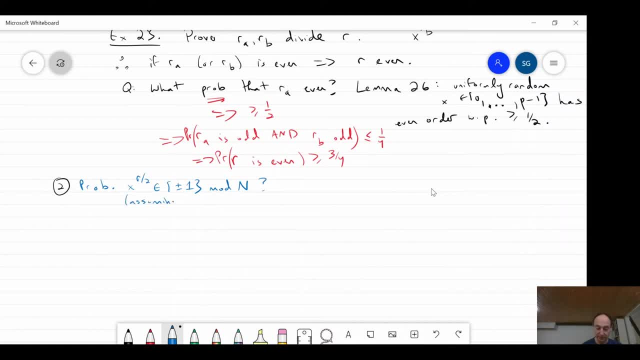 course this is assuming R is even so, we've already conditioned on passing the first step which we just perked. okay, so let's first make an observation. maybe I'll okay, let's just write here, so it's a bit cleaner. so the observation is that since we know that X to the R is 1 mod p times, 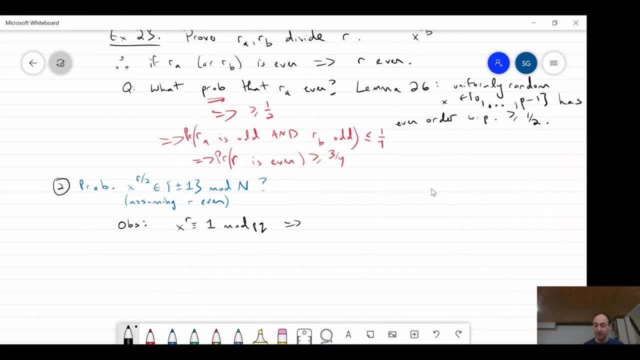 Q or n right. with a bit of thought, you can see that it's also true that X to the R is equivalent to 1 mod each of the primes individually. so and X to the R is equivalent to 1 mod Q right and and internally. the reason is because you 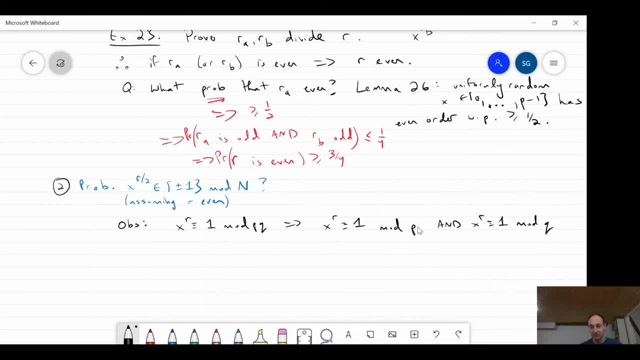 know what is P times Q. well, it's just mod P, but Q times right. so if you think of it that way, you can convince yourself pretty quickly, hopefully, that indeed you know both of these things are true. and if you think of it that way, you can convince yourself pretty quickly, hopefully, that indeed you know both these. 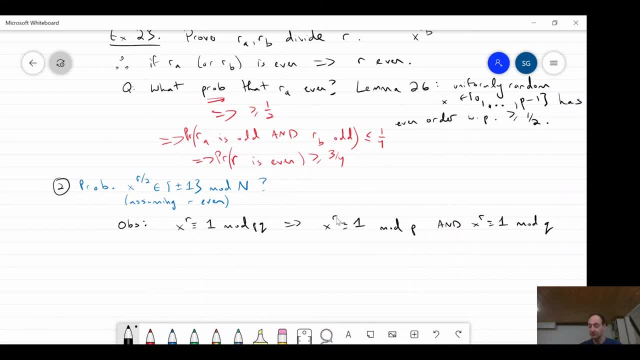 statements hold. okay now, of course, R is not necessarily the order of X. it was the order of X mod P- Q, but it might not be the order of X mod P. right, there might be now a smaller choice of exponent that still, mod P gives you one right. but 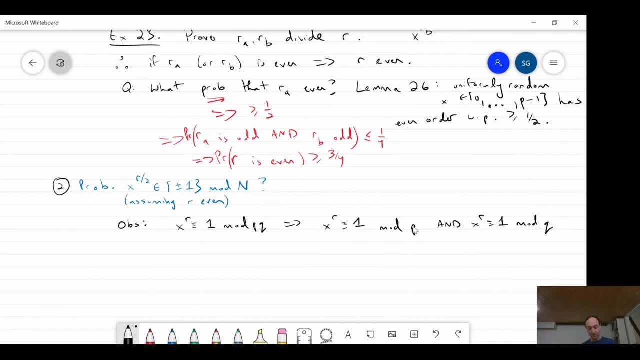 certainly this at least holds, okay, and so now we need an exercise. this is exercise 24, which states the following: it says, for all primes P, the equation X squared is equivalent to 1 mod P. okay, so again, it's very important, the modulus is prime has precisely two solutions. okay, what are? 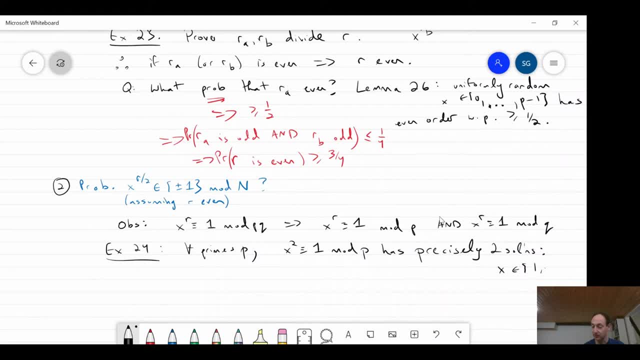 those two solutions. they are basically: X is either one. they're the ones you might expect. X is plus and minus one, right? so remember earlier we're looking for. X is plus and minus one, right? so remember earlier, we're looking for solutions to X- squared is equivalent to 1 mod n- that are non-trivial, right that? 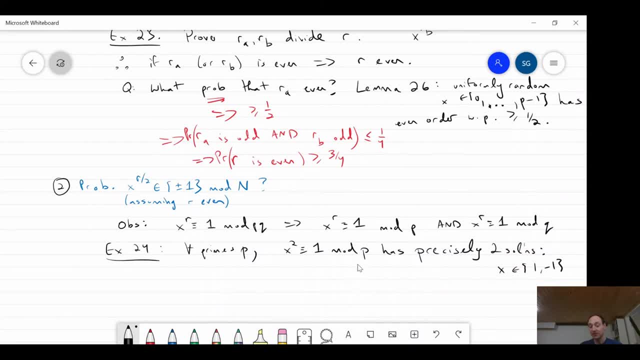 are not 1 and minus 1 and so that is possible because the modulus was not prime. but now the modulus is prime, right, so it turns out that modulus, when the modulus is prime, you really are kind of screwed. there are only the trivial solutions. okay, okay, so, of course, why are we doing this? well, intuitively, I mean. 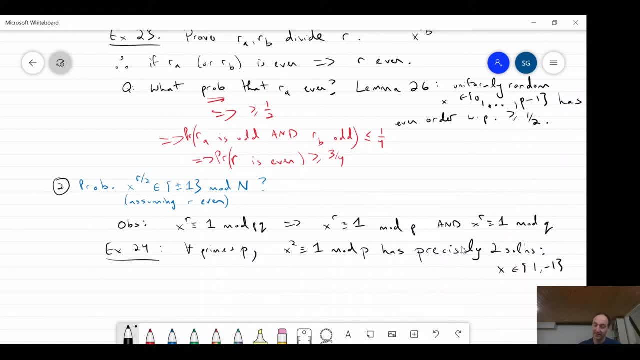 this is what we have here. well, okay, we're gonna get to that in a second. you know how do you prove this. well, intuitively, I mean: this is what we have here. well, okay, we're gonna get to that in a second. you know how do you prove this. 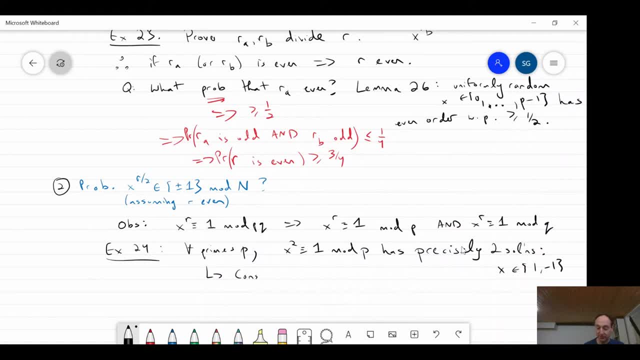 well, just think about, you know, consider, just rewrite the equation again as X plus one, X minus one is equivalent to zero mod P, right, and now P is a prime right. so think about all the numbers between zero and P, which P divides. well, there are only two numbers, right, either zero or P. that's what it means to be prime right. 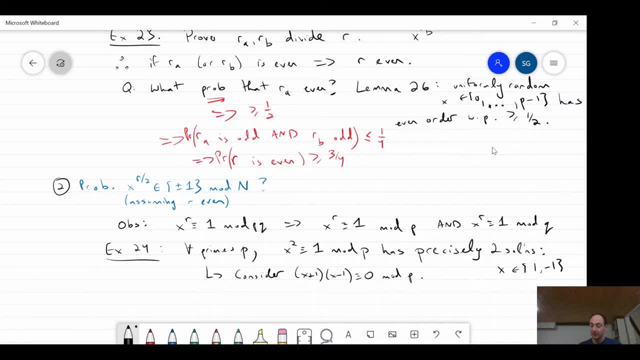 it doesn't divide one, two, three, up to P minus one. and so if this, what this is saying, is that P is supposed to divide, you know this product and so, because P is prime, you can't break it up. so you know P has to divide either this: 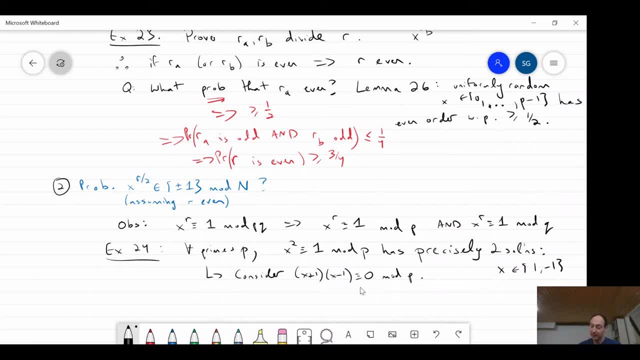 one or this one. that's the only thing that can work, and so in order for it to divide this one, you know, this thing has to equal to either zero or P- right, there's nothing else- which are of course equivalent mod P, and so how do you get? 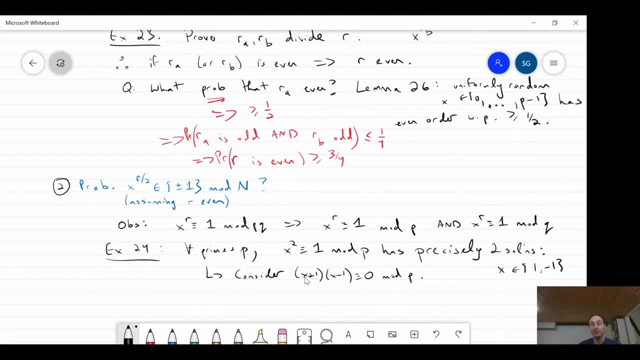 that. well, if X, for example, is P minus 1 or minus 1 equivalently mod P, then when you add one you will get zero mod, and then when you add one you will get zero mod, and then of course zero is divisible by P. okay, and likewise here, if I divide X to be: 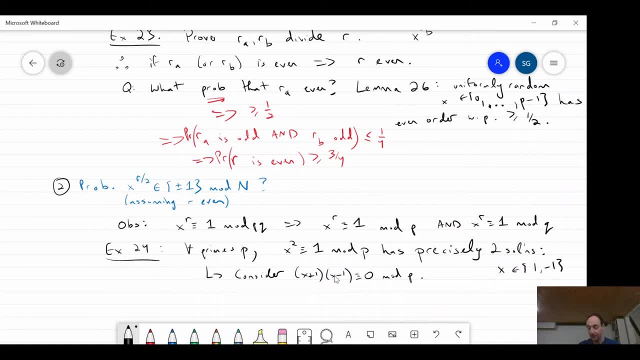 say 0, sorry, 1, which is the other solution. 1 minus 1 is 0 and of course, P divides 0. okay, so you know the. the upshot is that if my modulus is prime, then there are really only the solutions you would expect to this equation, which. 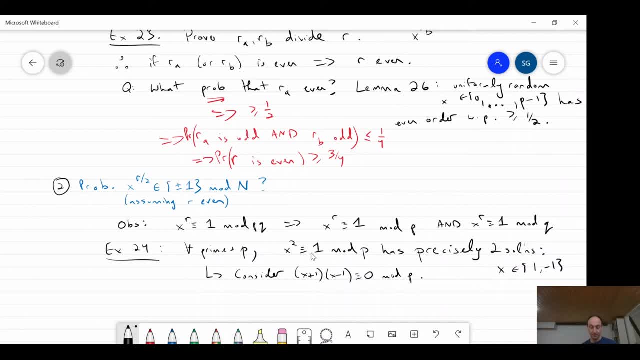 is X is either 1 or minus 1. okay, so you know why in the world do we want this? well, we want to kind of characterize all the possible square roots, basically because, remember, what we wanted to do is, you know, I'm looking at X to the R mod- X to the R is equivalent to 1. 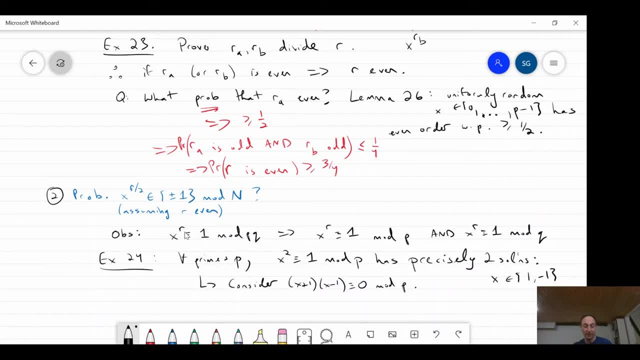 mod PQ right. this is my starting point, because R is even now I want to do a division by 2. I want I want to take the square root right. that was our plan of action and what we want to do now is characterize kind of all the numbers. 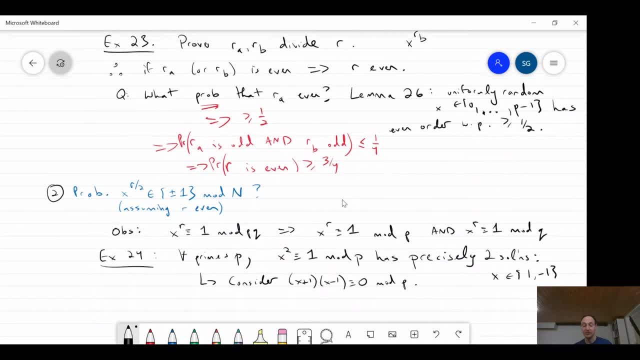 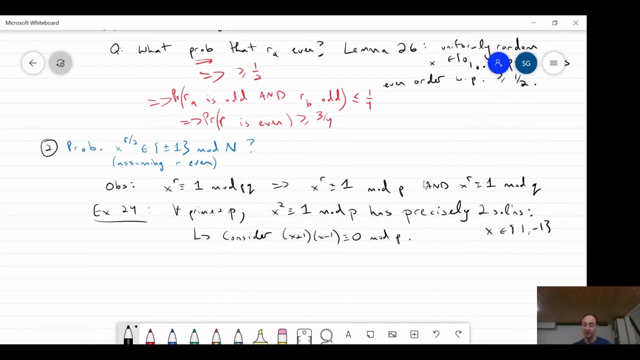 that can come up when we take that square root. okay, and it turns out that, you know, there are really only a very small number of possibilities- they're only 4, and we can kind of come up with all of them, characterize all of them, by just looking at these local orders, because locally, when these are prime, 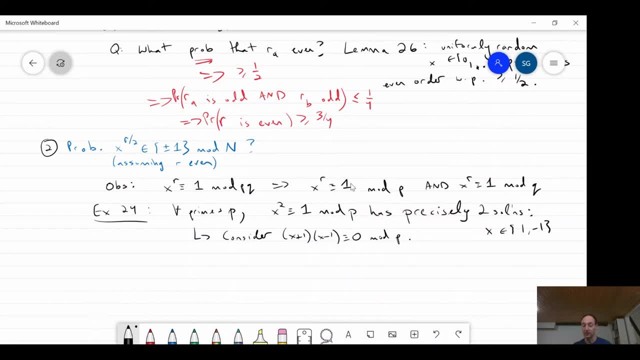 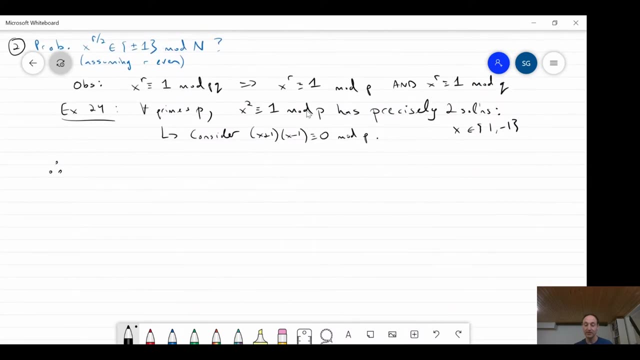 you know the square roots of 1. when I take R over 2 here, and hence the square root of the right side as well, the square roots are very limited. they're only the trivial ones. okay, so let's just put all that together. what does this tell us? right, if I take the square root mod P of X to the R and 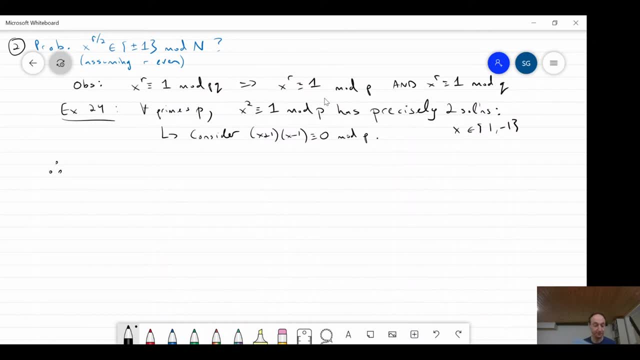 and hence also of 1, and same thing for q. what we say is that x to the r has precisely no more, no less, um two square roots. um, okay, it's by which, remember, i mean x to the r over 2. right, that's the square root. 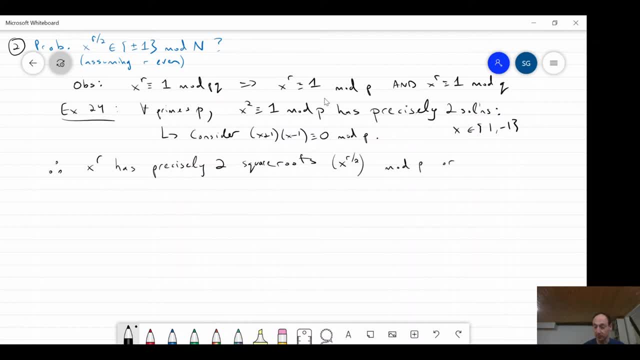 um, mod p or mod q, right, and those square roots are uh, 1 and minus 1, right? those are the only two square roots we can get out, and so that means that one of kind of four scenarios has to hold right. so i'm going to write down four scenarios. these are the scenarios i'm just going to give. 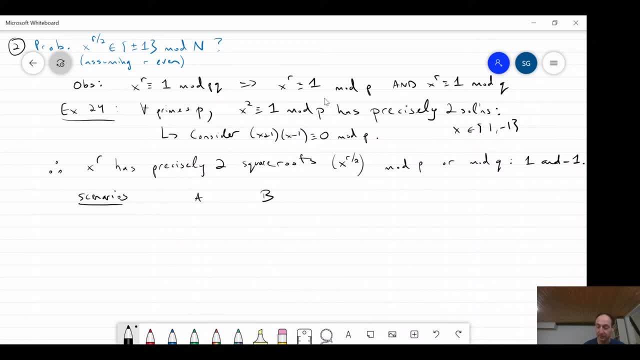 them names, but it doesn't really matter. we'll call them a, b, c and d. let me draw a bit further back, and so each of these scenarios, basically, i'm first, i'm going to write down four scenarios. these are the scenarios. i'm going to give them names. 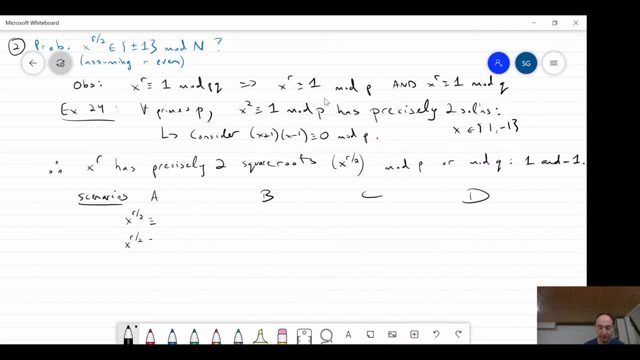 i'm just going to write the same thing over and over again. if i'm smart, i'll be able to copy and paste it without rewriting it. let's see if that's going to work. let's take this full thing. okay, let's see, copy paste. hey, that worked sort of. let's see. 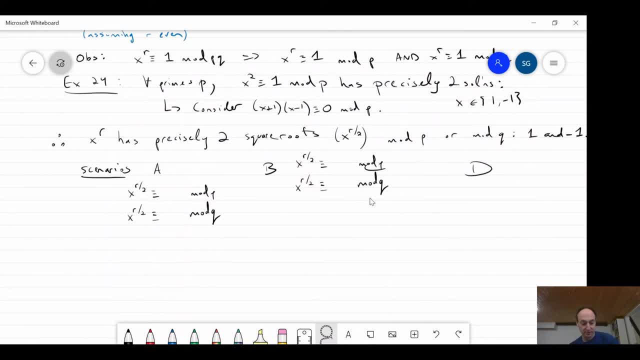 did that work, right? you know what did not? oh no, okay, let's not do that. i'm not entirely sure how to do that, right? okay, well, let's just rewrite it. probably be faster by the time i figure it out. so the only question, of course, is: you know, just so you're thinking, maybe you'll already figure. 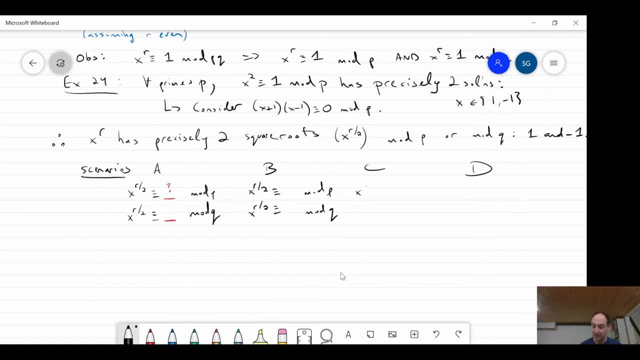 out what the answer is. you know. the question is: what do i put in? put in these gaps, right? what are the four possible ways to fill out these gaps, given what i've just told you about the possible square roots in mod p or mod q? okay, good, so now you've had some time to think about it. so you know, for each of these, there are: 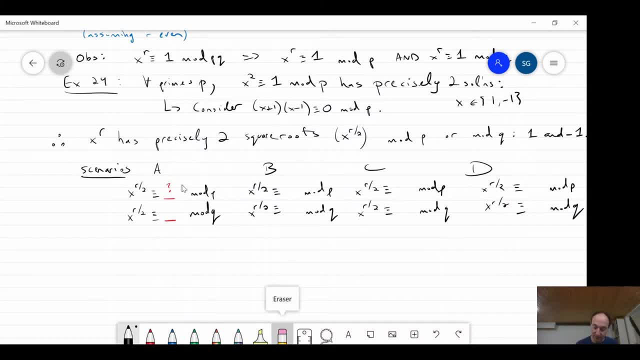 only two possible choices. it's plus one or minus one, so there'll be four possible combinations, right? so you know, either this is one- sorry, let's just do one and one first- or you can have one minus one, or you could have minus one one, or finally you could have both, being minus one, okay, and 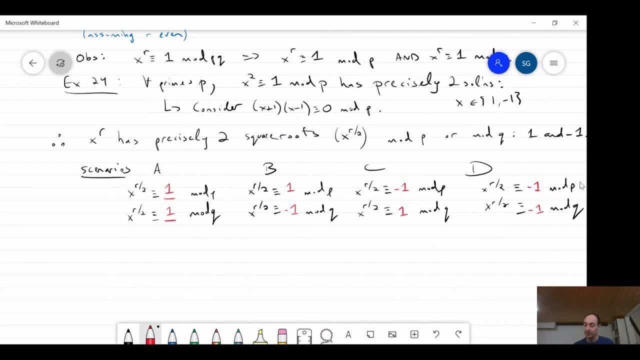 remember that, of course, minus one is equivalent to one minus one. so you can have one minus one, or you could have one minus one, okay, and remember that of course, minus one is equivalent to say: uh, p minus one, one, okay, okay. so these are. you know, one of these four has to hold. so, for whichever choice, 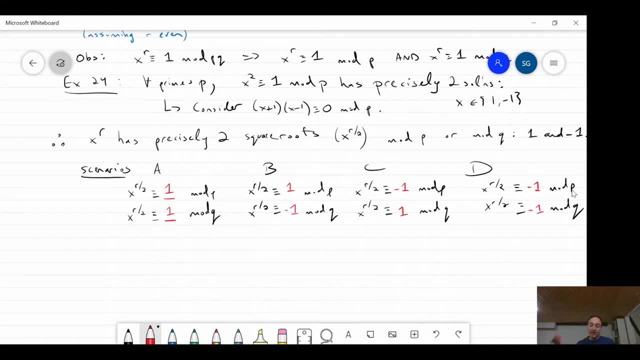 of x. i have in mind, right um, you know, when i take mod p, mod q um, with the square root of x to the r, right um, you know, one of these four kind of patterns has to come out, okay, and that depends on the choice of x. but remember, now that you know p and q are co-prime. so 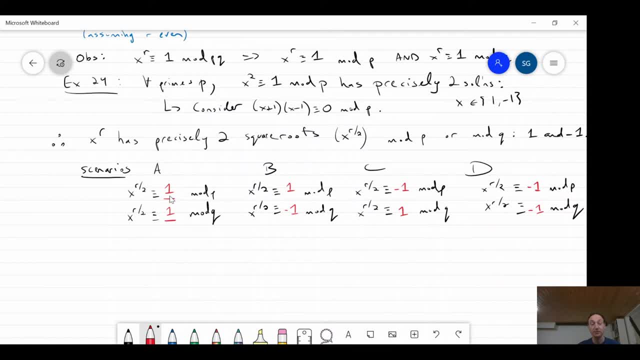 specifying, you know, these two right hand sides of this equation. right completely specifies what goes on the left hand side, right, that's just the chinese remainder theorem. you can go forwards and backwards between the global view, uh, in terms of p times q, and the local view in terms of. 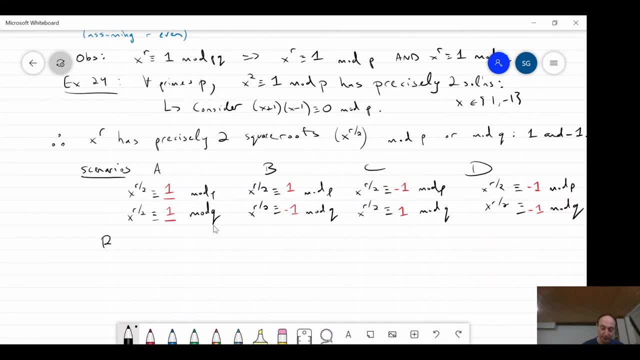 mod p or mod q. okay, so by the chinese remainder theorem, each scenario yields a unique kind of global solution: um. x to the r over 2, which, remember, is equivalent to um, it's just x to the r, of course, to the power half, because we took a square root and um, you know, mod n. what was x to the r? well, x to the r. 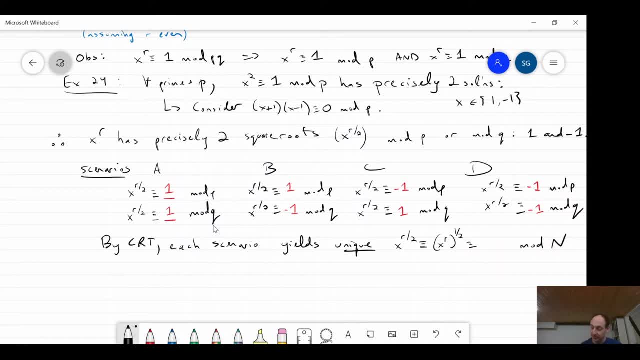 mod n is just one by you know, that was our assumption and so really, this is just, you know, one to the power, a half right. this is the square root of one, basically right, okay, so in other words, what we're saying is that you know each one of these four patterns, you know. 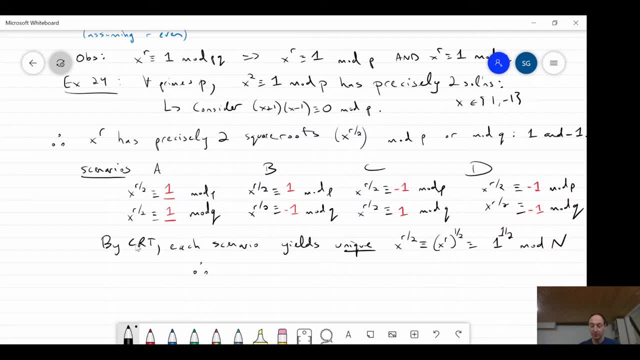 if you kind of interpolate, if you will, if you go backwards and you use the chinese remainder theorem to come up with a global solution, mod n, right um- each of those will give rise to one of the square roots, basically of one mod n. so in other words, there are precisely four square roots of one. 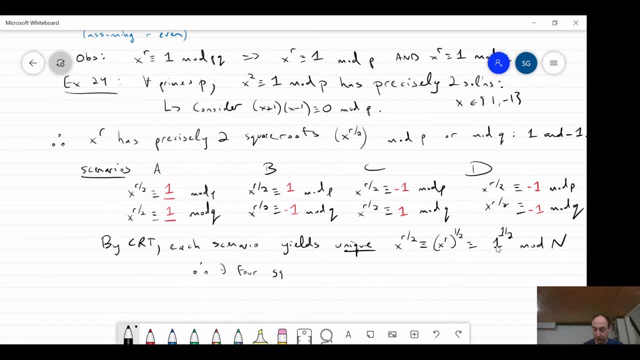 there exists, uh, four, precisely four, square roots of one mod: n, right and um and x to the r over 2 is one of these, right? okay, that's what this is saying. okay, and so what are the four square roots? well, um, so two such square roots are kind of the trivial ones, right, you always have the. 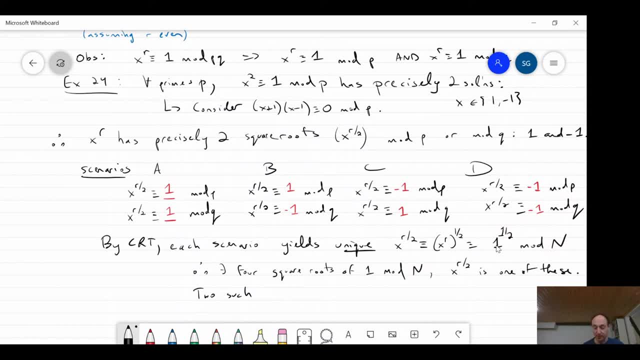 square roots 1 and minus 1, those are always square roots of 1, so two such square roots are where is this? 1 and minus 1, and these are, you know, the bad ones, right? These are the ones we don't want. 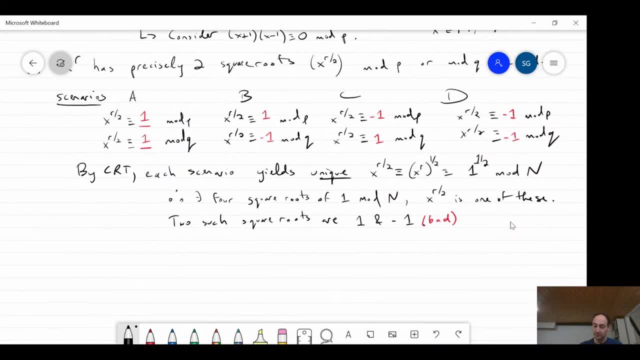 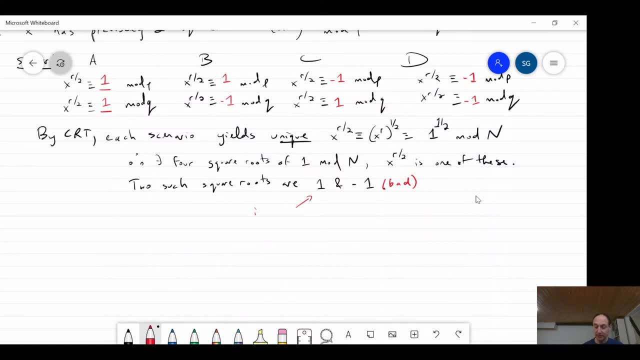 And now this is again going to be impossible, and remember the reason why is because if it's true that x to the r over 2 is equivalent to 1, right. if it's that square root mod n, then that contradicts the fact that r is the order of x. 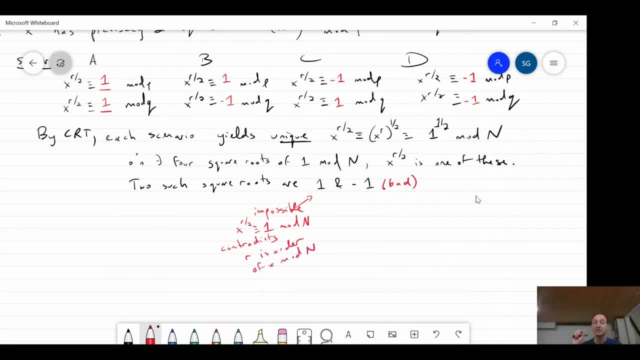 mod n right. So x to the r? r was supposed to be the smallest exponent that takes you to 1 mod n, and so we know that it cannot be true that you know x to the r over 2 is equivalent to 1.. Okay, 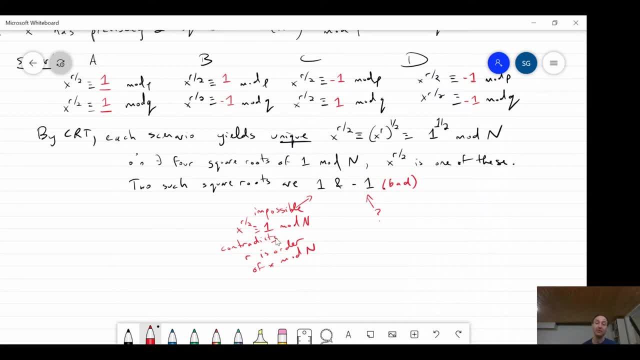 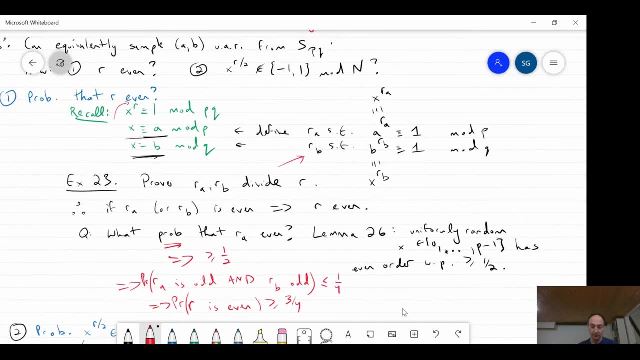 so this still kind of hangs around, though this is the other bad case, which is essentially what the statement of the theorem was saying. right, We wanted to say this thing, right? Well, in the statement of the theorem, we only listed the second case right, which was: 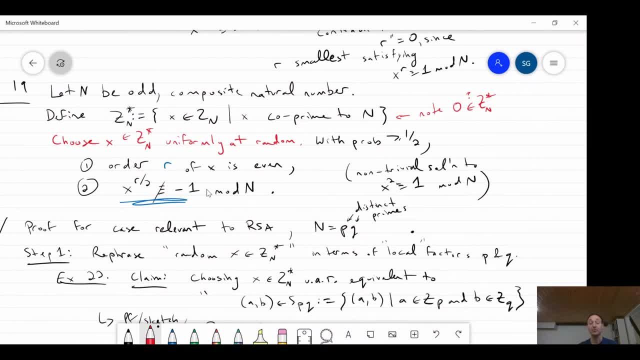 that's a pretty long theorem, huh. x to the r over 2 is not equivalent to 1 mod n, right, So this is the one we have to worry about, therefore. and so what are the odds that this is going to happen? 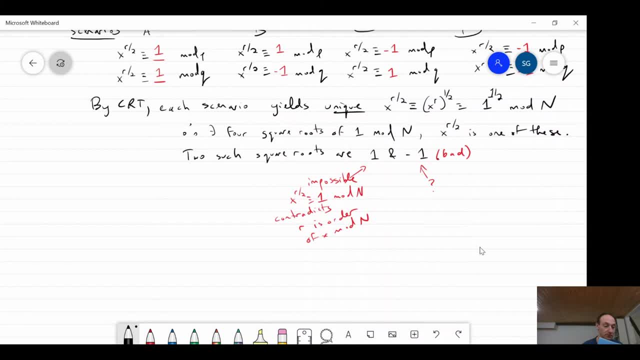 Okay, so the conclusion is therefore: let r denote the remaining three square roots of uh one of uh 1, mod n. Okay, zur uh. uh, those which are not equivalent to 1, right, Cuz we were able to remove uh 1, so there only 3 left. Okay, then you know. exercise 25 basically says that: um choosing. 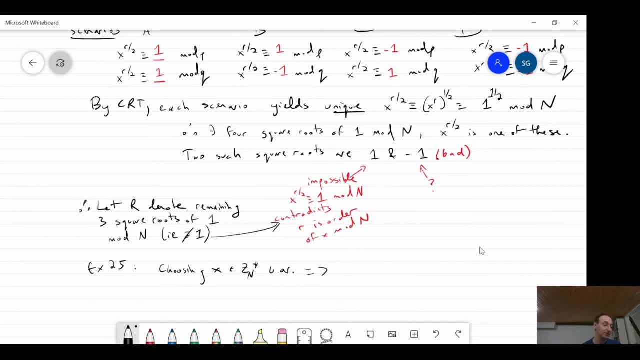 essentially assuming that, uh, the order er was even implies that, um, you know x to the r over 2, you know this kind of. the square root of n we get is uniformly at random from the set r i just defined. okay, so again, r is just: there are three square roots, we're basically picking one at random. 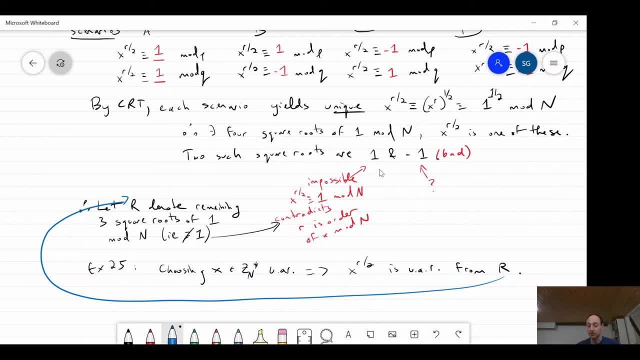 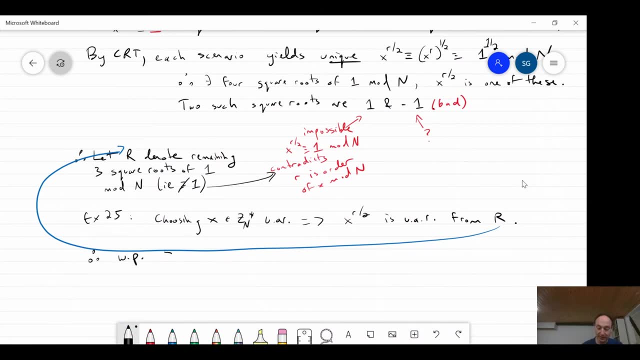 one of them is bad, the other two are good because those are the non-trivial ones. they're not one or minus one, okay, so this basically tells us that, uh, with probability at least two-thirds, um, we get a non-trivial root of one. okay, well, maybe i should, maybe a little bit more succinct, um. 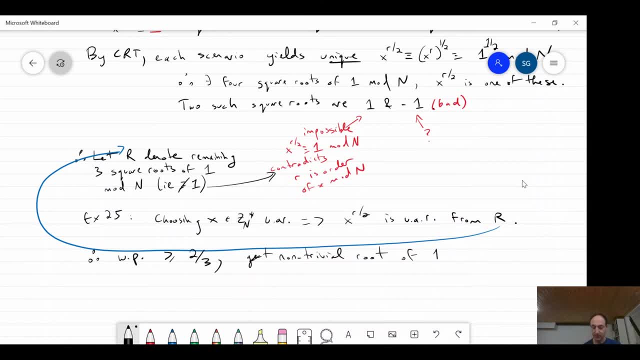 okay, it's lagging again, so maybe after this section i can pause and um reset. we'll finish order finding stuff and then i could reset the journal. okay, um x to the r over 2 is not equivalent to minus one mod n. okay, and so you know there are two things. 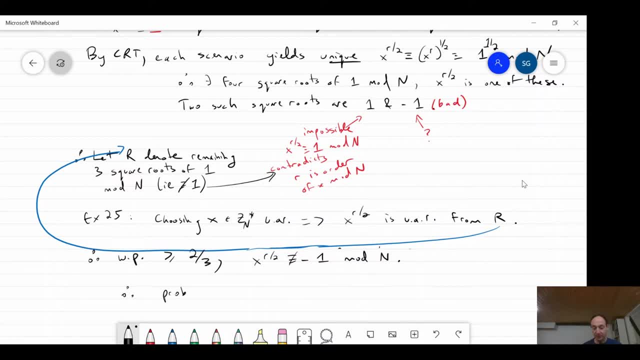 so the probability overall of uh success, right when i picked um, a random x was, remember i needed to. first i needed the order to be even and that was probability half. sorry, sorry, that was not probably half, that was probably three quarters, all right. and then um, once my order was even, then the probability that i got a non-trivial. 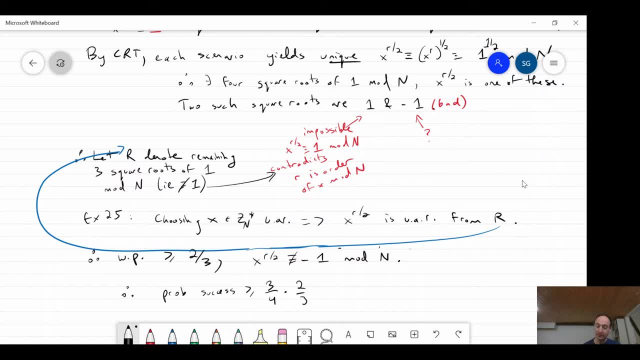 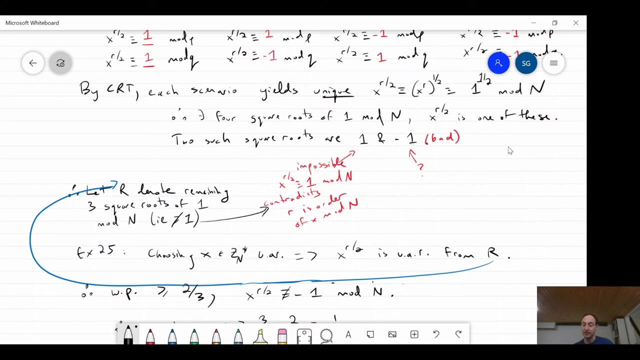 square root of uh one was two-thirds right, and of course then we combine these and we get the value of half. uh, we were looking for for the proof, okay, so that is basically um the proof. you know, that we can reduce factoring to order finding. okay, so just to recap, basically, um. 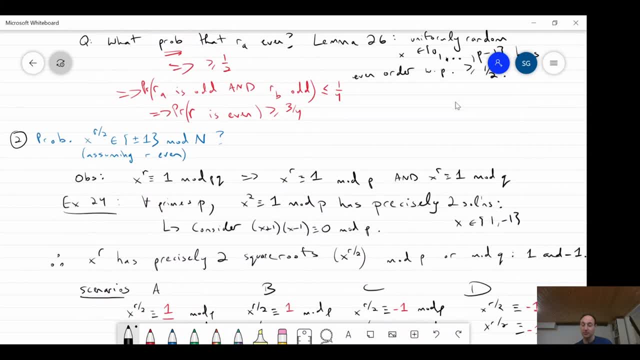 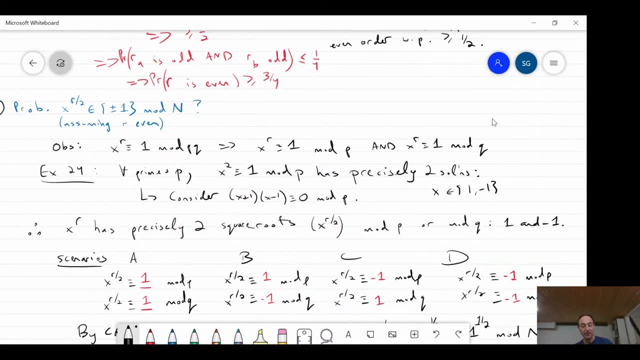 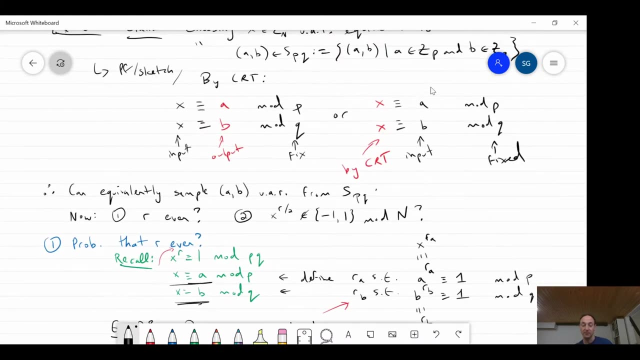 remember we said that if i can find a solution to x squared is equivalent to one mod n, such that the solution is non-trivial. so i can find a solution to x squared is equivalent to one trivial, then i can factor in. okay, i can rip out one of the prime factors. and um, then we said: well, 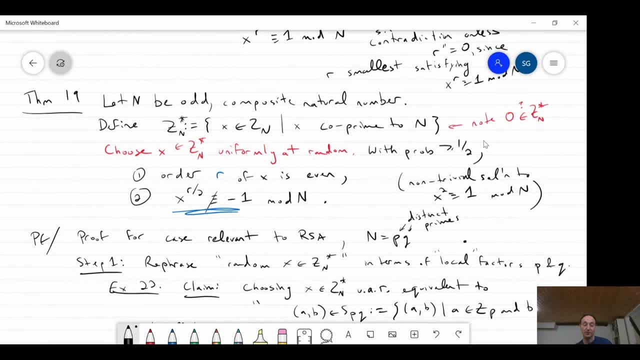 how do you find a solution to that? well, basically, it was sufficient to randomly sample x from z and star in such a way that number one, the order r, was even, so that then i could take a square root. and the reason, remember, we took the square root is because we want to satisfy something. 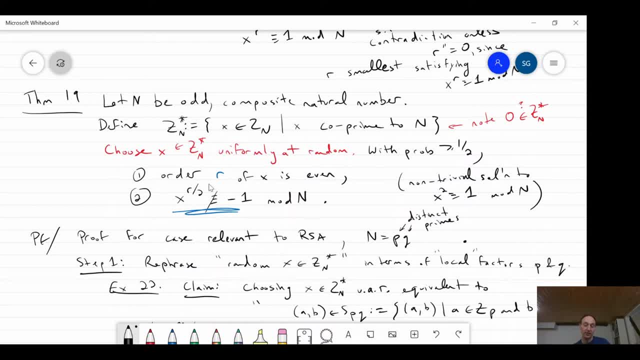 squared is equivalent to one mod n, and so if i take the square root, then when i square this back again, i'll get x to the r, which is equivalent to one mod n. okay, and the problem is that, you know, i know something about x and the r, but i also need to guarantee that when i take the square root, um. 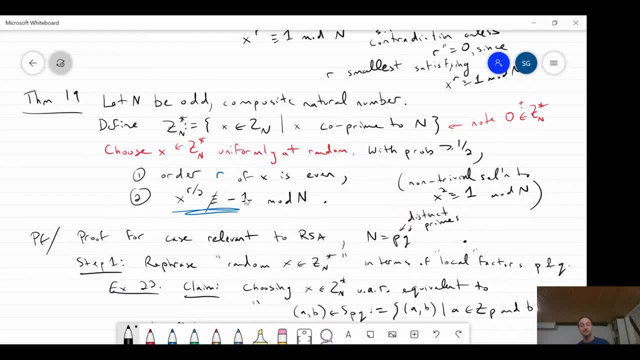 i don't get a trivial solution basically. so it shouldn't be minus one, okay, and um, and the probability of that happening is at least a half, okay, so you could repeat this, of course. um, this random sampling of x a number of times to bring the probability of failure, you know. 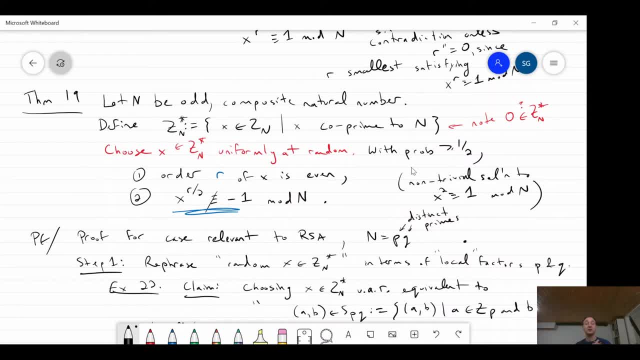 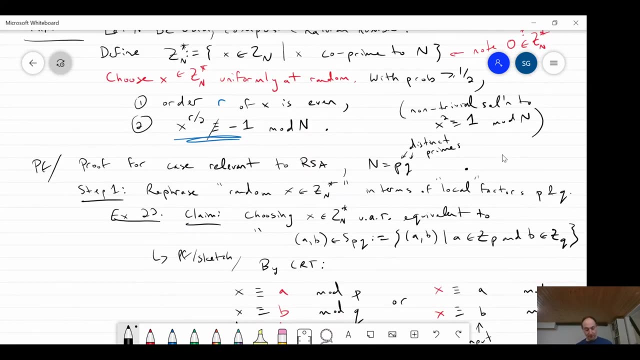 what you want, um, and then at that point, you you know, you can rest assured that, with high probability, um order finding will allow you to solve factoring. okay, so let's see how long this is gone. it's an hour and a half, so what i'm going to do is i'm not going to prove um, so there's a. 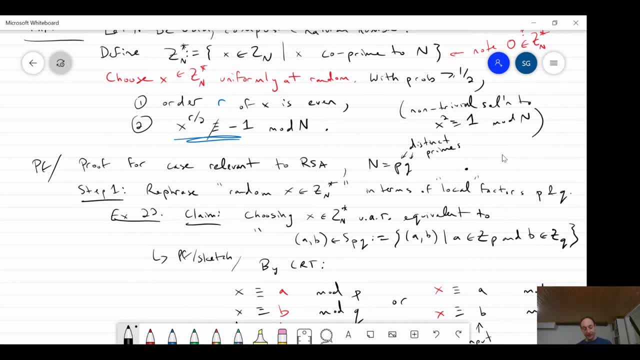 lemma in here, lemma 26, that we use during the proof of this mean theorem. that lemma is stated and proven in the course notes and you know it's just a couple of lines but in the interest of time i'm not going to prove that in the lecture. you're always welcome to go to the lecture notes. 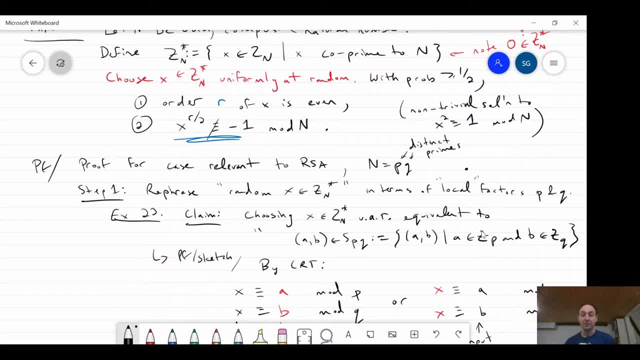 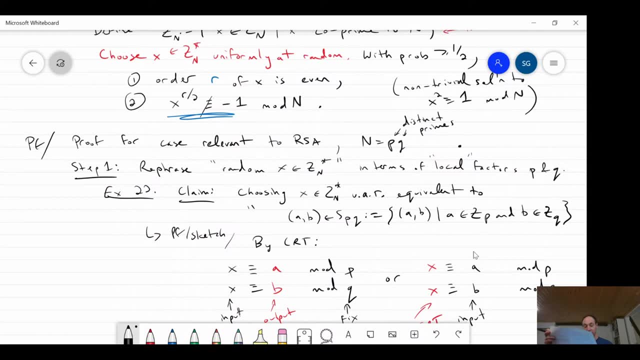 and look that up. okay, but instead in the in the remaining time, we have maybe about an hour left. um, i want to make sure we talk about the remaining part of the lecture, which is: how do we use quantum phase estimation and continued fractions and finally, you know, just quickly go over how we break. 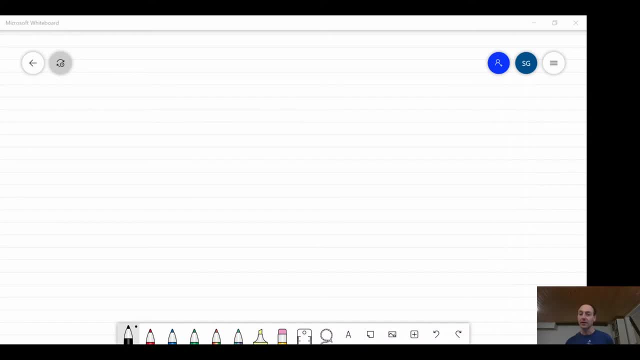 rsa. okay guys, so now that we've reduced factoring to order finding, now we can go ahead and solve the order finding problem using a quantum function. okay, so the algorithm will consist of two components, um: a quantum component, which is just basically quantum phase estimation, and a classical post-posting component, which is going to be the. 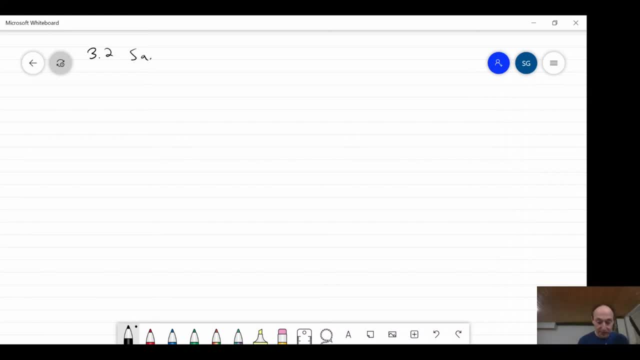 so-called continued fractions algorithm. so i'm going to start by telling you about how to do the first, the, the genuine, the only the only genuinely quantum part of this whole algorithm, which is sampling via quantum phase estimation. okay, so recall. therefore, the goal here is, you know, given: 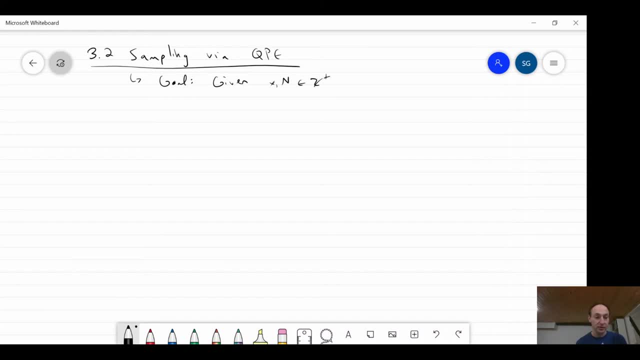 x, n positive integers such that x is co-prime to n. what is the order r of x mod n? all right, oops, okay. so basically what? the quantum algorithm is just going to be an application of quantum phase estimation, but of course there will be a few challenges to this right. it's not just going to be. 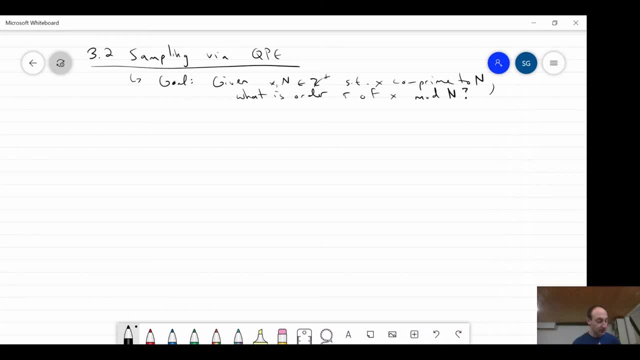 that straightforward. let me just remind you very briefly, in phase estimation, and you know the circuit looks like this. so this is figure one in the notes. but you know, let me just do a brief sketch on the side to jog your memory. so remember you can. seeking to solve a simple quantum phase estimation. 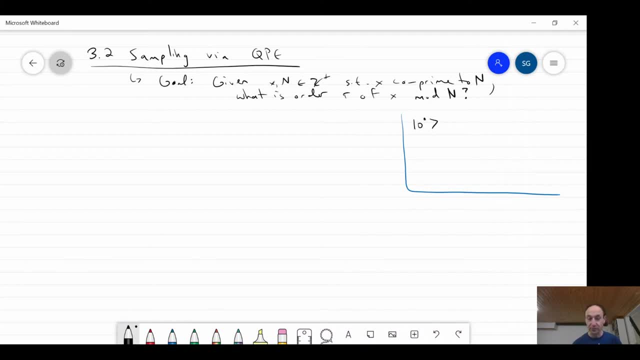 olhar for every xu wang you set to keyword one. you can count within this little ở yang to So remember in phase estimation. what it did is you gave me an eigenvector of a unitary and phase estimation gives us the phase of the corresponding eigenvalue for that eigenvector right. 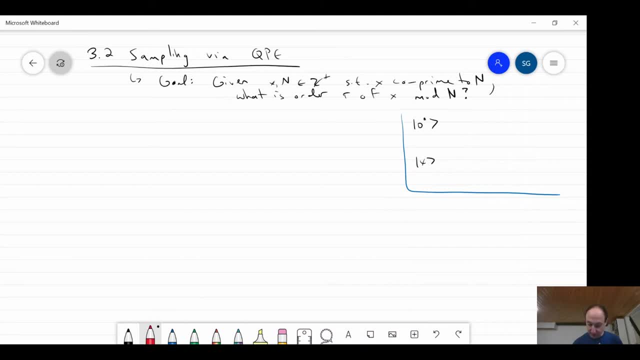 So you plug in two things. remember that this is going to be the eigenvector of the unitary in mind. this is going to be where the phase will get stored, so it starts with just being 0 to the n, and then we plug it into the circuit and from last class we saw what we first do. is you know? 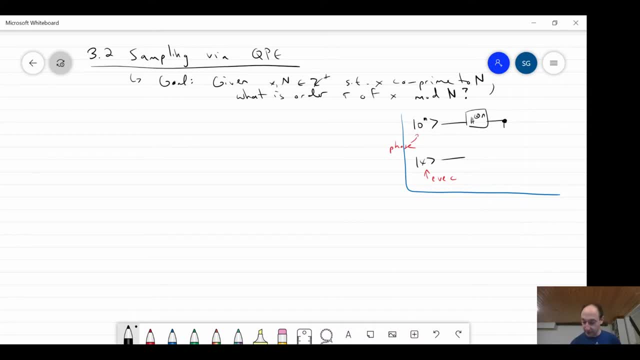 n Hadamard transforms in parallel, followed by a controlled u, to the power k operation right. So u psi is an eigenvector of the unitary u, remember, and so the control here dictates. you know to what power we're raising u basically. 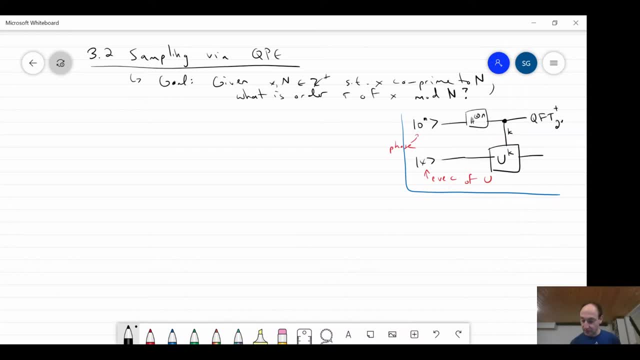 And then we did an inverse quantum Fourier transform. so if the details of that escape your mind, don't worry. I mean we're just going to use phase estimation as a black box. now this is just for you to you know, recall a little bit what this thing looked like. 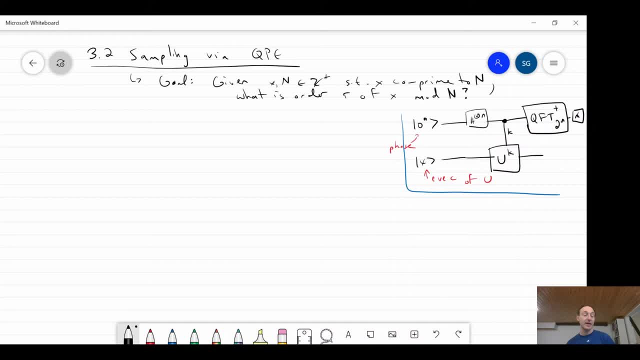 Okay, so now there are three questions we need to ask right, Whenever you're going to use phase estimation, right? Number one is, of course, I'm trying to solve the order finding problem and phase estimation requires me to you know, plug in some unitary u right? 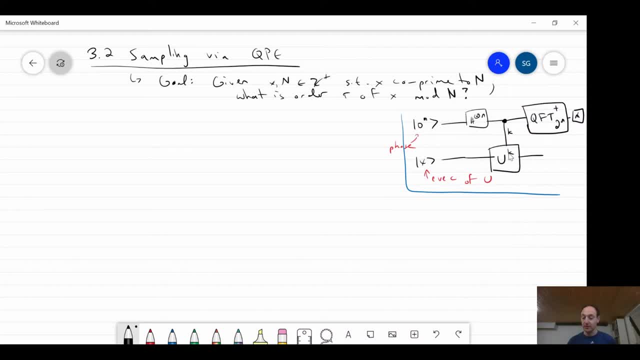 That's this gate over here, right? This one over here. So what is u right? How do I encode order finding into a unitary number one? Number two in my list is for phase estimation. I also need an eigenvector, right? 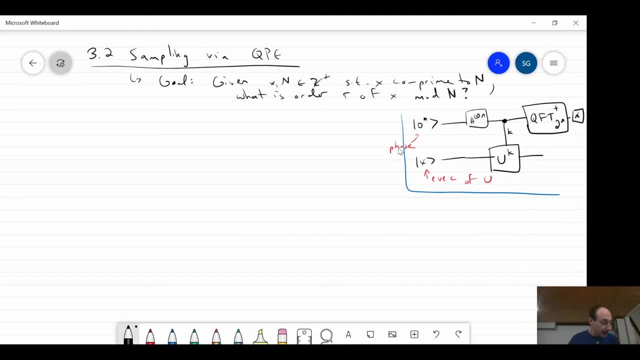 So where is this going to come from? Okay, And last but not, three phase estimation. remember, had this funny thing where the amount of precision I get kind of coming out of the phase in this first wire, right, That will depend strongly on, you know, the power to which I need to raise u here, right? 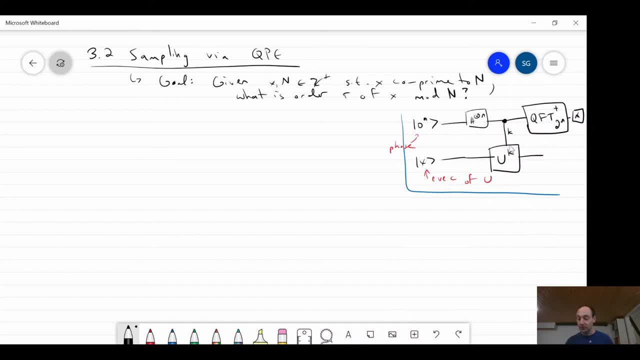 So, in particular, if you want n bits of precision, we need it to be able to raise u to the power 2 to the power n efficiently Right. So can we even do that For the choice of u which we have not yet specified? 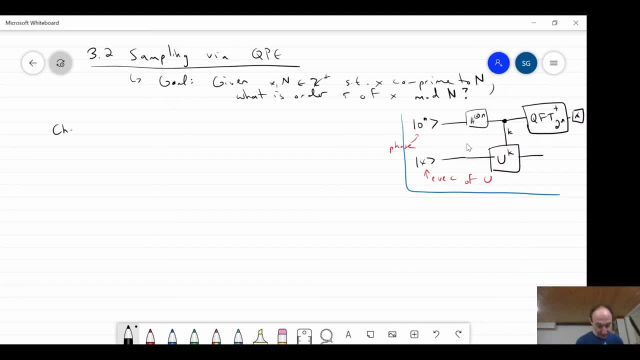 So let's start with you know the first challenge here, And once you know we answer these questions, then we just plug in phase estimation as a black box. So challenge one is: what is u Okay? so to what do we apply the phase estimation algorithm? 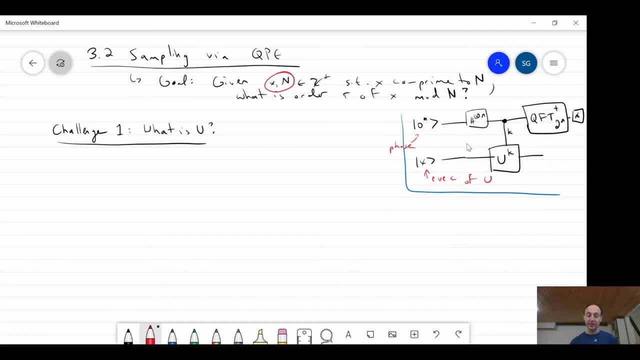 And so the input to order finding is this up here: right, It's x, m. So what we're going to do is just define the unitary u. So of course it depends on this input x, because that's kind of like, fixed as part of the input. now, 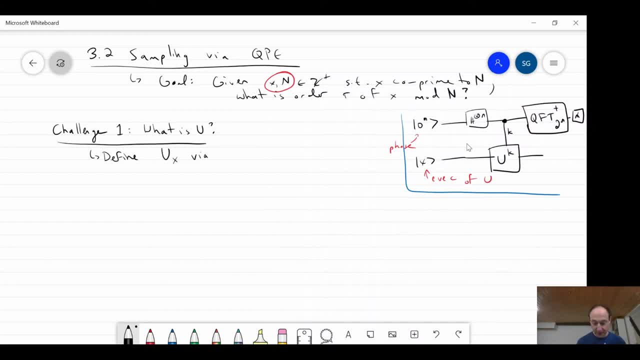 So we define the unitary u And again I just need to specify its action on a basis. So I'm just going to specify it on the standard basis. So if I apply u to you know some standard base element y. 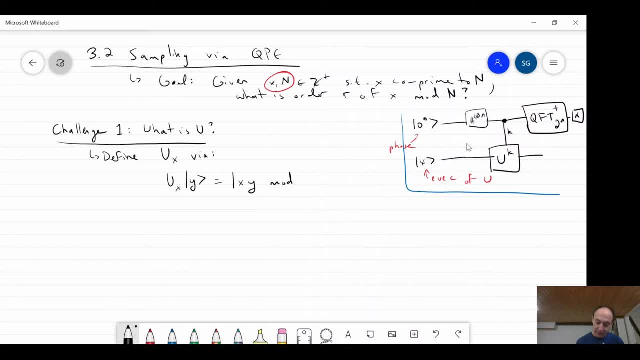 all it's going to do is x times y mod n. right, It's going to send it to the string which represents the answer of that computation. Okay, and so you can. you know the next two exercises, 27 and 28, in the notes. 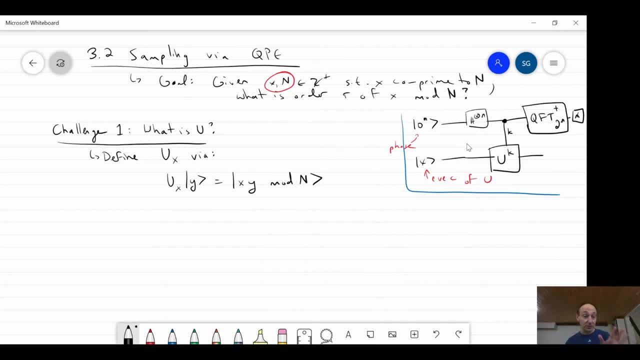 those exercises get you to convince yourself that, indeed, u is unitary, right. So that's the unitary u. Okay, and now let's try and understand. you know why does this work right? Because ultimately, you know the point of this is that there's got to be some eigenvector I can plug in. 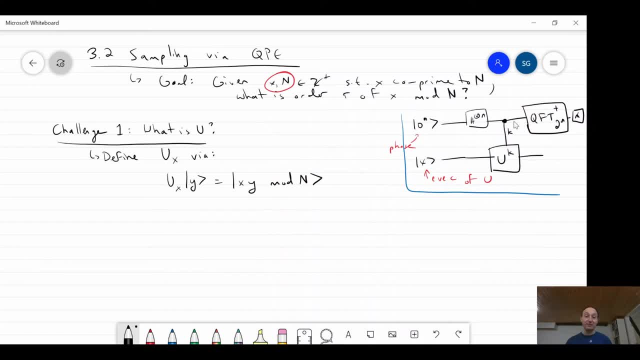 so that when I do phase estimation, the phase of that eigenvector is going to encode the function, The order of x mod n, right? So let's think a little bit about what are the eigenvectors of u and what do their eigenvalues tell us. okay? 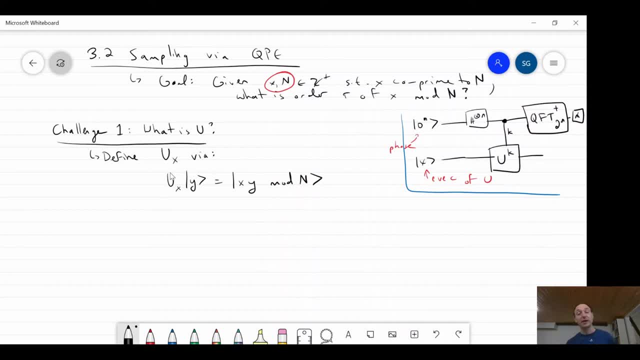 Okay. so what we're going to do is I'm going to try and build some intuition by building the eigenvectors of u kind of from the ground up. okay, So the question is, what are the eigenvectors of u? So here's attempt one. 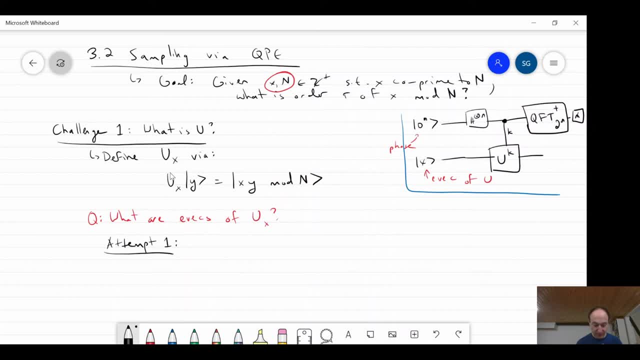 Obviously, I'm using the word attempt because it's not going to exactly work, But let's think about why we defined u this way. in some sense right. So what do we know? Here are two facts we know, right. So number one: I know that x to r is equivalent to 1 mod n, right? 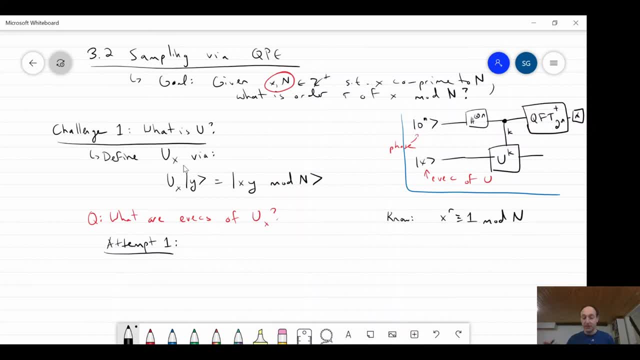 Just because, by definition, whatever r is the order it takes x back to 1, okay, And the other thing I know is that this operation, this one over here, right Basically the defining operation of u, what does it do? 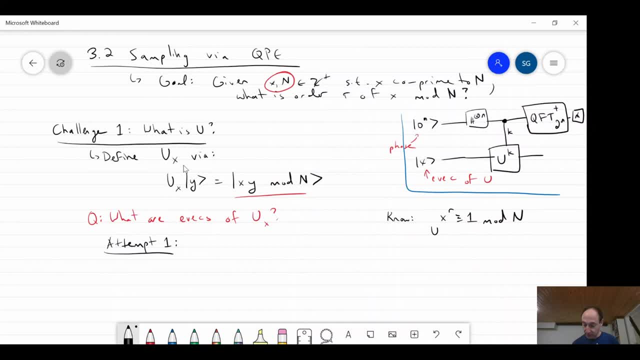 It allows us to produce this infinite sequence right. So u produces sequence 1, then x, x, squared, dot, dot, dot, x to the r minus 1.. And then of course it goes to x to the r, but that's just equal to 1. again, mod n right. 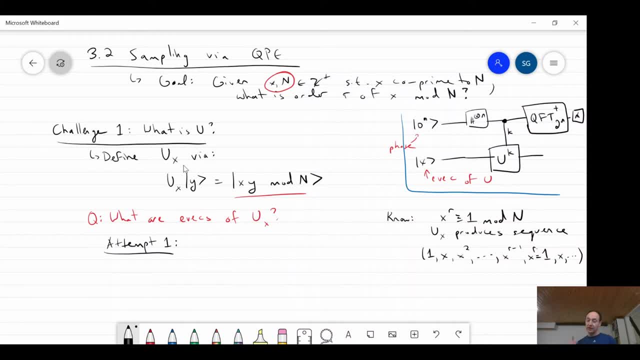 And then you know, the sequence repeats itself, right? So if I start with 1 and I keep applying u, it's just going to cycle through this sequence forever, okay, Good, So, since we have this kind of cyclic behavior, right? 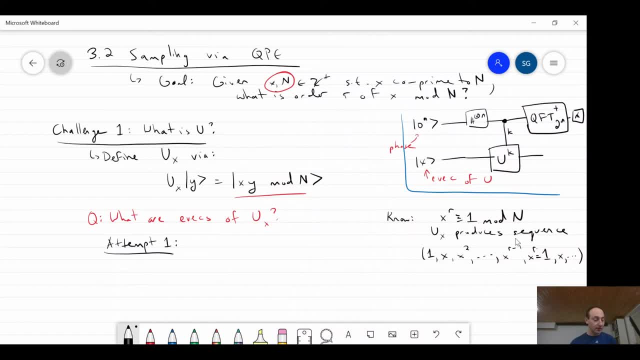 If I keep applying u, I get the cyclic behavior. A natural way to kind of define the first. an eigenvector of u is the following: right, We might say so let's just take a sum First. let's just take all these powers. 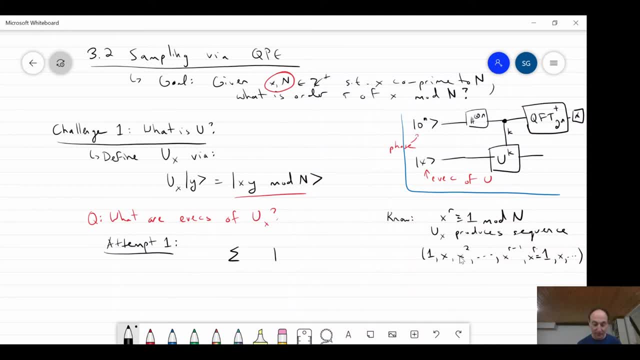 I'm basically going to encode the sequence, okay, into the cats. So I'm going to say x to the power, j mod n. Okay, so you know this thing is going to cycle. There are only r values for this thing, right. 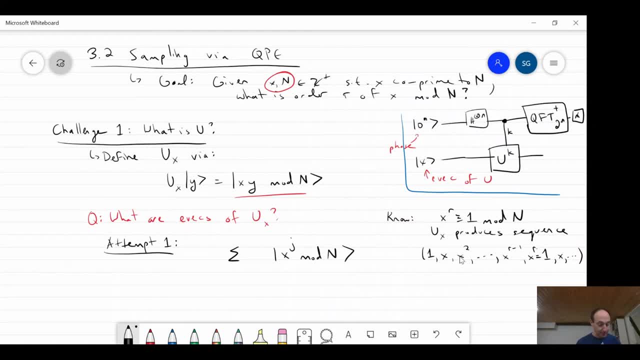 So, intuitively, we only expect r terms to turn up in the sum And indeed we're going to put: j equals to 0, up to r minus 1 and 1 over square root r. Okay, let me give this a name. 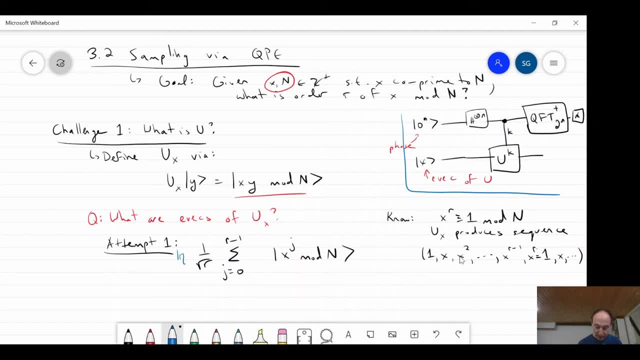 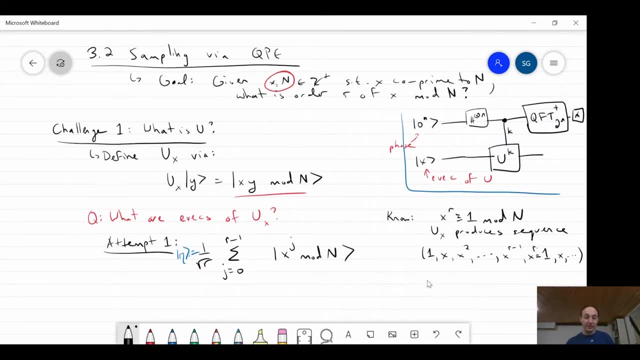 Let me just call it for our discussion, eta. Okay, so that is a natural first attempt at an eigenvector. Why do I say it's a natural first attempt? Well, because what happens, right, if I hit this thing with u on the left? 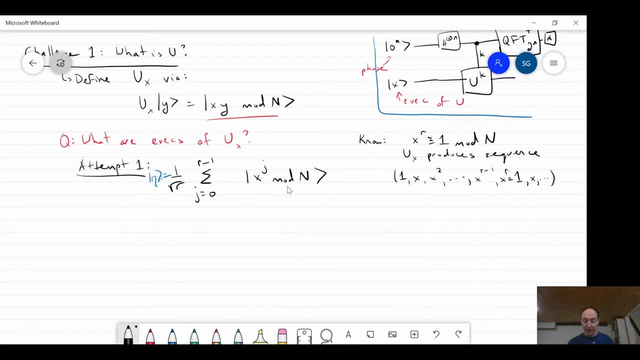 what's going to happen is that, you know, each of these cats, like x to the j, mod n, is going to get kind of upgraded to the next term in the sequence, right. So it's going to go to x to the j plus 1 mod n, right? 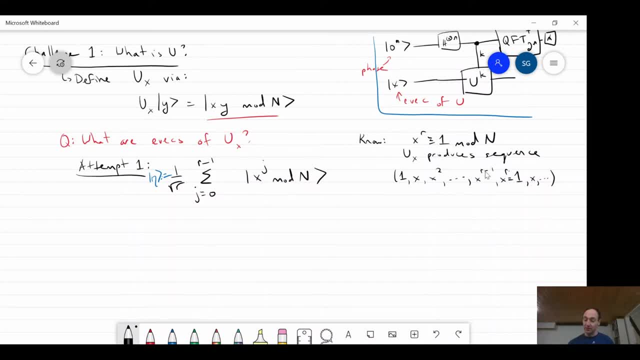 And the very last term in the sequence, of course you know this- x to the r minus 1, that one wraps around and just goes right back to the beginning. So, in other words, every time I hit this thing with u right. 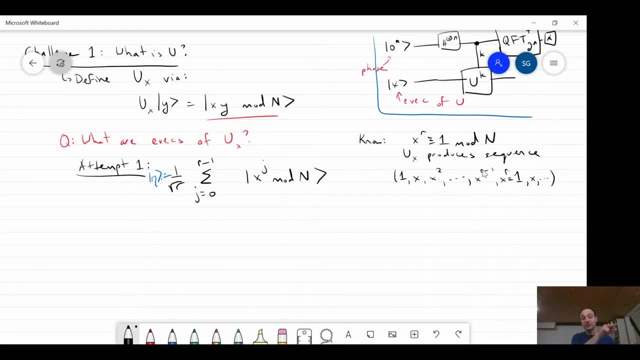 all the terms will kind of take a step forward and the last guy will go back to the first slot, right, So it's just going to cycle through the elements basically every time I apply u. So if you think about this a little bit, you'll see that u times eta is just eta. 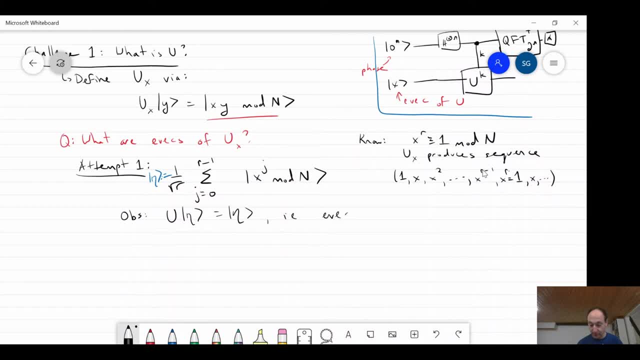 Okay, so it's- indeed it's- an eigenvector. Okay, so it's good in the sense that we know how to construct some eigenvectors, now at least one eigenvector. It's bad in the sense that you know. so now I have a u. 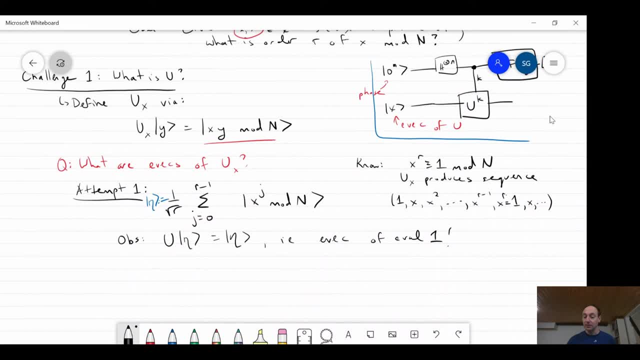 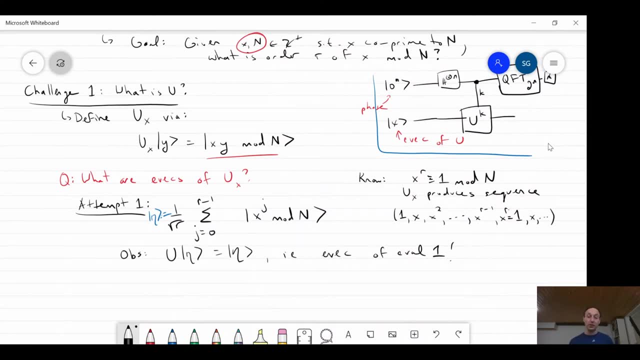 I have something I can plug in as an eigenvector into phase estimation. but ultimately what phase estimation does is? it gives me the corresponding phase of that eigenvector and that was supposed to encode the order of x. right And clearly you know, the constant 1 is independent of x. 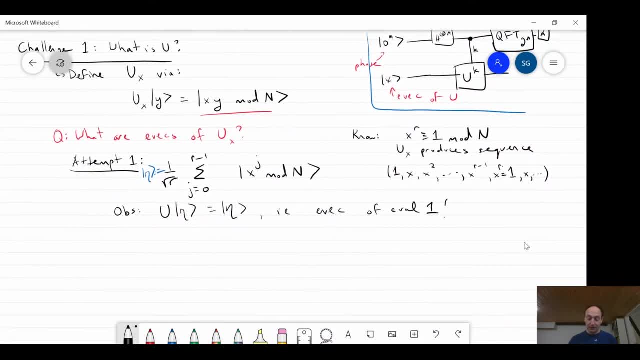 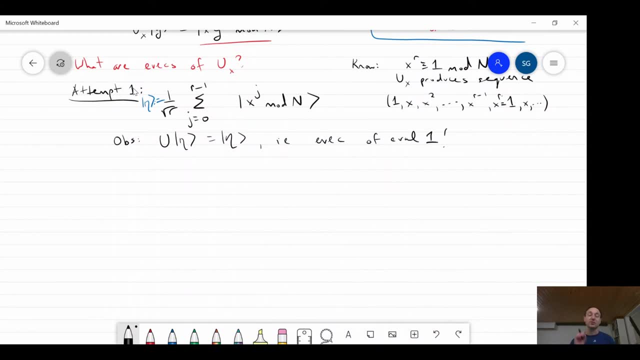 so it cannot encode the order of x. Okay, so that's attempt 1.. And so, even though 1 might not seem very exciting as an eigenvalue, it turns out we're actually very close to the right. We need to construct this eigenvector. 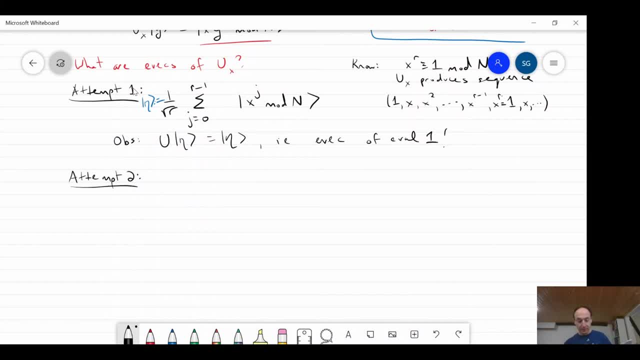 So let's go to attempt 2.. So what we're going to do is: you know we've used this wraparound property right That because the order of x is r. you know, if we keep increasing the power of x, 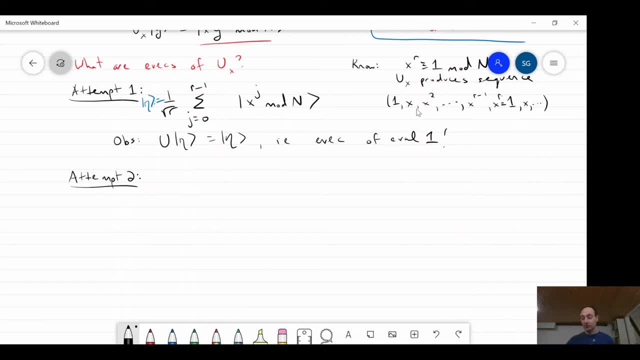 you know, eventually it wraps around and you know, this thing kind of goes over and over again. There's a little bit, there's one extra degree of freedom we have not harnessed here right, And that is, you know, the phase. 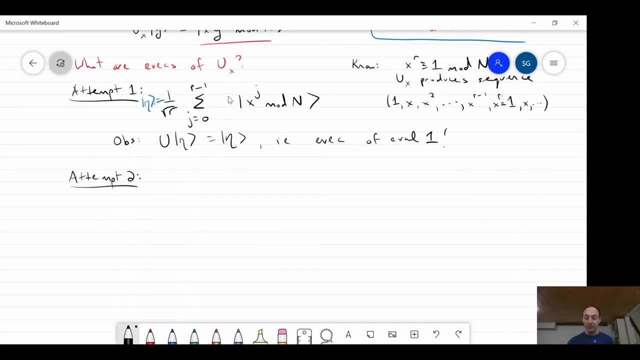 I haven't written a phase in here, right? So again we have the cyclic equation, Again we have the cyclic property for the kets And you know- luckily for us- you know when you talk about complex phases. 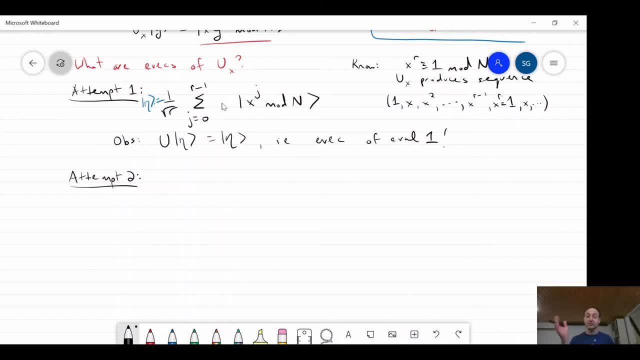 there's also a cyclic property, right? The cyclic property is, if you look at the roots of unity, right? I mean, if you go around the circle, eventually you wrap around and you keep going right, And so the natural thing to do if you want to embed a cyclic choice of phases here. 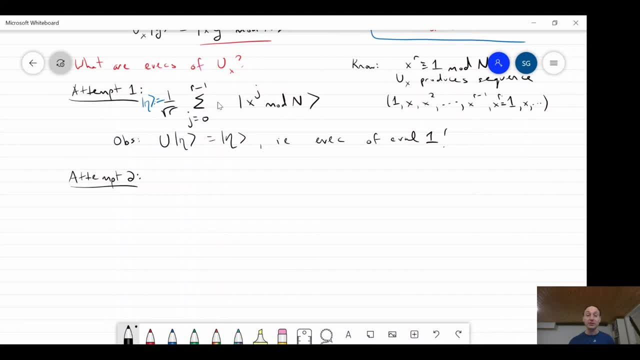 is you're just going to put down the rth roots of unity, basically. Okay. So recall, If we define the principal rth root of unity right From last lecture. So it's just this thing: e to the 2 pi, i over r right. 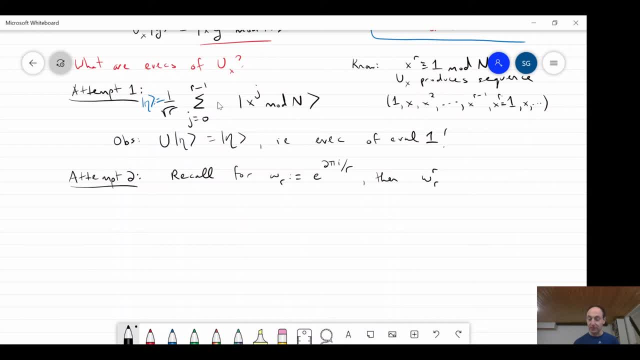 Then this thing wraps around right, If you raise it to a sufficiently high power, namely r, right, Then it just goes back to 1, right, You've gone all the way around the unit circle, And so now let's just do the same thing. 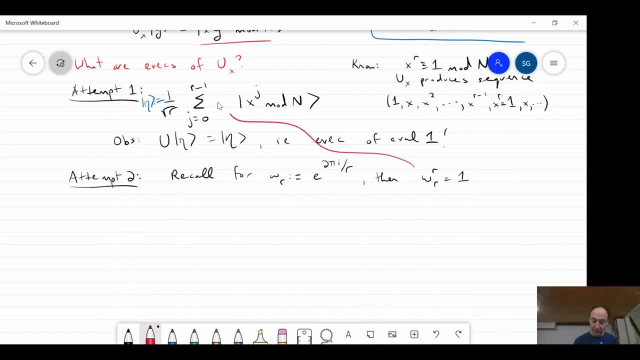 Let's just plug these guys right Into here. basically: Okay, So that when we go from j equals to j plus 1,. Okay, So that when we go from j equals to j plus 1, not only will the ket kind of get upgraded to the next member of the sequence, 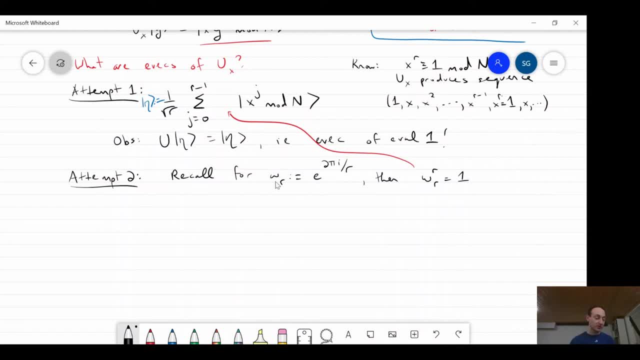 but now you know, omega r will get upgraded to the next power in its sequence. Okay, So then eventually, everything will wrap around. So let's be formal, Let's define this. So let's instead define 1 over root r, right? 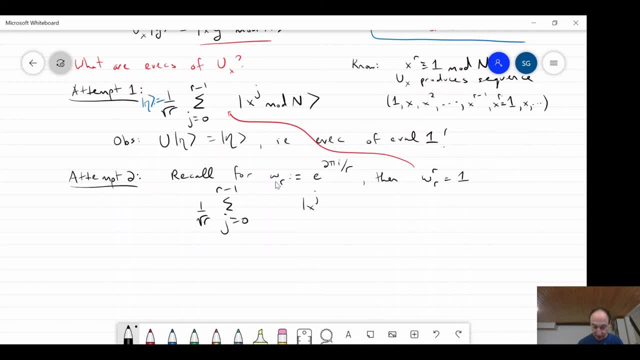 Sum over j equals to r minus 1 x to the j mod n. Okay, So that was just eta from before, But now what I'm going to do is I'm going to put in 1 to the 2 pi i j over r, right. 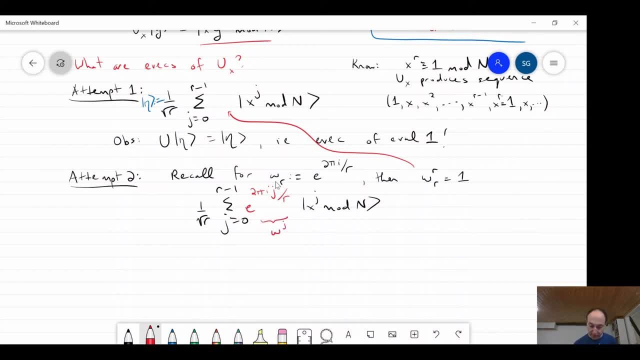 And so this is just omega to the j right. That's all it is Sorry. Omega r to the j right: Rth root of unity, Rth, principal root of unity, And let me give this a new name, right. 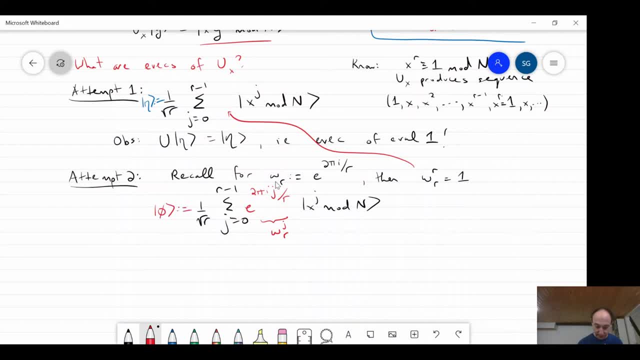 So this is now phi. Okay, And now. well, first of all, this is interesting because now, of course, this thing actually has something to do with r in terms of a phase And phases are. you know, we're a little bit closer to getting something out of a phase. 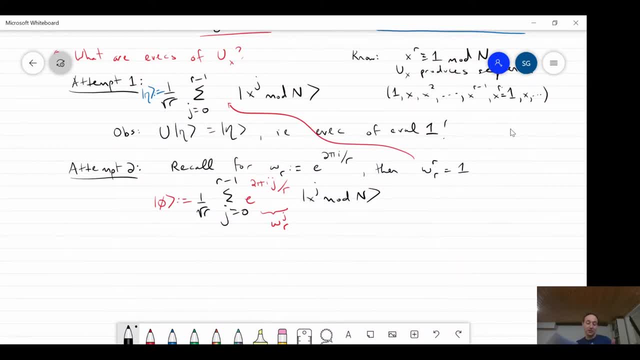 in terms of phase estimation. But, of course, what we need to do is we need to check that phi is, as written, is an eigenvector of u ux and that the corresponding phase of that eigenvector indeed contains. 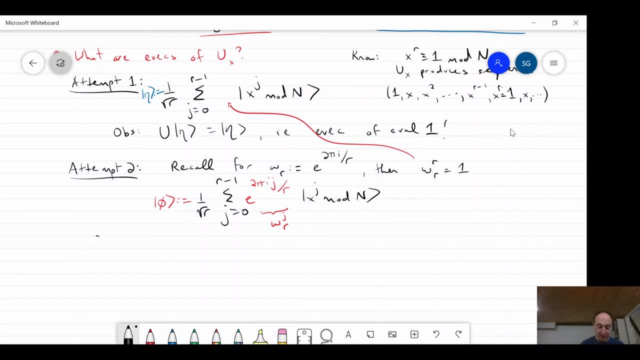 you know this little r the order. So this is exercise. I'm not going to do it, but it should be fairly straightforward. Exercise 30, which states that ux times phi, it's none other than, indeed, phi right. 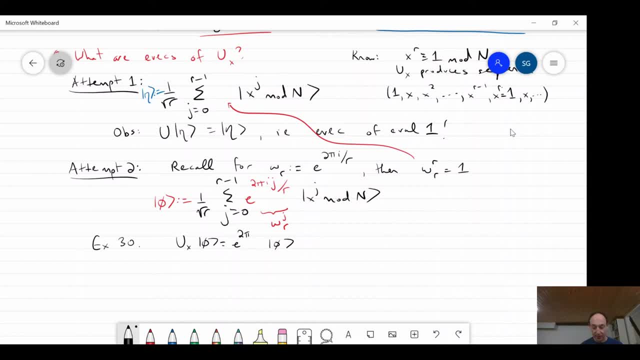 But it's going to be e to the 2 pi i and then over r. Okay, Yay, right, So there you go, So there's u, And so if I can only get my hands on this eigenvector phi. 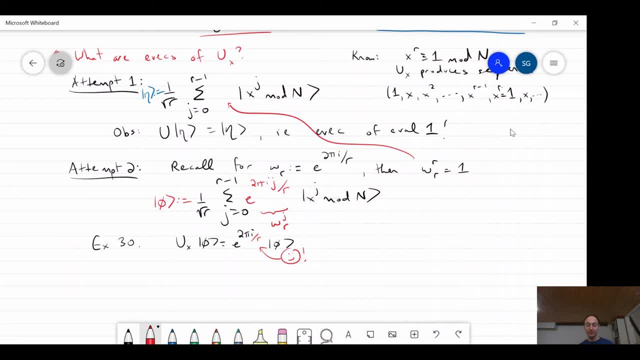 then you know I could run phase estimation in theory, And so therefore, quantum phase estimation on phi yields- remember, it's going to be an estimate. depending on how much precision I want an estimate for 1 over r, basically right. 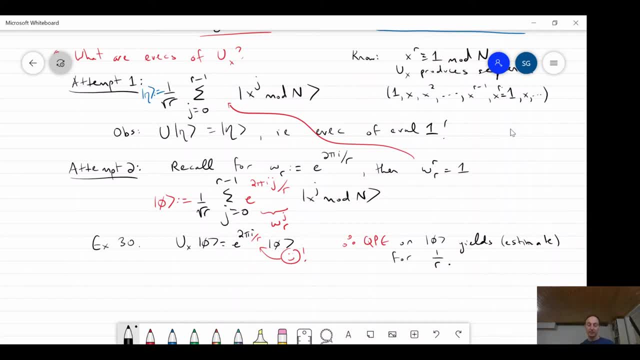 The phase is 1 over r, the way we had defined it, I believe. Okay, so that's great, right. In principle, it sounds like you know. life is going to be good. Okay, now there's only one problem. 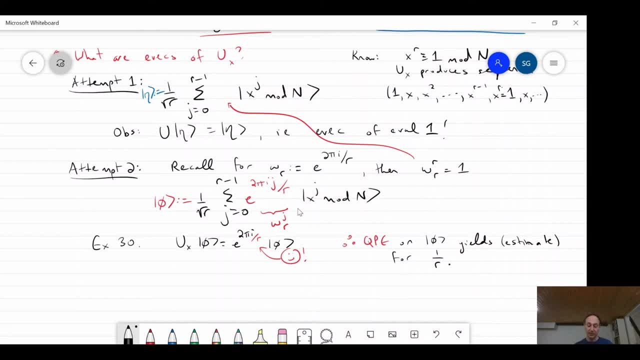 which is: you know, how in the world do I prepare phi or phi right? This thing over here, How do I prepare this vector right? Because sure, if I knew r, then I could prepare this superposition with these faces. 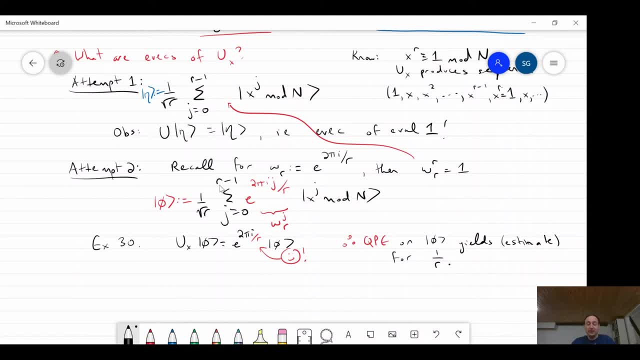 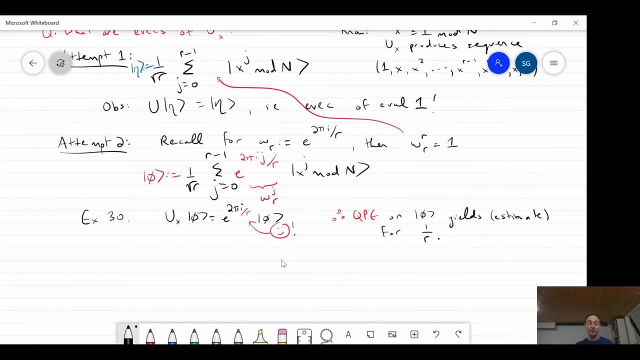 But I don't know r. right, I'm looking for r. So what do you mean? There's a chicken and the egg problem here, right, And so, indeed, it turns out that it's not clear. So, even though we've solved this problem of you know, 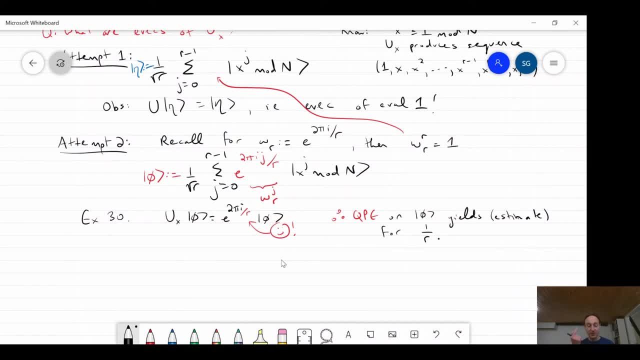 what unitary do we apply it on? and that it has like a good eigenvector, if you will. it's not clear how to prepare that good eigenvector, And that's challenge two right, Which is how to prepare phi. 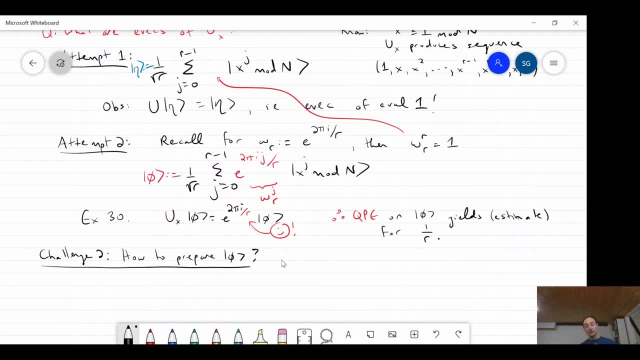 Okay. Now the short answer is: we don't okay. Okay, more accurately, you know we don't know how to, and so we have to find a way around this, right, Okay, And Intuitively, I mean. so let me first sketch the idea. 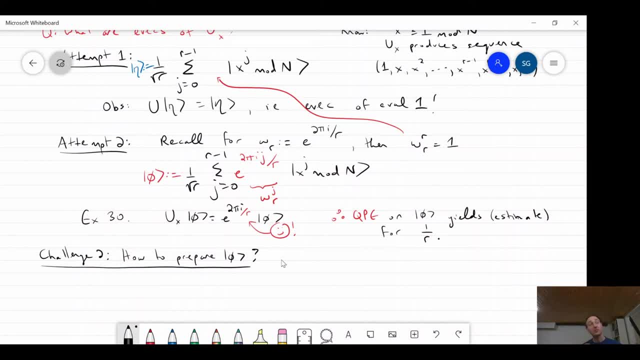 The point is that, very roughly, what we'll instead do is we'll prepare another state which is easy to prepare and which has a quote-unquote nice overlap with phi right, So that when you run phase estimation on this other state, 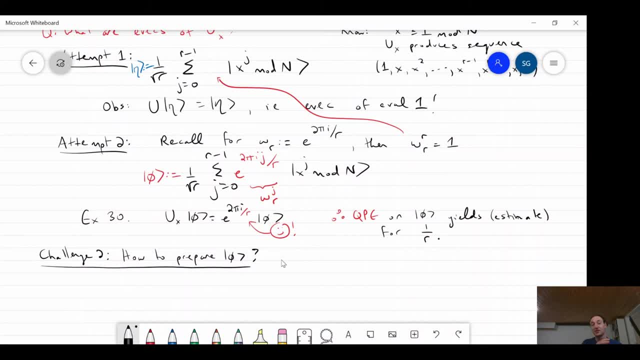 which is easy to prepare. you know, some kind of fraction of it is going to actually simulate running phase estimation on the real state we desire phi. So let me be a little bit more formal. So the answer is: we don't, at least not directly. 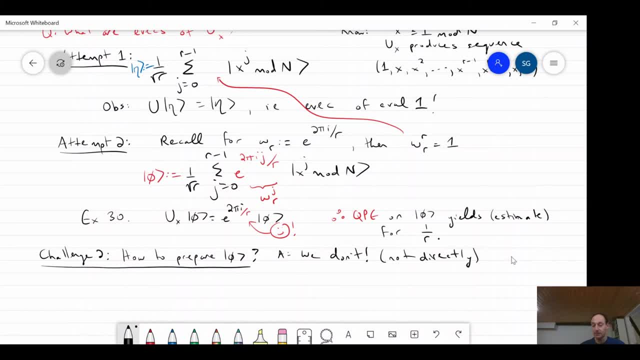 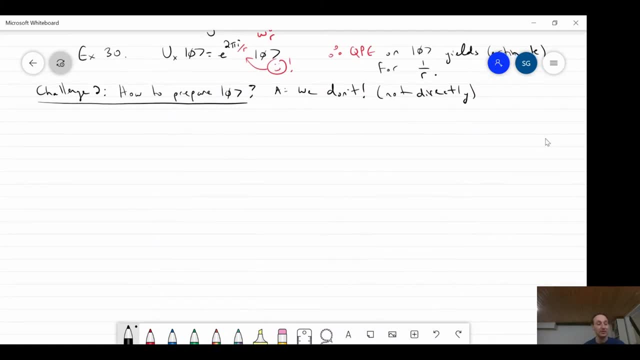 Okay, We don't know how to do that, And maybe you can even prove that it's equivalent to solving for R. You know, I haven't really thought about it, but it might be a nice exercise. Okay, So what we do is, you know, let's just extend phi. 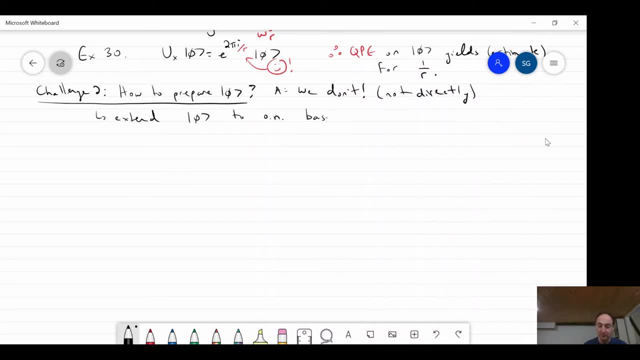 to an orthonormal basis. Let's just call it b. Okay, So it's just going to be some set of states, And this is for the space ux acts on Right, So ux is unitary, So whatever Hilbert space it's acting on. 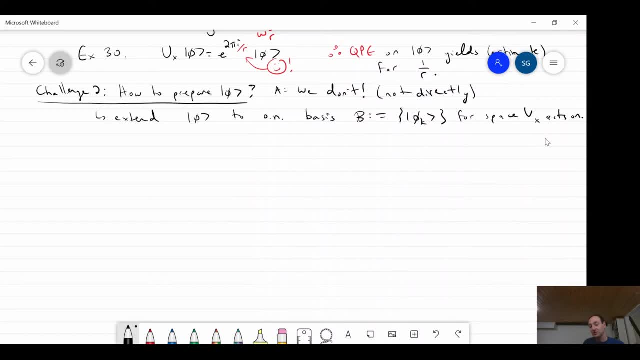 whatever number of qubits. let's just take phi as an eigenvector in that space. So we'll let that be the first phi1.. I'll just define as what we were originally calling phi. Okay, So that's this guy. 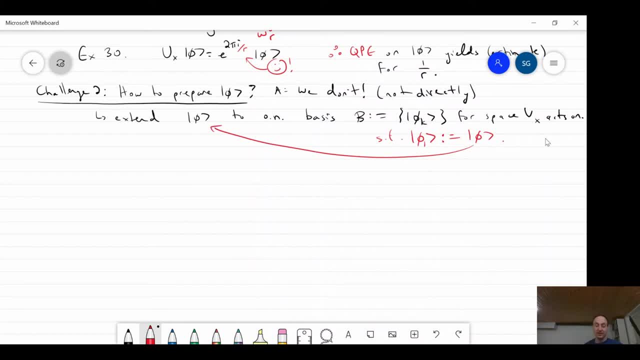 So I'll let that be the first element of the basis and everybody else, I'll just extend it to a basis for the full space. Okay, And of course, sorry for the space, and let me give a name for the space. 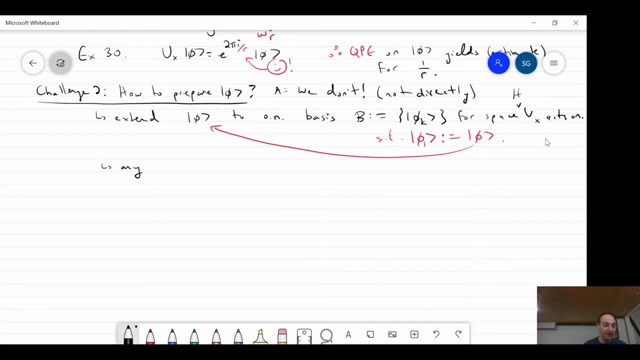 let's just call the space h, So any vector psi in that space, of course, can be decomposed in terms of this basis, Right? So written psi equals sum over k, alpha k for some coefficients that sum in square to 1 of phi k. 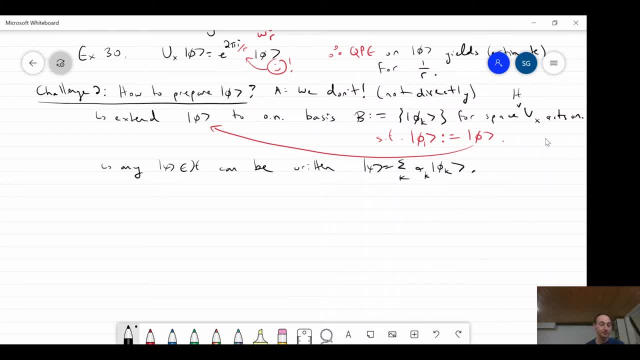 Okay, Sum over k of alpha k squared is 1.. Okay, And now therefore, since phase estimation is just a unitary operator, in particular, this means it's linear. This means that if I plug into phase estimation- right. 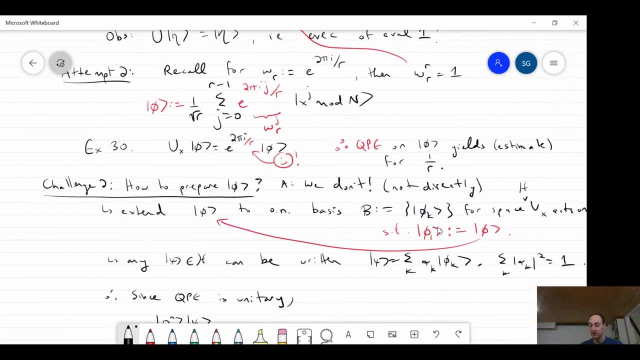 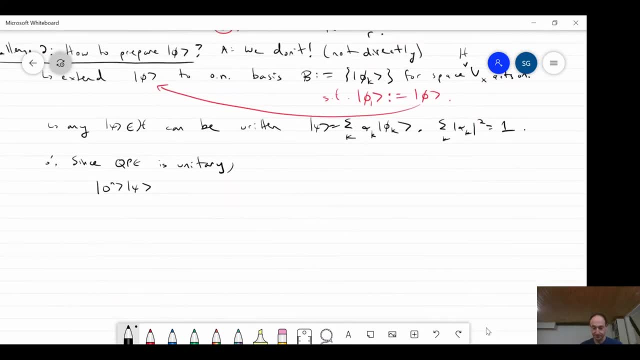 In phase estimation. I'm going to plug in. there are two registers right. They were zero to the n and my eigenvector, or it doesn't have to be an eigenvector, right? It's the point of what I'm showing you. 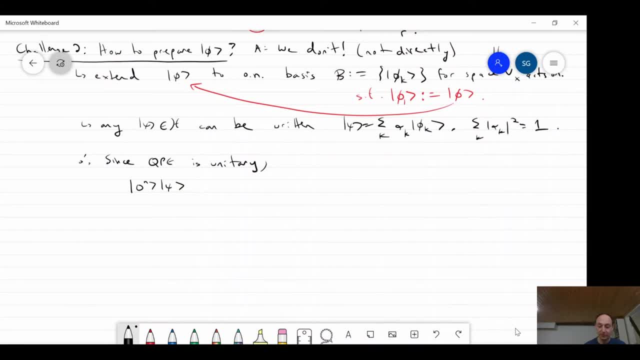 Okay, So I plug these two things into phase estimation. This can just be rewritten, as we just did, in terms of this basis we defined. So sum over k, alpha k. I'll stick that there, And then here I have your phi k. 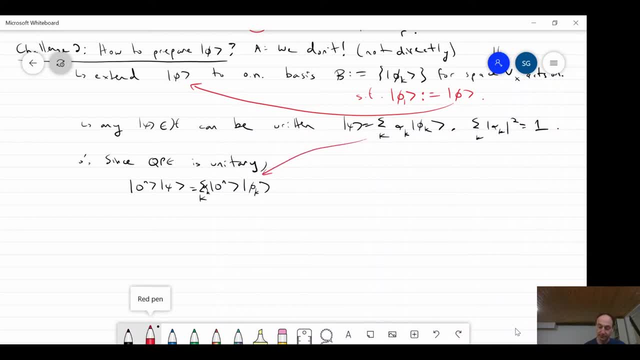 Right. So that was just this. And now, if I apply quantum phase estimation, what it's going to do is it's just going to do things. it acts linearly, right? It's just a linear operator, So it acts independently on each of. 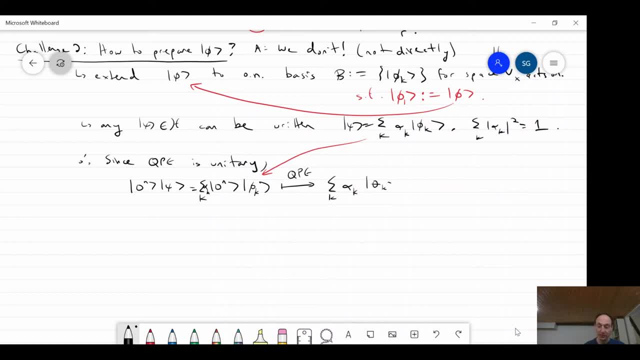 sorry, that should be a phase on each of the terms in the superposition. Okay, So this thing is theta k is an approximation to phase for phi k. Okay, So you know whatever eigenvector you happen to have in the superposition. 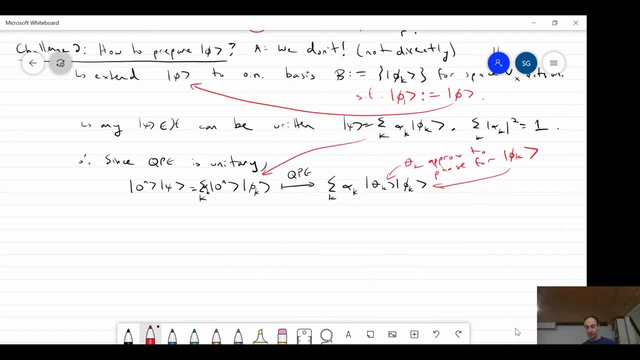 the phase of that will get put next to it. Okay, And so kind of intuitively, you know, if you were to just measure the first phase register now, then you know, with probability, absolute value of alpha squared, you'd see the phase corresponding to. you know, phi 1,. 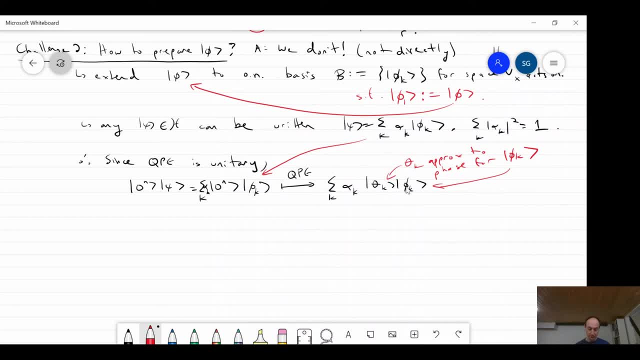 the one we actually wanted, right, Okay, And now? so the question is: you know, what should psi be right? Can I come up with a psi? Or, in particular, you know, can I pick a good choice of basis right? 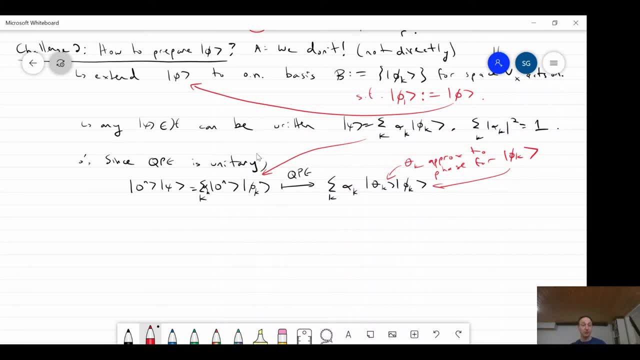 So that you know, so that I think we just, yeah, if we just take an equal superposition over these basis elements, so if I choose this basis here cleverly and I take an equal superposition over the first r terms of that basis, 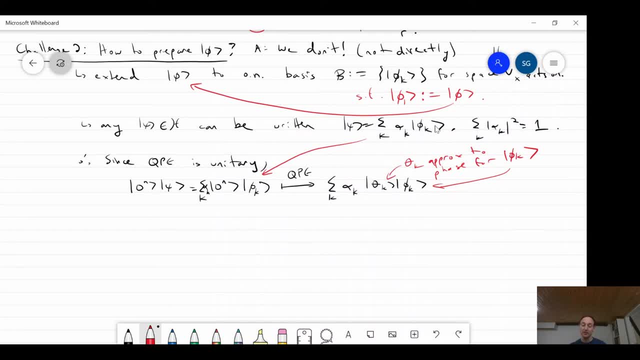 where the first term is, of course, the real phi we want. can I make it so that you know the psi you get? the full sum of all of them is something nice, that's easy to prepare And the idea is as follows: right, 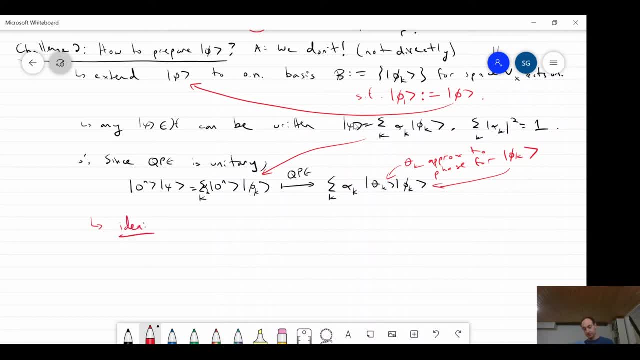 I'm going to present it slightly backwards to the way it's written in the notes. So let's just think for a second. You know, I have some state phi 1, which I know exactly what it is. you know, assuming I know r. 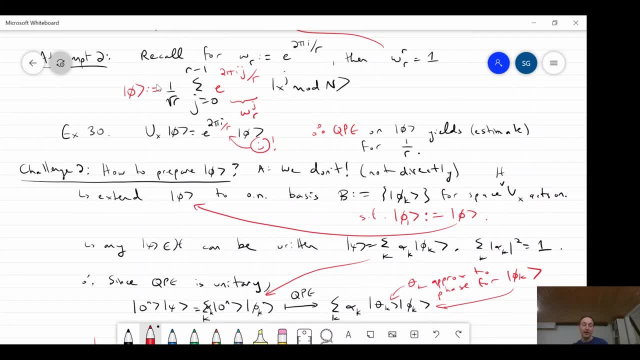 I mean, if I knew r, then phi 1 was just this state right. And now what I want to do is I want to construct r minus 1 vectors orthogonal to this one right. I want to fill out that basis. 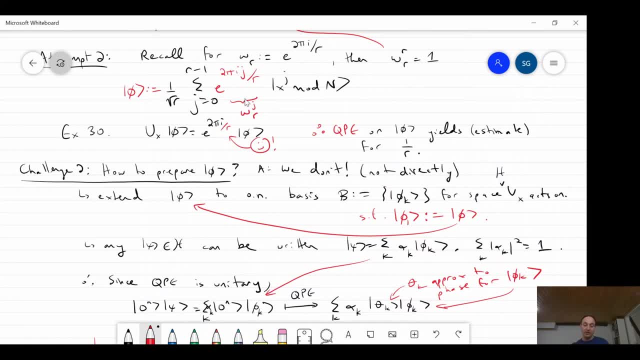 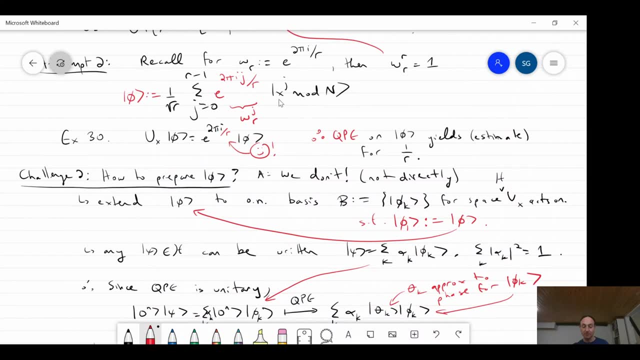 So how am I going to do this right? So here I want you to think back again to the Fourier transform lecture And in particular, I want you to notice that essentially, you know up to relabeling of these basis vectors. 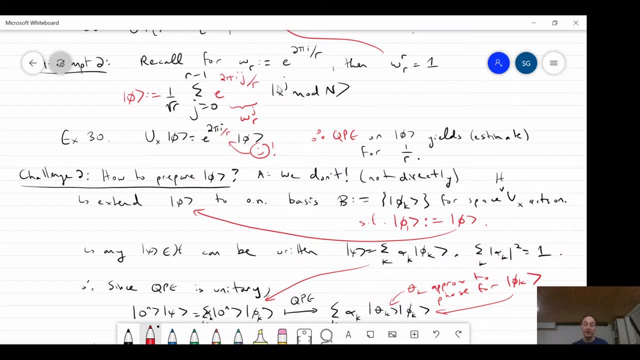 now they're labeled x to the j mod n, but instead I could have just relabeled them j. This is nothing other than one of the columns of a Vandermonde matrix. right, It's basically. you take the principal root of unity. 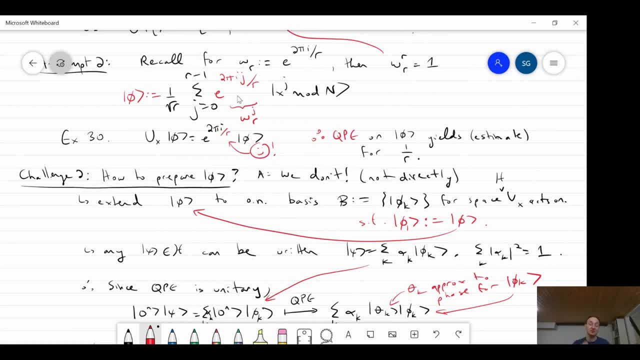 and then you basically raise it to higher and higher powers. right, This is exactly what we did in Vandermonde matrices. And remember that you know the way we came up with the Fourier transform was we took, you know, that principal root of unity. 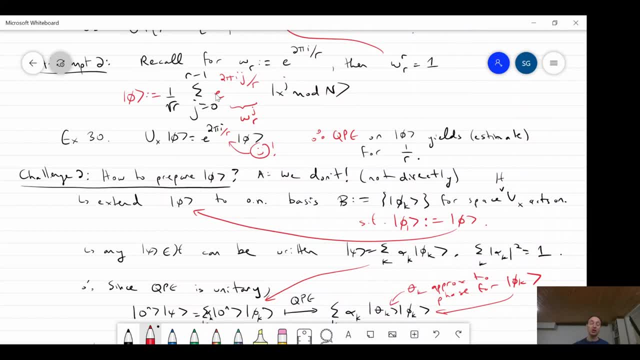 and then we raised it to higher and higher powers. to start each column, okay. And then, with each column, you raise each of the roots of unity to higher and higher powers, And in doing so, we came up with a set of columns which were all orthonormal. 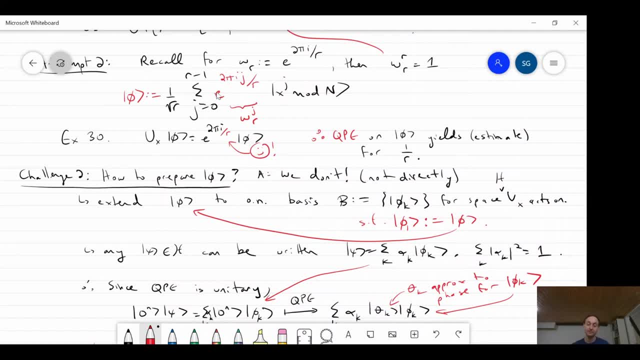 They were unit vectors orthogonal, and they gave us the Fourier transform. So we're just going to steal a page from that playbook, We're going to think of this as representing one column of a Vandermonde matrix, And so then, 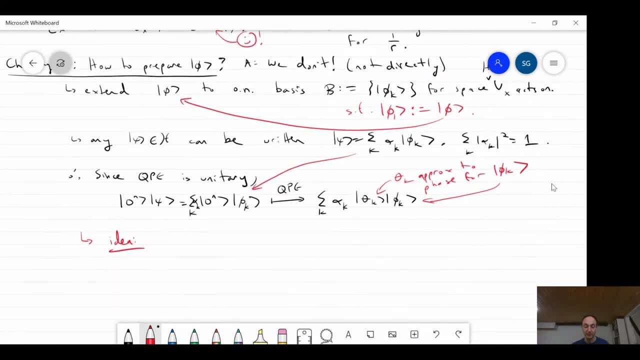 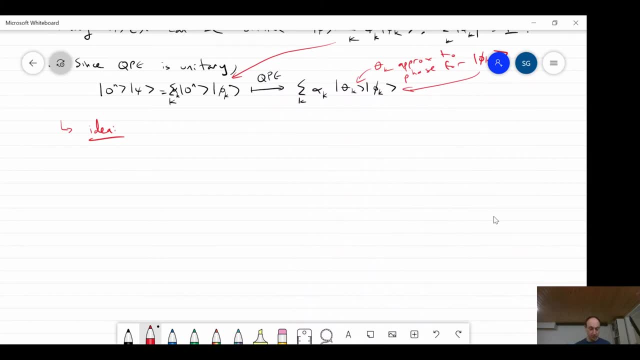 we know exactly what the other columns would look like just by following the pattern of a Vandermonde matrix. Okay so, let me be a bit more formal now. Okay so, observe that phi1, which, remember, was just equal to phi. 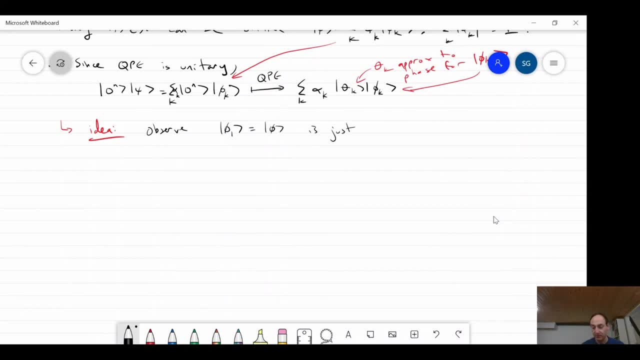 is just. I mean it's approximately this up to relabeling of the cats. It's basically going to be a column of a Vandermonde matrix Right, or a row if you like. So it basically looks like this. It's like a. 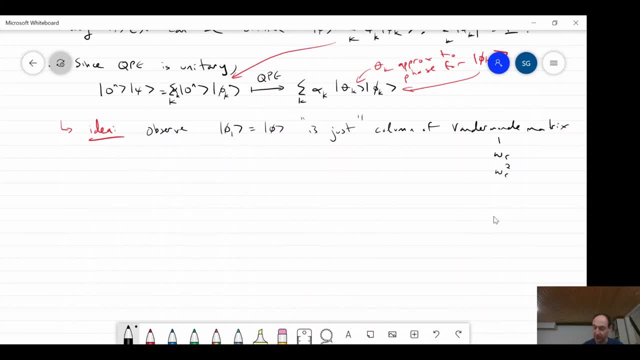 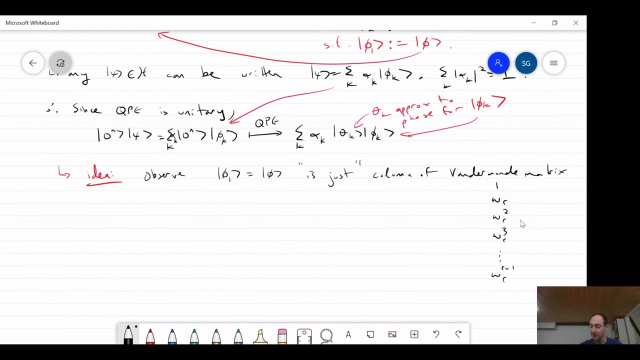 1. omega r, omega r, squared omega r, cubed, dot dot dot. omega r to the r minus 1, right. If you look at phi, these are the phases you see showing up Right, And we already know how to. 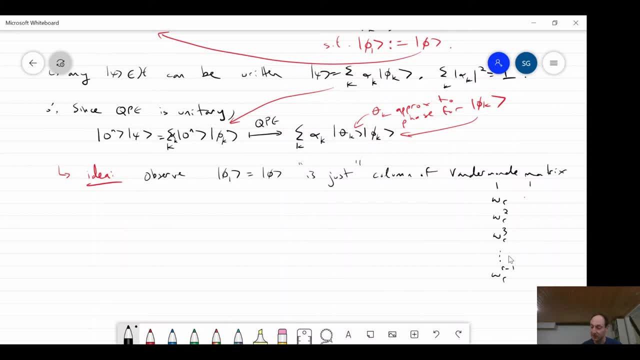 come up with vectors orthogonal to this right. The next column in the Vandermonde matrix looked like this: You would start with the square of that principal root and then you'd square the square Right Squared Square cubed. 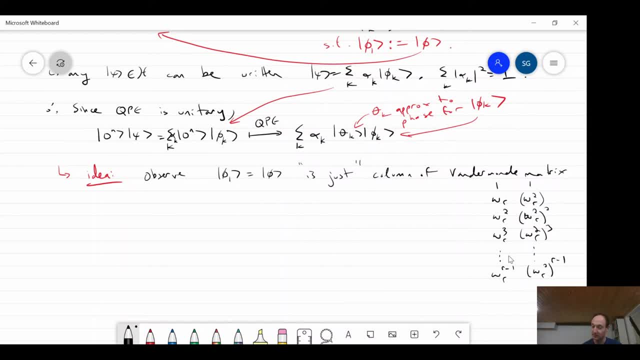 So forth, right r minus 1.. And so if we take phi and replace the phases in it, these guys, with these ones, then you'd get an orthonormal vector. That's what Vandermonde matrices taught us. Okay, and so. 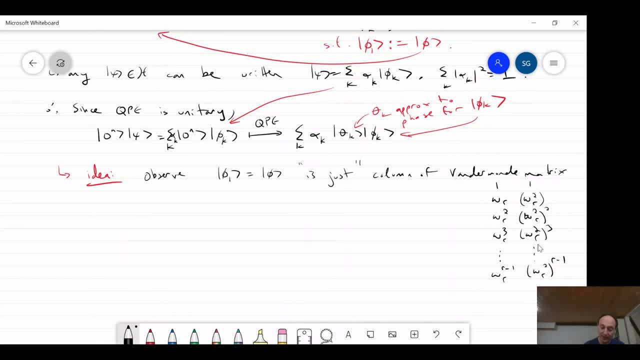 we're going to do the exact same trick. now I'm going to define phi k more generally in my basis for k going from 1 up to r, I guess, or 0,, 0 up to r minus 1, is going to be essentially the same thing. 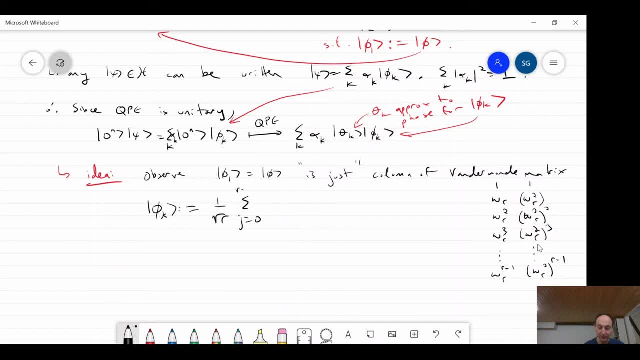 as what we had before. So the black things I'll write will the black ink will denote the what we had before, right, And the new part I'll write in red. So this we had before we had over r right. 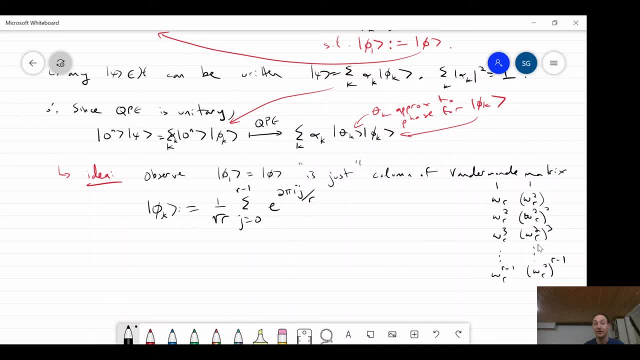 So this was the principal root, because it's 1 over r, which we raised to higher powers j, And again we had x to the j mod n right. So that was just phi 1 right now, And what I'm going to do is: 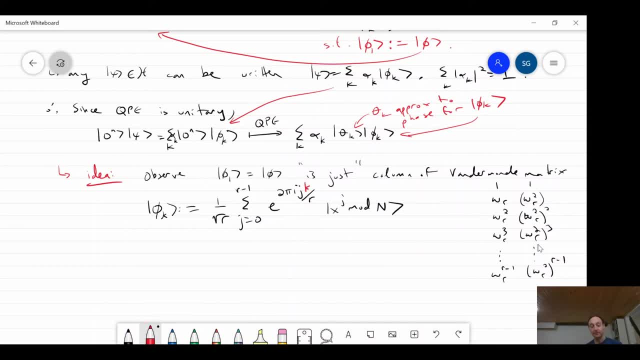 I'm just going to add this k here. Okay, So you can think of this as none other than omega r. k, right All to the power j. Okay, So you're in column number k and you're in row j. 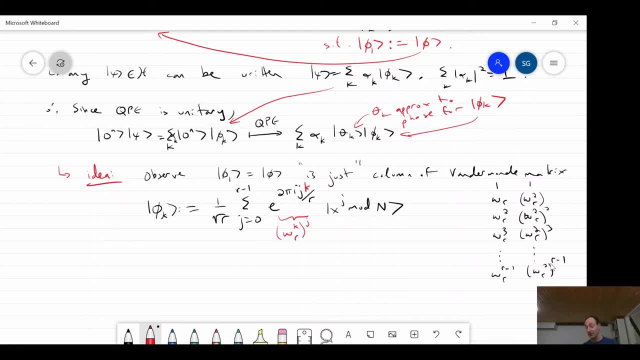 the way I wrote it here. Okay, So it's just like a Vandermonde matrix. Those things are beautiful, right? So this is really why I wanted to take the time to talk about them last lecture. Good, So this means that we get. 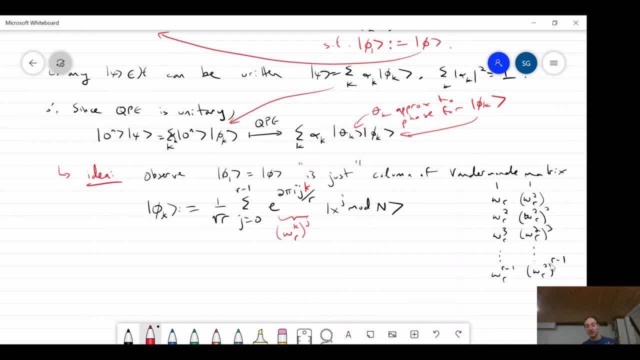 we can construct r whatever r is right, Orthonormal basis vector, starting with the vector we want, phi 1.. And now something magical happens. So, by the way, I'm not going to prove that these things are orthonormal. 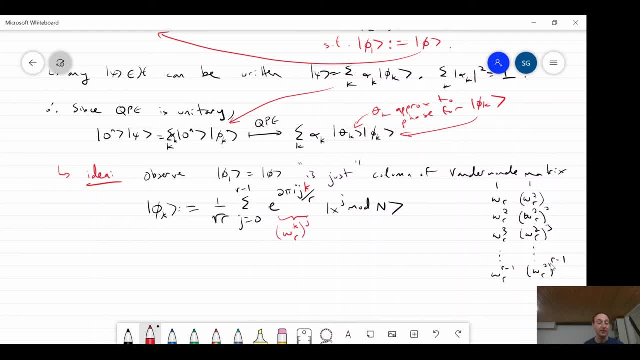 I mean you get it more or less for free, if you believe the Vandermonde stuff we did last class. But consequences Number one. now, if I apply u to the kth, such basis vector I created, right, What phase do I get? 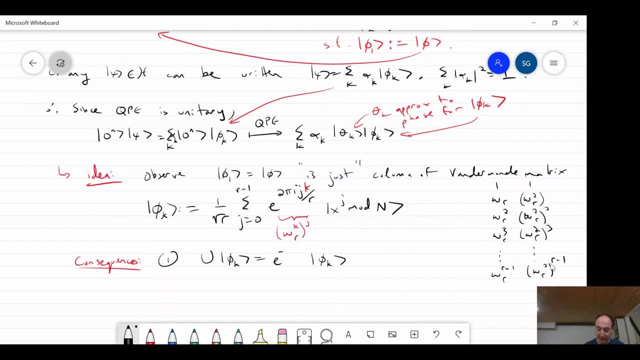 Okay, so it is going to be an eigenvector, And what you're going to get is e to the 2 pi i. So again you'll have over r, just like before. But what's new now is you have this funny k here. 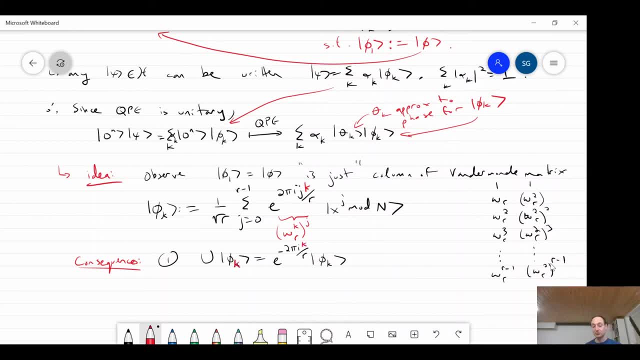 right, This is the same k. Depending on which basis vectors you chose, you're going to have k in your numerator now. Okay, and I'll come back to this in a second Kind of the more interesting thing now before we get. 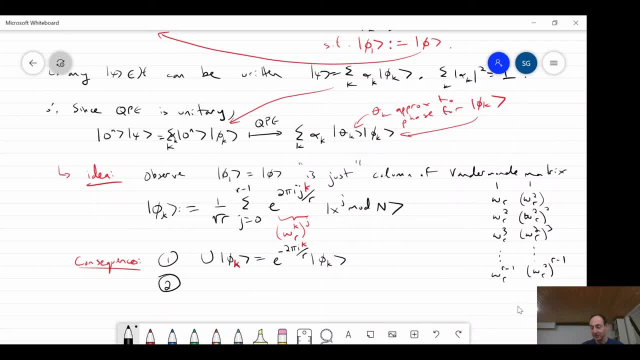 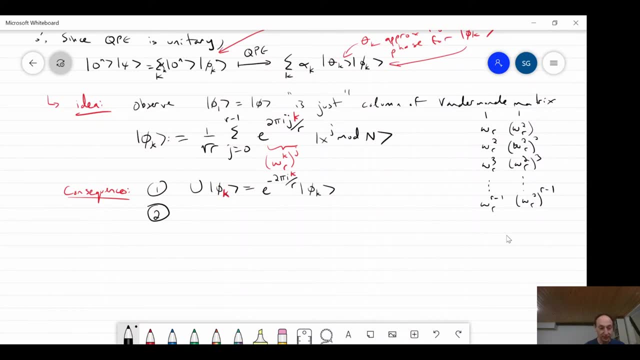 I mean, that's interesting too. but slightly more relevant at this moment is that, magically, if I take phi, k and I just sum them all up with equal weights r minus 1, and I have to of course normalize that. 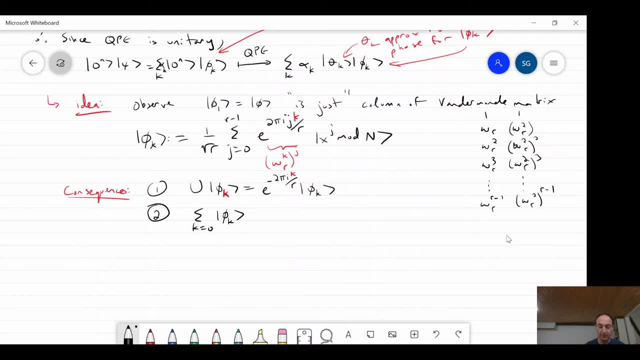 So if I take phi k and I just sum them all up with equal weights r minus 1, and I have to of course normalize them because they're all orthonormal- what state is the sum? It is nothing other. 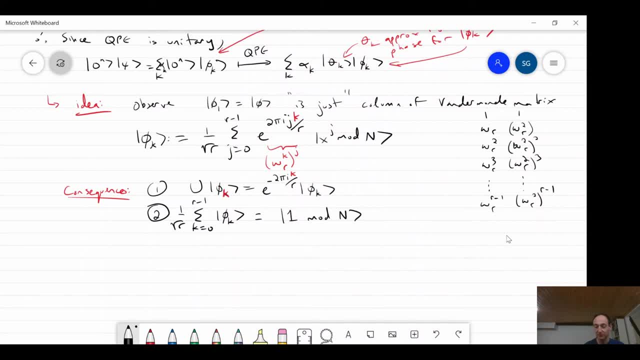 than essentially the binary encoding of the number 1, mod n. Okay, This is trivial to prepare, right? I mean the state encoding 1 is easy, right? So, magically, I don't know how to prepare phi 1,. 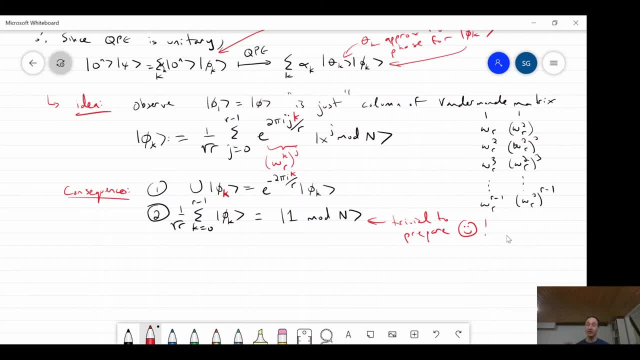 phi, 2, or any of them, right, But if I can prepare 1,, which is trivial, you could also think of that as just being a superposition of all those states uniformly Okay. So magic, right, Black magic. 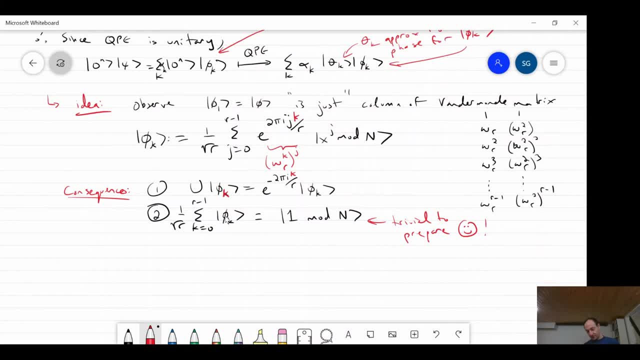 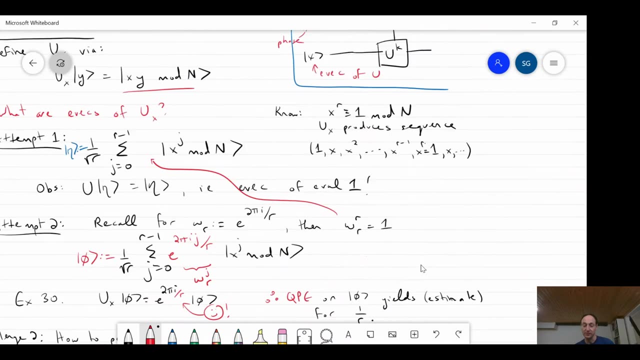 right, Good, Okay. So now, if I combine these two, if I take both of these guys together, what does it tell me, Right? Well, it tells me: if I prepare, when I run phase estimation- right, What am I going to do? 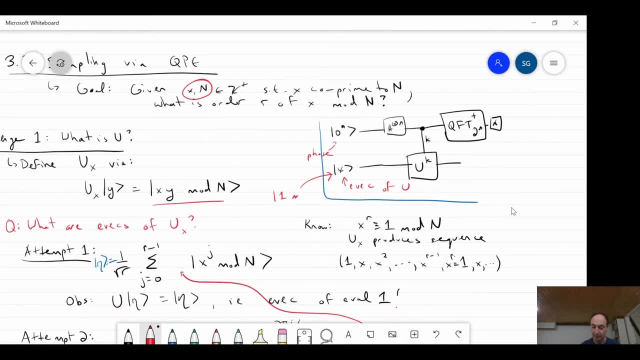 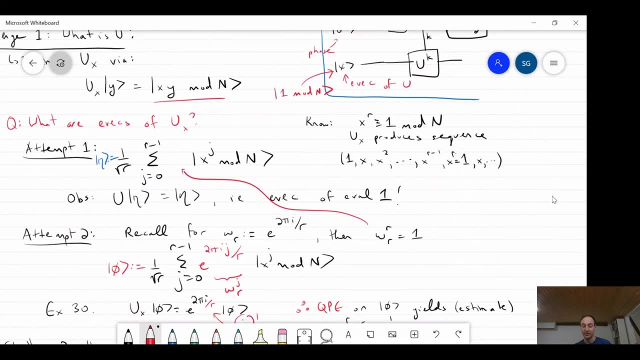 If over here you know, I plug in 1 mod n right And then I run phase estimation. This thing is a superposition of those r basis vectors I constructed And then I measure right. So I prepare 1 mod n. 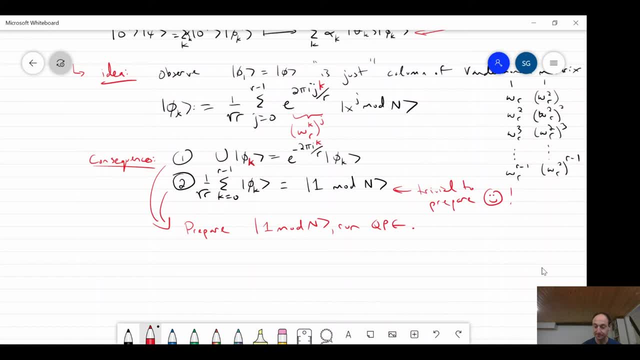 and I run quantum phase estimation right, And so this was my state, psi that I was trying to construct. That was this nice state, And is that so measuring the first register in the QPE diagram yields? so now I have. 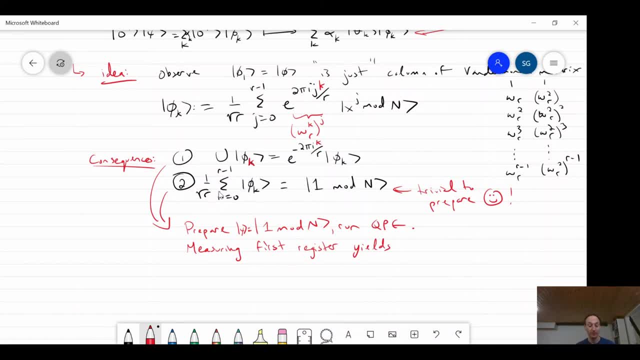 a superposition right. This state is not one state, it's k states right, And they're all equally weighted. So with probability 1 over r, it's going to be uniform. So with probability 1 over r. 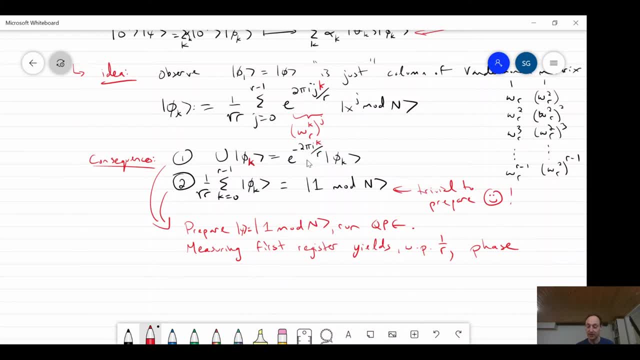 it's going to be the phase corresponding to the kth eigenvector, phi k. So you're going to get the phase corresponding to the kth eigenvector, which would be k, over and again. I'll do this in black. 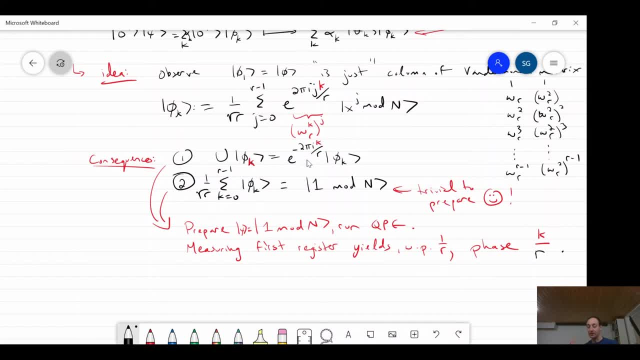 just so you know it's the old version. Okay, So the k is the part that's new. So measuring the first register uniformly at random gives me k over r for sum, for clarity, right. So this means that what we can do, 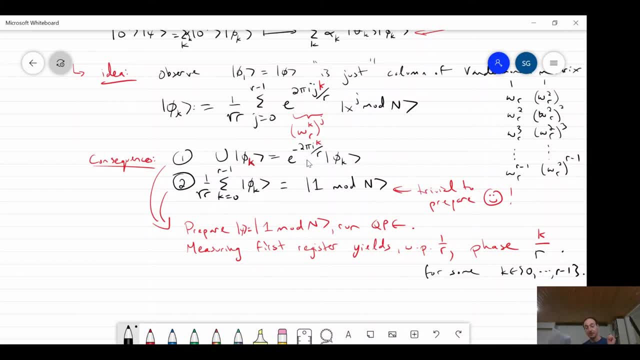 efficiently given the quantum phase estimation algorithm is we can do this well, I still can't figure out r necessarily right. If you give me 1 over r, then of course I could invert it to get r right. But 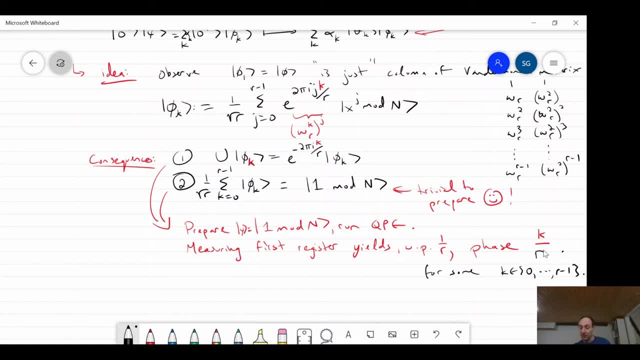 you're not giving me r right. You're giving me k over r for some random k, okay. So what have we learned? We've learned that we can sample uniformly at random from the set. I gave it a name s equals to. 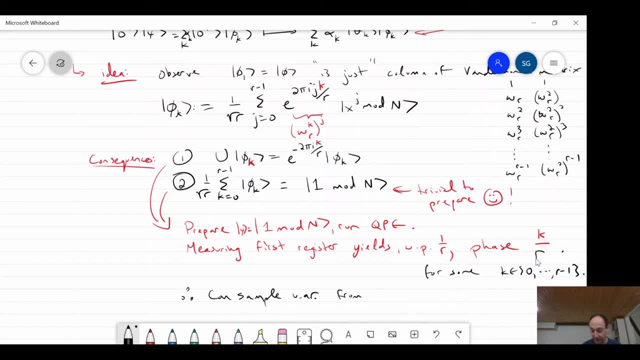 1 over r. 2 over r up to r minus 1. I guess this will be a 1 here r minus 1. I guess this will be a 1. here s equals to 1 over r, 2 over r up to r minus 1. 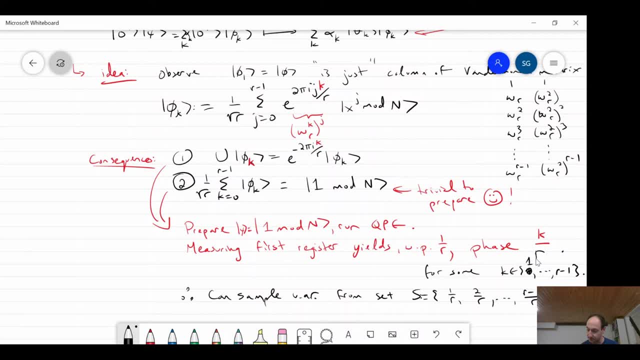 r minus 1 over r, okay. So every time I run phase estimation I measure. basically I get one of these phases uniformly at random, okay, And obviously if I get 1 over r I'm happy. I just invert it. but you know. 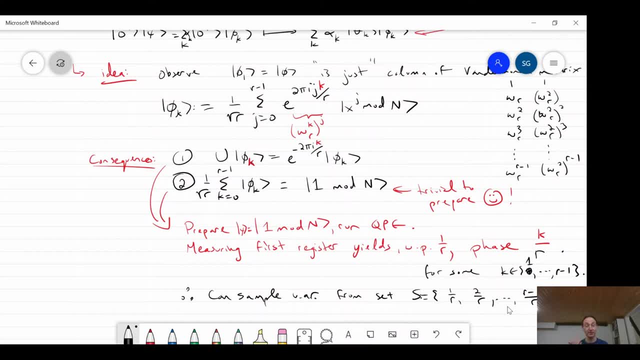 r could be very big. right r in principle can be as large. you know, the set is very, very large. it might take me a very, very long time until I sample to see this 1 over r okay, but nevertheless I can do this sort of sampling. 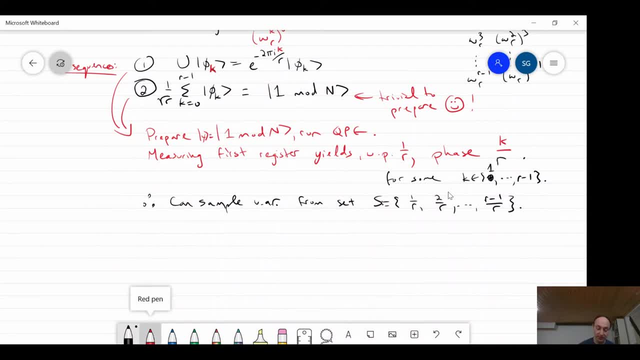 and the question is: you know, given a random sample from the set, can we recover r Okay? so that's the question: given a random sample from s, can we recover r? Okay? and the answer is yes. again, more magic by something called. 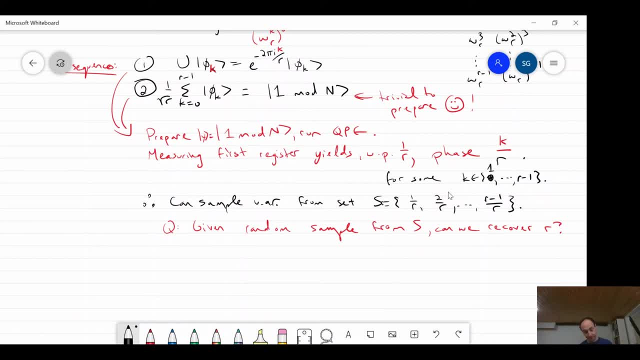 the continued fractions algorithm, so we're going to get to that in a second, okay, but before that there's one more thing we have to deal with, which is the third challenge in using phase estimation, right, And the question is now a matter of precision. so how many bits of precision? 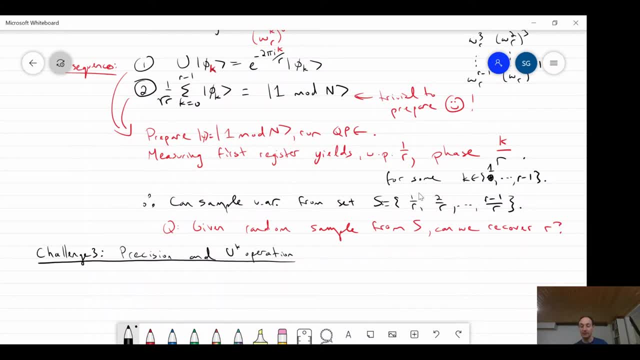 do we need Right. so you know, my phase estimation algorithm will give me an estimate of, you know, k over r, randomly sampled right Right up here, but of course it's not going to be perfect. right k over r might not even have. 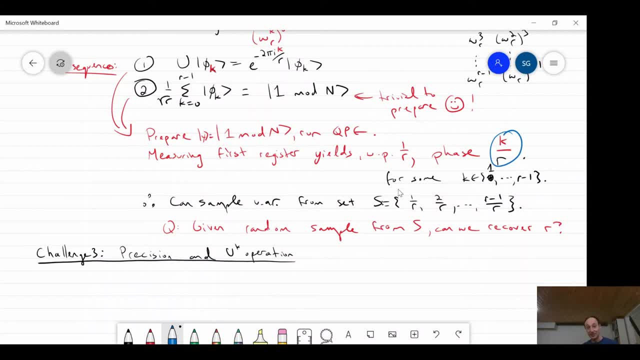 a finite expansion right. So you know, I'm only able to approximate this to within some number of bits of. precision of bits is, let's say that number of bits is n. I then need to be able to implement u to the power 2. 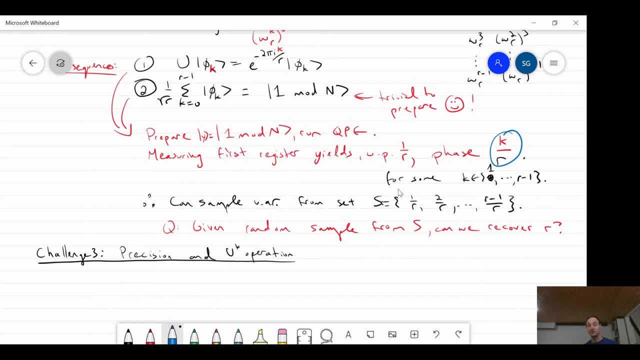 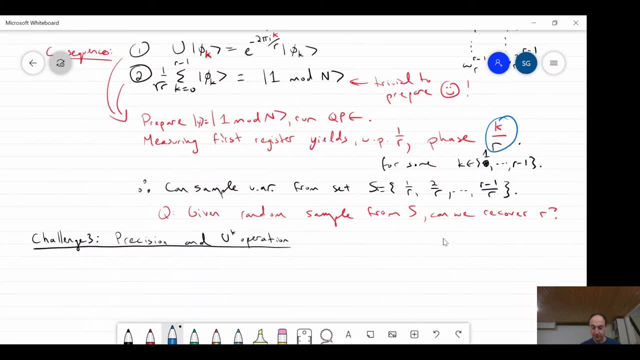 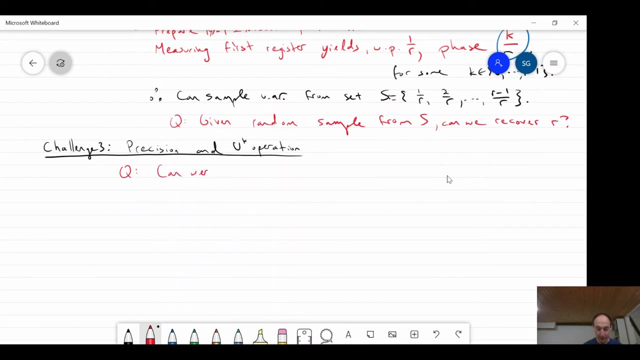 to the power n. okay, So I need to be able to do that efficiently, okay, okay, so you know. question: can we, can we whoops, efficiently run qpe to the precision required to recover r from? and you know this is now going to be an approximate. 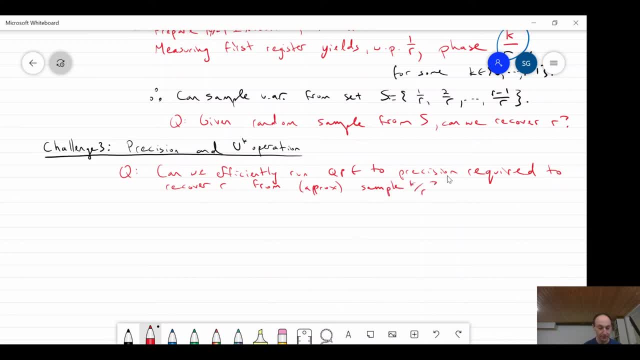 sample k over r. okay, Okay, and so to answer this question, right um. so let's just recall that the input to factor was this um the composite number n. technically, we also had a threshold, but let's just forget about that for a second. 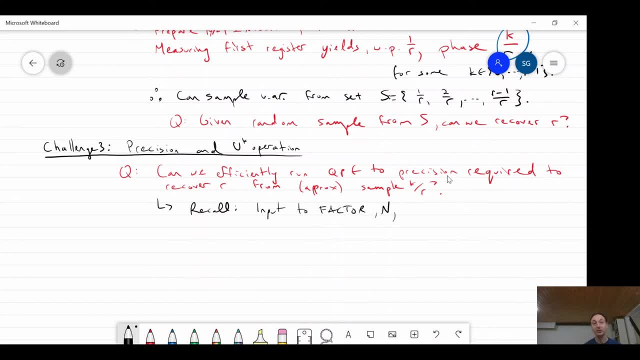 so input to factor, which is just the integer n. its input size is encoded via um. and now I'll define little n to be the number of qubits or bits. sorry, very precise, uh, log base, two ceiling plus one. okay, so that's the number of bits. 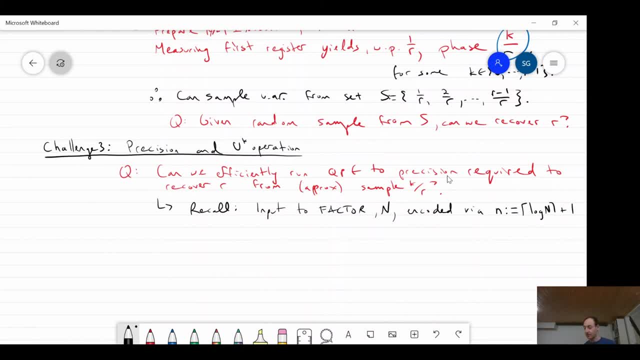 you need to encode it. so basically, log n is the point. okay, so everything I talk about will be in terms of little n, because this is your input parameter, right? this is the, the size you need to run in time polynomial in little n to be efficient. 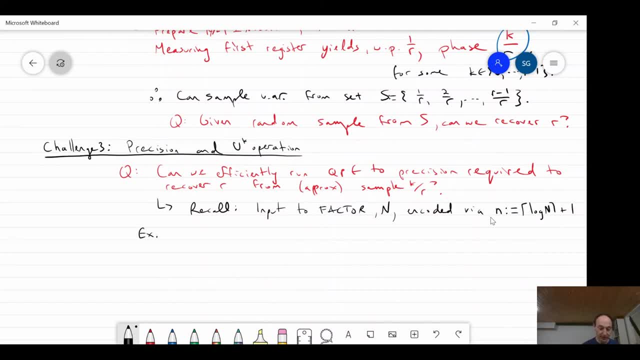 okay, and now just a cute exercise, right? so suppose, just to get a sense of what we're up against, right? suppose I have um two positive integers, k and r. let's just say k is smaller than r, and these are both representable exactly in just n bits. 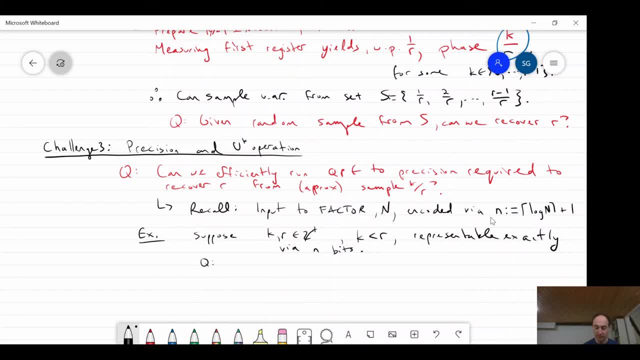 okay, and so the question is: how many bits to express now the ratio? okay, and by bits I mean, you know, I want a decimal expansion like b1, b2, right? I don't mean some other succinct encoding, right? and so okay, because we know um that basically. 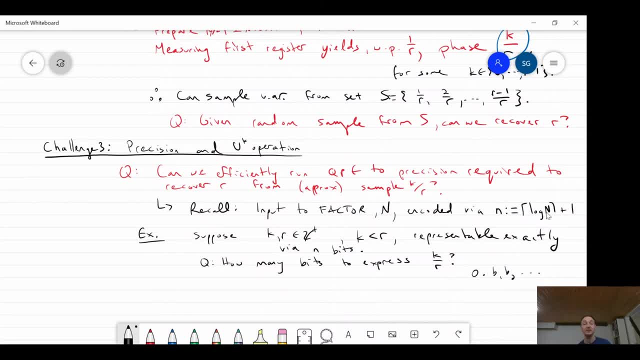 for example r, little r requires only little n bits because it's at most capital n in size. so I have a bound on how big k and r are going to be. so can I bound how big k over r will be? and the answer is not necessarily. 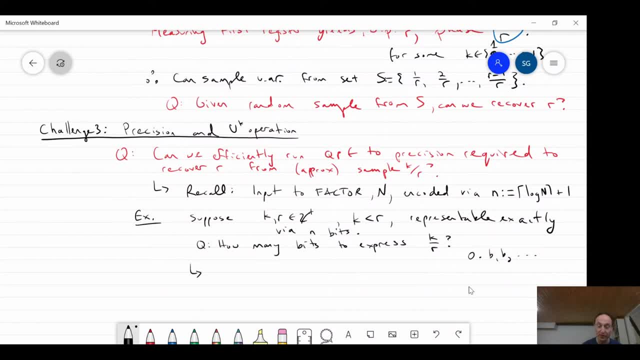 right, let's do a very quick counter example. so, if you want, you can take a moment to pause the video and think about a counter example to this claim that, in fact, in general, this expansion might be infinite even though k and r could be represented using a finite number of bits. 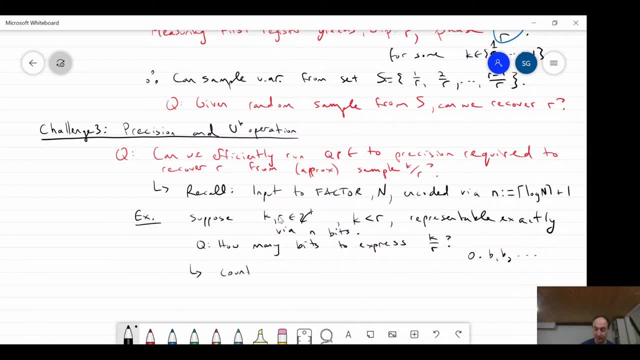 so here's an example, counter example, that suggests there is no bound in general, which is: you know, if k equals to 1 and r equals to 3, right, both of those can be represented using two bits and the ratio is one third, which is has an infinite expansion. 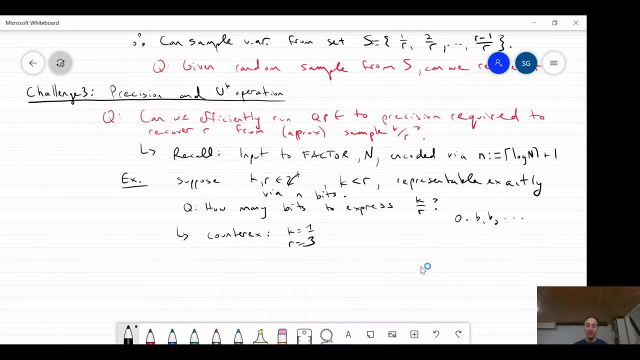 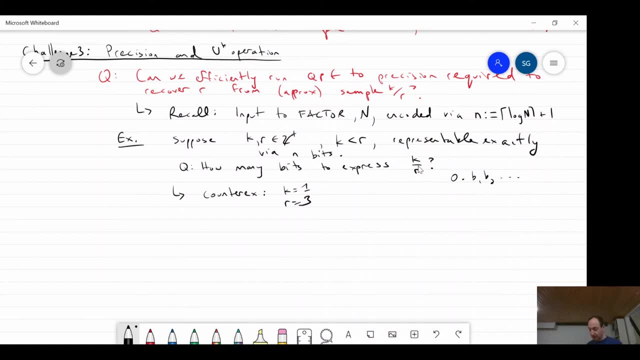 right, so just as a very simple counter example. so the point of this is that, even though I know bounds on the length of k and r, I don't necessarily know bounds on k over r. okay, so let's try and get a bit of the exact number of bits. 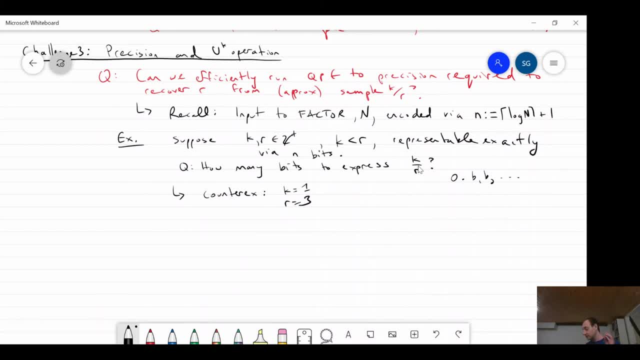 of precision we'll need for k over r will turn out, you know, to come from a theorem later when we talk about continued fractions, but we'll be blatantly stupid and making wild conjectures. okay, okay, so. so the answer is that no a priori bound right. 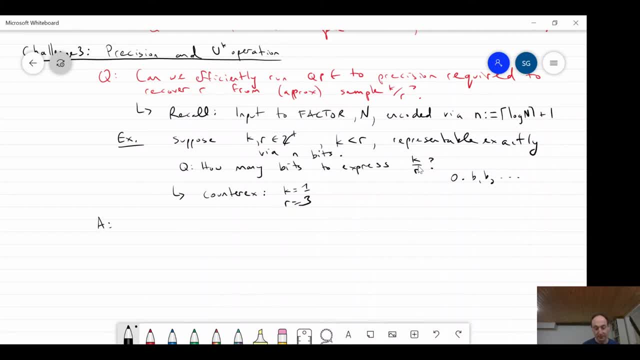 in general it could be unbounded, okay, but let's try and get a bit of intuition right. if k and r are n bits each right, then k and r are n bits each right, and k and r are n bits each right. and then I mean, if you 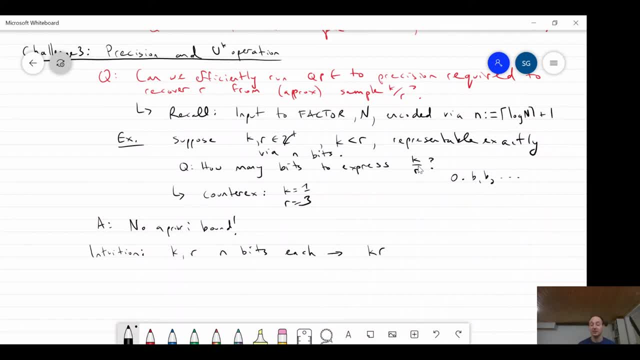 stare at this long enough you'll see that you'll realize that you know k times. r is a number is another integer requires you know something like two n plus one bits to write down right. basically, the number of bits is going to double. okay, so you might somehow expect. 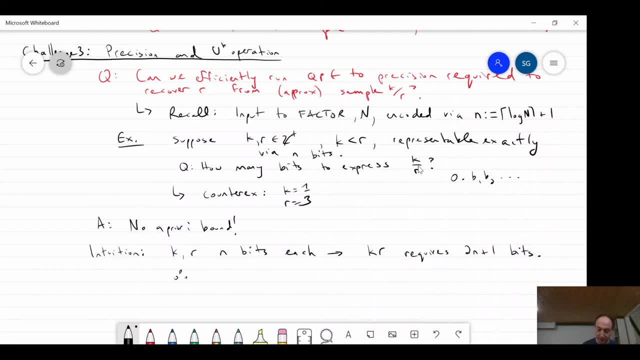 you know waving hands again here. I'm not saying this is rigorous, that therefore you know in big red, maybe question mark right k over r can be. you know the character of it if you will in some sense, or the- that's not a formal term- in the setting. 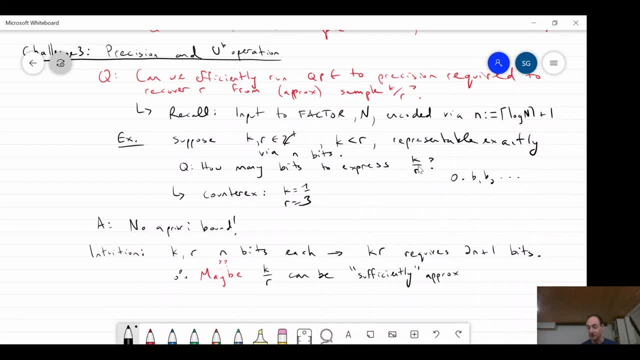 maybe k over r can be sufficiently approximated, at least for the purposes of recovering r, with two n plus one bits. okay, so, since the product requires that much. so maybe we can take this same number of bits as an estimate for k over r instead. okay, because k over r. 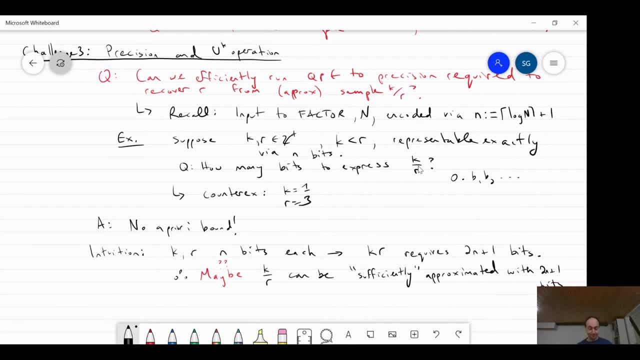 is also technically a product- k and the reciprocal of r. again, this is just trying to give you some intuition, and it will turn out that, indeed, two n plus one bits will suffice, if we can estimate, you know, k over r to two n plus one bits using quantum phase estimation. 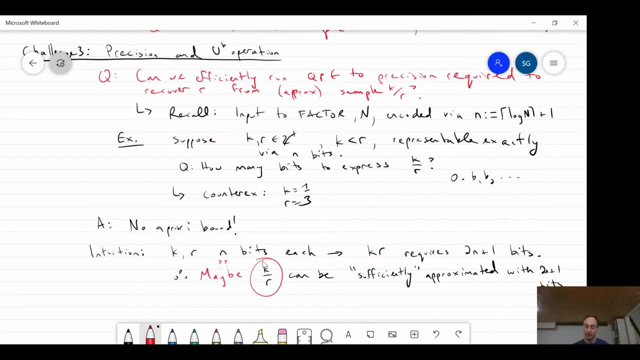 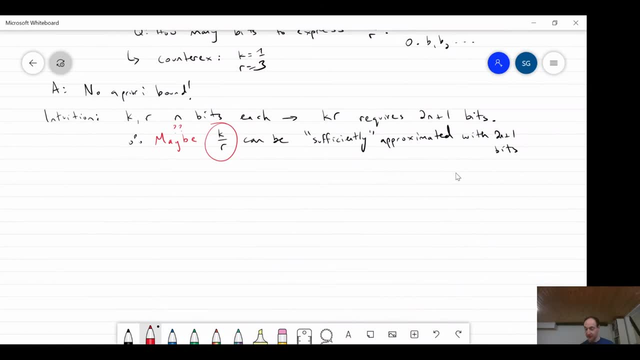 then continuing fractions will work. okay, we will be able to recover r. okay. so again, we'll get to continuing fractions in a second. so let's see so later, two n plus one bits will suffice, okay, good, now, fine, so we want to. so, therefore, we want to. 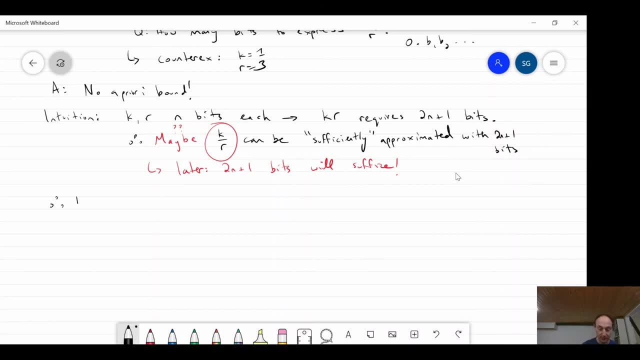 run q quantum phase estimation to two n plus one bits of precision, right? so in that first register, in phase estimation, where the phase is the number of bits there you know should be two. number of qubits is two n plus one. okay, and, and we want success, 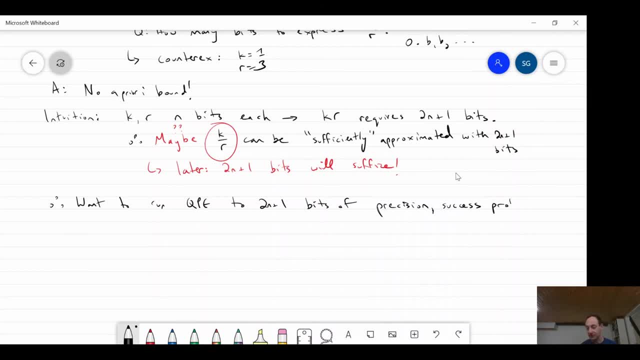 remember, qp is not perfect, so it had some success, probably, which we are allowed to play with. so let's say we want probability of success, at least one minus epsilon. so what did we have to do? we had to do two things right. the first register of qpe. 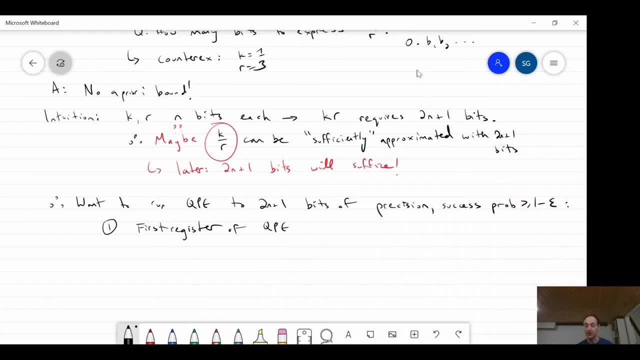 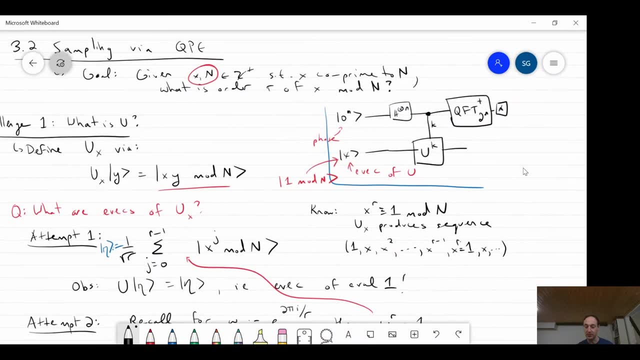 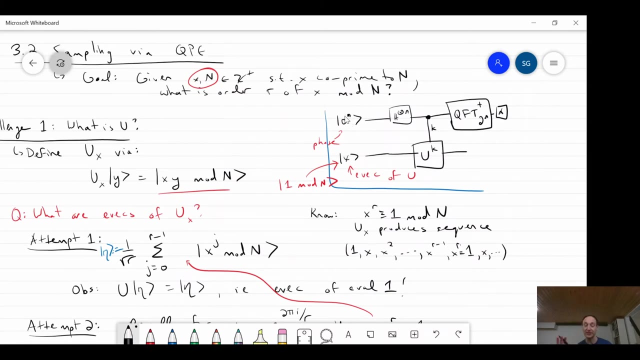 instead of setting it to be precisely two n plus one bits. so i mean, let's just, rather than me frantically waving my hands, let me just show you this diagram again. right, so you know, the phase is going to have to be the probability of success. so how much? 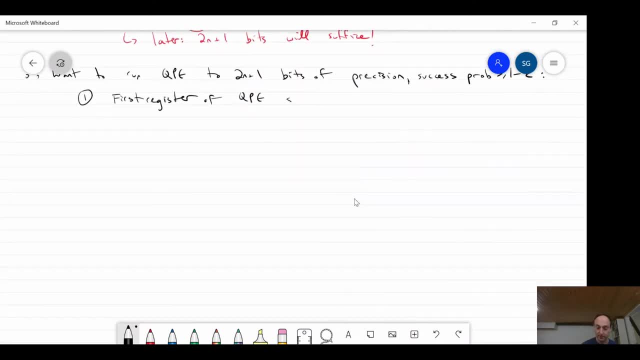 bigger. did we have to grow it? the analysis from last lecture said that we needed to set it to n prime being. you know that's the size of the register. this is what we wanted: two n plus one plus a small overhead, basically, so something plus, you know. 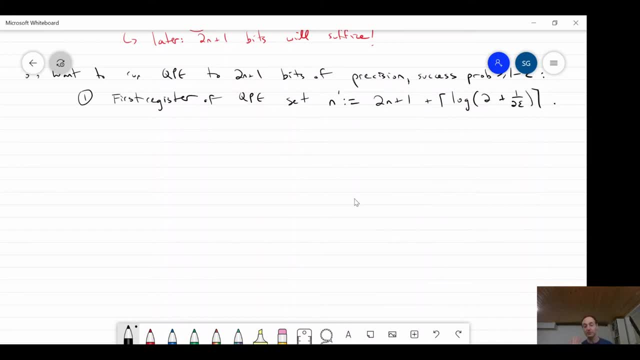 the ceiling of. so this is going to be the number of qubits in the first register of phase estimation. you know that alone is not a huge problem. we just grow the register a little bit. okay, now the more annoying part is that if i want to set 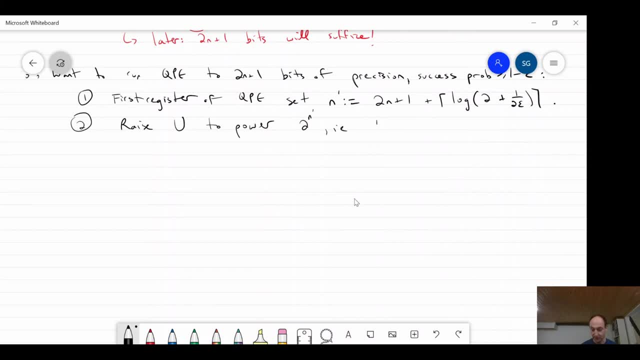 n prime to that. so i need to be able to run u to the 2 to the n prime, which is of course, just in. 2 to the n prime is, of course, order. 2 to the n. like this thing is huge, right, okay, so that's. 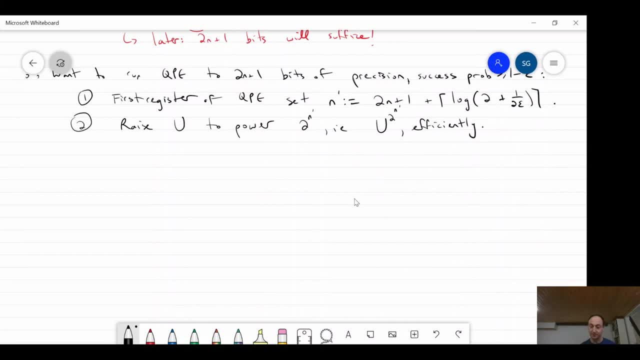 exponential, of course, in our encoding size, right, and so how are we going to do this? equivalently, what we are saying is that we want to be able to compute. what did u do? it, just, you know, did x times y, mod n right, but if i raise u, 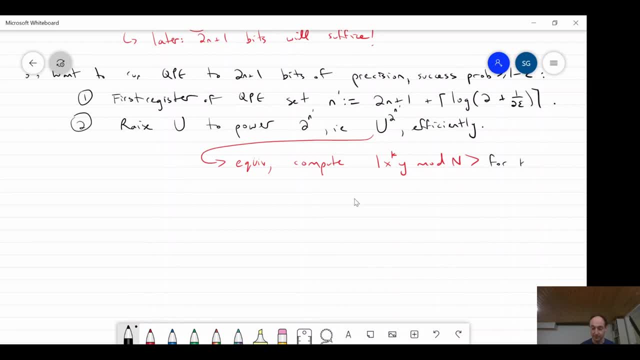 to a very high power, whatever that power is. it's just the same thing, as you know, multiplying by x k times n. and what we need to do is, of course, we need to do it in time. poly n- right, that's the input size, not 2. 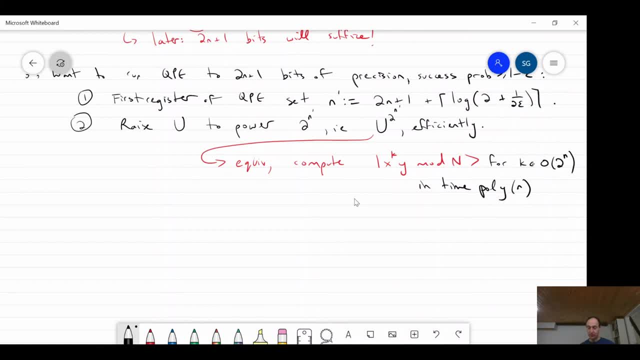 to the n. okay, so a priori, it seems like you're in a bit of trouble. you know you want to exponentiate x to this. okay, so there is an algorithm that will do exactly this right, which is that if i have an x- well, not exactly. 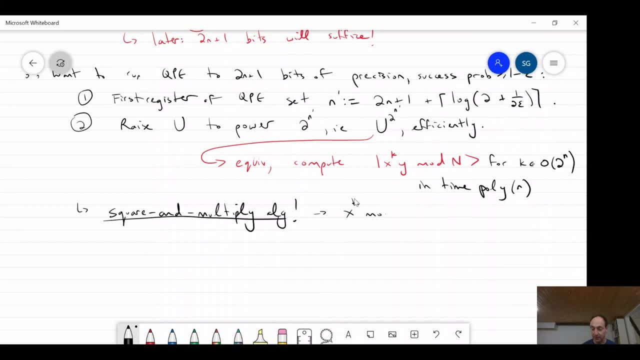 this slightly off. basically it will. um allows us to compute x to the k mod. whatever you want, let's just say n. well, let me give it another name, just to be clear. that has nothing to do with n in this particular equation. so it can do this. 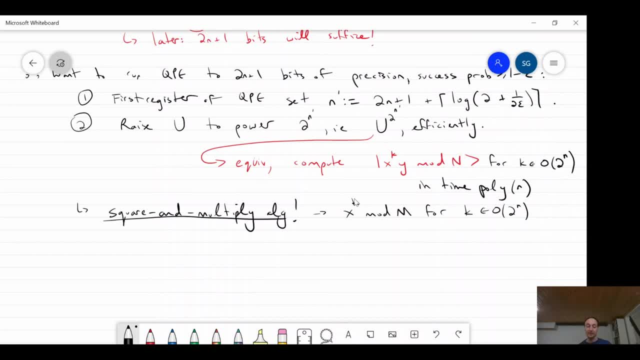 exponentiation efficiently okay, and it's a classical algorithm. so what we can do is we can do this basically coherently in quantum superposition, basically okay. so just a quick sanity check, right. i mean, if i'm taking x, whatever x is, even if it's. 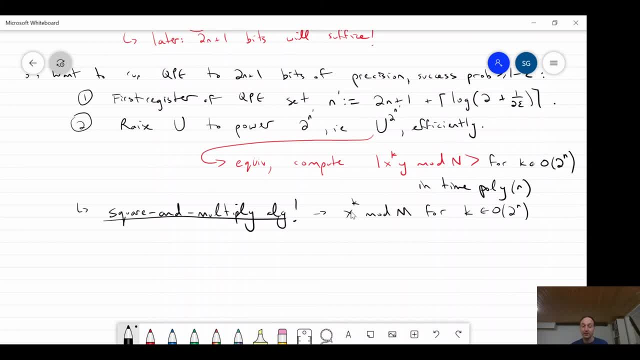 a constant number of x. i can do this explicitly. so how do i get around this? this is um. no, it's not an exercise. well, keep in mind, you have this mod hanging around right, and so that just means that whenever your number gets too big, let's say, 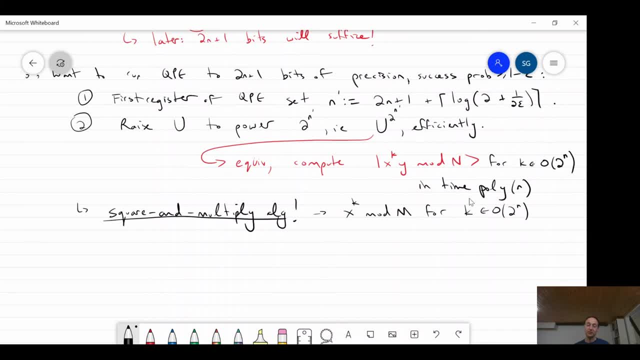 after each time you multiply through by x, you could always, you know, apply another mod m and kind of squish things back down to this nice manageable space. so it's very the number x to the k. i can control how much it blows up. basically okay good. 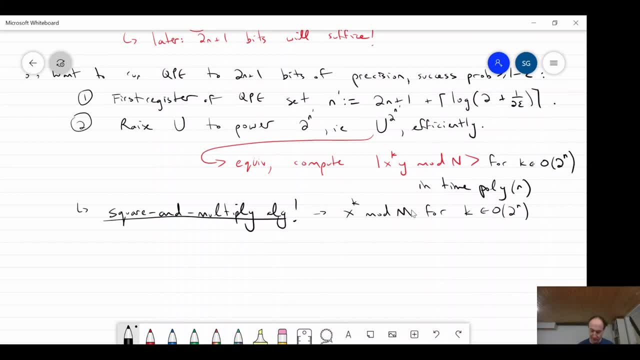 so i'm gonna rewrite this slightly differently. um, okay, so maybe i'll just write what's in the notes, just to be consistent. so this computes basically: oops a to the power b, whatever a and b are right, mod m, and how many times does it need something? 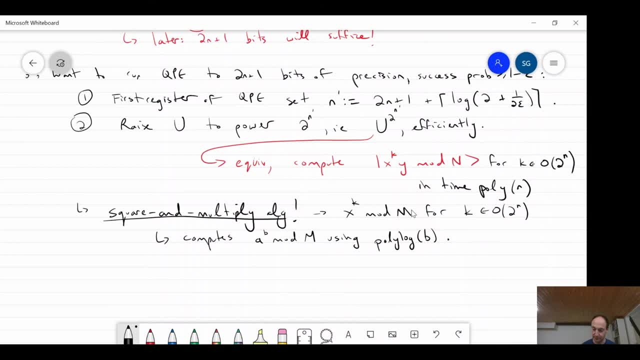 like poly log of the exponent b. um, okay, maybe i shouldn't call them field operations, maybe it's a ring operation because m doesn't have to be prime. but anyway, you get the point. like i'm not talking about bit complexity here. right, i'm counting the number of. 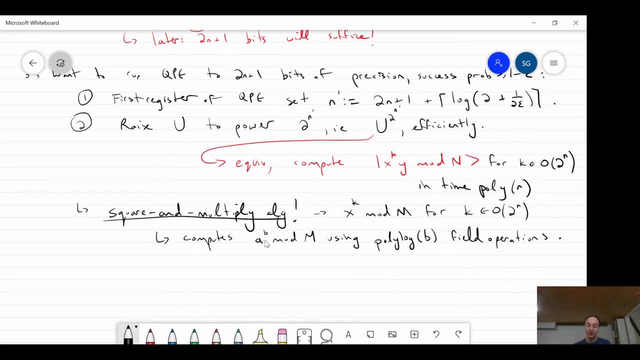 multiplications you have to do, for example, okay, so um and so naively. that's a super naive way. and so um square and multiply doesn't take, you know, um b multiplications. it takes poly log b, so it's exponentially faster and that's of course. 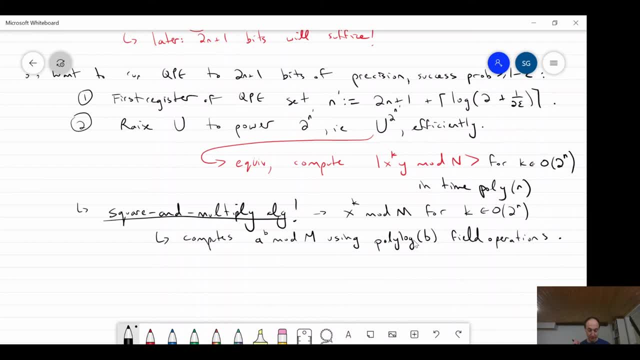 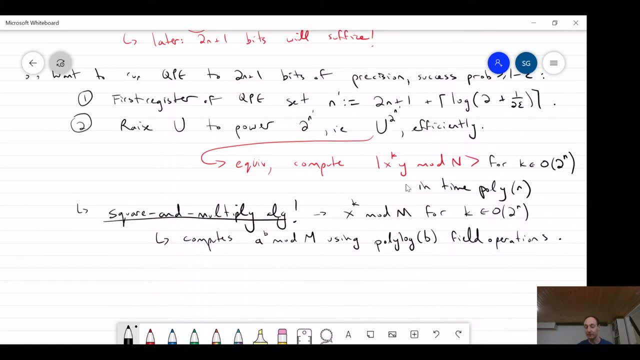 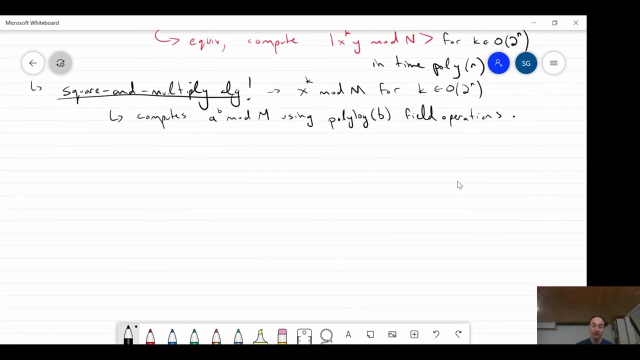 what we need, because in our case, b is huge, b is, b isn't exponential. so you know this log will get rid of that exponential for us. okay, so let's do this classical multiplication to high powers. how do i do it? so there's a basic idea. 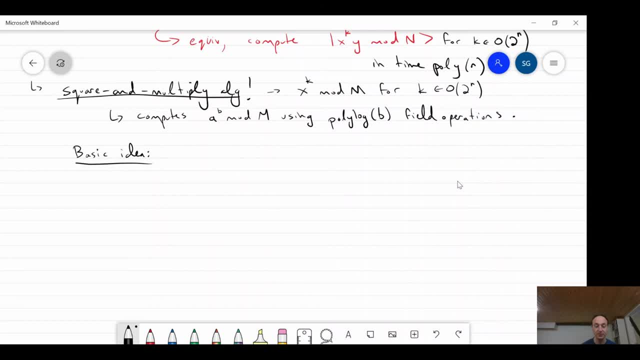 and then there's a simple way to generalize that to more general inputs. so let me just give you the basic idea that kind of has everything you need, and let's just suppose b is a power of two, right? so here i'm expanding. um, you know, b is just. 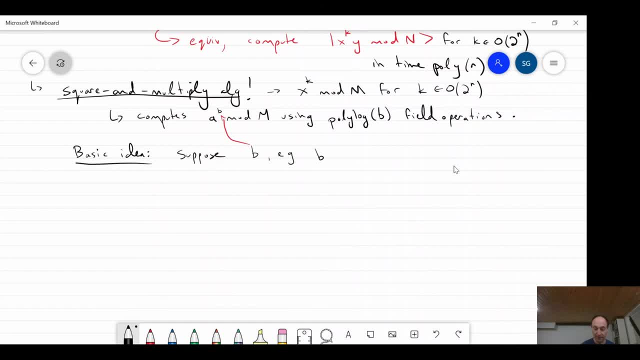 the exponent right. so let's just suppose that b equals two to n. okay, so trivial observation, really trivial. here's your observation. this is the magic of the entire scheme. okay, if i want to talk about a to the b right, that's completely equivalent. um, okay, fine. 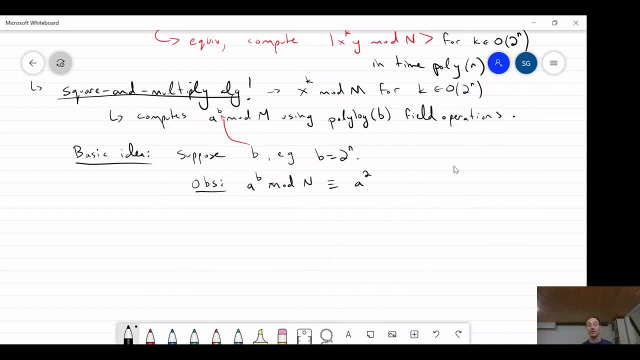 we can do mod n, just to be precise. that is completely equivalent. whether or not you have the mod n, frankly, it's just the exponent down in half, okay? so again, this looks completely trivial if you stare at it, but it does bias something, right? basically what this is. 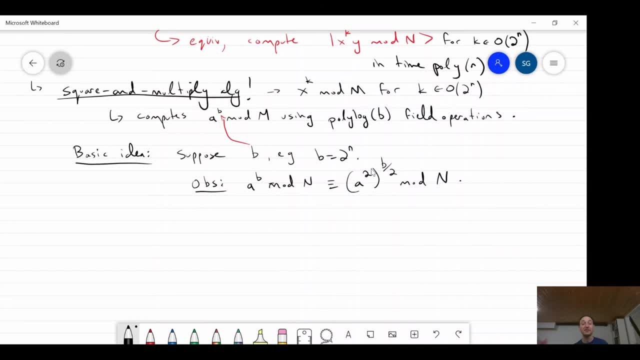 saying is that, instead of i, if i raise a to the power b, that's completely equivalent. instead, i can cut the exponent, the expensive part, right in half. as long as i don't start, it will recursively apply this idea right, it will recursively keep cutting the exponent. 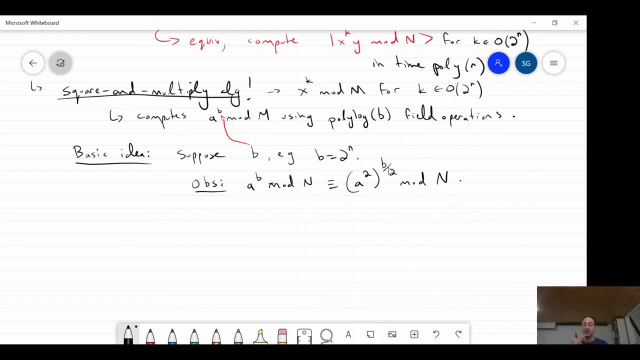 in half, basically, and instead it just squares. uh, you know this underlying term, that it's got here. okay, so you just apply this uh recursively right until, basically, b goes to zero, or, i guess, to one, technically or whatever. okay, but that's the basic idea and you know. 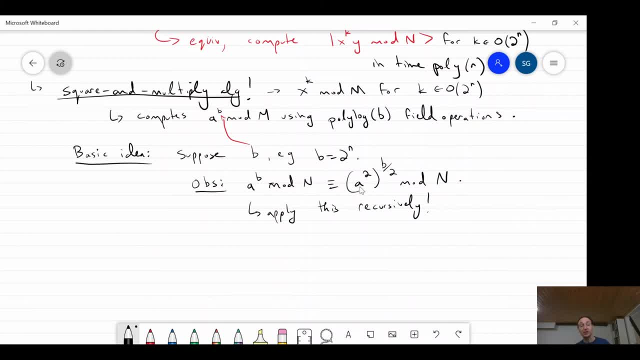 and each time i do this, by the way, of course, i'm doing a square operation, right? so i have one multiplication. um, well, i'm dividing b by two each time. so you know the number of operations, the number of iterations of this is going to be, at most, 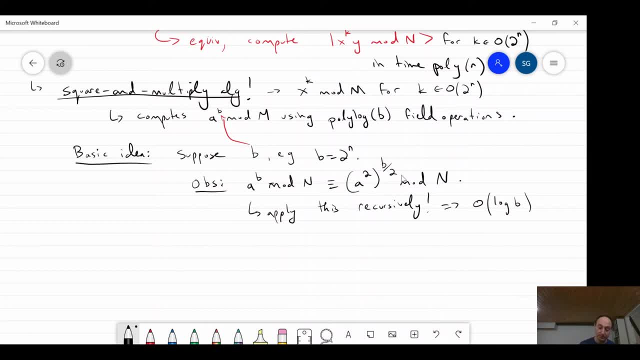 the log of b, right. that's. that's the beauty of it. that's where the b comes from. sorry, the log b comes from right. good, so that's the basic idea. when b was just a power of 2, then we update the recursive step. basically so if 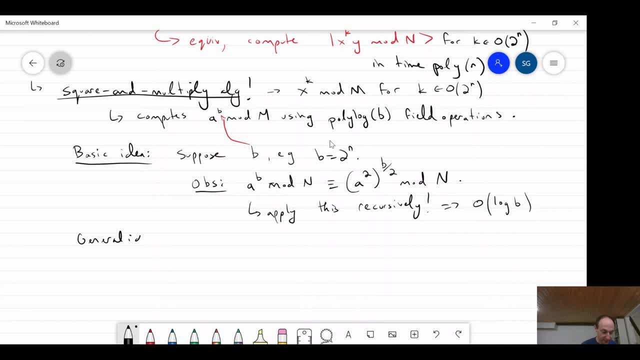 b is not a power of 2, then if b is not a power of 2, then we update the recursive step, basically so, if b is not a power of 2, then we update the recursive step, basically so, basically, we have to um apply one of. 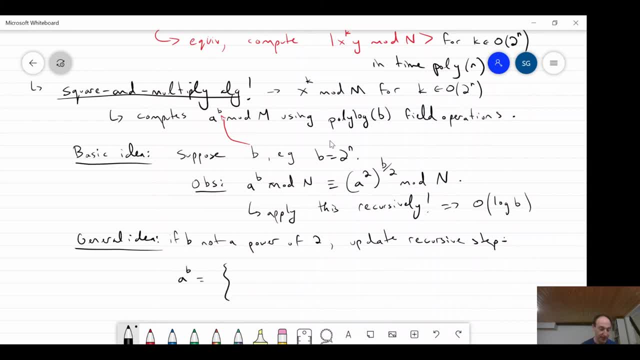 these two cases depending on um. now, whatever a to the, whatever b is right, there'll be two cases. so in the previous basic idea you know we're always, in this case right, b was always even because it was a power of two. so we hit an odd. 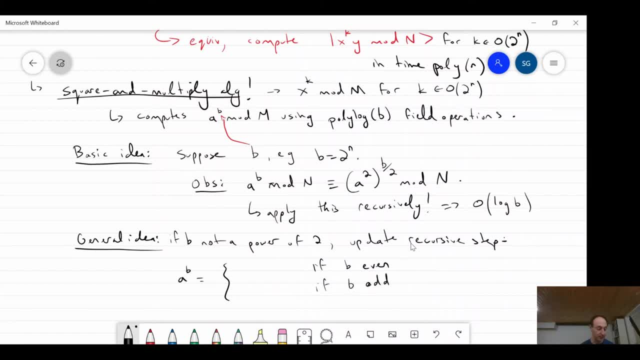 factor right, and then you have to worry about b being odd. that's how this is going to show up now, and you know this is just exactly what we had before. right, there's nothing new here. if b was even so, the new equation we have to subtract. 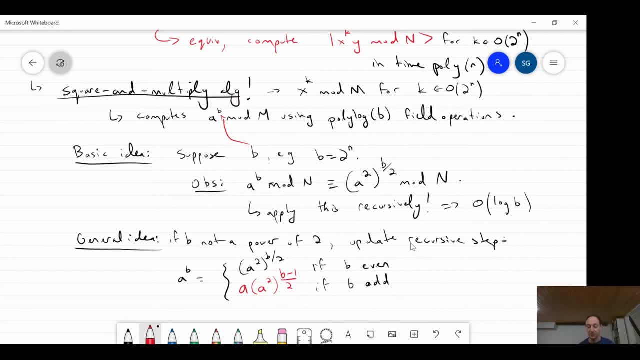 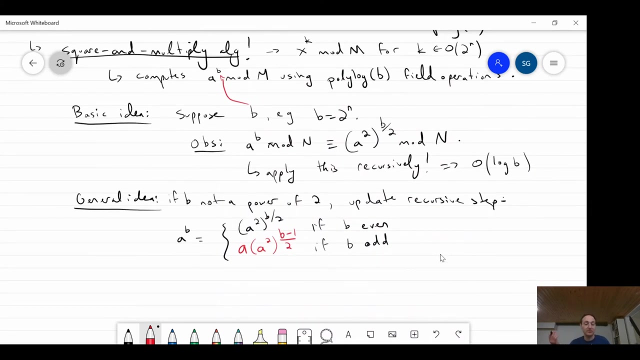 one from b, because now b goes. b used to be odd and now it's even. and then, of course, now i could divide by two, because b minus one is even. okay, that's square multiply, okay. so now just keep applying this until b goes to zero. and then 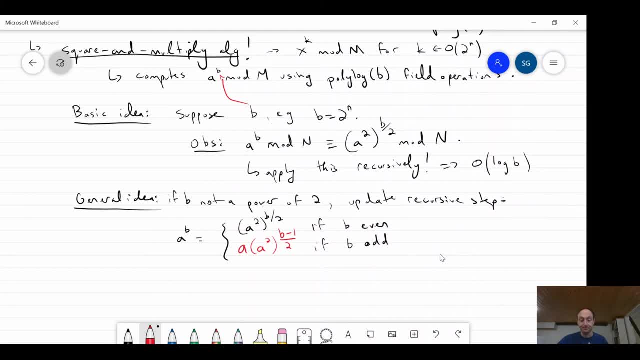 you will see that it's very well known. it's certainly not unique to the quantum factoring algorithm. okay, and we'll see, for example, later on. when we talk about rsa, i mean you know the equation. we've specified the unitary that we're going to. 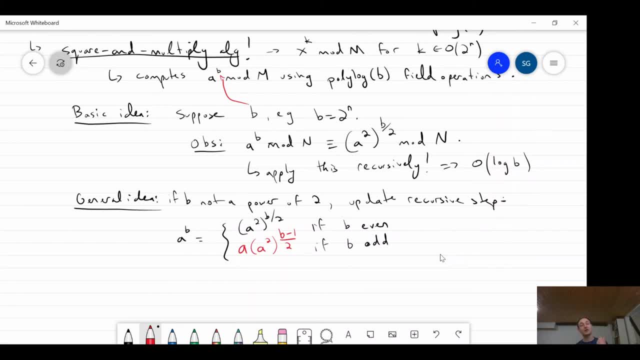 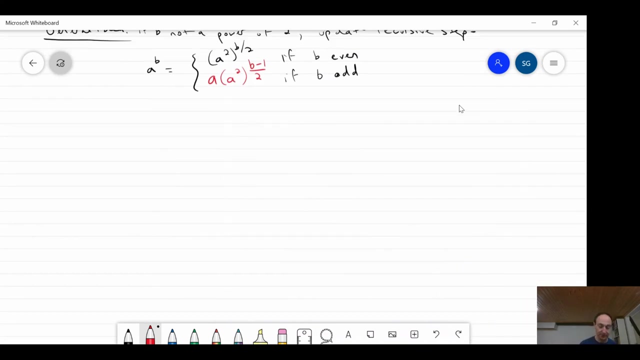 run. we've specified how to get around the fact that we don't know how to prepare an eigenvector, so let's go back to the last phase of the phase estimation. i'm sorry. the factoring algorithm which states the following: 3.3 post. 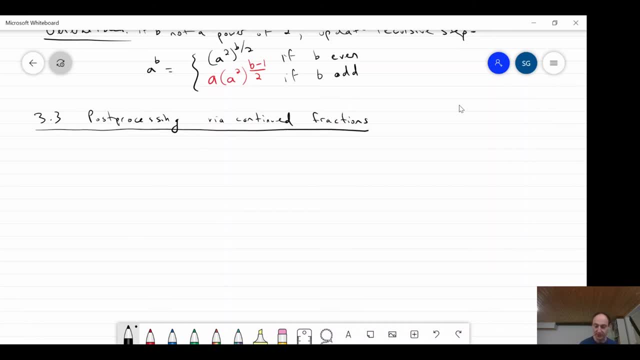 processing via continued fractions, and here you know some things that we don't know. so in section 3.2 we use quantum phase estimation to uniformly at random sample. i should- i guess i should have said sample uniformly at random from the last phase. so in particular, 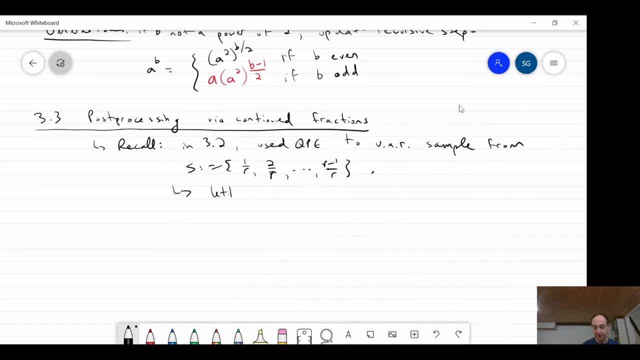 what we really got was letting n equals to basically the log, so this was the encoding size right at the input. so each time we have one bit approximation to a uniformly at random choice of k over r, okay, some element of s right, so i guess i should. 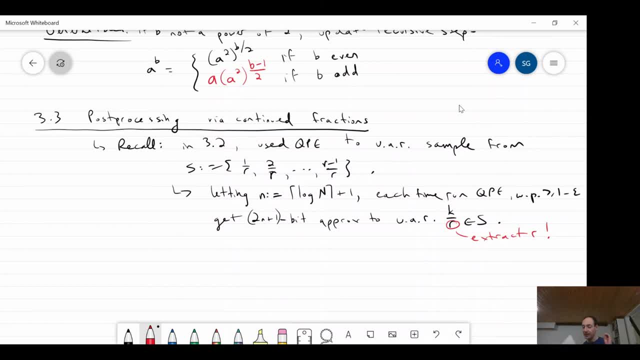 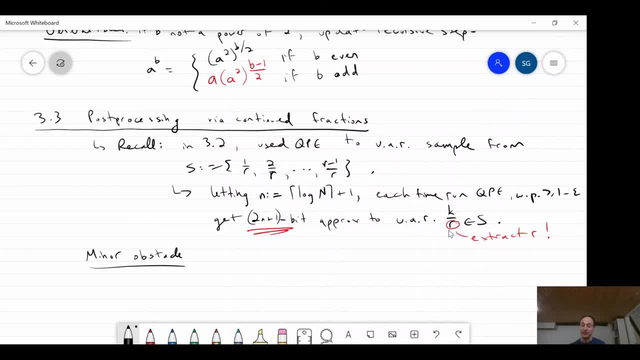 the answer to this question right. so we have one side that i have to figure out the denominator of this thing in lowest terms. you know I'm done, I'll know what r is okay, so if k and r, so okay. so basically, if we want to have any hope of extracting r, 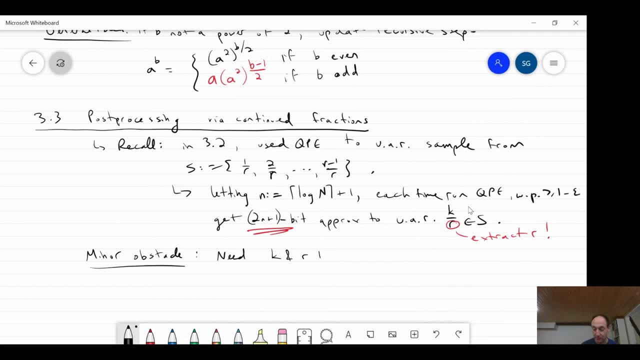 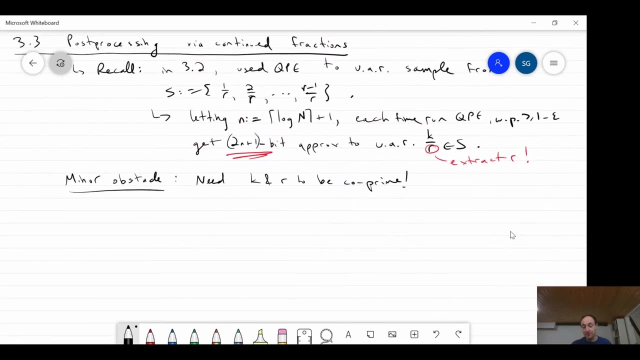 we need k and r to be co-prime, okay, otherwise that fraction k over r is not in lowest terms, okay. and so there are various ways you can get around this. I'm going to give you just the simplest one, because, again, it's just elegant and it just does the job, okay, so it turns out. 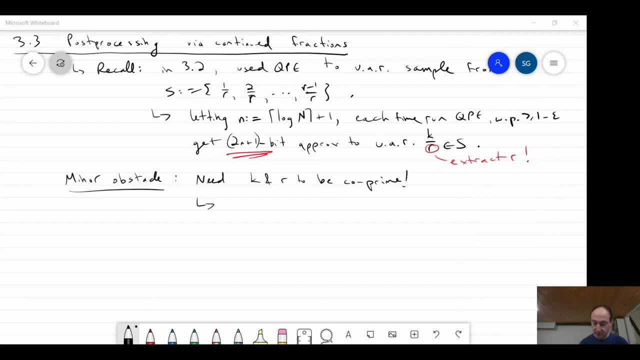 that you know, since you know k is basically in the range, it's, it's basically an integer smaller than r, right? if we just pick it, since k is being picked uniformly at random, you know if the number of numbers smaller than r co-primed it is sufficiently large. 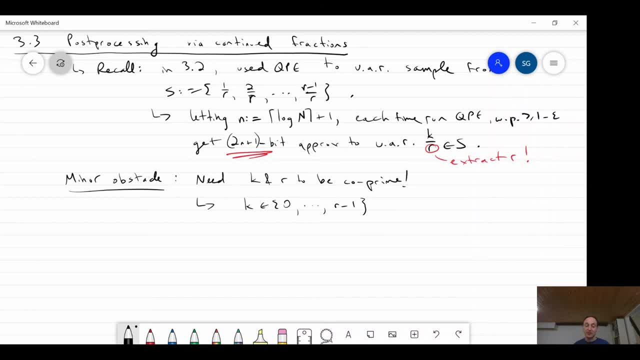 then we can get around this a little bit more easily. so if we just put k in lower terms, then that means with high probability we're going to get exactly this property, that k and r will be co-prime, And actually there's a quantity exactly for this. 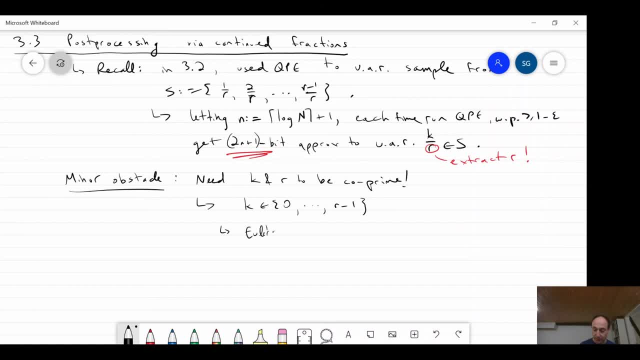 So if you go look up Euler's torsion function, okay, and in this case it would be phi of r- That function basically is just literally the number of integers- I guess natural numbers smaller than r- which are co-prime to r. 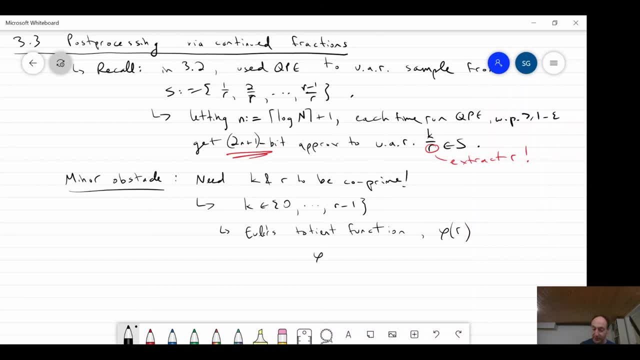 Right, and there are estimates for this number And, roughly speaking, what you're looking at is this thing is larger than r over log log r, It's something like this. Okay, so in other words, the vast majority of natural numbers smaller than r. 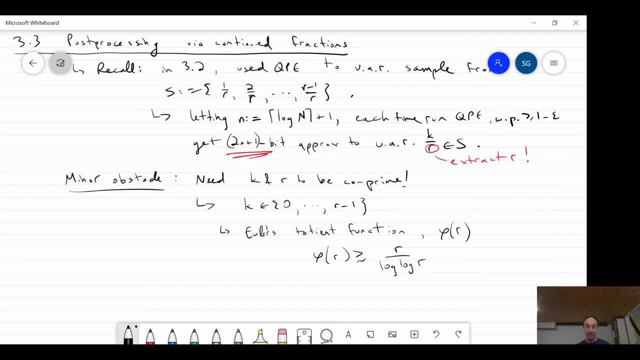 are going to be co-prime to r. Okay, And since we're picking k uniformly at random from the range zero to r minus one, then that means, with very high probability, you're going to get, indeed, k and r being co-prime. 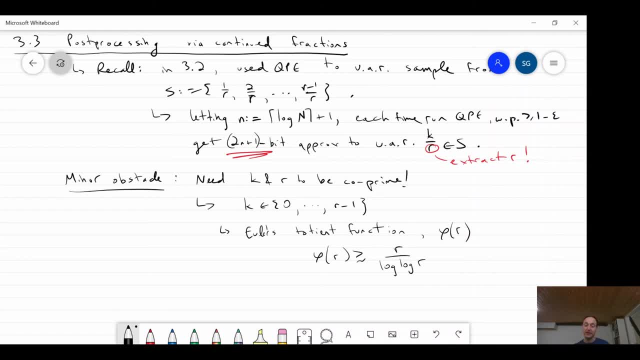 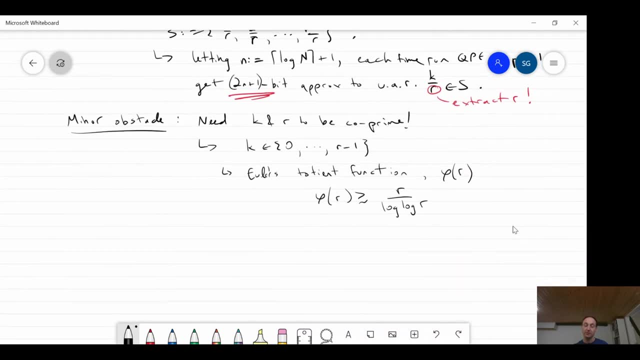 Okay, so you could repeat this a few, repeat the whole experiment like this QPE a few times And, you know, with high probability you'll see a sample k over r where k and r are going to be co-prime. 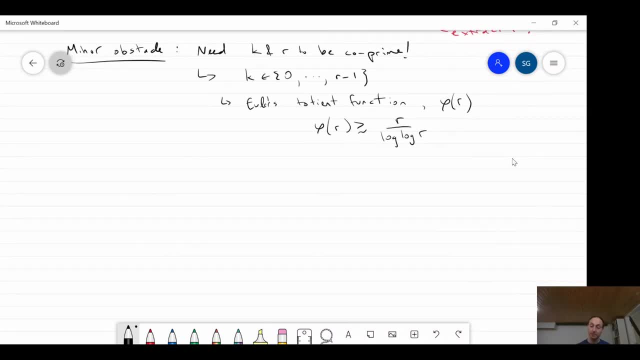 So that's all I wanted to say. Henceforth, we're just going to assume that k and r are indeed co-prime, And that means that the ratio- henceforth assume the ratio k over r- is going to be co-prime. 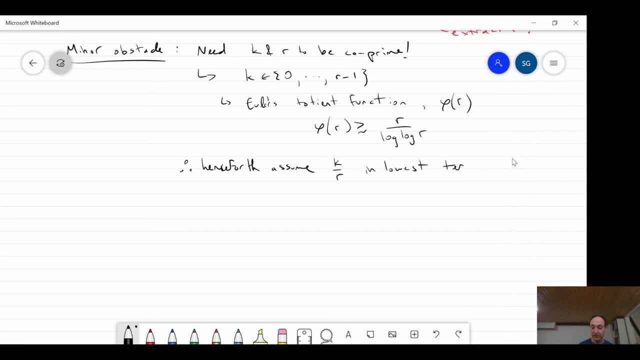 The ratio k over r is in lowest terms. Okay, so if I could figure out the denominator of this ratio, then it will tell me exactly what r is. Okay, so now I can tell you about the continued fractions algorithm. So, continued fractions. 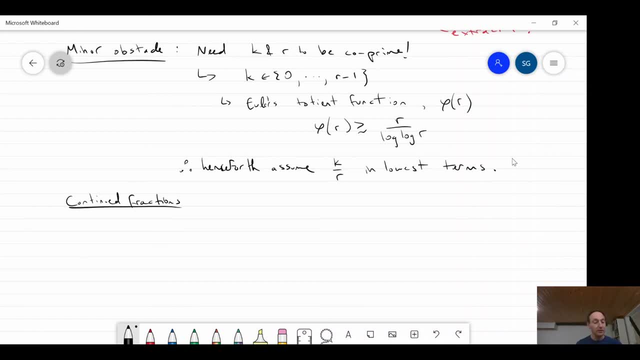 So what is continued fractions In a nutshell? basically, you know, if I have a rational number- a over b- right, Let's just assume that a and b are going to be some positive integers, right? Continued fractions is just, Or the continued fraction expansion as it's called. 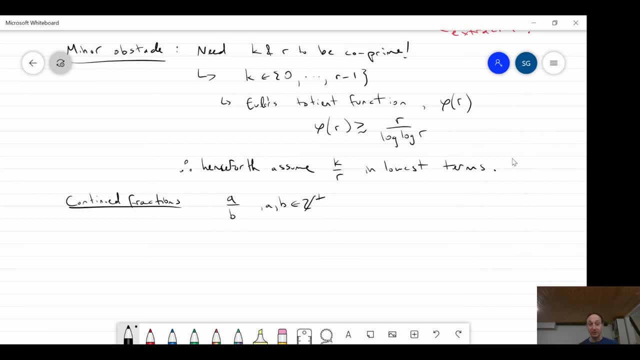 is just an equivalent way of writing this rational number: a over b. That's all it is Okay. Okay, so it's going to be an equivalent expression for a over b. It's just another way of writing it down, right, but of course this way will have its own advantages, right? so instead of writing a over b, 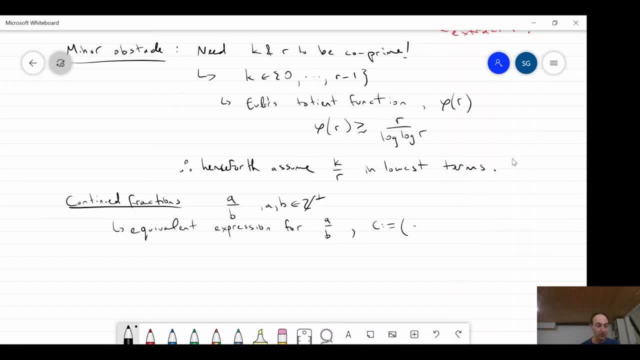 instead, what we're going to do is we're going to write a larger list of integers: c0, c1. that's a typo in the notes. okay, um, cm, right, and what is the relationship between a over b and this funny sequence c? i've written down: um well, the fraction a over b equals precisely what happens if we do. 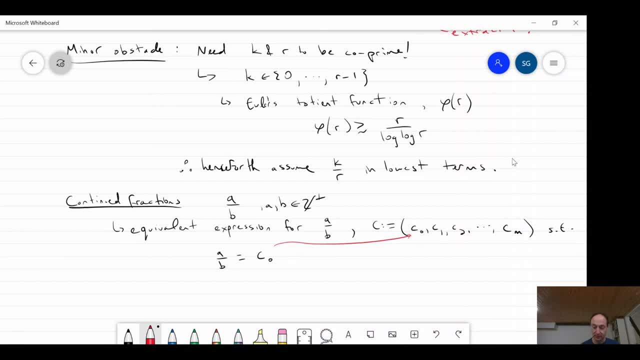 this. so first we take the first uh term- here's c0, right, and then what you do is you invert. and then you take the second term, c1, okay, that's this one, right, and so forth. and now you keep repeating this: add and invert, add and invert, right, plus one over c, two um again, as you can see, this is going to get. 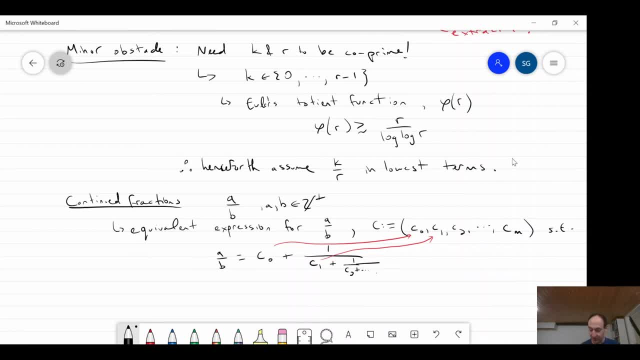 a little bit messy, plus dot dot dot, and eventually you're going to get something like plus one over cm. okay, so that's the continued fraction. so that's the continued fraction of a over b. okay, it's just this weird funny recursive structure where you just add the next term, ci, and then you invert the rest. 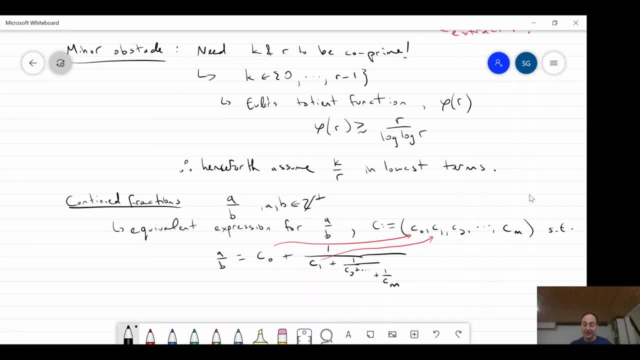 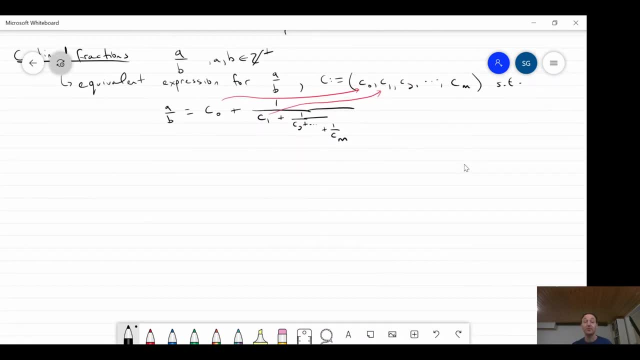 okay, so why in the world would you do this? right? it's uh, we used to have two numbers and now we have m numbers, so you know, we just made things more complicated, right? well, there's, of course, a huge benefit for us, which is the following: so note that 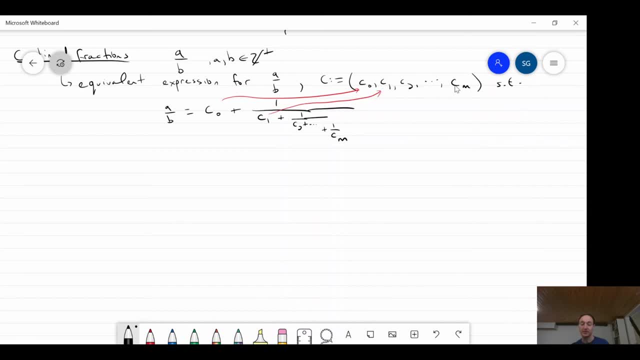 technically speaking. you know, if i were to use all the coefficients, uh, in this expansion, right then indeed i recover a over b, but i can instead think of this as a sequence, not just a single rational number, but really is representing a list of rational numbers or sequence of rational numbers right? because you 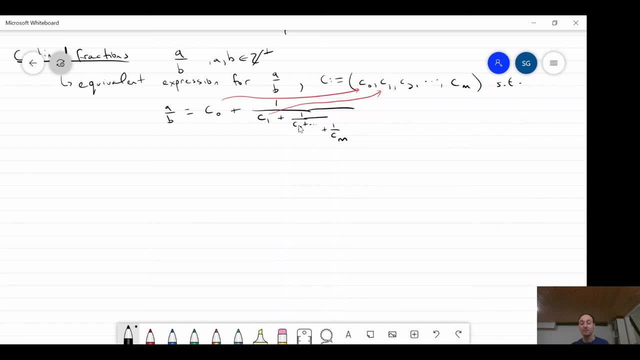 know, in this kind of expansion process where i keep adding and inverting, i don't necessarily have to use all the way up to m, right, i could maybe just use c0, c1, c2, and then i just have three layers of this expansion and that's some rational number. it's not a over b, but it's something i 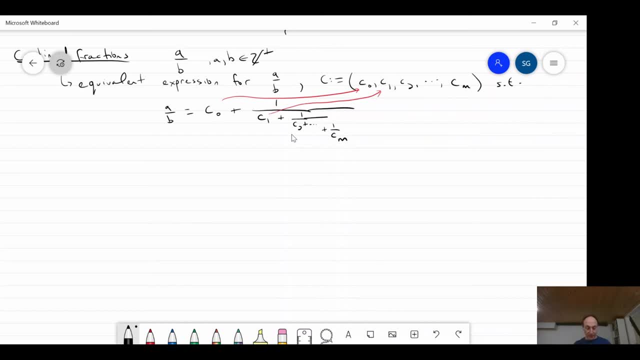 could still write down right and so, in particular, you know, we define or give this thing a name. um, you know, ck is just going to be the sub sequence of c, which is just zero up to the kth term. okay, we don't go all the way. 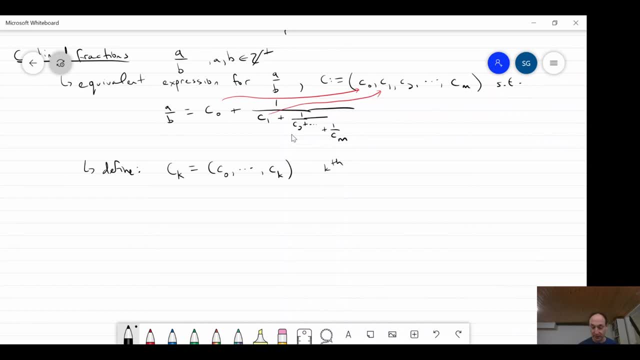 to the end. we don't go all the way to m. this is the kth convergent. okay, this is a definition, okay and um, so what did we have in in phase estimation? right, what we had is that, you know, we don't have k over r. 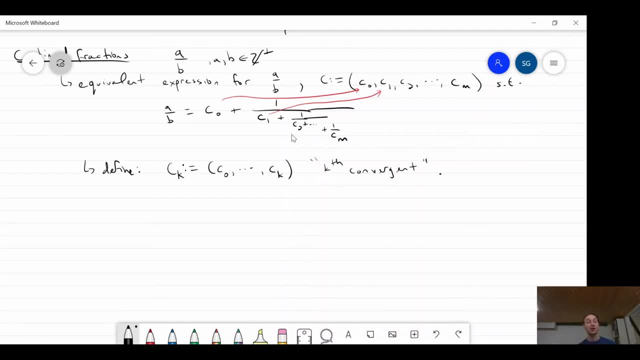 right. what we have is a very good approximation to k over r. we have a rational number, okay, so maybe i should remind you. so qpe gives a finite meaning, a 2n plus one bit approximation to k over r. so in particular we don't have that, and so let's call this approximation just x for now. so x is 2n plus. 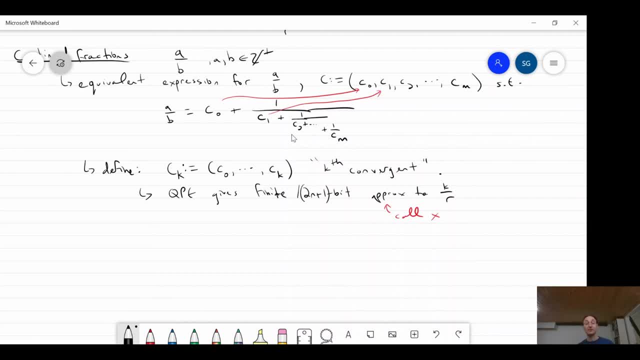 one bits and it approximates k over r. that means k, by the way, is rational, not because it approximates k over r, but because it's a. it's a has a finite binary expansion, right, so it's certainly rational. so this is rational and that means that in principle, um, i could write down the continued. 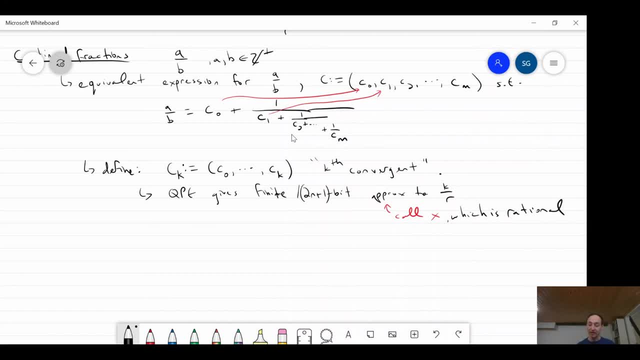 fractions. expansion of x. okay, also in practice i could do it. and the other thing i know is that, um you know, k over r to quite high precision, right, It gets the first 2n plus 1 bits. So in fact you know. 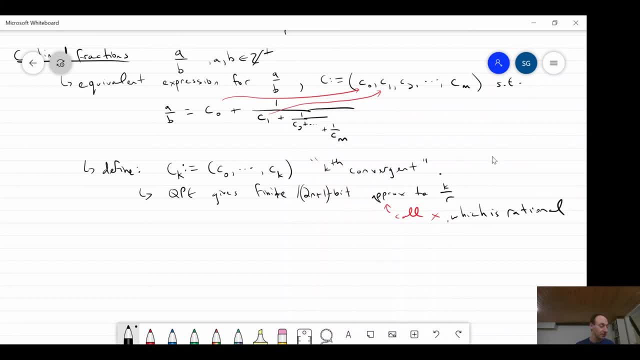 this funny rational number, x is quite close to k over r, And the point is that if I take the continued fraction, so if x is a rational number that's very close to my target, it turns out that if I write down the continued fractions, expansion of x, then there exists a convergence. So if I 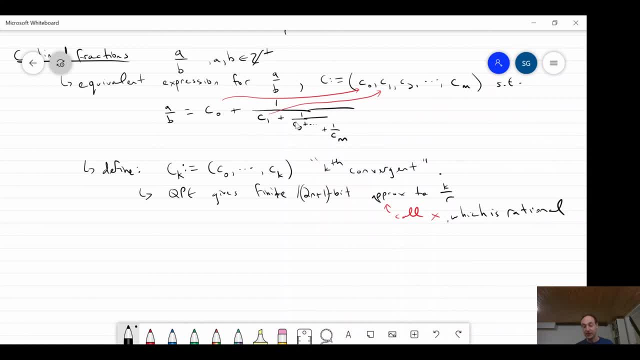 cut off the sequence at the appropriate point. you know the continued fractions expansion I would get for that convergent would give me exactly k over r. So in other words, even though x is just an approximation to k over r, it would give me a way to basically snap x back to k over r exactly. 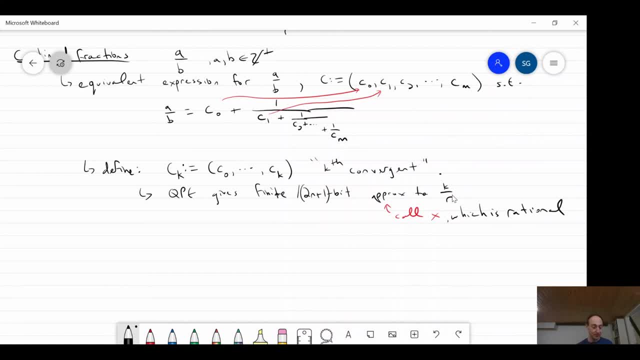 in some sense. okay, to kind of round it off. So let me give you the theorem that states this. We're not going to prove it. It says we have k? r being positive integers. x is a rational number. that's what this q is. 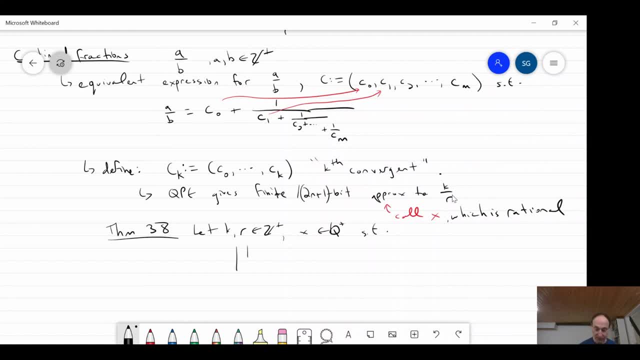 And these guys satisfy the following: bound: right. So I want k over r. that's not what I have. Instead, I have the estimate x. that's what we have. okay, And as long as the estimate is good enough, right, it's close enough. So what does good enough mean? Well, it's smaller than you. 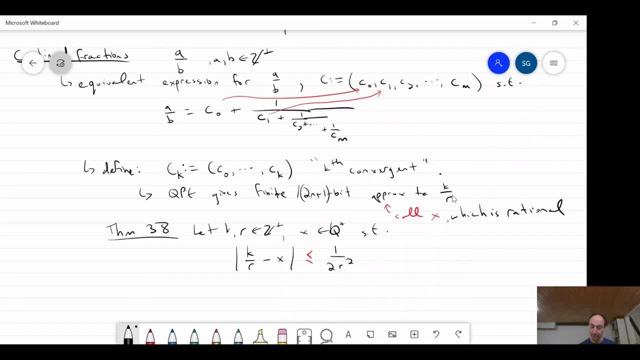 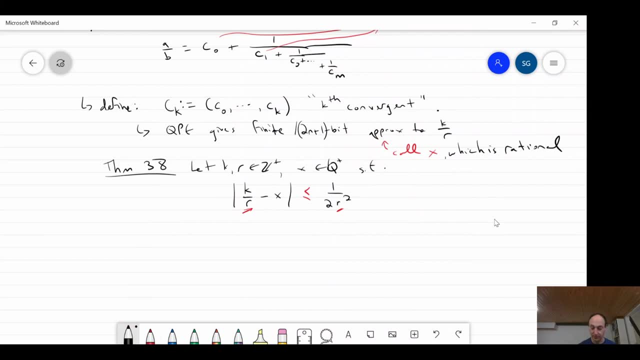 know, whatever 2r squared is Okay. so notice how r is, of course, the same. this is the order in our case, right? As long as this is true, your estimate is close enough, Then if we see you know again, c is going to be the continued. 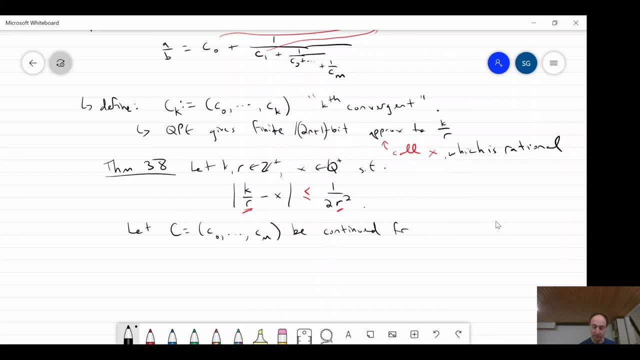 fractions expansion- expansion of x. right, so this is what we get out of phase estimation. In our case, it's very close to what we want. So if I take the continued fractions expansion of x as theNet ramp, What's gonna happen here? 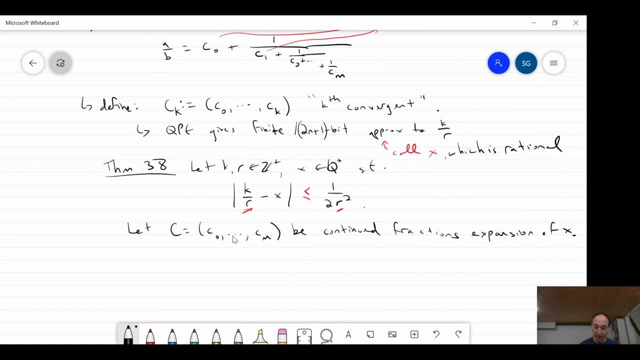 So let's call it this: that's taking it all the way to the end. then there exists an index k in this expansion, such that that kth convergent, meaning, if you just expand this thing up to order, ck, up to c0, up to ck. 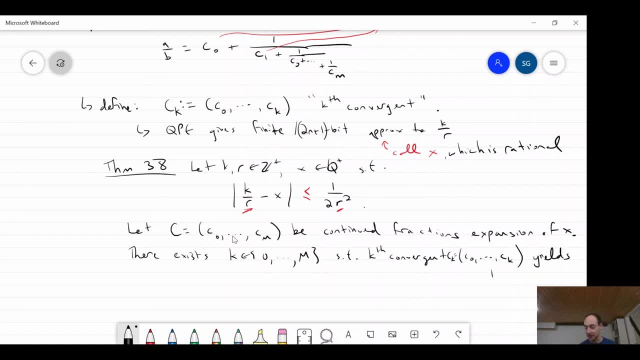 this thing represents k over r, exactly Okay. So that's amazing, right? So, even though I have this weird approximation to k over r, there's a sense in which I can recover k over r, exactly Okay. and so exercise 39 asks you to double check. 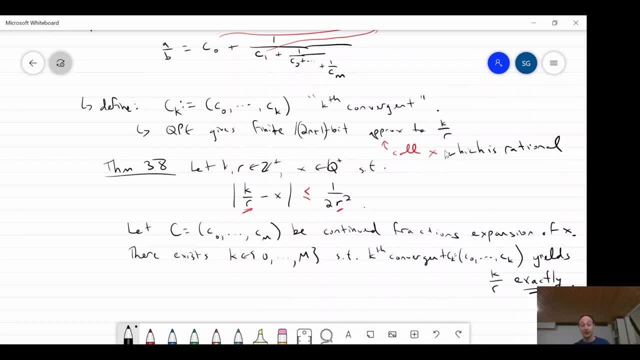 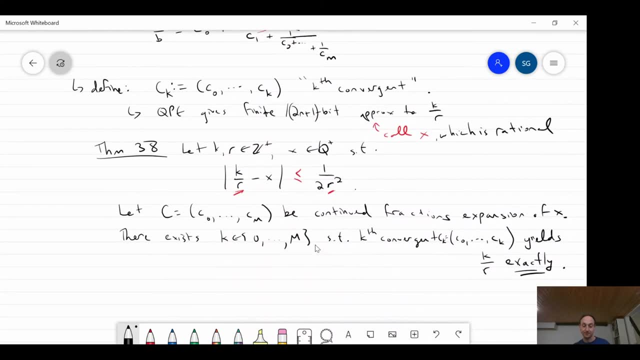 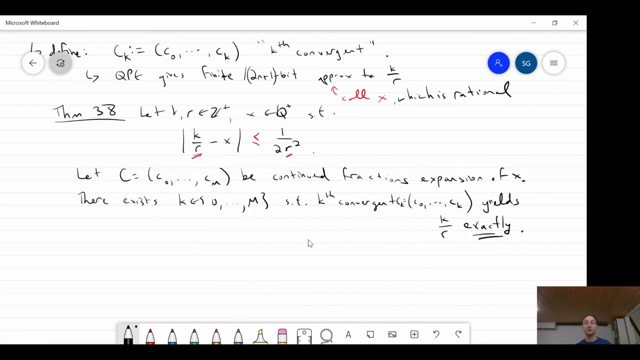 that, since we use two n plus one bits of precision to approximate k over r, you can check that. indeed, you know, this bound holds. Okay, so I'll leave that as an exercise. Okay, so you know, this almost gives us what we want. 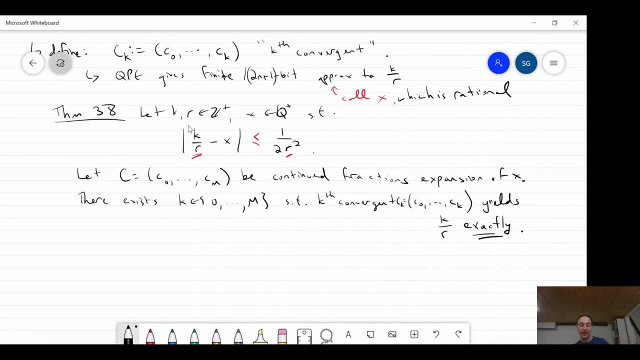 because this means that, you know, given my funny approximation x, I can get k over r exactly. In particular, I get a continuing fractions expansion of k over r. So therefore, given x, can extract a continued fractions expansion of k over r, right? 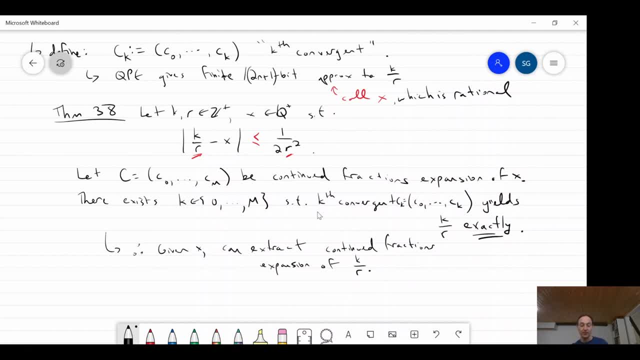 That's what I've got so far And, of course, let me just make a quick comment A priori: we don't know which convergent for x. right, It's supposed to give us k over r. That's not obvious. 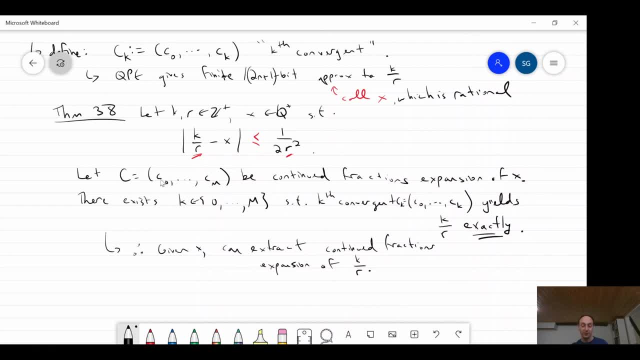 I mean, if you look at the proof, obviously you can figure out which one it is. But you know, if I just give you this expansion, it's not clear which one it should be. But you know, you can prove that. 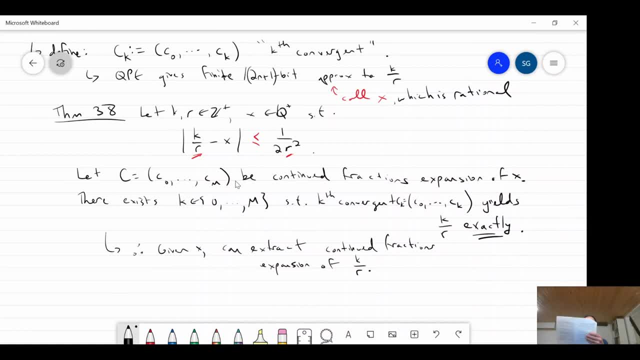 and I think we're gonna get to that in a second. Yes, we're gonna do that in a second. It turns out that you know this m the number of terms in the expansion is always polynomial in the encoding size, right. 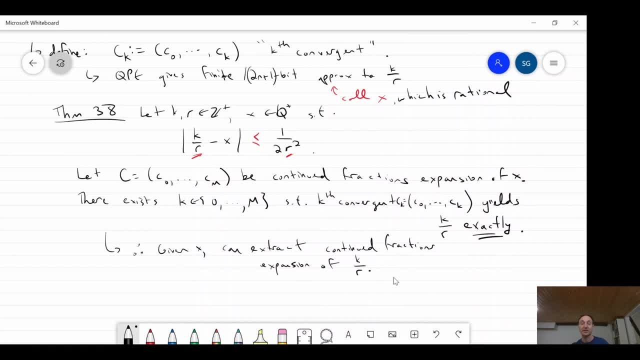 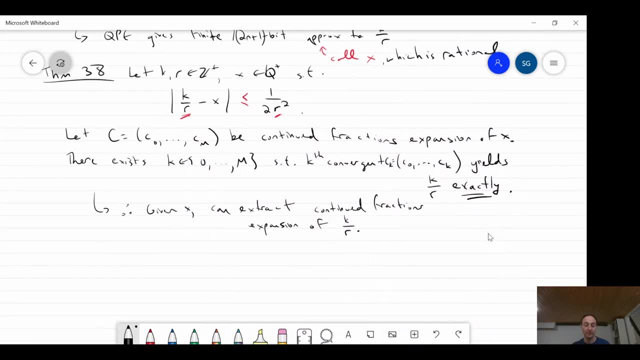 So you can actually just try all the convergence and see if you're able to extract a proper order r and then factor your integer n. Okay, so you can just try all the convergences, the short story, okay. Okay. so given x, we can extract. 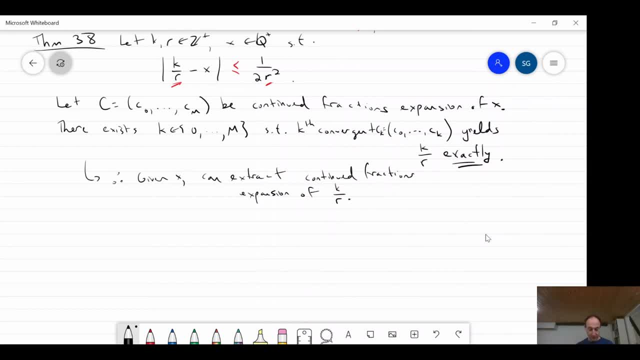 the continued fractions expansion of k over r. Okay, Okay, but we don't want that. We want r, not k over r, right? So now I know exactly k over r, but of course now I need to still get r. 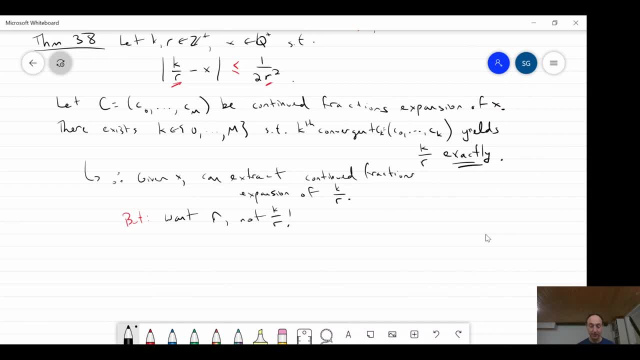 Okay, so there are three questions left right. Number one is: how large is m in theorem 38?? Okay, so, if I look at you, know this m over here? right, I'm taking the continued fractions. expansion of x. 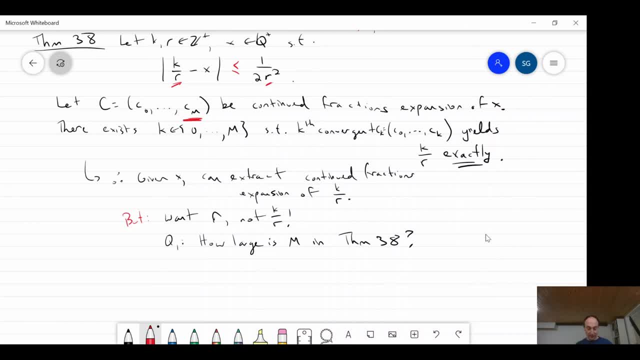 how big is it? Well, it turns out that- and we won't prove this here- it turns out that, since k and r are n-bit ints, we can choose m being order n Okay. so the point is that you know. 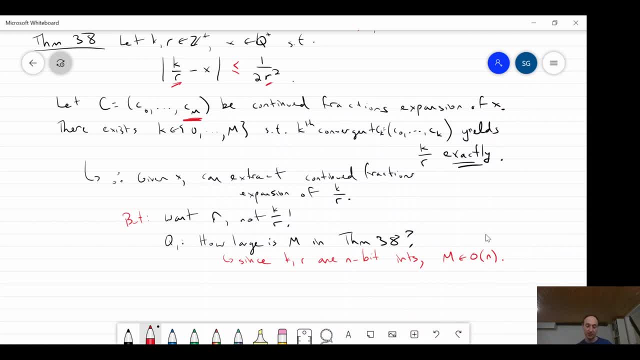 the number of terms in the expansion does not blow up exponentially. It's fine. it's just linear in the input size. Okay, so that's very good. They're just a linear number of convergence. we would need to cycle through to figure out which convergent gives us k over r. 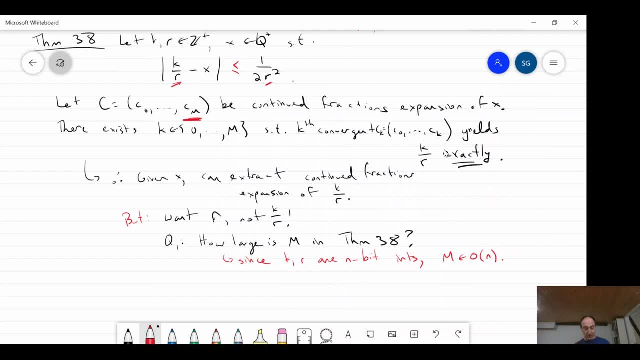 Okay, And now the other two things that I haven't really told you about is well, number one: if I started with x and I said I compute the continued fractions, expansion of it, well, how do I do that? Right, I haven't told you that. 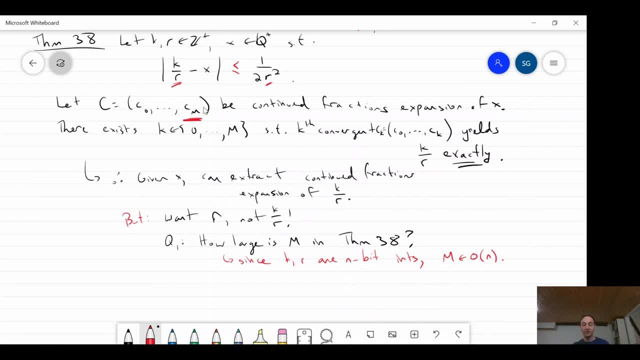 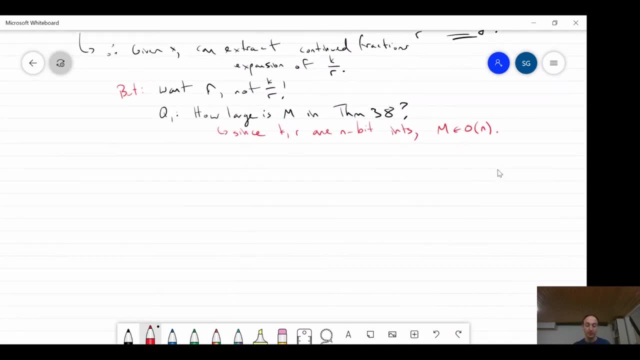 And number two is: once I've, you know, got my hands on the convergent of this thing, which really does give me k over r, then how do I extract r? So those are the last two things we have to quickly discuss. 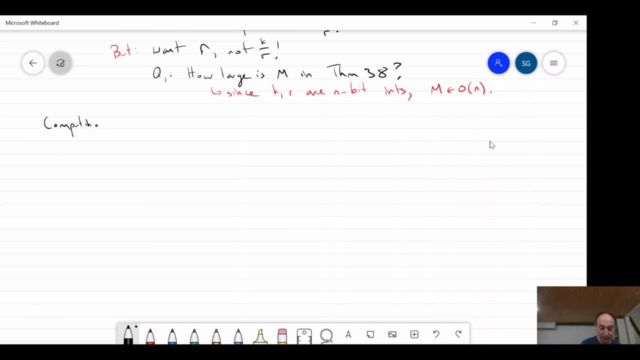 So number one is: let's show how you would compute the continued fractions expansion, And so the algorithm is very simple. actually. There's nothing, there's no magic to it. It's kind of like what you would come up with if you just stared at the expansion. 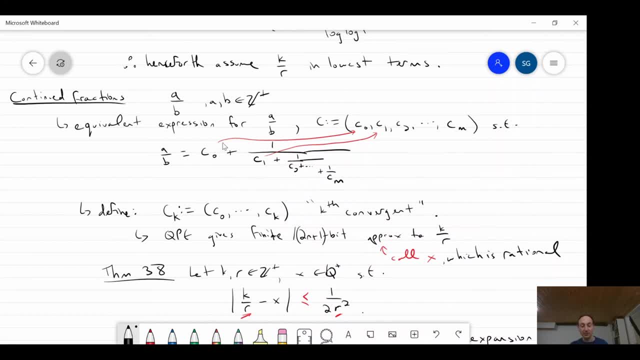 for long enough and tried to reverse engineer it like literally. So it's literally trying to implement. you know, you start with a over b and then you literally try to strip off a term and then invert the rest and you repeat this over and over again. 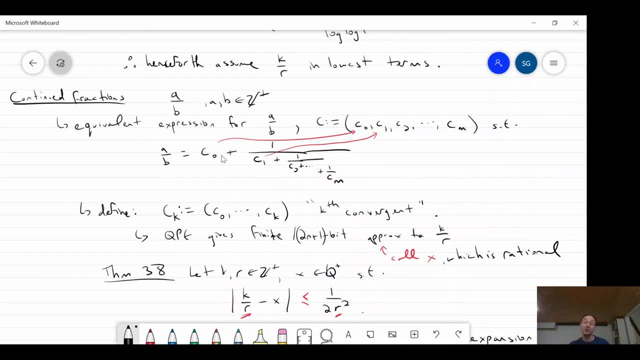 And the only question is: well, what do you strip off here? And the rule is gonna be: be greedy. Okay, it's a greedy algorithm. It's gonna strip off the largest integer it can, And then it's only gonna have a rational component left. 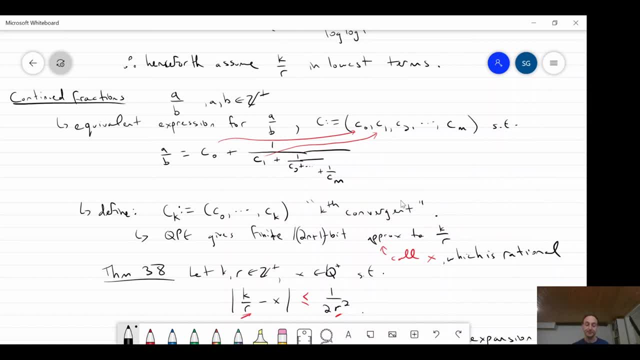 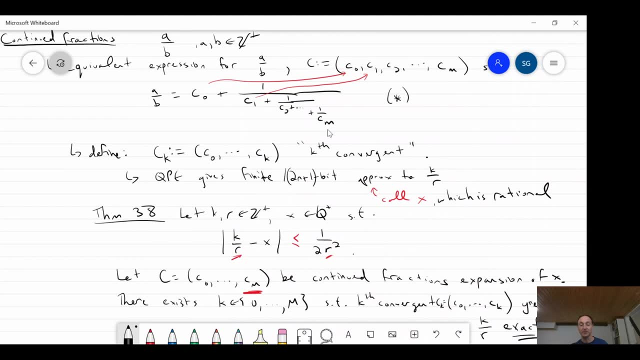 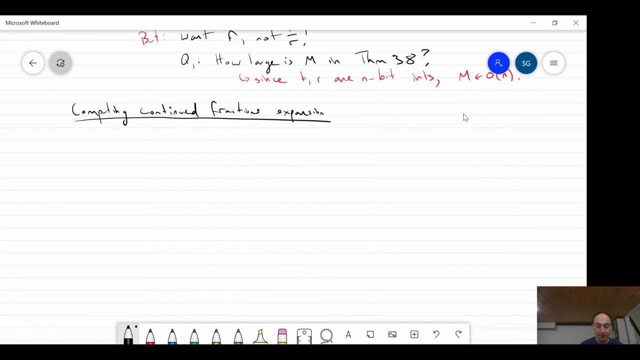 and it's the rational part. it will invert and it will repeat. So basically, we want to. if I call this equation star, we want to implement the star basically in a greedy fashion. Okay, so let me give you best way to do this is to be an example. 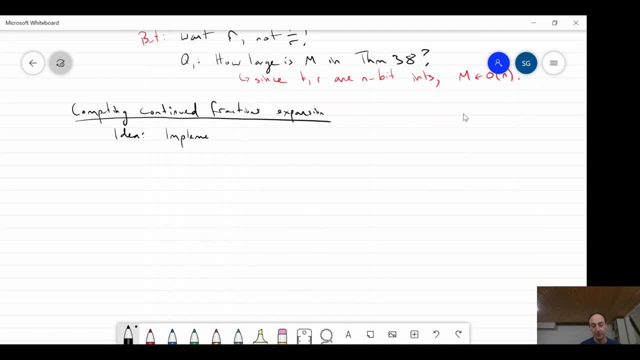 So the idea is to implement equation star greedily, quote, unquote. And let's just start with this example: 23 over nine. Let's write down the continued fractions expansion for this. So remember what we did is that you always split off. 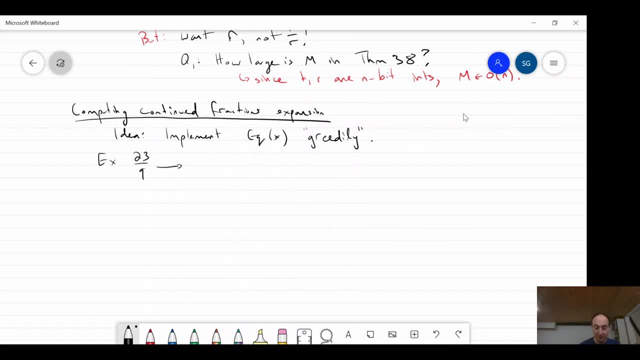 a term and then you invert the rest. That was the trick. So first the split will make it greedy, We will split off the largest integer possible, right? So you know, nine goes into 23,. two times plus some of our remainder. 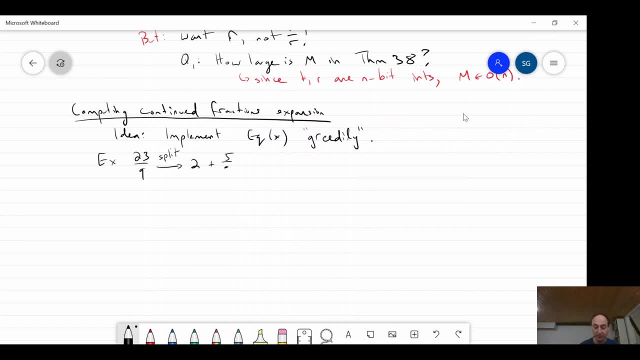 So that's the integer part, And the fractional part is this: one five over nine right, And now I'm gonna invert. Now I do the inversion step where I invert the second half of this right. So it's two plus one over, and then maybe I'll write this: 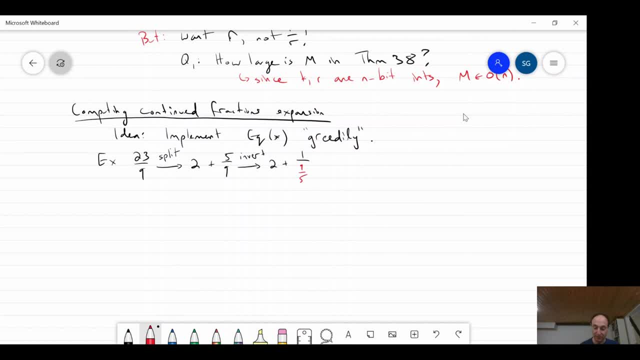 Okay, And then maybe I'll write this in red. This is nine over five. you know, that's just the inverse of this thing here And now I just recurse on the nine over five. exactly the same thing over again, right? 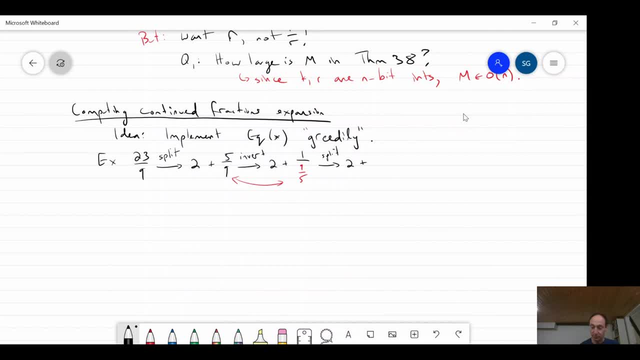 So again, I'm gonna have a split step, which is just two plus one over, and now nine over five. Well, that's just one plus four over five. right there, I just did my split step, and now I do my invert step again. 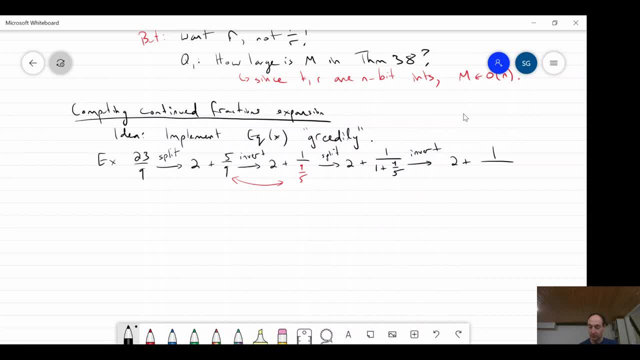 So I get a two plus one over one plus one over five over four. Let me just do it this way. There we go, Okay, And I think we just need one more and we're done. So I'll just scram it here. 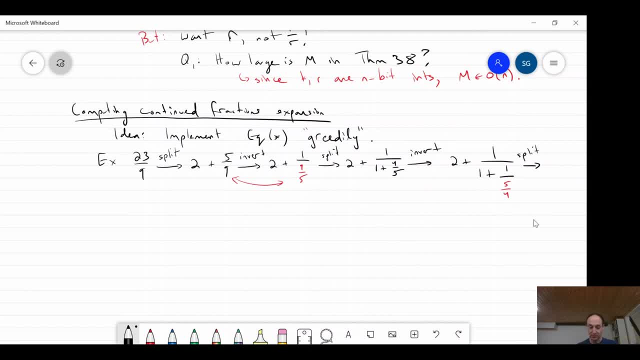 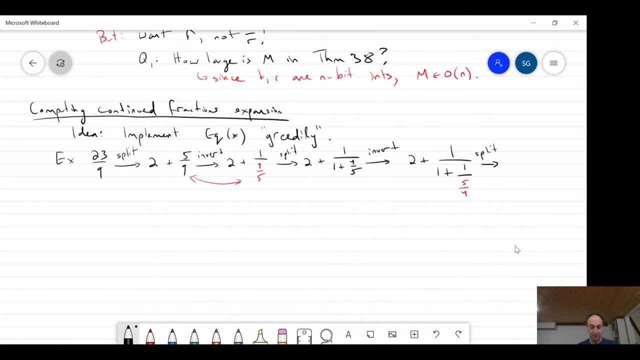 So one more split step, which is: let me just move this slightly over to the left Yellow Screen does not wanna move. Maybe it did. did it There? Two plus one over one plus one over one plus one quarter, Right. 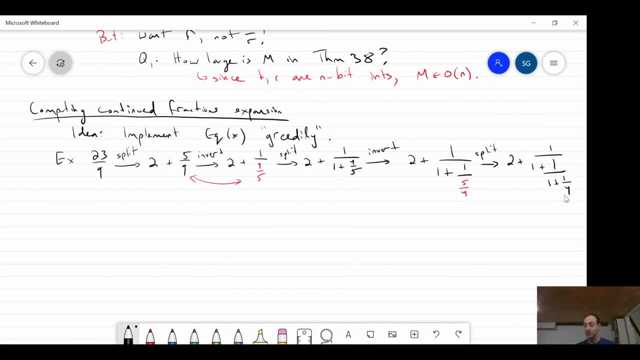 And now we're done, because, you know, the last rational number I came up with is one over something right, So now I'm done. So that is the continued fractions expansion for this number: 23 over nine. Okay, You can prove, I won't do it. exercise 41,. 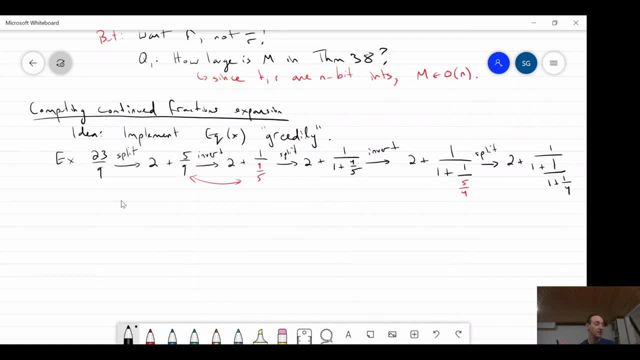 that if you start with any well, I mean, we've sort of already given away the answer right. We said that the continued fractions expansion will have. if each of these guys takes n bits to write down, then you know the expansion will need only order n steps. 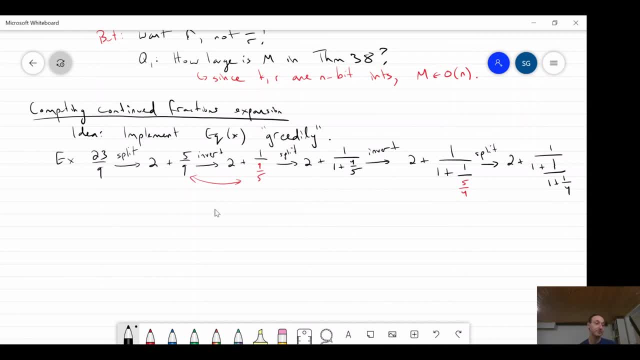 And that in particular means that of course this thing is finite, the expansion. So this tells us: you know, given the x that we got from our QPE estimate, quantum phase estimation, I can compute the continued fractions expansion of it. 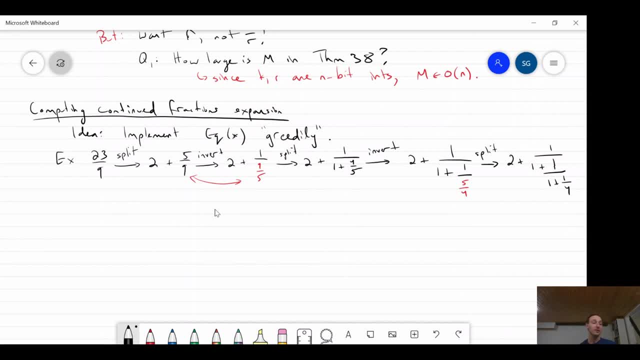 One of the conversions will be what I'm looking for: K over R. And now, given that convergent- whichever one that is, I want to invert it and extract back the numerator K and the denominator R, And that's the last thing we need to cover for the algorithm. 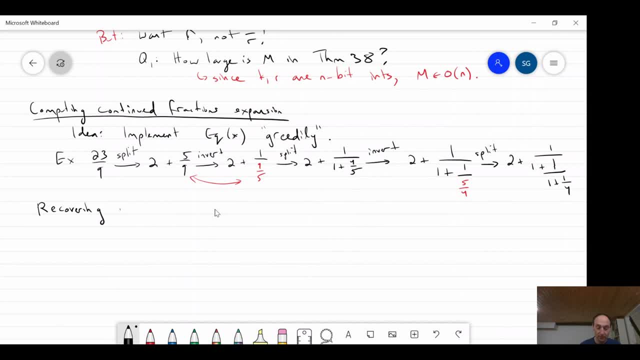 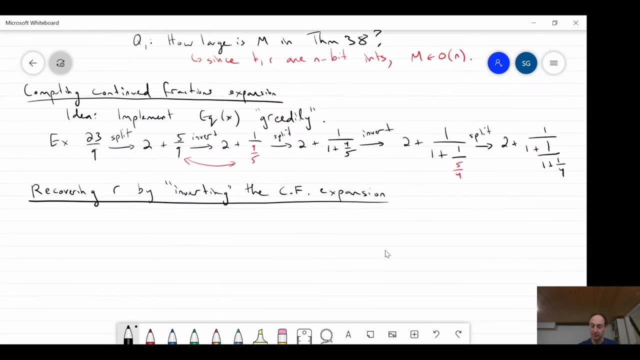 the factoring algorithm, which is recovering R by basically inverting the continued fractions expansion. So I'll just write CF from now on. I probably should have started doing this right. I should have been doing that much earlier. Okay And okay. 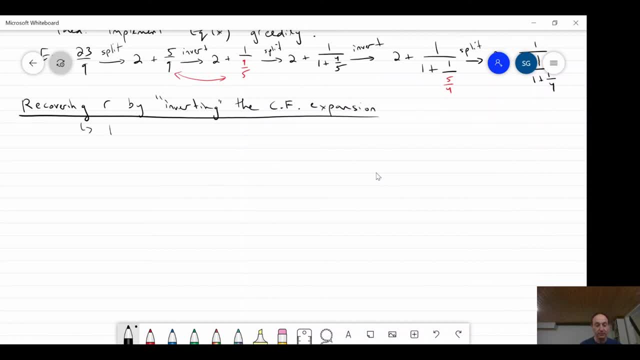 So basically the idea here is that so, having computed now, C equals to, you know, C, zero C. one dot dot dot CM of x. Remember, this is the x, is not K over R, it's the estimate of it. 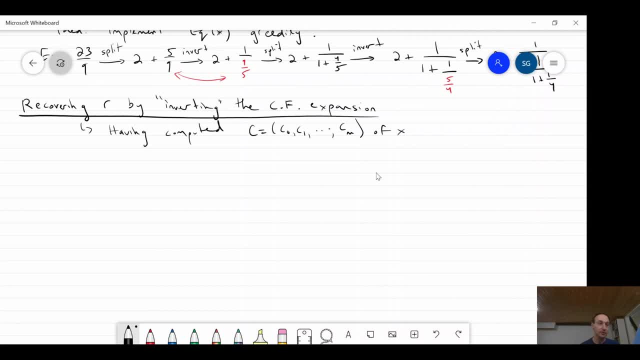 Right. So by sorry, let me just remember which theorem this was. So by theorem 38, we can try all convergence of x till we hit K over R, the convergent for K over R Right, And this will take polynomial time. 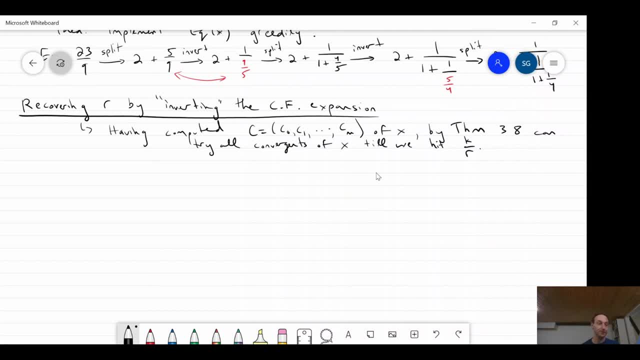 because we said the number of convergence is polynomial in the encoding size, little n, And so given the convergent now for K over R. so therefore, given the convergent for K over R, we apply this theorem. Okay, so what theorem is this? 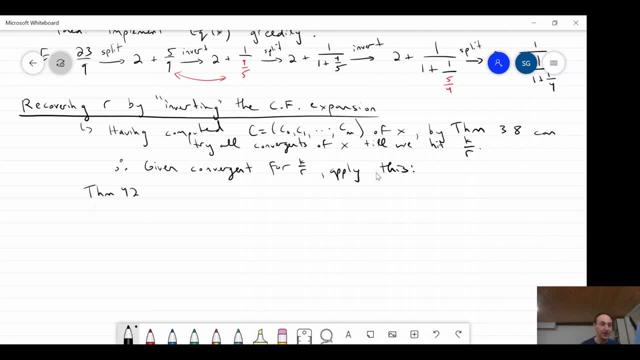 It's the final theorem, which is theorem 42.. And it states the following: Given, you know, whatever the K-th convergent is, convergent CK equals to C, zero up to CK. These are all positive integers, And then what we'll do is we'll define, you know. 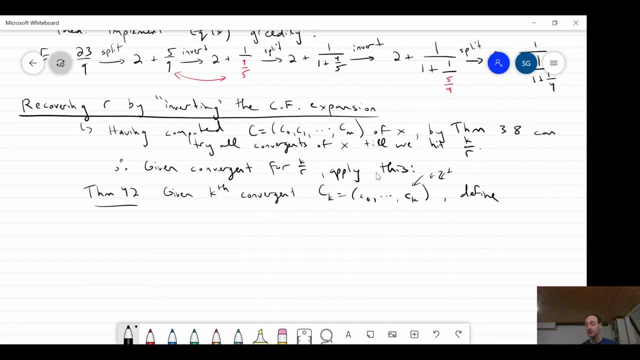 again. you can cut off this convergent at any point and that will give you another rational number. And so let's just define that sequence of rational numbers, Define basically AI over BI as, and we'll do it recursively. So the very first choice: A zero, B zero. 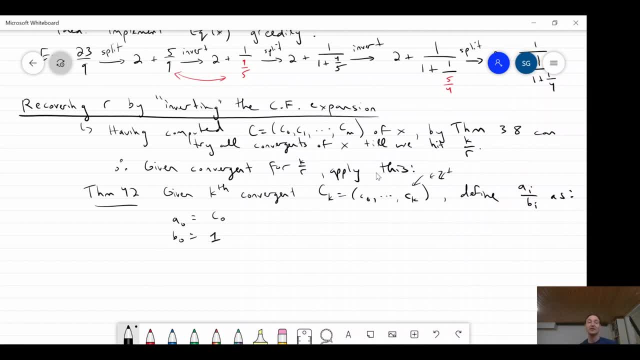 that's just going to be a C zero and one, And the exact things I'm going to write down don't really matter. The point is what will come out of the stem, right, But let me just show it to you for completeness. 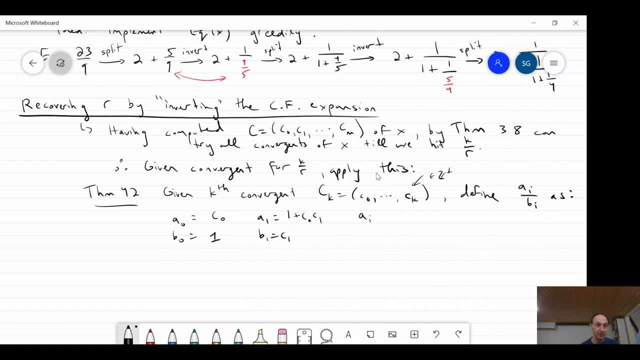 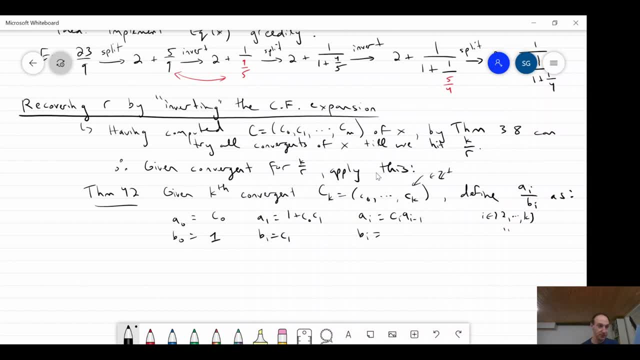 This equals to CI AI minus one. so you see, it's recursive plus AI minus two. Okay, and you can probably just reverse engineer this just by staring at that equation star which gives you the continued fractions expansion, Okay. So in particular then the expansion CK. 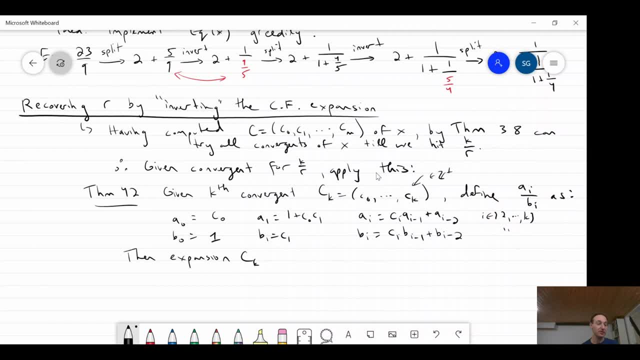 So in particular, then the expansion CK. So in particular then the expansion CK. so if you really take the full expansion, then it's equivalent, or any partial expansion to AK over BK right, to AK over BK right. So if you cut the expansion basically at any point, 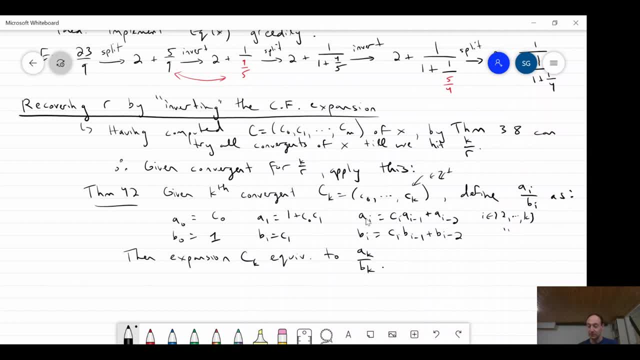 that will be equivalent to the fraction. you know, whatever point you stopped at, let's say AI, it'll be AI over BI, whatever that fraction is okay. So, basically, this gives us a way to you know. So, basically, this gives us a way to you know. 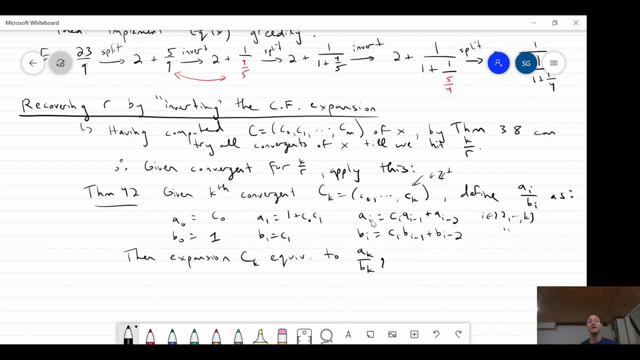 even a continued fractions expansion to recover the ratio to which it corresponds. and AK and BK. if you stare at the proof long enough, you'll see that they're actually co-prime. Okay, so AK over BK is in lowest terms And that's exactly what we wanted, right. 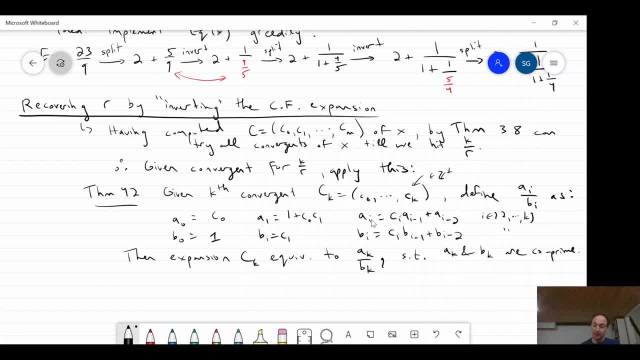 Because, remember, we assumed. we assumed that K over R was in lowest terms, right, K and R work. we assumed that they're co-prime And therefore you know if I have the continued fractions expansion of K over R like this or sorry. 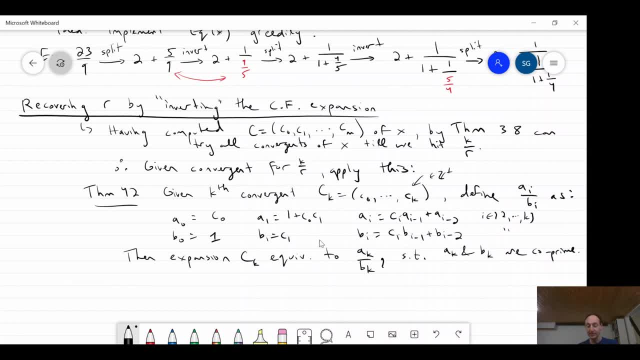 whichever conversion, it was this one, then I can apply this theorem. I could just invert the sequence C zero to CK to recover basically K over R And in particular I won't just get K over R, of course, I'll get both the numerator. 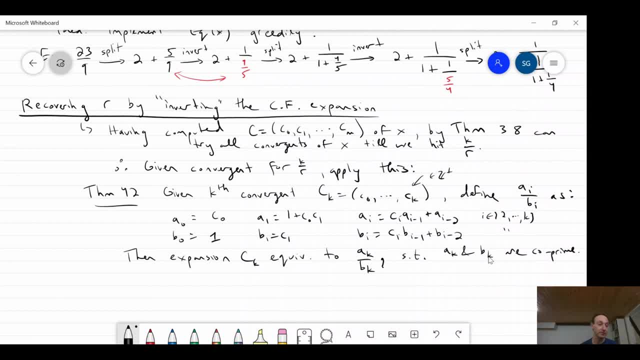 and the denominator separately, It'll break them apart for me, okay. So so by combining theorem 38 and 42 can recover K and R from K over R. Okay, that's the trick. Boom, all right, that's the full factoring algorithm. 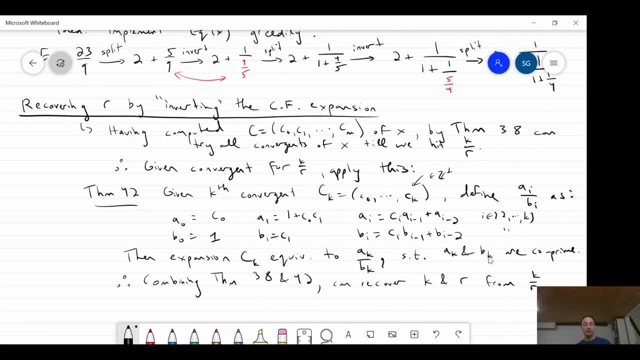 from beginning to end. okay, So just to quickly recap, we started with reducing factoring to order finding. then we used quantum phase estimation to sample elements of the form. So if the order was R, we sampled K over R, the numbers K over R. 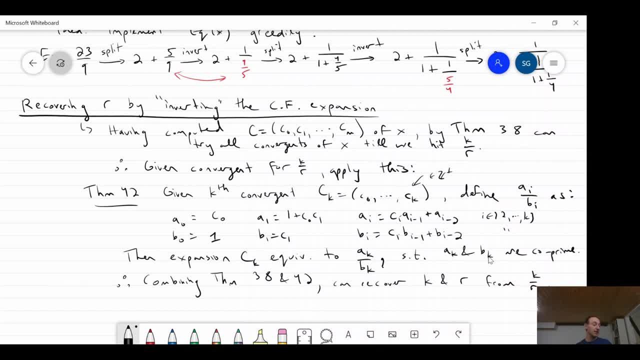 uniformly random for K between zero and R minus one. And finally, given those samples, we showed how to extract R using continued fractions. The only part of that algorithm which is quantum is just the phase estimation. Everything else is classical. Okay, and so that is the full factoring algorithm. 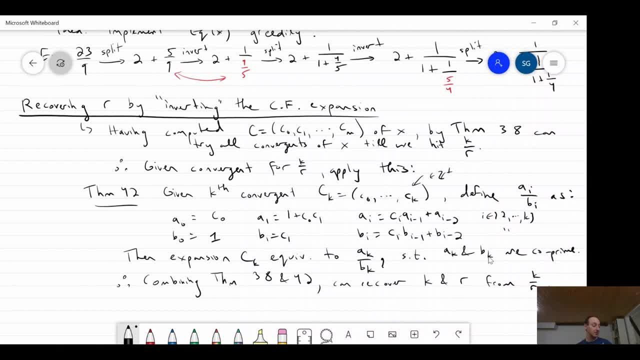 Why do we care? Because it breaks RSA. So let's just take maybe 10 minutes and wrap up the lecture by showing how factoring- breaking factoring- allows you to break RSA. okay, I mean, you can't have a full story unless you. 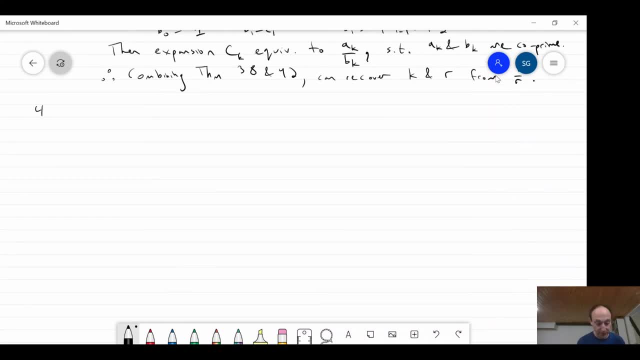 I think you see this. So that's the final section in the notes, And now we can apply this to break RSA. Okay, so you know, I'm gonna go over this briefly. I'm not gonna prove anything. That's not the purpose of this lecture, of course. 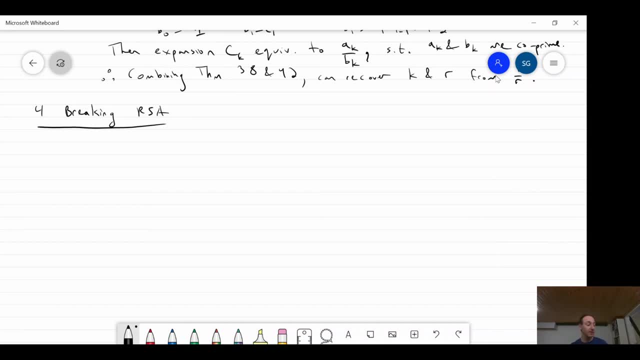 But basically, what is RSA? RSA is a crypto system, right, And you imagine that. you know you have a party, So in the notes I called her Alice, right, And what Alice wants to do is she wants it. 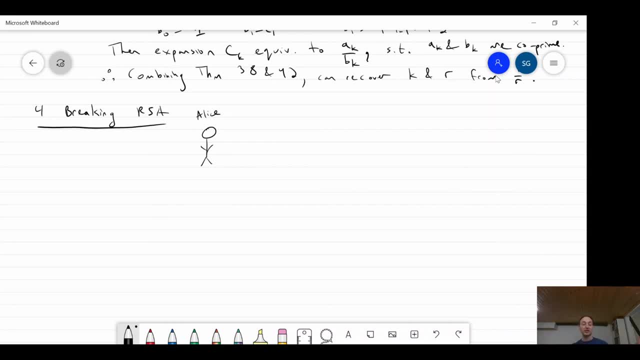 she wants to make it possible for everybody else in the world to share her secret messages, basically so that she can read the messages but nobody else other than her and that particular sender of that particular message can read that message. okay, So how do you do that, right? 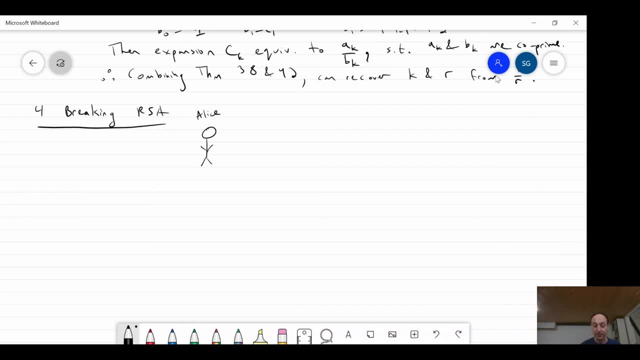 Well, what she does is she prepares, basically, she keeps the RSA. well, okay, what is RSA? It's called the public key crypto system. Okay, and what does it mean to be public key? Well, basically, what this means is that the scheme. 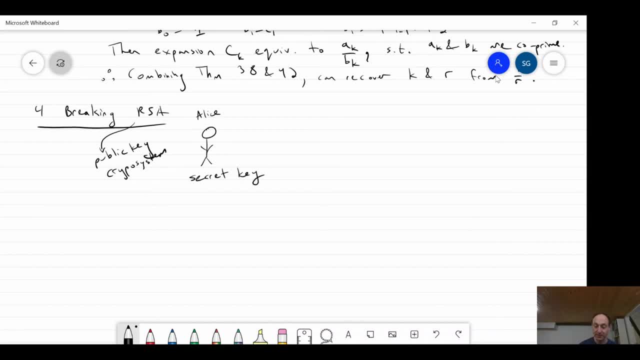 will consist of two things, which we'll define. There will be a secret key S that Alice keeps in her possession and this is what she uses to decrypt incoming messages, And what she will do is she will broadcast out a public key K. 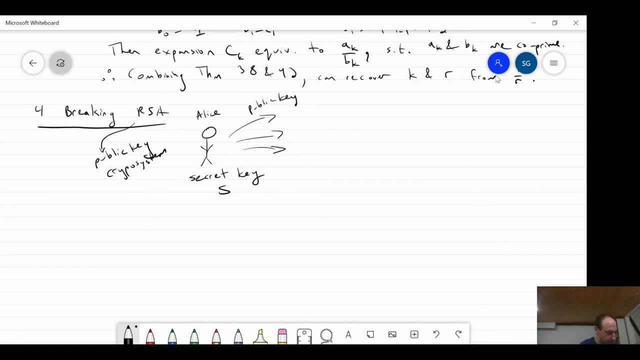 Sorry, I think I called it P in the notes, right? Okay, and so that's public knowledge. So anybody who wants to send Alice a message, they would use P to basically encrypt whatever message they have in mind and they would send that off to Alice. 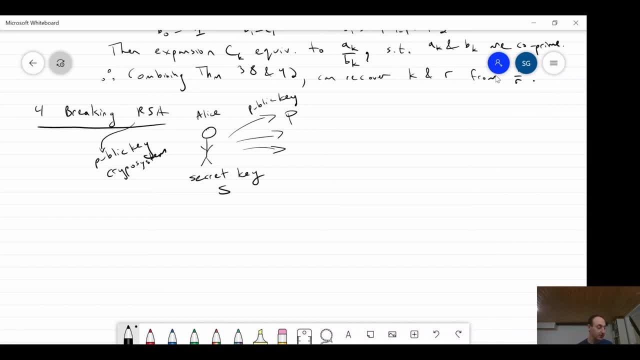 and Alice would decrypt the message using her secret key. Okay, so it's one way. in this regard, Security is kind of incoming to Alice. Okay, so let's very briefly define how RSA works, and then we'll observe, you know. 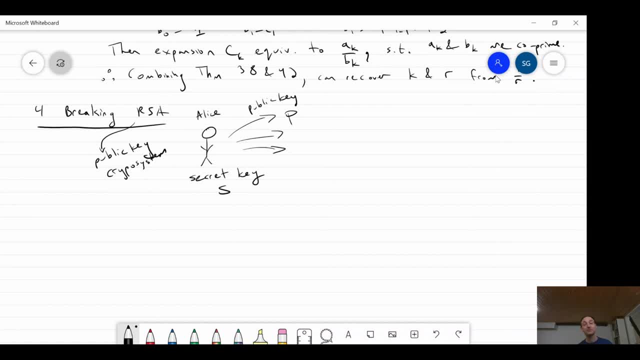 quite obviously how being able to factor is gonna allow us to break RSA very easily, So maybe I'll do A, B, C, D. So in RSA, how does Alice create the keys: the secret key S and the public key P? 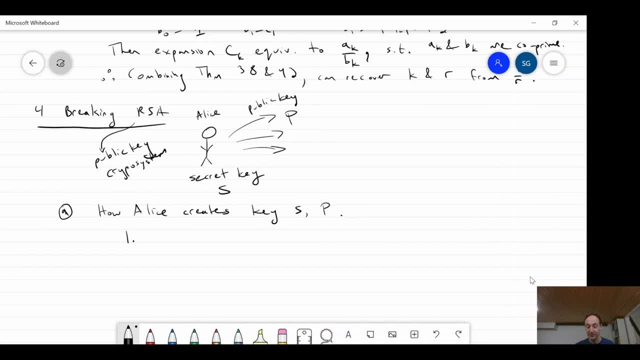 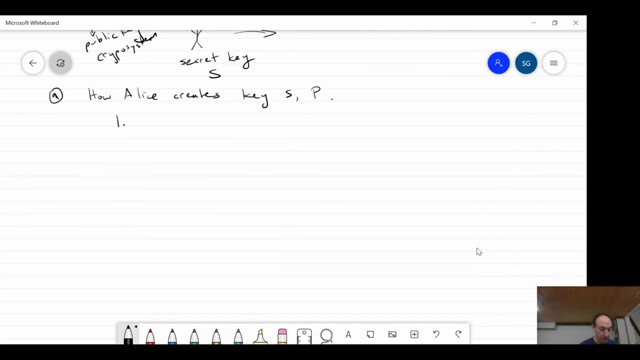 Okay, so she just follows these steps. It's gonna obviously involve modular arithmetic, just like before. Okay, so what does she do? She chooses large, distinct primes, P and Q, and she computes N equals PQ. Okay, so this is why we were talking about factoring. 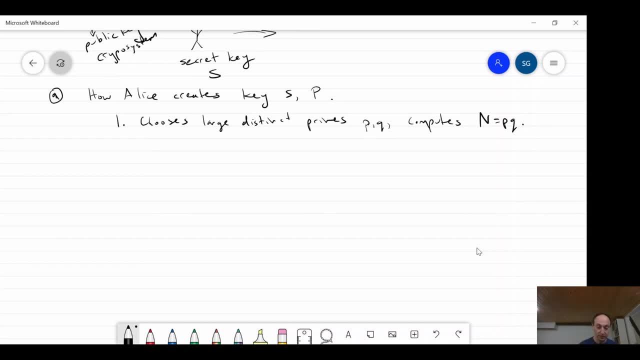 integers N, which are a power of just two primes. So she randomly chooses a small odd element, E, of the integers, which is co-prime to this funny thing. So P minus one times Q minus one, okay, And so she knows P and Q. 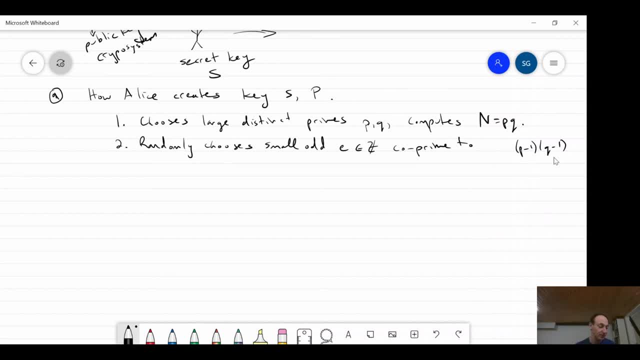 So she can also compute, you know, the product of P minus one times Q minus one. Let's just give this a name. The name is phi of N. Okay, I guess I could have more accurately written phi of PQ. And you know, given E, what she can do. 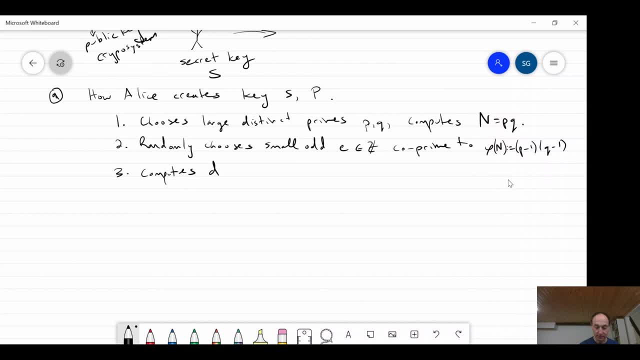 she computes the unique element D, because E is co-prime to that thing. there should be a unique. do I want to call it phi? Just be consistent with my notes. yeah, So she computes a D satisfying E times D is equivalent to one. 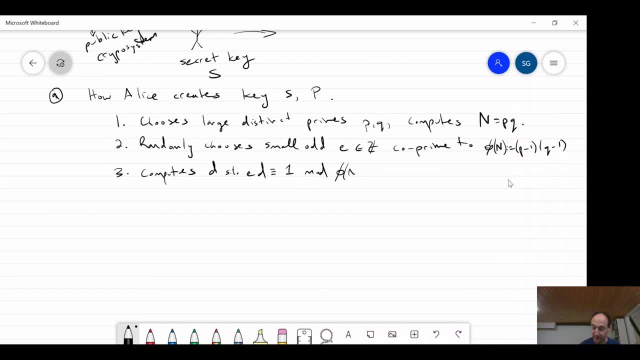 mod. you know this funny phi of N that we defined here. What in the world is this? Okay, So modulo this thing. So basically she computes the inverse of E mod, phi of N, Okay, and that's basically it. 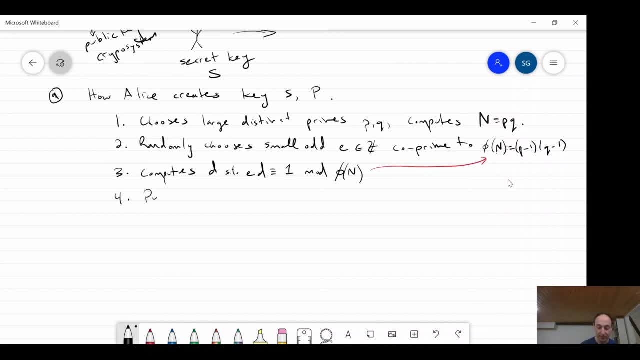 Now the question is: what's the public key and what's the private key? Well, she publicly releases the public key. the public key, which is it consists of two things: N is public right, That's the thing that we want to factor. 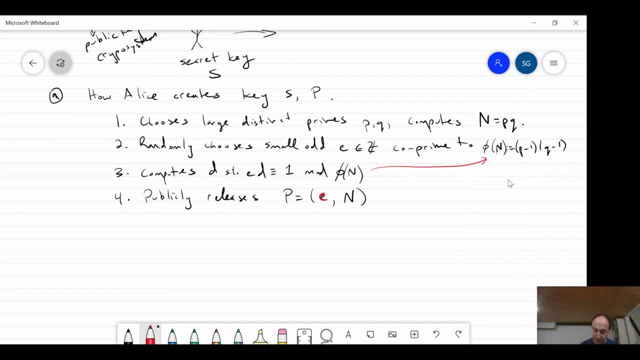 And the public key is E, right, So maybe I'll do this in red. This E was chosen here, right, And she privately stores S, which is equal to maybe I'll. I don't know why this thing's not switching colors. 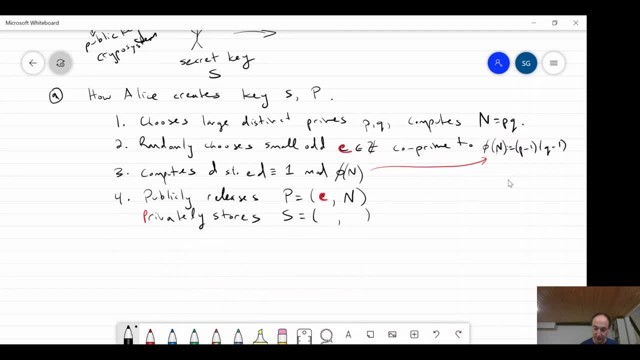 There it goes. Okay, She privately stores N again. I mean, N is public anyway, You don't actually need to store it, of course, in that regard. But she stores that and D, right, And so that's D, and you know, here was D over here, right? 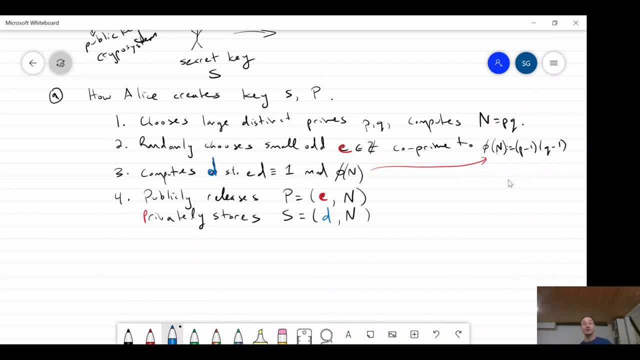 D was in step three, It was the inverse of E mod, this phi of N. Okay, so what is the trick to all this? right, The trick to all this, intuitively, is that you know N is public knowledge, but kind of the key. 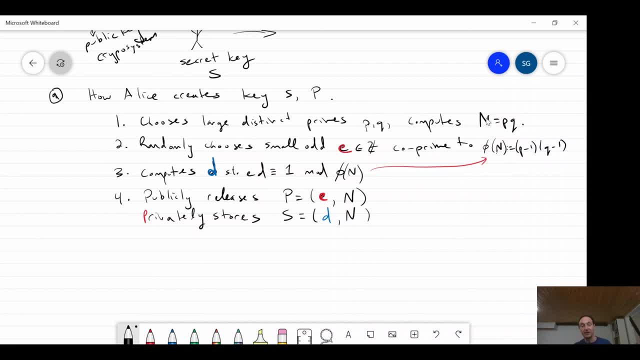 to really getting under the hood of the scheme is: you don't want N, right? You don't want P times Q. You actually want P minus one times Q minus one. This is really what you want, right? This phi of N. 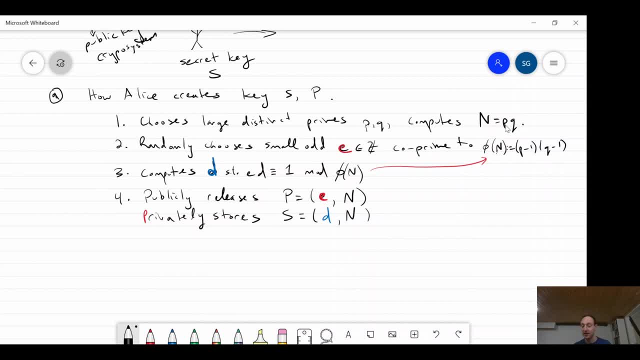 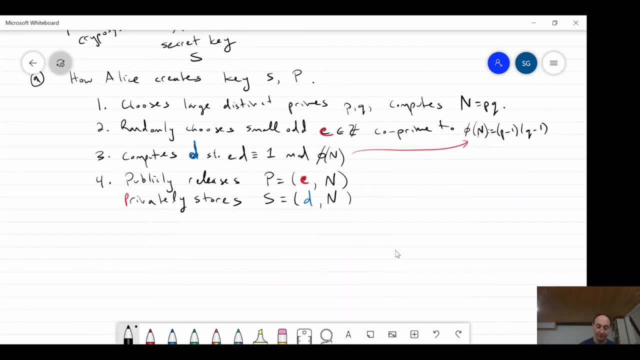 You want to get your hands on that? okay, And so, given just N, it's not clear how to compute this thing. That's, intuitively, why this is believed hard. We'll talk about this briefly in a second again. Okay, so that's how she creates the keys. 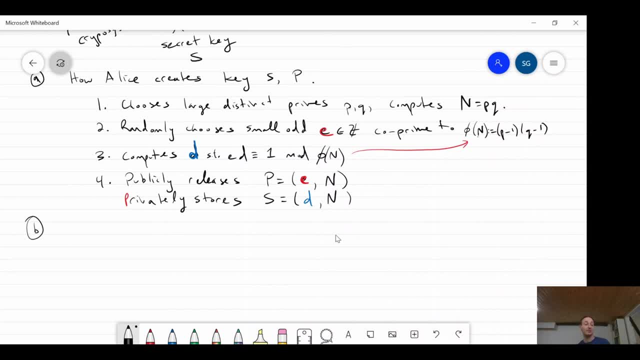 And now let's see how a member of the public encodes a message to Alice, How the public encrypts a message: oops, using your public key, P. okay, So suppose Bob wants to encrypt some string, right? So it's a string of zeros and ones. 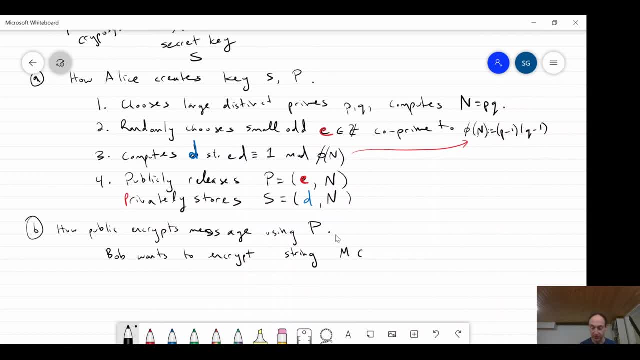 and that means he'd also think of it as an integer, of course. So he wants to encode the string, and the string needs to be at most log of N bits long. And you know, exercise 44 gets you to think about. 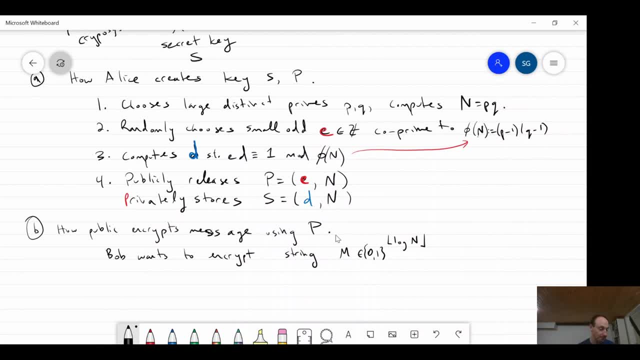 why that's an upper bound, given kind of the parameters I've chosen so far. Okay, and what does he do? He computes. So now let's think of M, naught as a string, of course. Just think of it as the integer that that string represents. 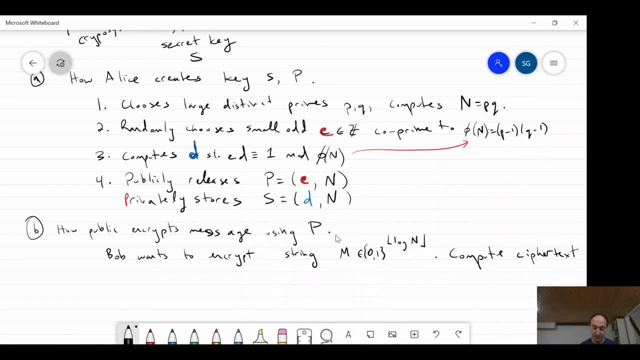 So he computes the ciphertext or the encryption, And then he encrypts the text as follows. So M is the message. so we'll define the ciphertext as E of M And it's very simple: square multiply, right. 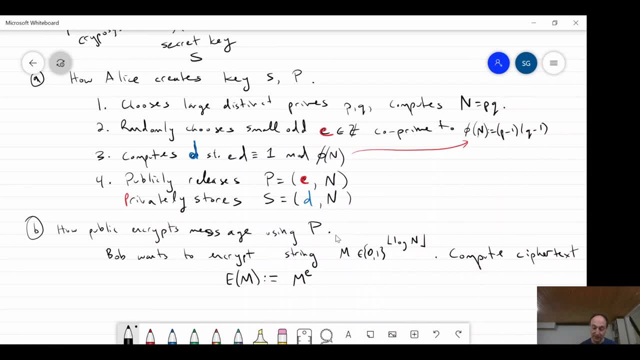 Takes the message, raises it to the power. E remember, E is coming from the public key, right, It's over here, that's E right there. So E is coming from the public key. and then, of course, mod N. 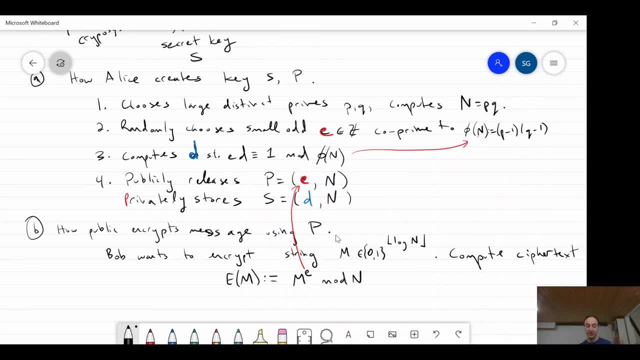 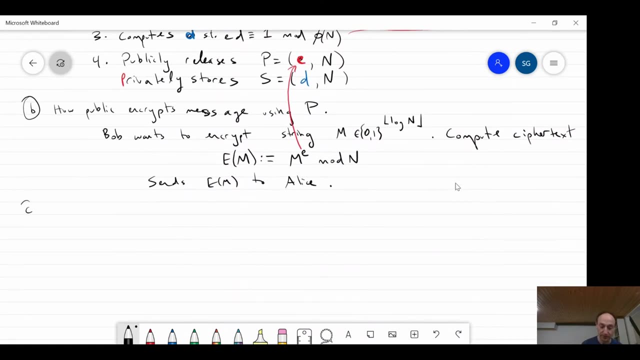 Okay, so E and N were parts of the public key and M is his own personal message, okay, And then he puts it in the ciphertext, right? And then he just sends E to Alice. That's how Bob encrypts a message to Alice. 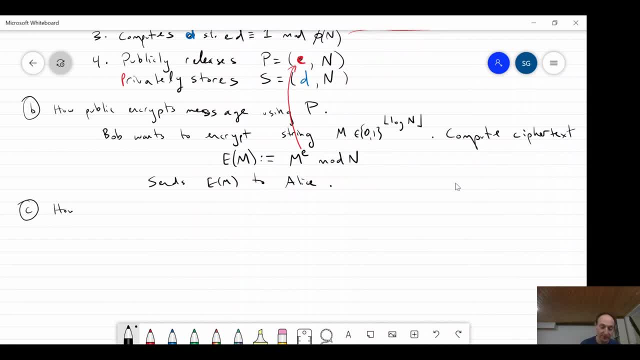 There's nothing to prove there, that's just a fact. How Alice decrypts now, given her secret key. there is a bit of a proof required here, which I'm going to skip, And ciphertext: E. So what does Alice do? She takes E. so that's what Bob sent to her. that's a sum string or an integer if you like. 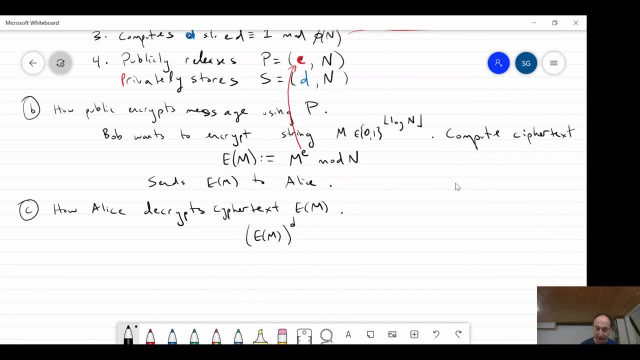 and she raises that to the power d. Remember, d is her secret key right over here. that's this thing over here, That's part of her secret key And mod n. And then takes a mod n And this: the claim is that this will allow her to recover the message n. 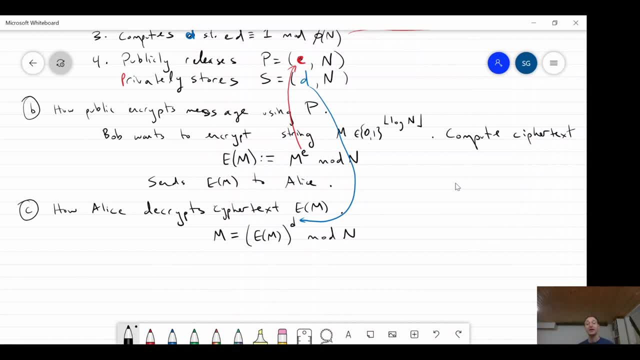 If you take the encoded thing, you raise it to the power d again square and multiply mod n, you will recover the message perfectly. Again, I'm not going to prove this. it's not too difficult. it takes a couple of lines. 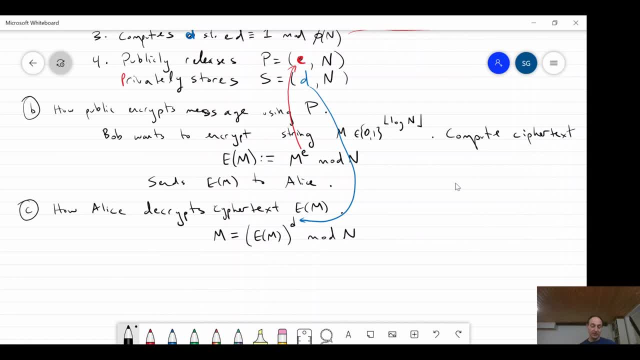 but let's not sidetrack from the story here. So the point is that this is how the keys are produced, this is how a message is encrypted and this is how a message is decrypted. So the last thing we care about- the purpose of this whole lecture. 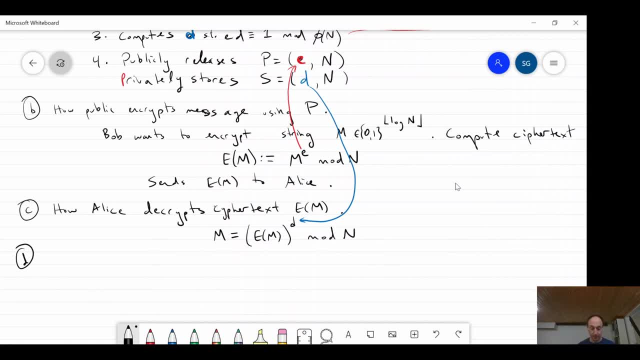 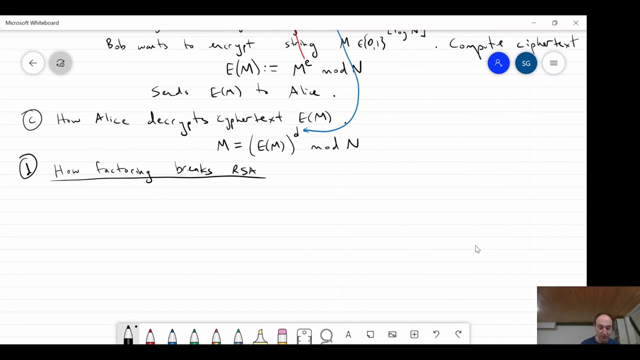 Is how do we break the scheme? So how factoring breaks RSA. So let's assume there is an adversary. we've got to give this person an eve, so we'll call this evil person eve. Sorry, we've got to give him a name, so we'll call this evil person eve, right. 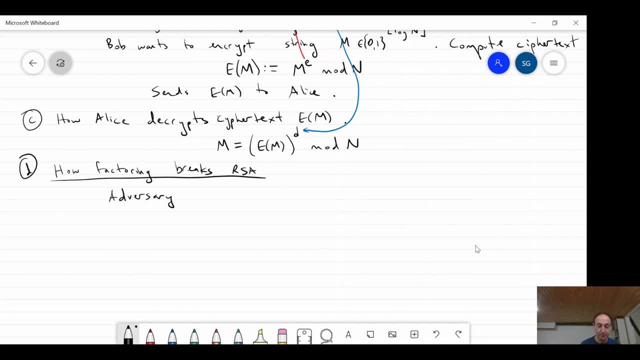 So let's suppose I have an adversary Substitute whatever name you want. Okay, Whatever name you want Can factor. remember the public key was n and e. so can factor n equals pq right into the primes p and q. So suppose they're able to do this. they have a quantum computer, say okay. 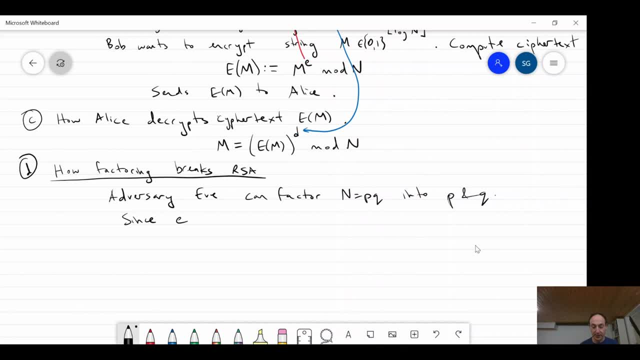 So, since e is public knowledge, right, that was part of the public key. the public key was both this capital n and this little e. She can herself, she can recompute the only other missing parameter, which was, you know, e times. d was supposed to be equivalent to 1 mod. this funny phi event, right. 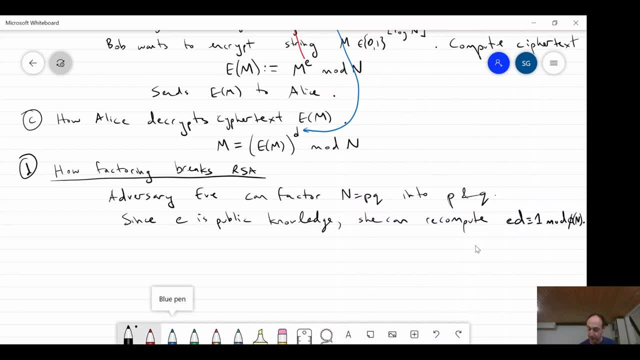 So she herself can, she can recompute d, sorry, So that's sitting right here, Okay, Thus obtaining, Okay, Okay, That's obtaining basically the private key, which is s of d comma m. Okay, So you know, let's quickly scroll up right. 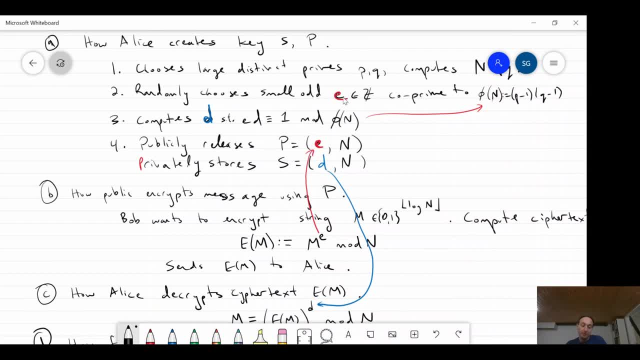 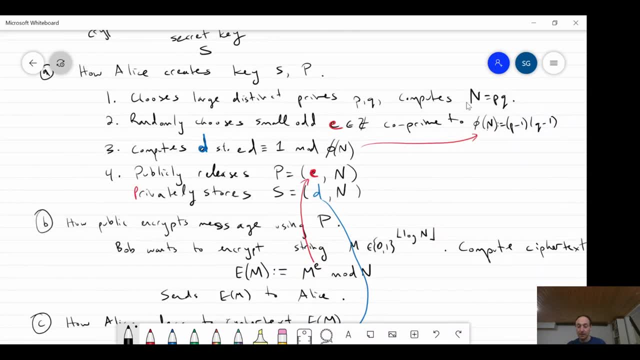 So what happened here is: remember, Alice picked this random element, e, That was publicly announced right, And so was capital N, And so basically, but since eve knows not just n but given n, she's able to recover p and q, that means she can compute. you know this funny phi event. 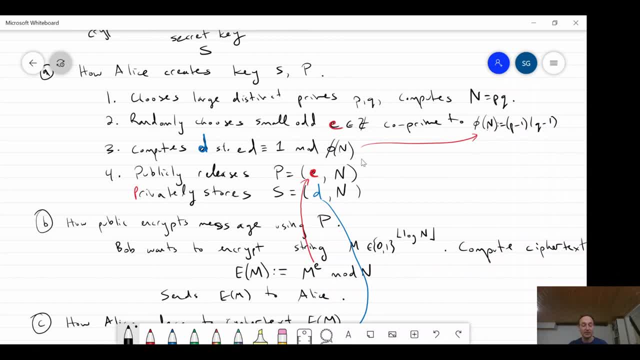 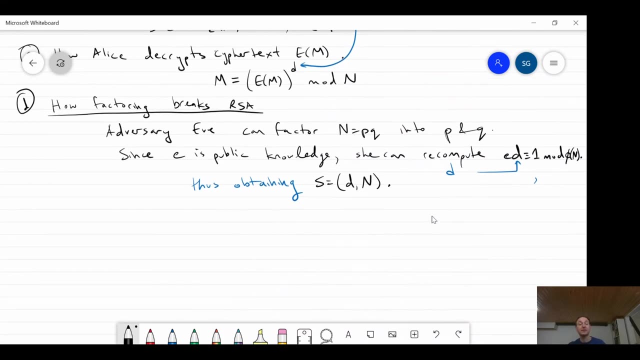 And she knows e. That means she too can execute line three, just like Alice did. right, She can compute this unique d, And that means she knows not just the public key, but also the private key. She knows d, And so what that means is that, of course, she can not only decrypt any incoming messages.